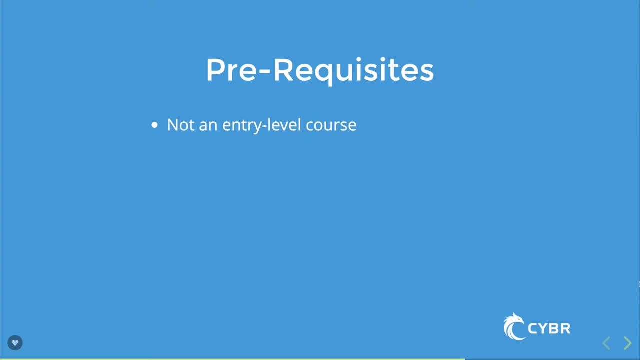 started in IT. To fully understand the concepts and attacks you have to have a basic understanding of web development, and SQL experience is definitely a plus, although we will cover the very basics of SQL just in case you're rusty and need a reminder And if you've never touched. 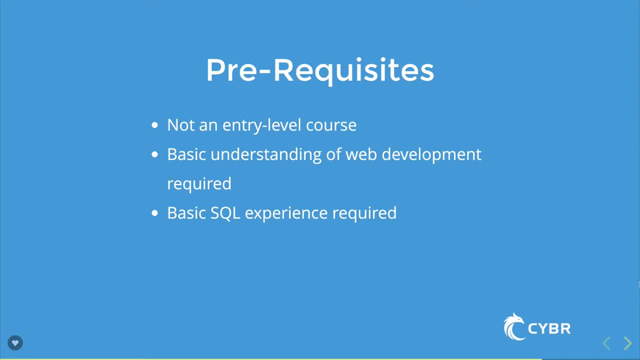 code before, or you don't understand the concepts of a web application, including HTTP requests like GET and POST. you will struggle to understand this course and I do recommend that you start there first. Now, a great language to learn is JavaScript, so I'd recommend that you pause here. 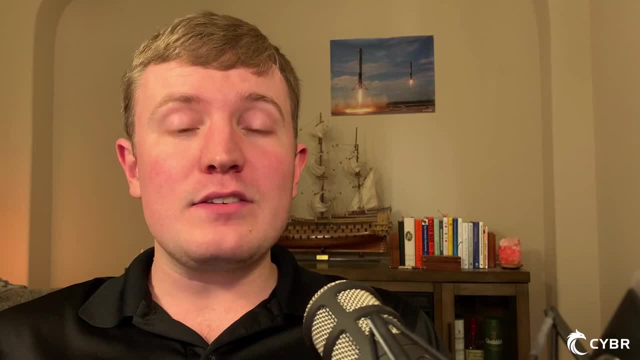 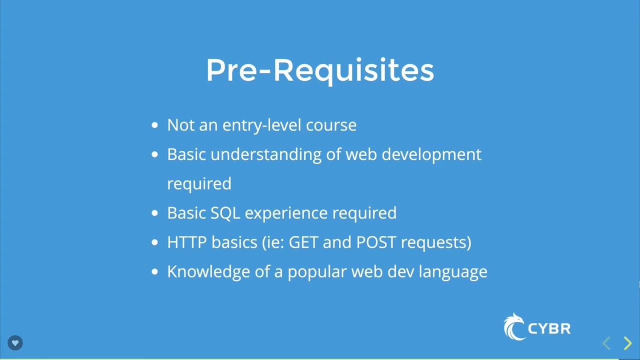 go find a great JavaScript course and then come back once you've at least set up that JavaScript web application connected to a database. You don't have to be knowledgeable in any specific programming language to be successful in this course, but, again, an understanding of 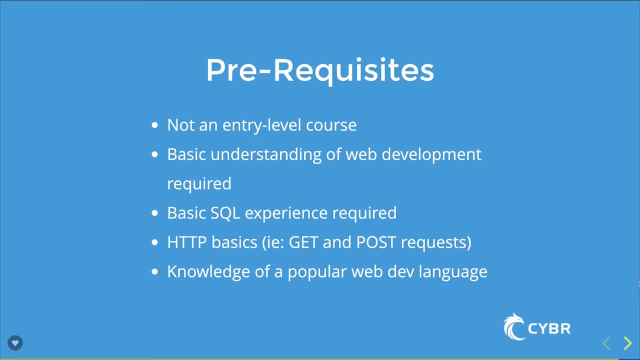 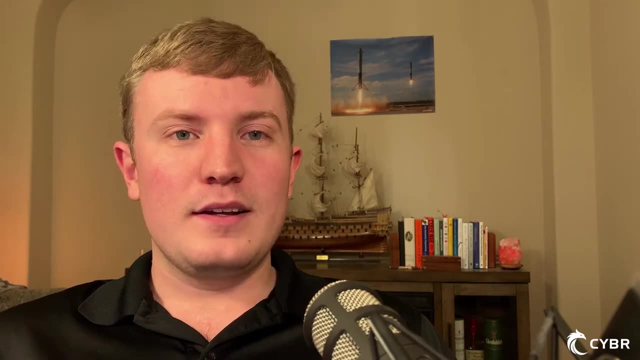 JavaScript or PHP or really any other popular web language will definitely help. Otherwise, if you're still listening, then I'm excited to have you here and to continue on with this course Now. in the rest of this lesson I will be talking more about my background and who. 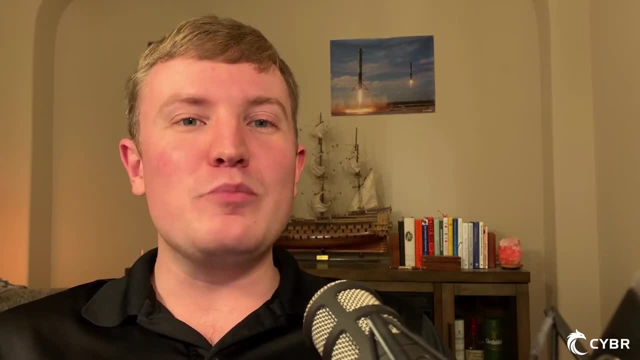 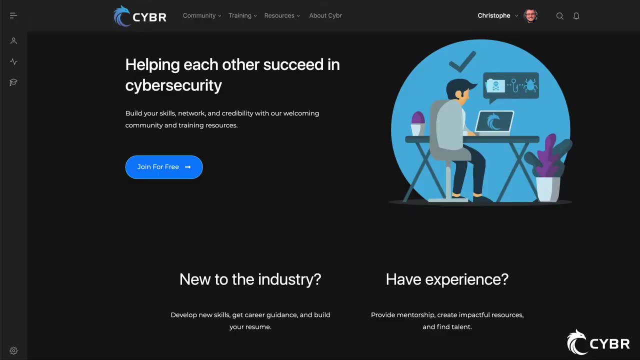 I am, so if you've already taken lessons from me before, you can go ahead and move on to the next lesson, since you've already likely heard this story. But otherwise, I'm a co-founder of cybercom, where we've built a cybersecurity community with training resources, and I first got started in IT. 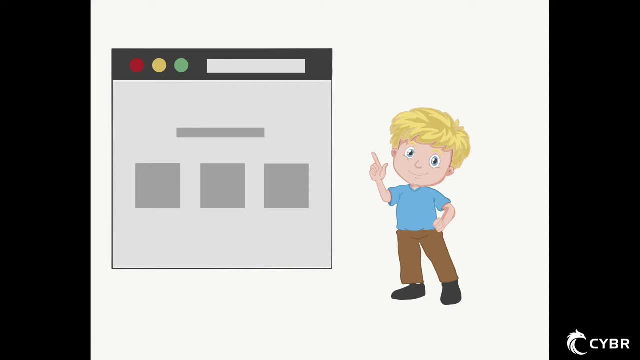 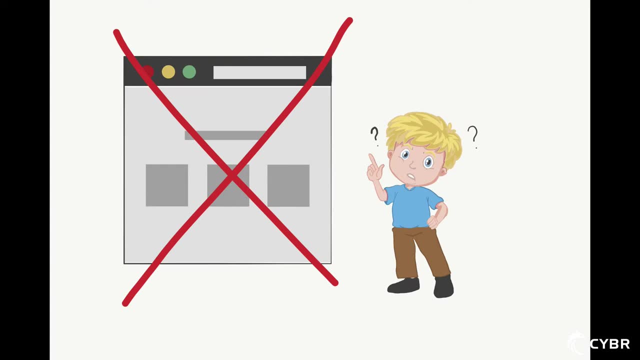 after setting up websites for video game clans, And these clans made a lot of competitive enemies, so our websites were constantly getting attacked and compromised and we had to learn how to defend them. Now, nothing serious came of it, thankfully, since we were just teenagers, but I absolutely. 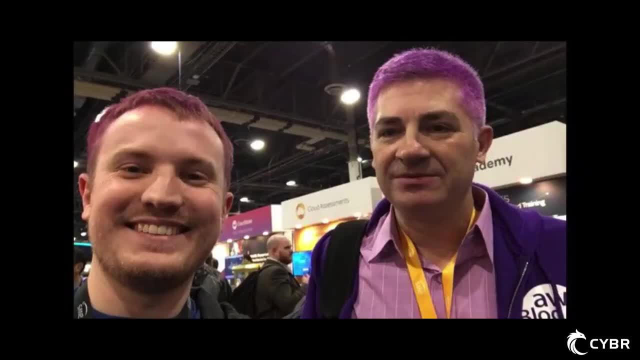 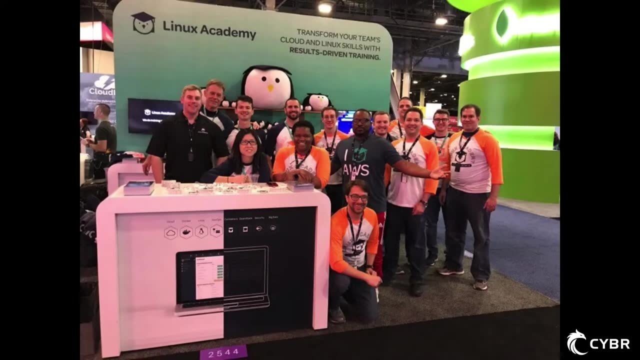 loved it and immediately got hooked into it. Fast forward a few years and I jumped on the cloud computing train that was really starting to take off. I joined a fairly small online training platform at the time and helped grow it into a leading cloud training platform. 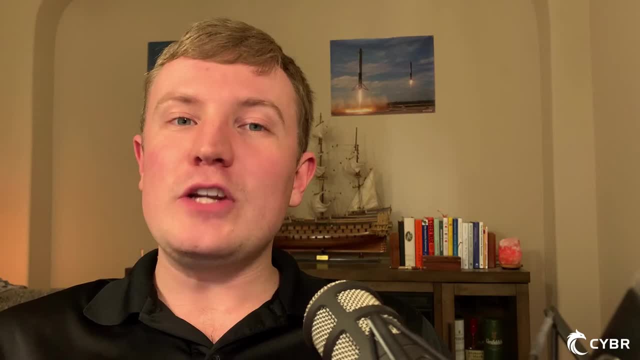 before I was able to get into it. So let's get started Before we were acquired in 2019.. Along the way, I couldn't help but notice a similar challenge that organizations and individuals were facing, with the constant news articles announcing large 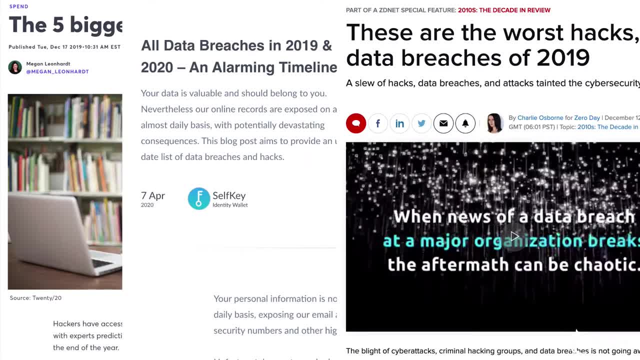 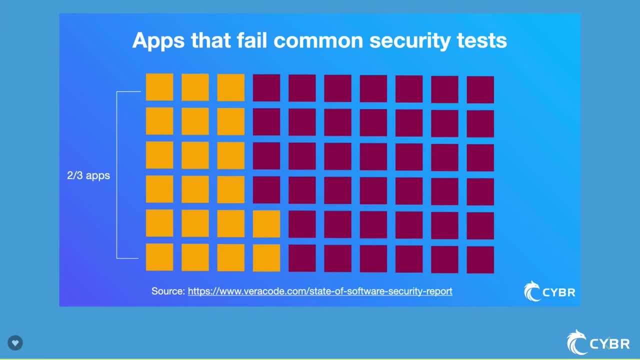 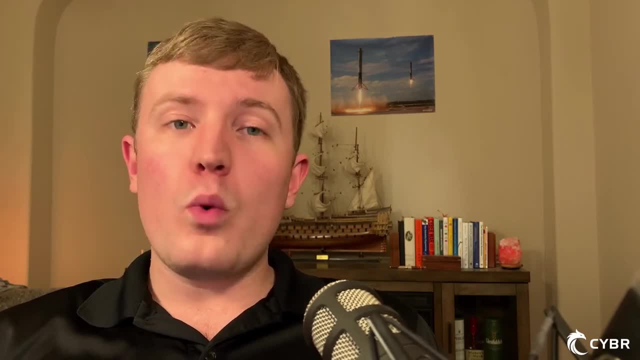 scale hacks that were oftentimes caused by simple issues, And after doing further digging on the state of web and application security, it was quite shocking to see how many applications currently in production have known vulnerabilities. There are a number of reasons for this and not one simple solution, but one thing is clear: We need more. 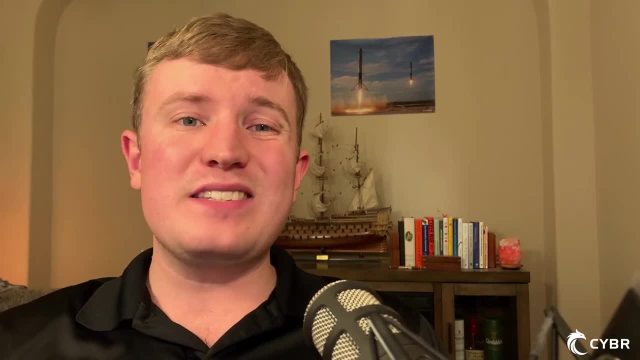 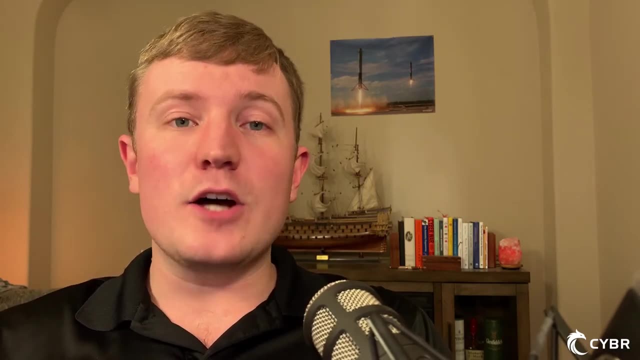 developers, who are empowered to learn about the risks facing their web applications today, because if they're not familiar with those risks and how to defend against them, then they'll likely end up on that long list of vulnerable applications and perhaps, even worse, they'll end up in the news. 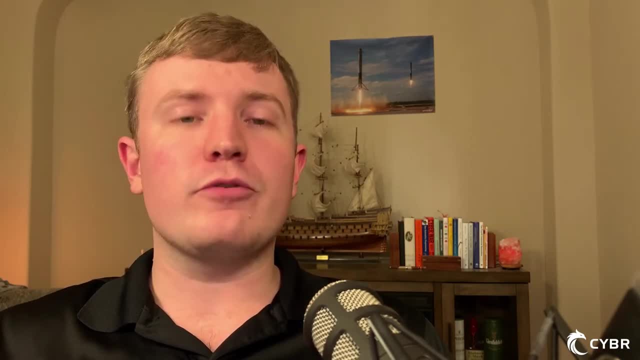 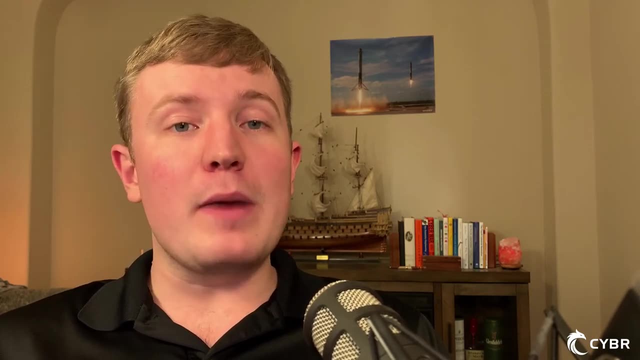 So, all that to say, I've always had a passion not just for IT, but also for helping people learn and helping make the world a more secure place, And this course is built from my years of experience in working with web applications and architectures and software development. I've been working with a number of companies for a long time. 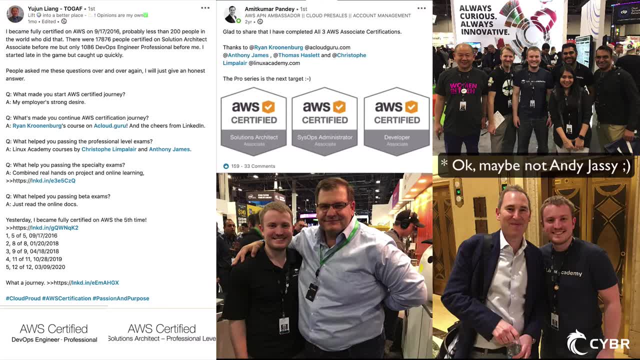 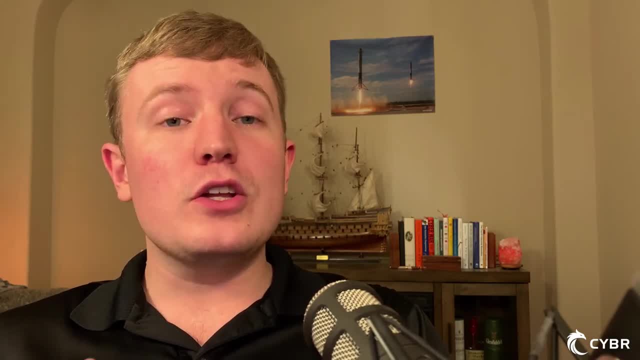 and I've been working with a number of companies for a long time of training individual engineers, IT managers and executives at companies, large and small, And hours upon hours of research that I've compiled for you so that you can learn in a safe 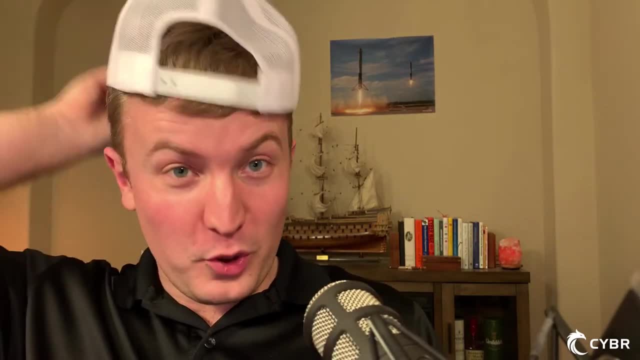 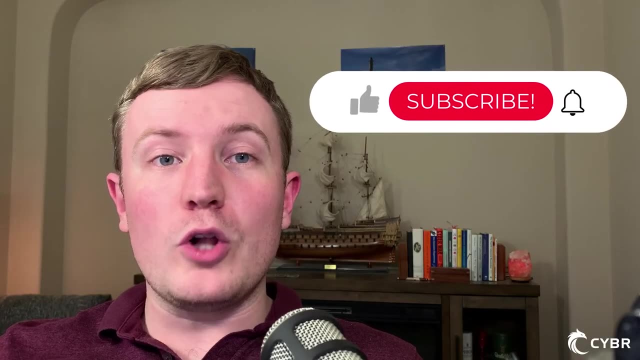 practical and engaging way. So strap in, put on your white hat and let's get ready to do some ethical hacking. In this lesson, we walk through setting up an environment in order to follow along with our hands-on demonstrations throughout this course. 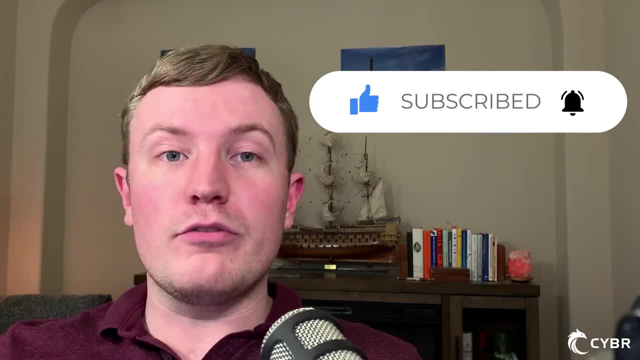 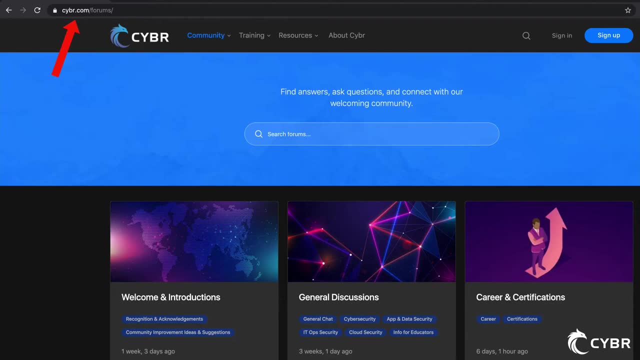 And this is a lesson that is important to complete if you plan on following along with our hands-on demonstrations. So if you get stuck at any point in time, please reach out and we'll help you resolve the issue so that you can move on. 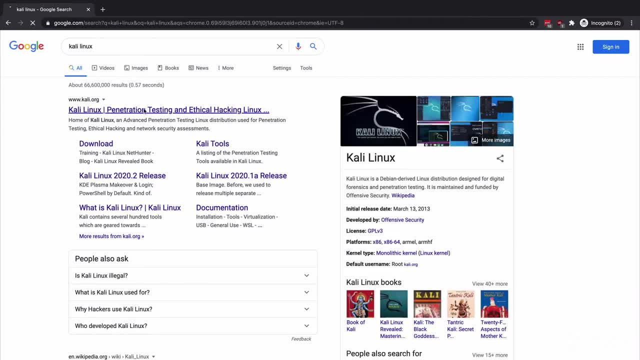 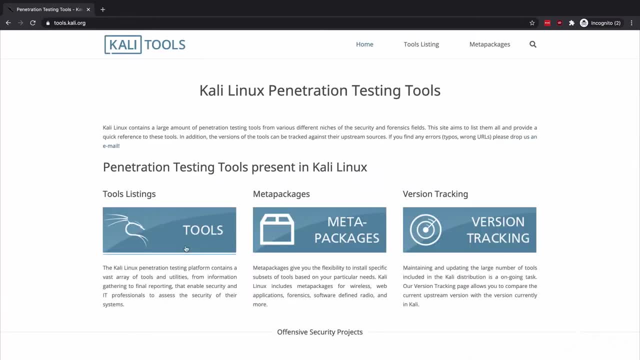 Now, the first thing we need to configure is Kali Linux, which is a free Linux distribution that's often used for digital forensics and penetration testing, And the reason that we want to use Kali is because it comes pre-installed with many of the tools that we'll be using. 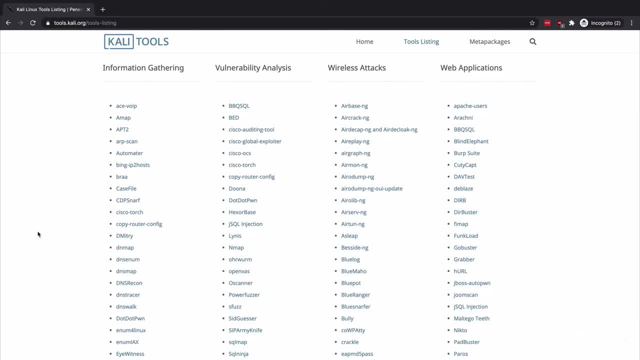 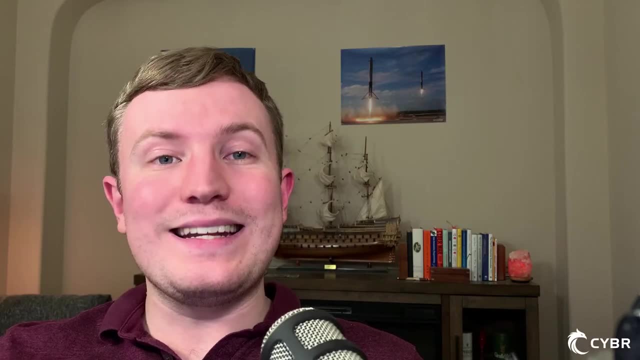 throughout the course, which will help us get going and avoid issues that can come from running different operating systems. And if you don't already have VirtualBox or VMware installed, go ahead and download those, and I will be using VirtualBox. All you have to do is go to VirtualBoxorg and download the latest version for your 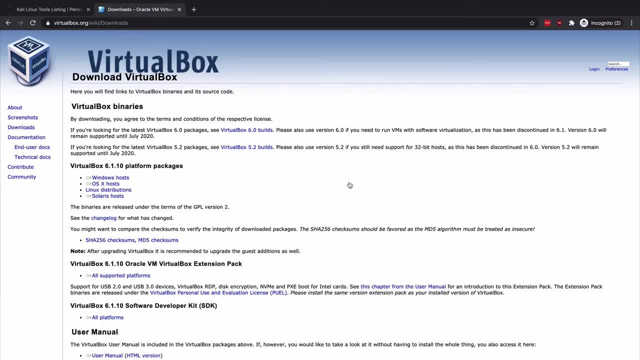 current operating system. Now. I'm on a Mac right now, so I'll download the OS X version, but if you're on Windows, you would download that version. Then follow the steps to install VirtualBox Now at this point. if you have any issues during the 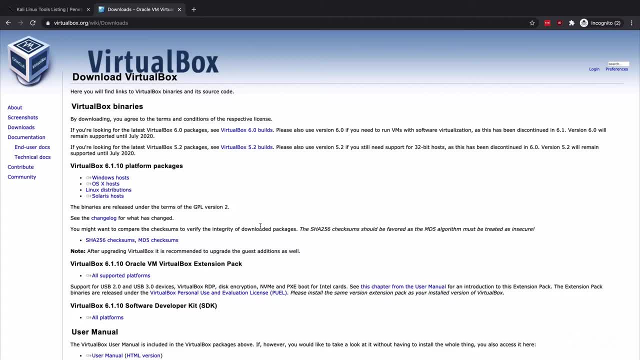 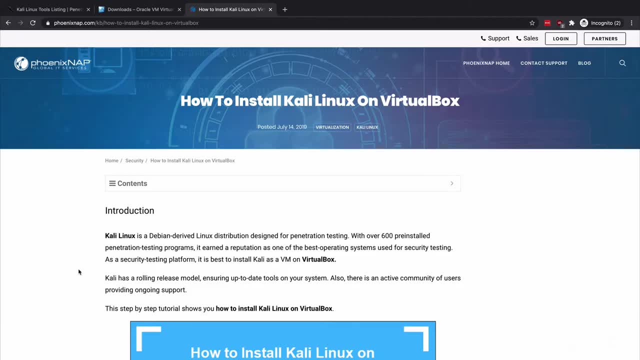 installation and you can't figure out a solution, please reach out in our forums and we'll be more than happy to help. And once you have VirtualBox installed and running, it is time to set up Kali Linux, And there's a great tutorial located at this URL with instructions, so I won't go into. 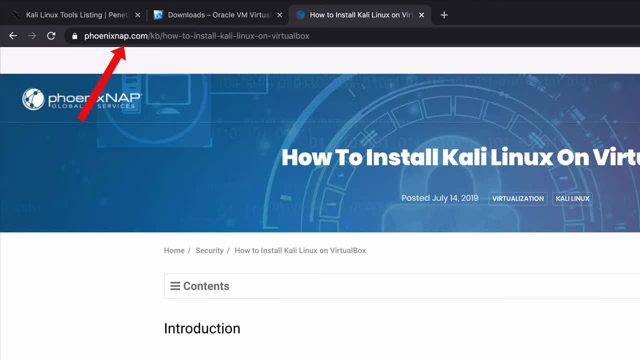 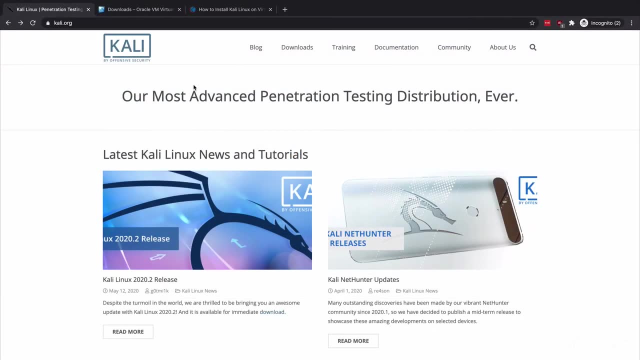 too much depth if you want to install Kali using an ISO, which provides a bit more customizability, but it does take longer and it does require more configurations, So instead I'll use an OVA version. First, we'll want to download Kali at this URL, and if you want an ISO image of Kali, 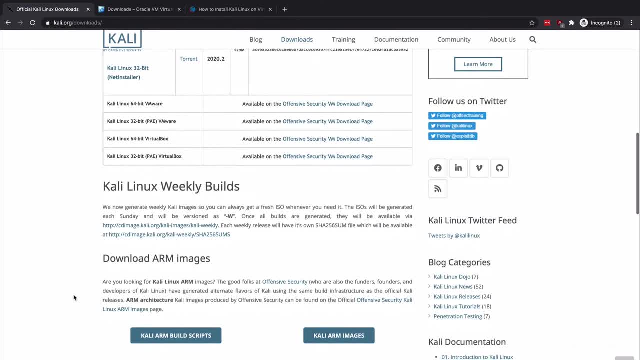 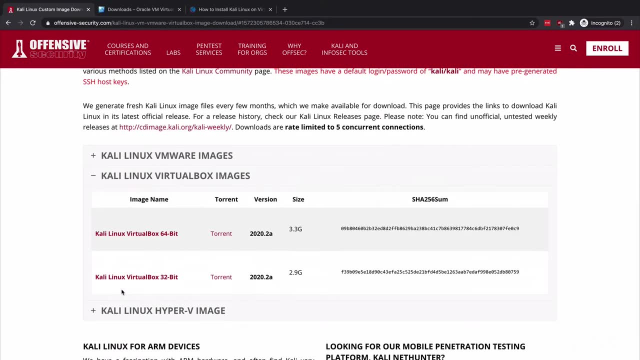 to be able to boot from it, then you can download it from here. but since we're using VirtualBox, we'll need to click on this link And we'll download the 64-bit version, and this can take a few minutes depending on your internet connection. 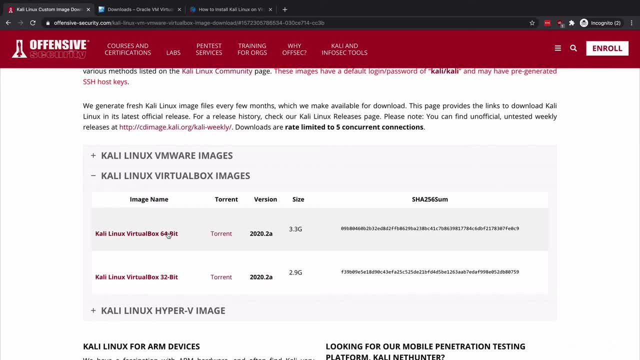 so I'll go ahead and fast forward Now. the main difference between OVA and ISO is that OVA will import Kali into VirtualBox instead of installing it, as if we were inserting a CD version of Kali. This is a very simple way of getting Kali up and running without having to. 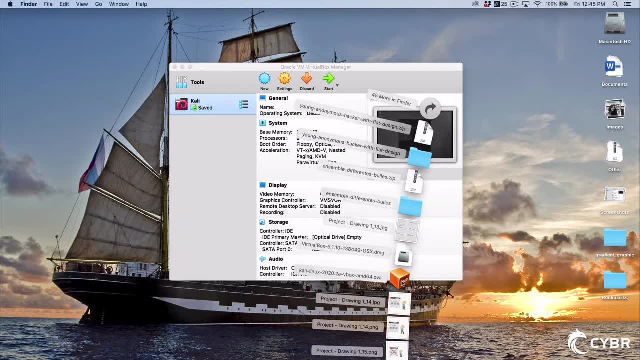 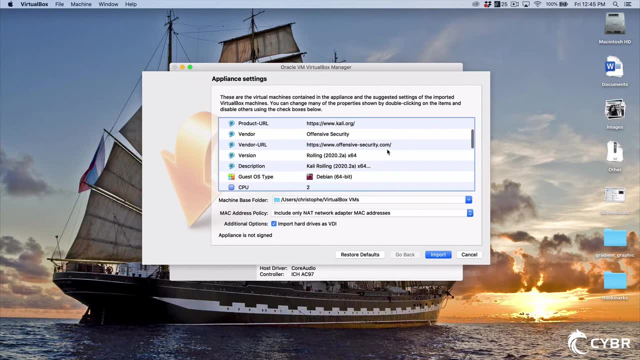 configure a lot of things And, as we import it, we'll want to check on some of the configuration settings And we can see information about the virtual system, such as the name, the product vendor, guest OS type and other important information. 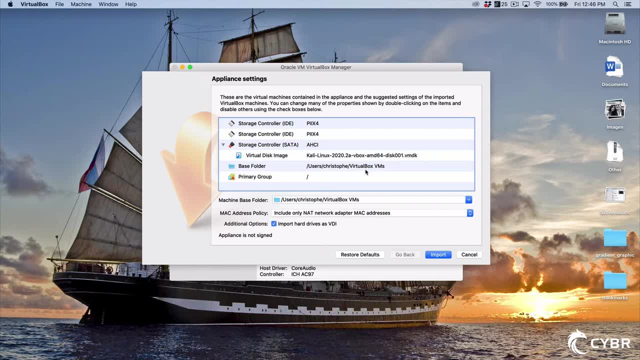 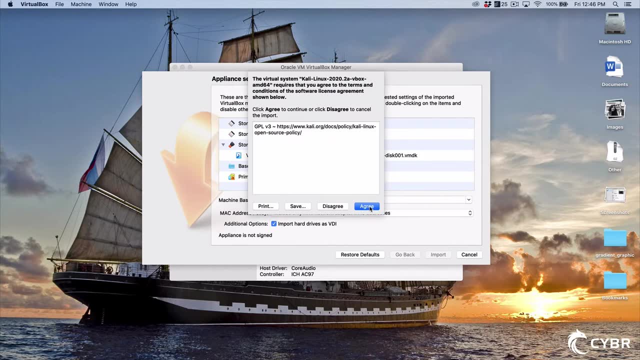 We can make some modifications here if we need to, but at this point I don't need to make any modifications, so I'll go ahead and click on import. I'll agree to the terms of service and software license agreement and it will start the import. 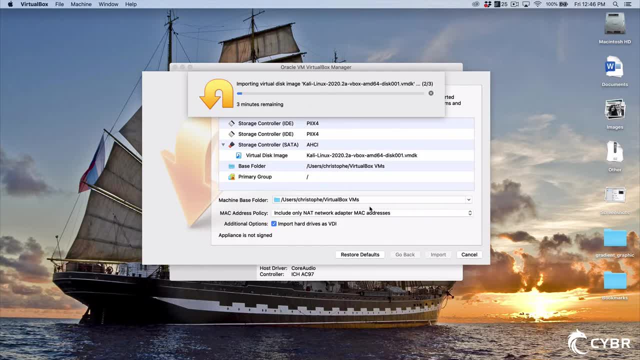 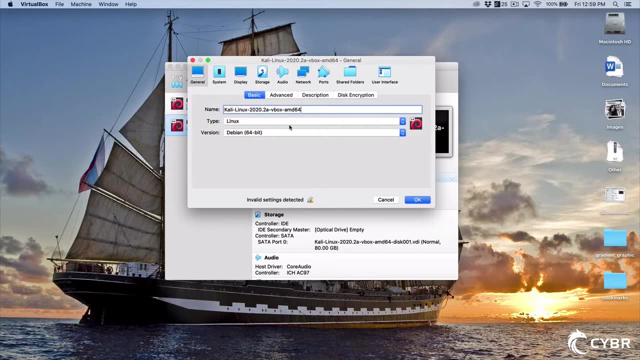 process. Now, this again can be a fairly lengthy process, so I'll go ahead and fast forward And once imported, we get another chance to look at some of the settings for this virtual machine. We can rename it, we can change some of the properties here. 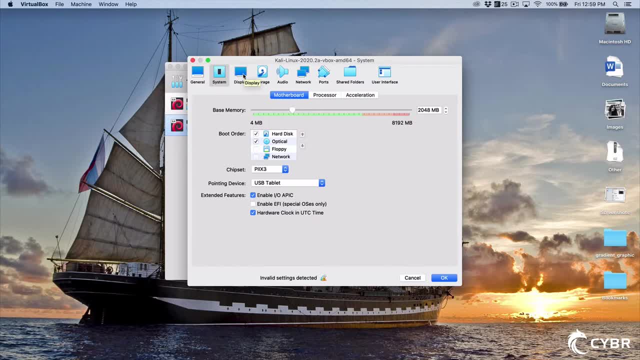 but we can also look at more important things, such as how much memory to allocate to this virtual machine, whether we or what order we want to have things booting. We can change some of the display properties, such as video memory, graphics controller and acceleration storage audio. 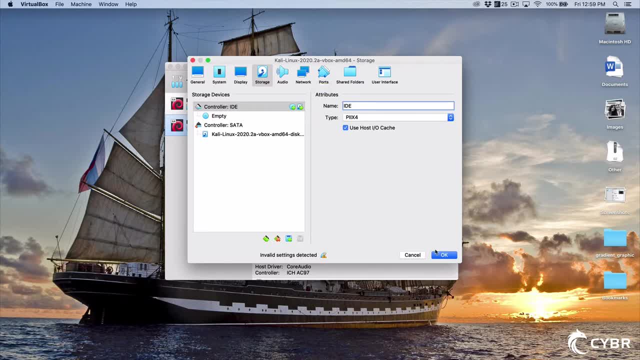 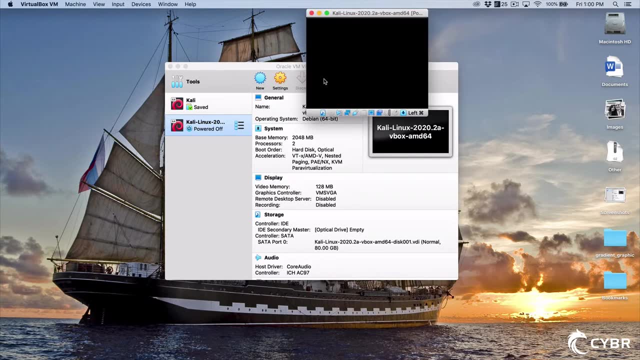 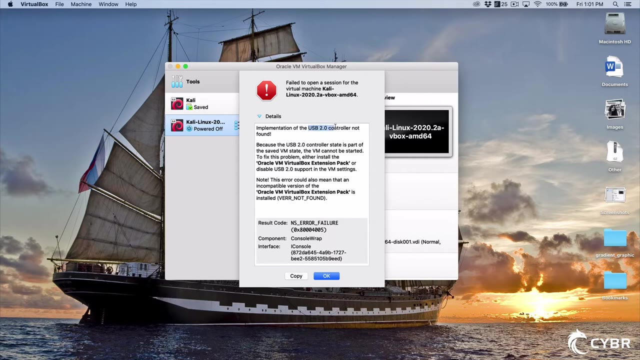 etc. At this point, I'm not going to make any modifications, but I just wanted to show you that, Instead, I'll go ahead and launch this virtual machine. Hmm, okay, since we get an error and it has to do with the USB 2.0 controller. 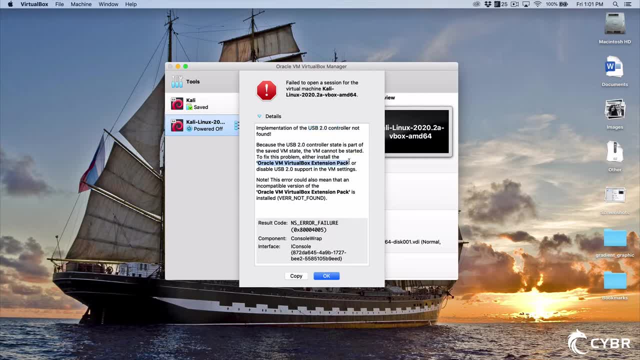 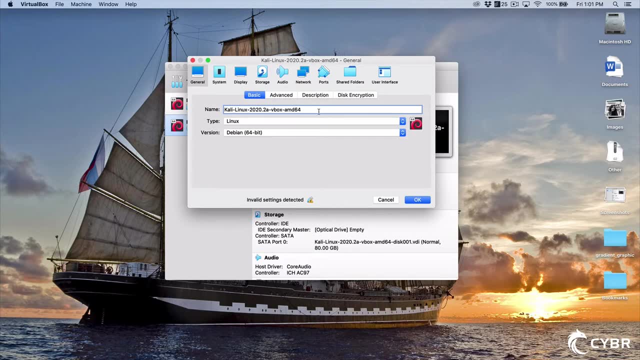 it sounds like we can either install this package here or we can disable USB 2.0 in the settings. so let me go back to the settings. This will probably be the fastest way of doing it. We can also see, by the way at the bottom here that it says invalid settings detected. 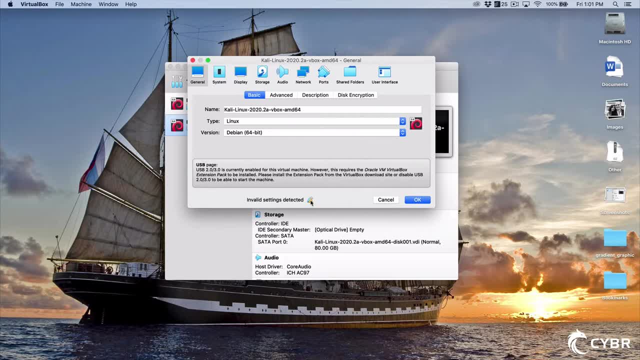 for the USB 2.0 and 3.0 is currently enabled. However, this requires that extension, so I actually missed that the first time around. So let's go ahead and disable a USB. We'll go over to ports. We have serial ports, then we have USB and I can simply do enable or check the box to. 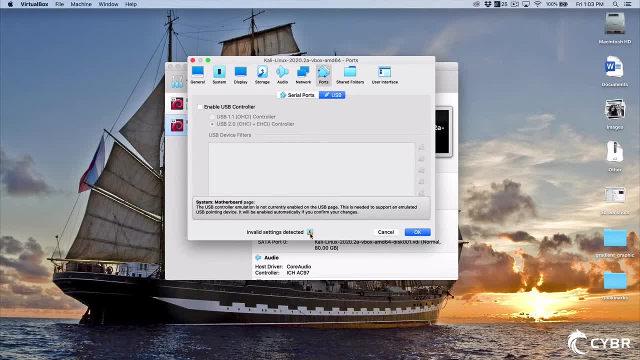 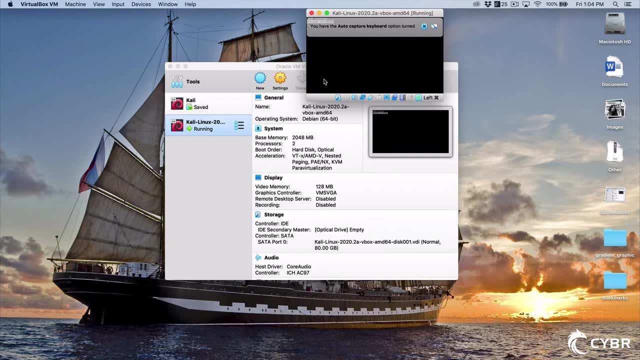 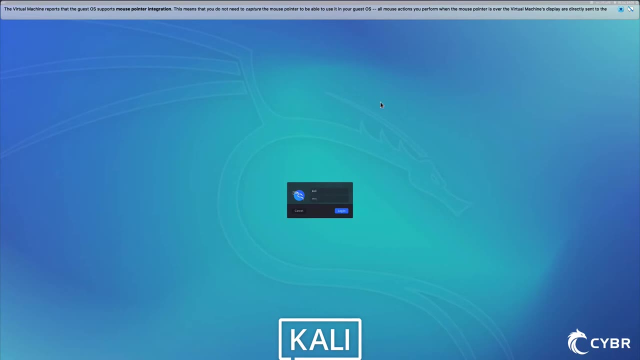 disable the USB controller. Let's check what this says here. Okay, let's go ahead and save these changes and let's try again. Okay, this time we're getting further, which is a good sign. All right, we're now asked to log in and we can use Kali and Kali for the username and password. 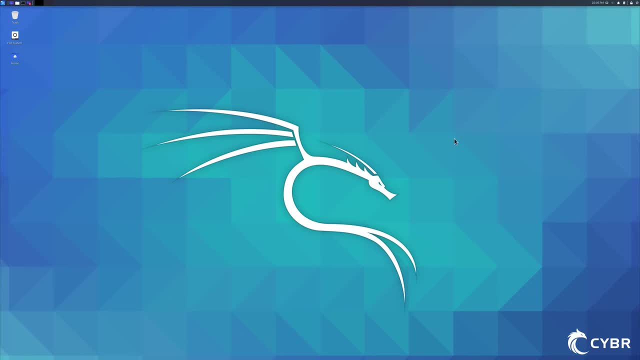 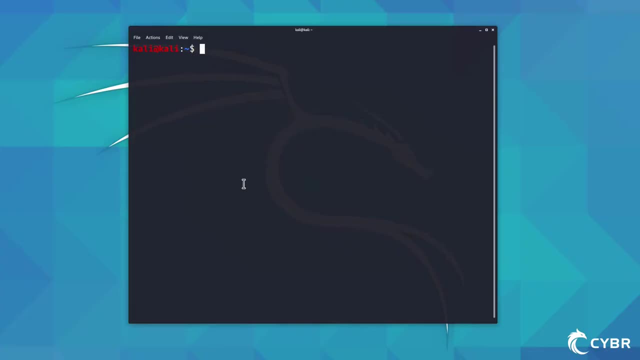 And we've successfully logged into our Kali Linux virtual machine. So the next thing I want to do, really quickly, is change the password, and we can do that by opening up a terminal window and then typing in the command: passwd. The current password is Kali. then you'll type in a new password. 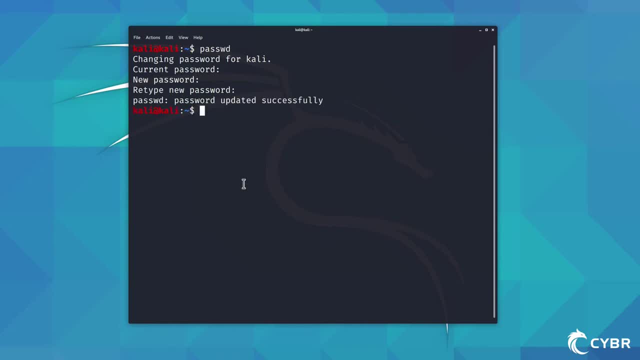 and you confirm that new password, And we're now good to go. Okay, so we're now ready to install the software that we will use throughout the course. First, we'll add a Docker PGP key, and we do this for privacy, but also for file integrity. 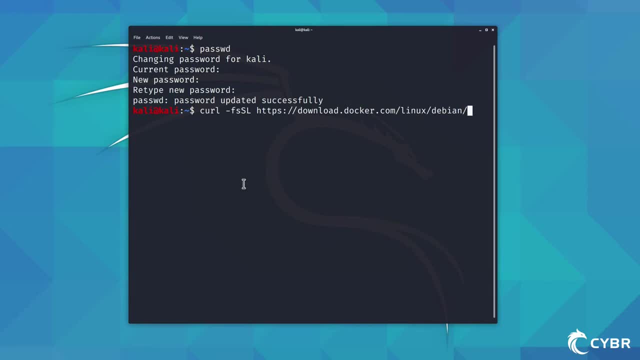 to help make sure that no one is tampering with our download, And I don't know why, but I always do apt-get instead of apt-key. It gets me every single time for some reason. Next we'll need to add the Docker APT repository. 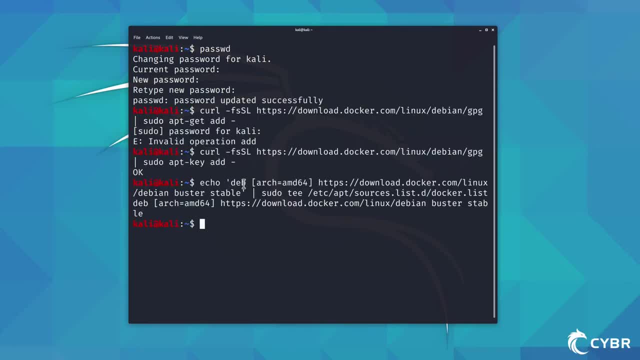 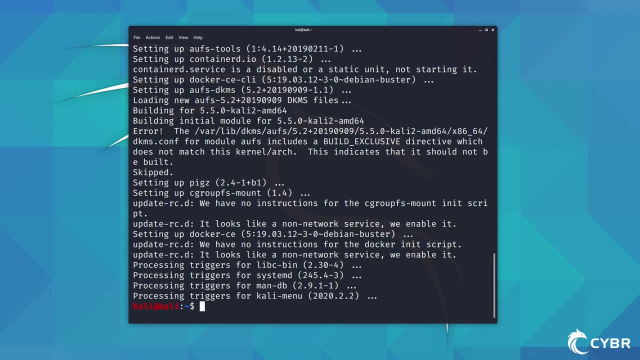 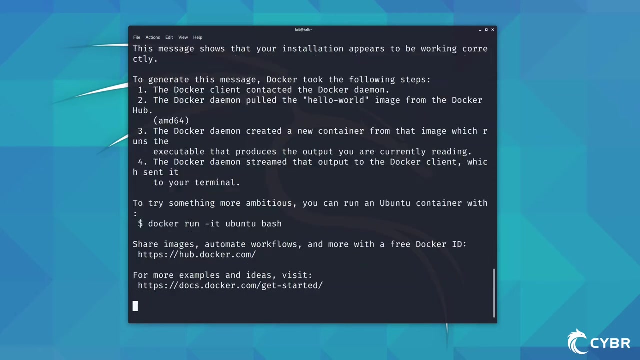 We'll do a sudo apt-get update And now it's time to install Docker, And that might take a couple of minutes, but once we're done we can test our installation by running sudo. docker run hello-world, And as long as we see this, that means we're good to go. 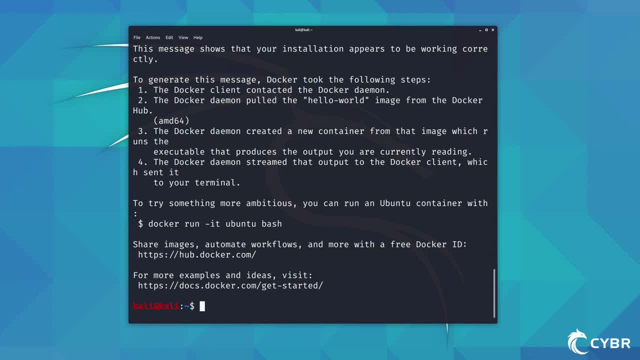 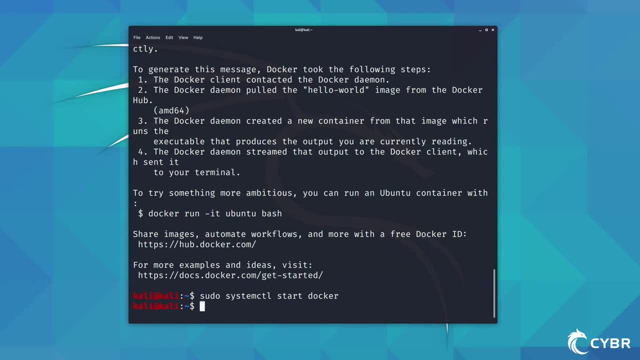 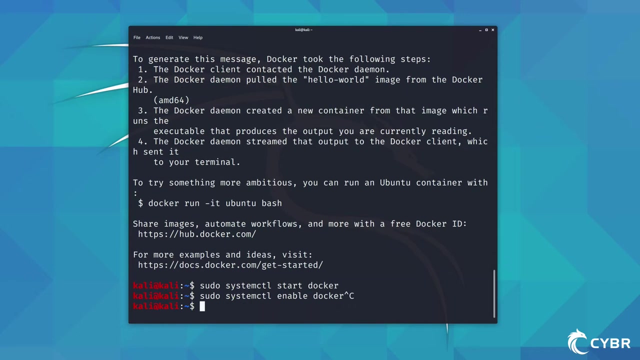 Now, at this point, Docker's service is still running, so we can test our application, And if we want to enable Docker to start automatically after a reboot- which will not be the case by default- then instead what we could do is sudo systemctl enable docker. But I prefer not to do that because I don't always use Docker when. 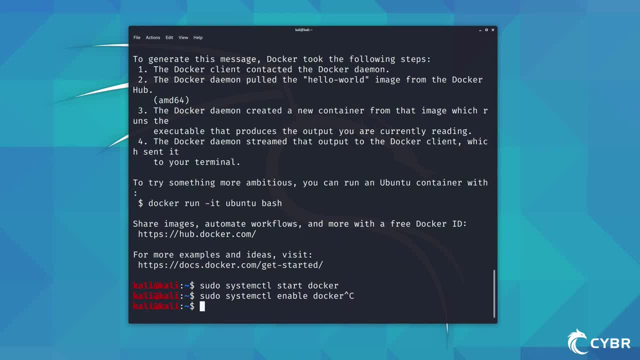 I start this VM, so I just won't do that yet, but you can if you want to Step 3.. Now the last step is to add our nonroot user to the docker group so that we can use docker. We'll do sudo group-add docker, but it already exists. just wanted to make sure. 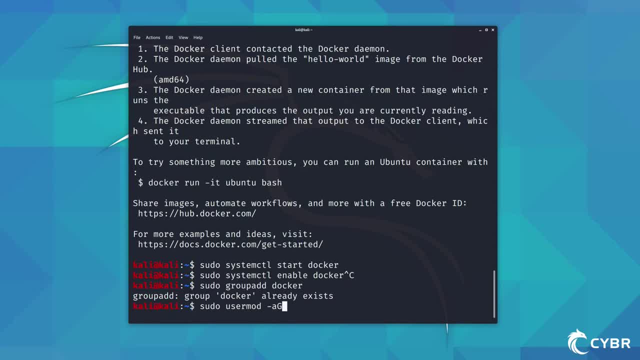 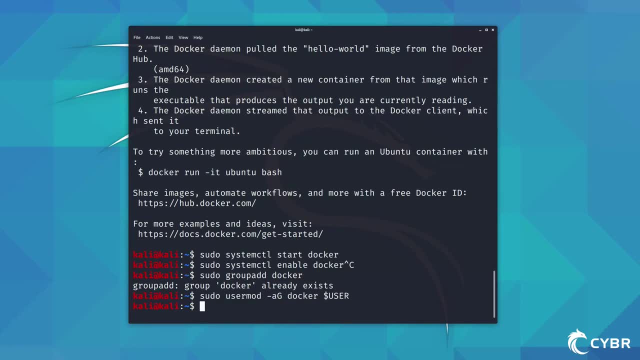 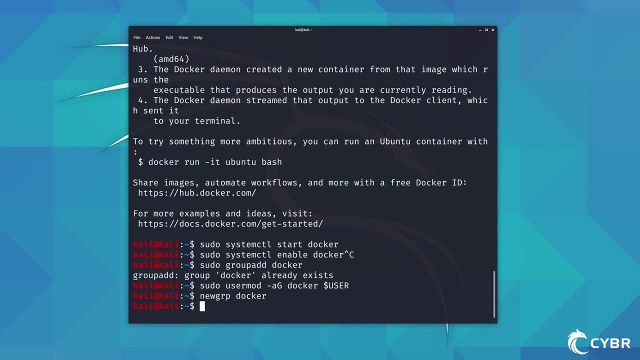 And then we'll do sudo user-mod dash a capital-G docker dollar sign user, And now we need to reload the setting so that the permissions change applies. We can do that with new group-docker. however, the best way to reload permissions is to log out and back in again, And if that doesn't work, try to reboot the system. Otherwise, 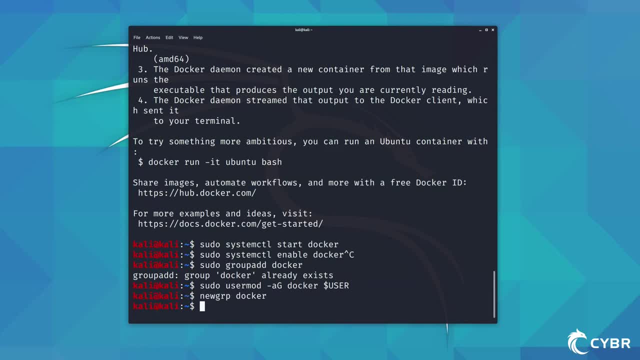 you may find that other terminal windows have not reloaded your settings and you may get that permissions denied error, which is annoying. But if you'd rather not log out or reboot at this time, you can use this command and it should work fine. Now. with Docker installed, we can now pull in. 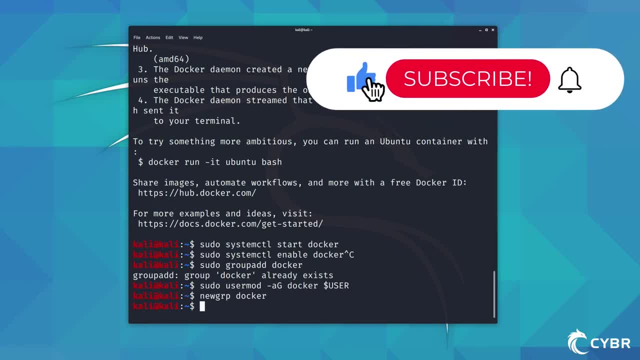 different environments as we need them, without having to install any other software for those environments. So, for example, if we want to run the damnvotable web application, we can do that with this simple command. We can type docker: run dash dash rm, dash it dash p for port, and we'll. 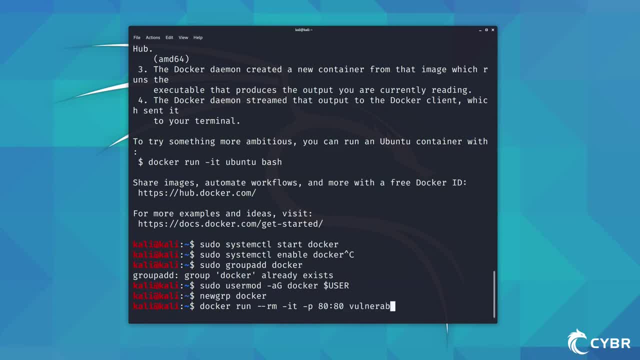 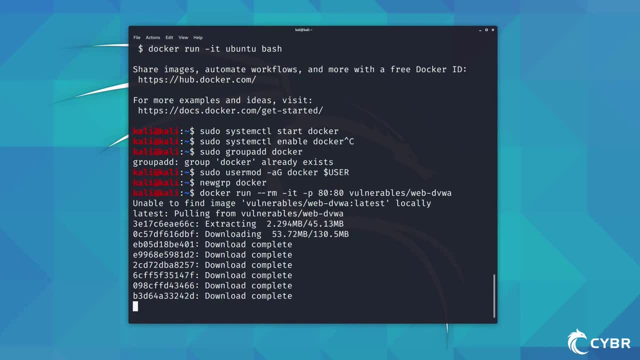 open that up at port 80 and then we'll bring in the image vulnerables forward slash web dash dvwa. It won't find it locally, since we haven't done this before. It'll download everything that it needs and then we'll be good to go. So just give that a couple minutes. So, after it completes, 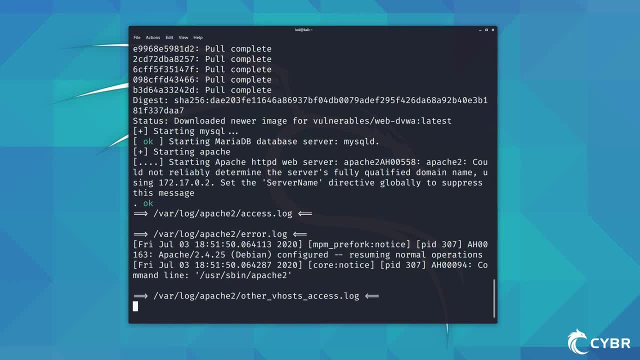 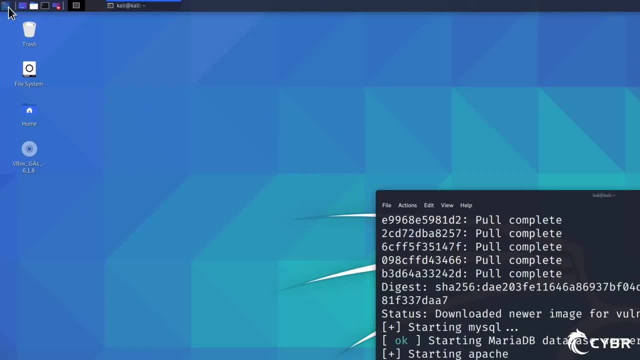 launching the container. we now have started Apache and we're monitoring the Apache web application, So we're going to go ahead and launch the container and we're going to access logs. We can go ahead and open up a browser of our choice. In my case, I'll do Firefox. 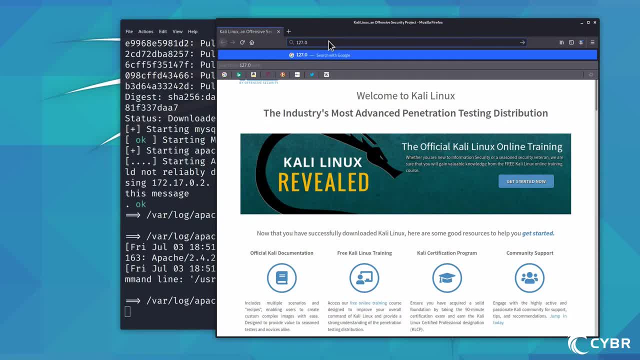 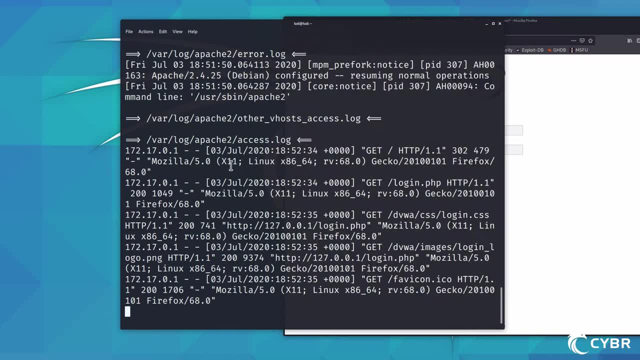 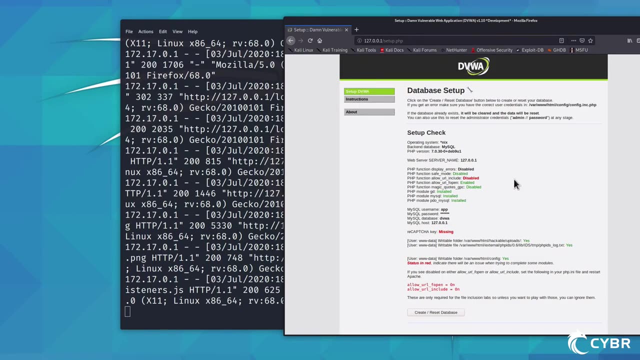 And we can navigate to 127.0.0.1 and it will pull up the damnvotable web application and we'll also see our requests coming through the access logs. here We can log in with admin password and the first time around we'll need to create and reset the database. Once we do that, we can go ahead. 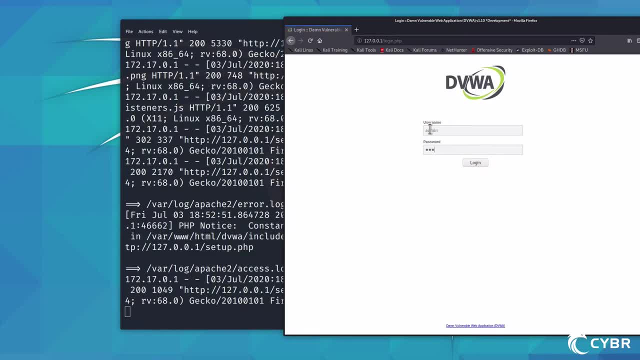 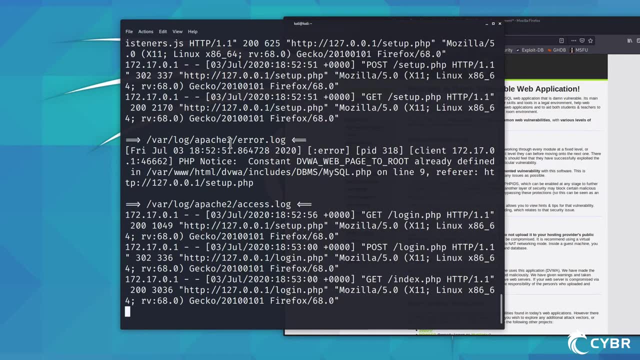 and log in again using admin and password of password again And we are now ready to use the damnvotable web application. But for this course we're also going to use something called the OWASP juice shop a lot, And the juice shop is one of the most modern and sophisticated. 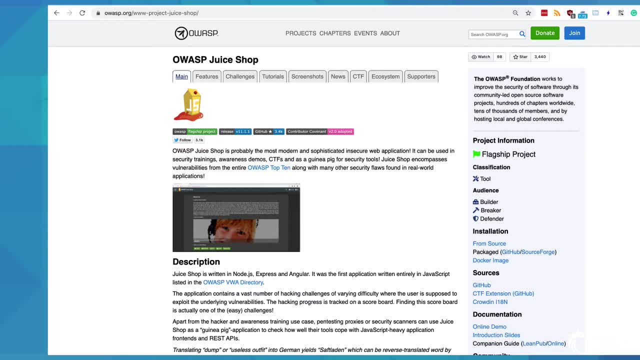 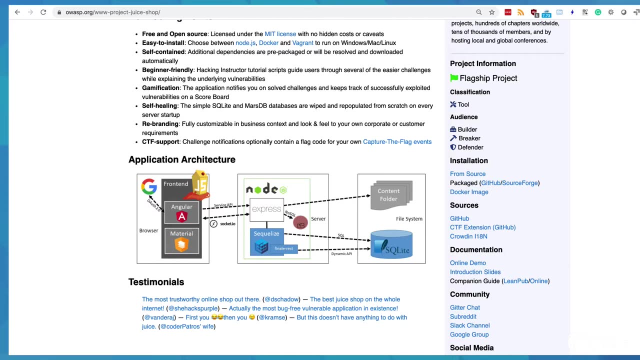 insecure web applications designed to be used in security training, and it includes vulnerabilities for all of the OWASP top 10, making it a perfect choice for this course, and especially because it has SQL injection vulnerabilities. It uses modern languages and frameworks like Angular, JavaScript, Nodejs and SQLite for 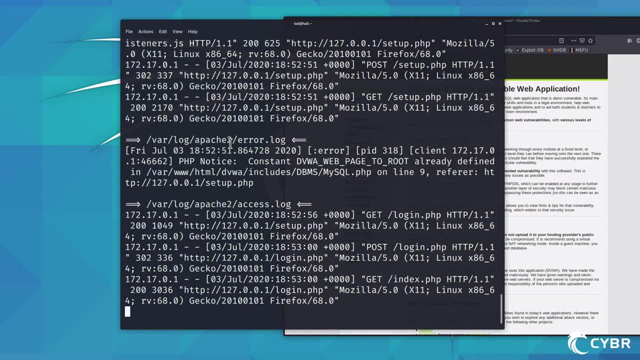 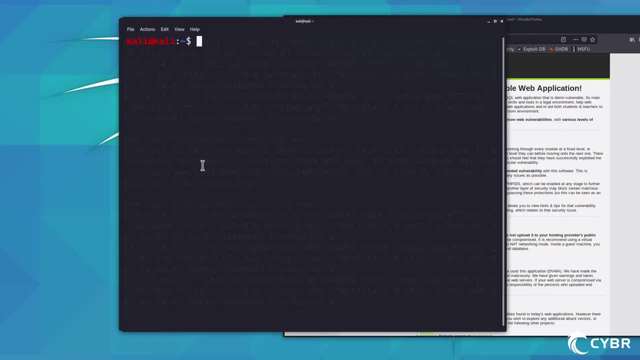 the database, and so, instead of having to spend a bunch of time setting up the application, we can run it via docker, just like we did. Let's go ahead and open up a different terminal window, And this time we'll run docker, run dash, dash, rm, dash p, and we'll open up port 3000.. 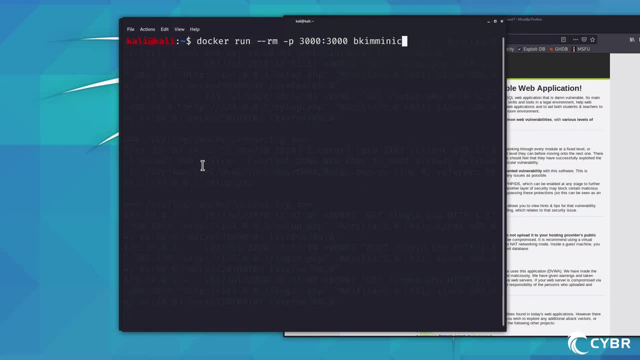 We'll use the image b-k-i-m-m-i-n-i-c-h forward slash juice shop And, as you can see here we get a permission denied. That's because, like I said, we haven't logged out in it again, so we have to reload our 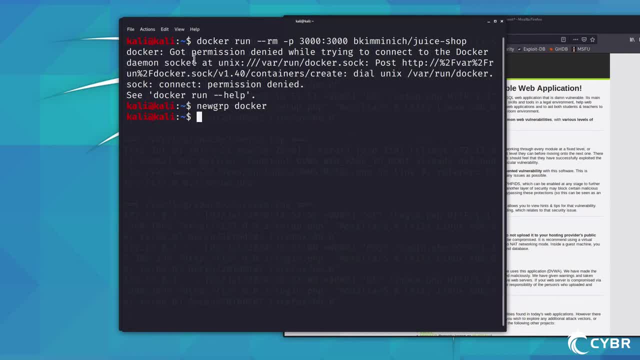 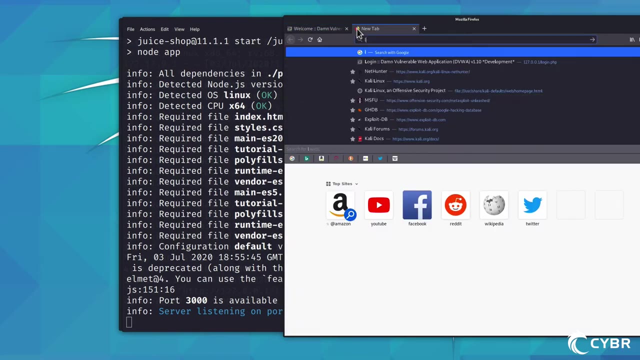 group docker permissions. Let's try that command one more time And this time it runs And with that, complete, we can go back to our docker. If we go back to Firefox, we can open up a different tab and we can go to localhost. 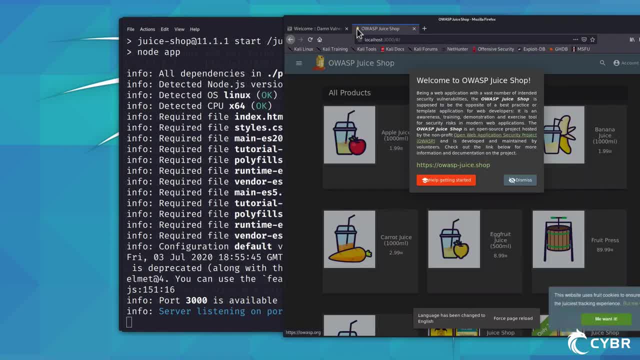 port 3000 to open up the juice shop, And since we're running the DVWA on port 80, we can run this juice shop on port 3000 at the same time, making it really easy to switch back and forth. We've now properly configured our environment and we're ready to move on. 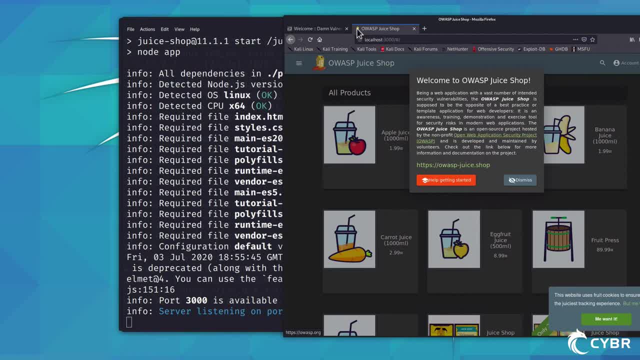 And in the next lesson we will do a brief walkthrough of a tool that we will use throughout the course, called OWASP ZAP, And it is a free tool That comes pre-installed in Kali. So go ahead and complete this lesson and I'll see you in the next one. 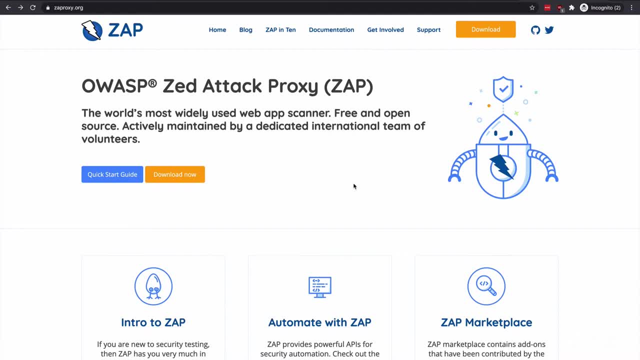 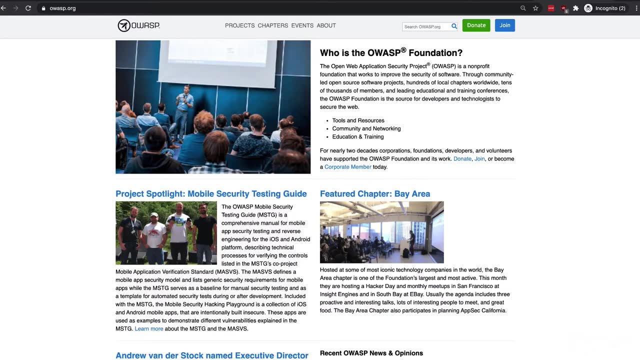 In this lesson, we get started with a tool called OWASP, ZAP, And ZAP stands for Zed Attack Proxy, and it is a free, open source penetration testing tool being maintained under the umbrella of the OWASP organization, And if you're not familiar with OWASP, definitely check it out. 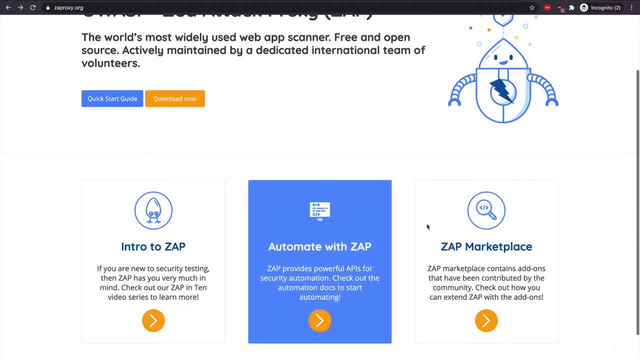 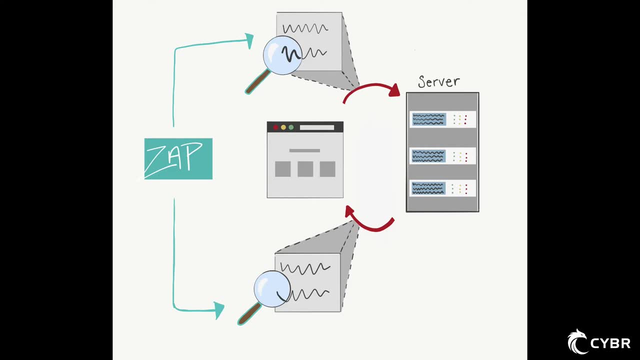 Now. ZAP is designed specifically for testing web applications and is both flexible and extensible with plugins and custom scripts. This implies ZAP is what's known as a man-in-the-middle proxy. Basically, it stands between the tester's browser and the web application, so that it 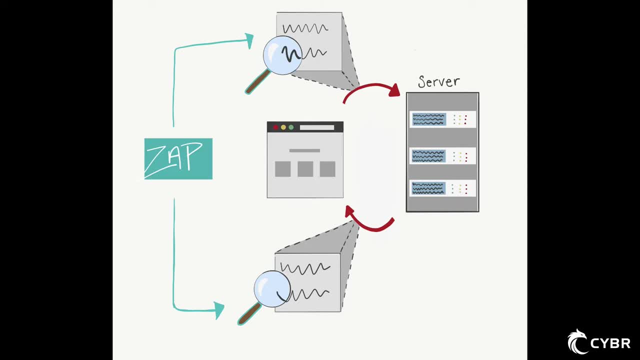 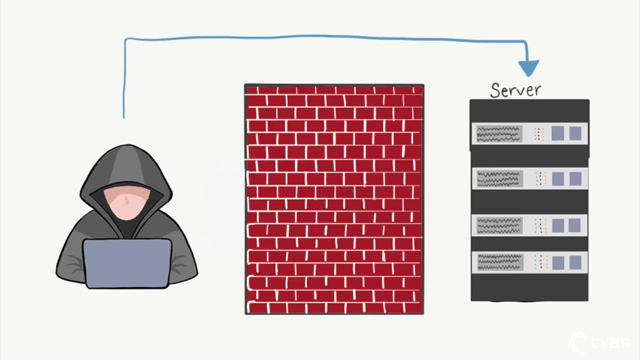 can intercept and inspect messages sent between the browser and the web application. So this is extremely helpful when pentesting, because it allows us to inspect and modify the contents of a message and then forward the packets onto the destination. So this means that even if the application has security mechanisms on the front end, 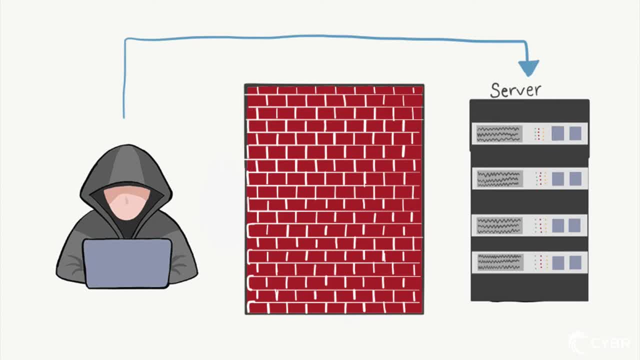 we can bypass them And this, by the way, is one of the reasons that we need to have multiple layers of security. You can have the most secure front end in the world and an attacker could simply bypass that layer of security and go directly to your backend. 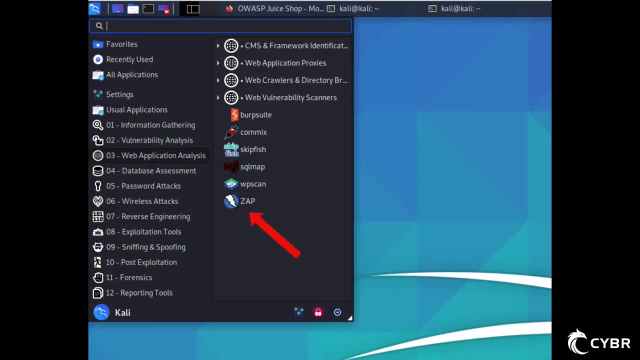 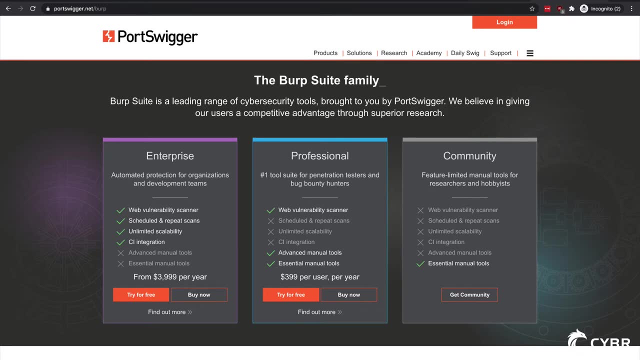 In any case, ZAP comes pre-installed in Kali, so you shouldn't have to install anything else for this to work, And a popular alternative to ZAP is Burp Suite, which also comes with a free version, But for this course we won't be using Burp. 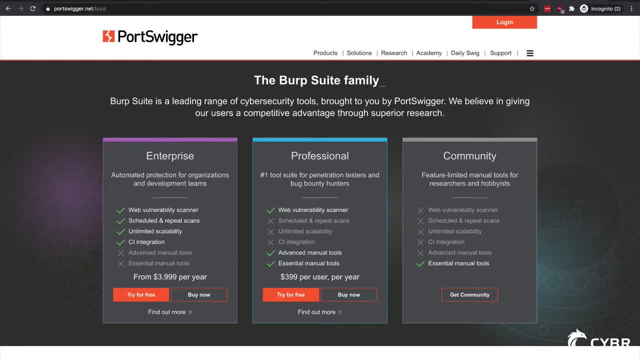 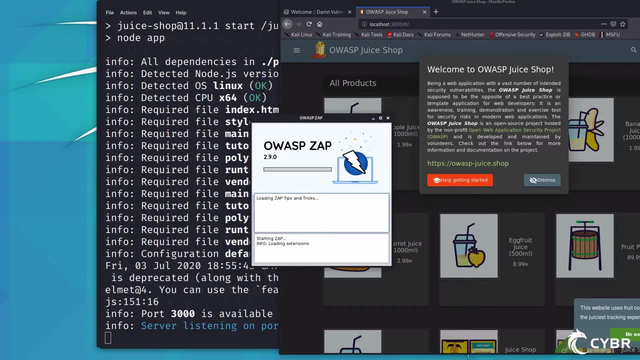 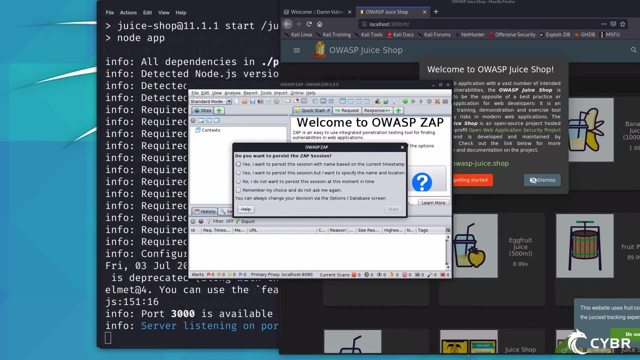 Most of the concepts translate fairly well, So if you do insist on using Burp, you can certainly do that. So let's go ahead and pull up ZAP When we first open it. it will give us a few different options. The first option is to persist this session with the name based on the current timestamp. 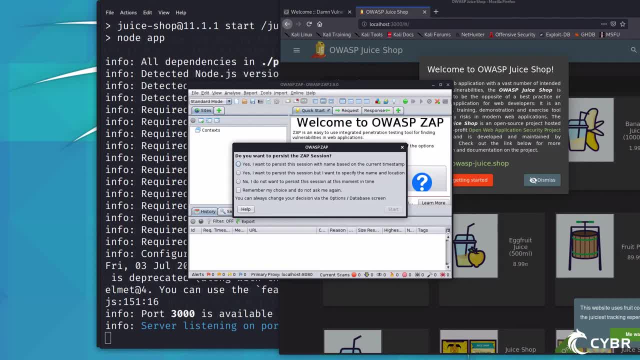 and with the second option, persisting the session as well, but you get to specify the name and the location. The third option and final option is, if you do not want to persist the session- maybe because you're just exploring for the first time- you have no need to save that session. 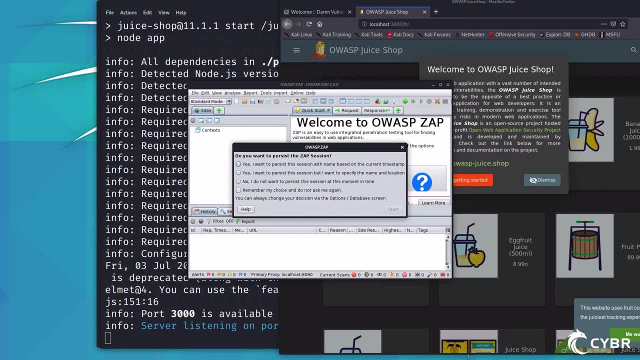 And then, finally, you can remember your choice so that OWASP ZAP does not ask you again For this video. I will select yes, I want to persist the session with the name based on the current timestamp. Next, it will ask us to manage our add-ons, including with the marketplace. 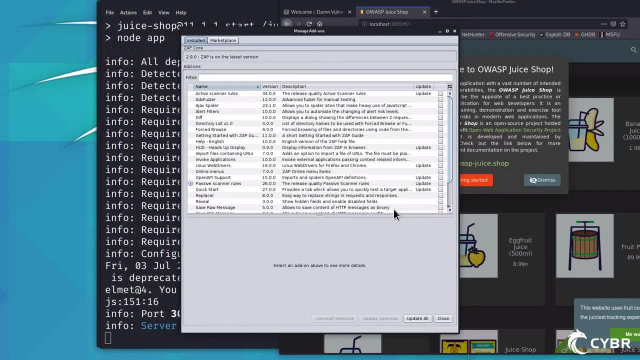 Now I do see here that there are some add-ons that have some updates, so let's go ahead and update all of them, And technically I could let the updates run in the background and close this window. but since I don't have a whole lot of updates, it should go pretty fast, so let's go ahead. 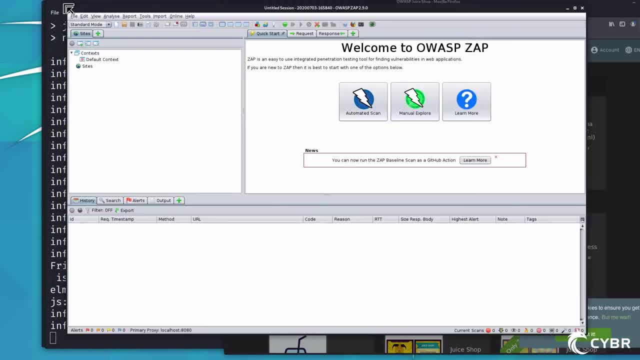 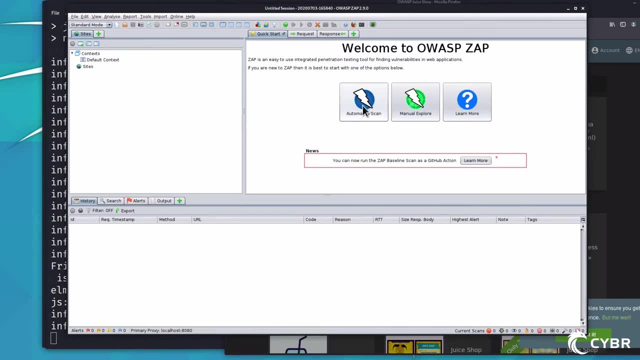 and just fast forward through it. Once complete, I can close this window and we can go ahead and get started Instead of doing a walkthrough of ZAP at this point. I'll just point out that we could do an automated scan of a web app target and we can also manually explore. 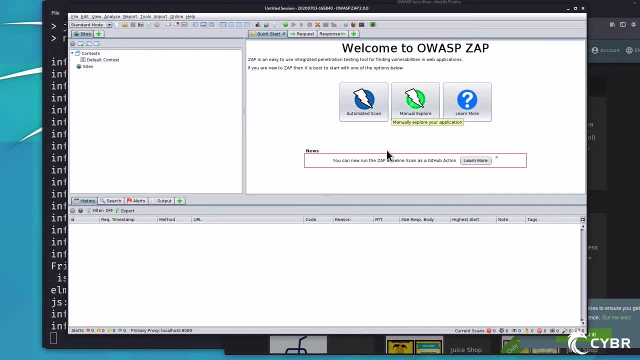 Now automated scans crawl the target application to find potential issues, while the manual exploration is what it sounds like. It is a way for you to manually explore your target, And since we're going to be spending a lot of time on this, I'm going to go ahead and 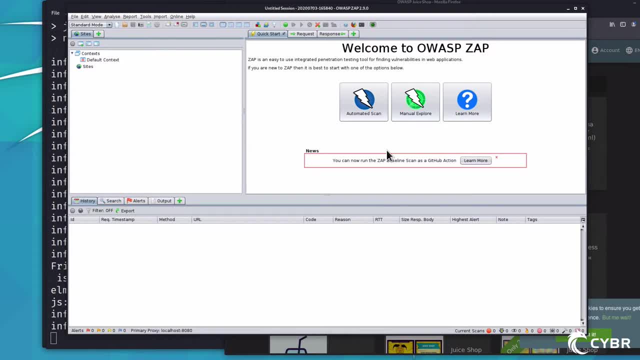 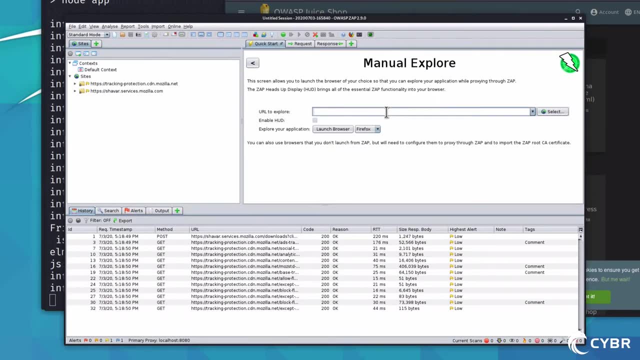 just leave it at that for now, and we'll get started with a manual exploration Now. since we launched the OWASP Juice Shop app from a prior lesson, we can simply type the URL here And then we can specify which browser to use, and I'll keep it at Firefox for now. 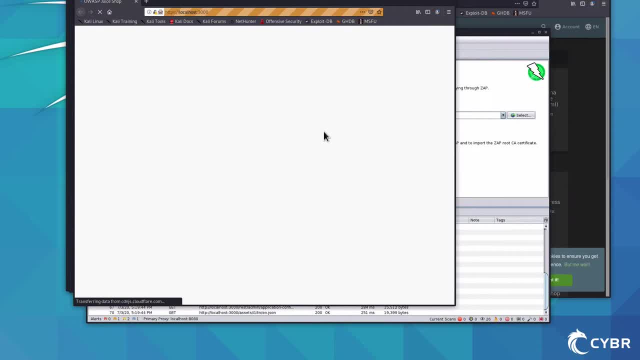 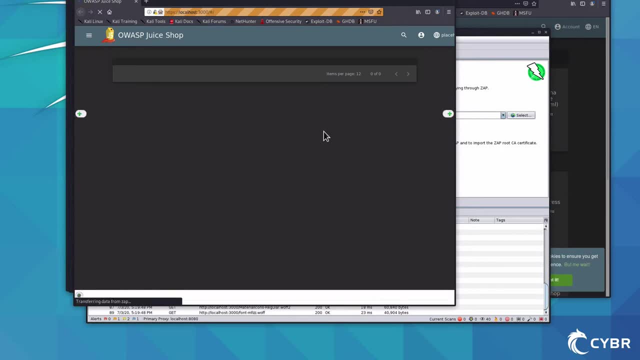 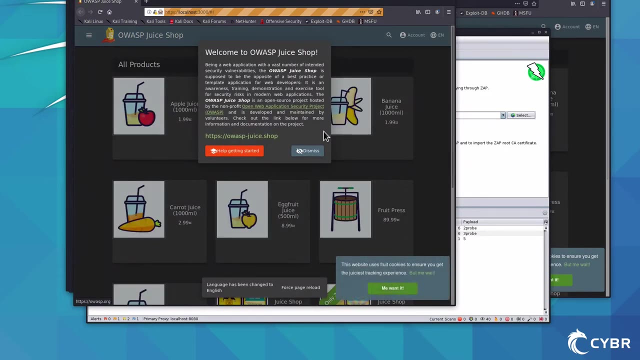 Then we click on launch browser, And by launching the browser this way, ZAP automatically configures it to proxy through ZAP, making it so that you won't have to worry about certificate validation warnings for sites that use HTTPS. Keep in mind, though, that you could configure your regular browser to proxy through ZAP, and. 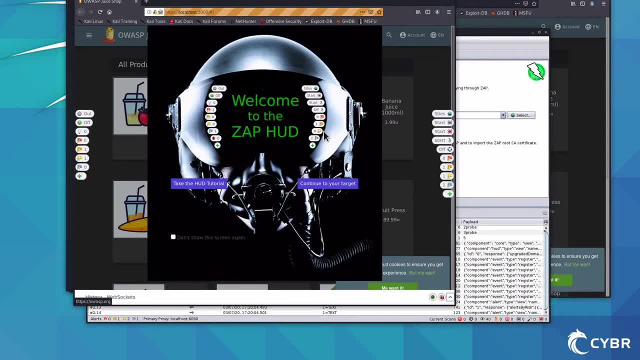 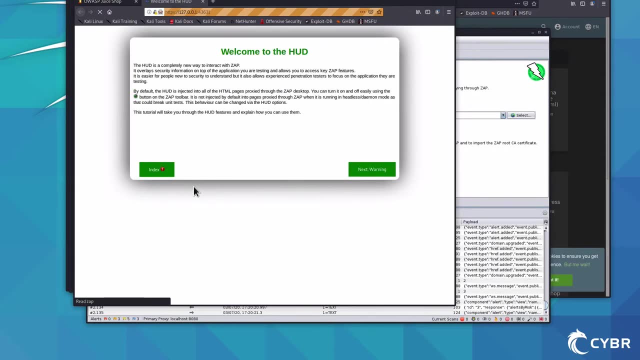 use that instead, but this does make it easier And as you open up the browser you should see a welcome to ZAP hud popup. You can either continue to your target or you can take the hud tutorial. I really recommend that you take the hud tutorial to get started, but I won't be showing you. 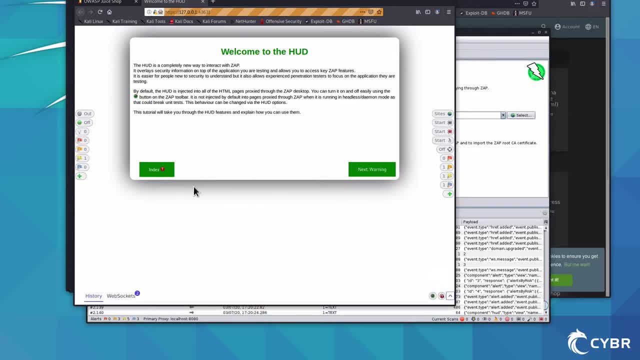 that walkthrough, since it is self-guided. So go ahead and complete this lesson, Walk through this tutorial and then I'll see you in the next lessons. At some point in time we will come back to ZAP and we'll actually use it for some pen. 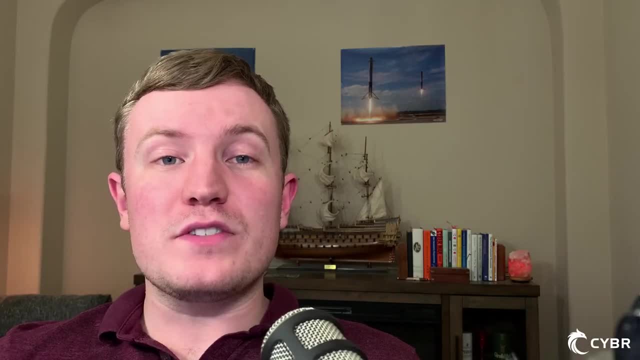 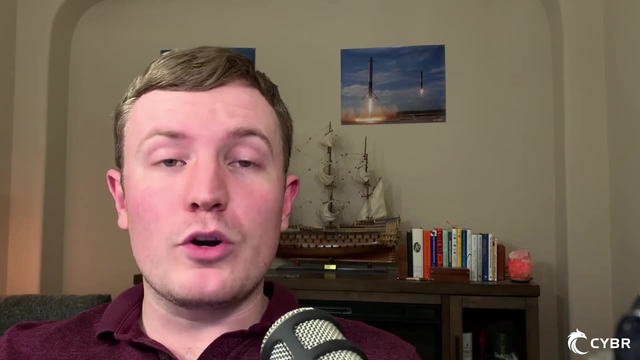 testing attacks. And again, if you have any issues at all with the steps that we just completed, please let us know in the forums on cybercom, because this is an important step to complete if you want to follow along with the hands-on demonstrations throughout this course. 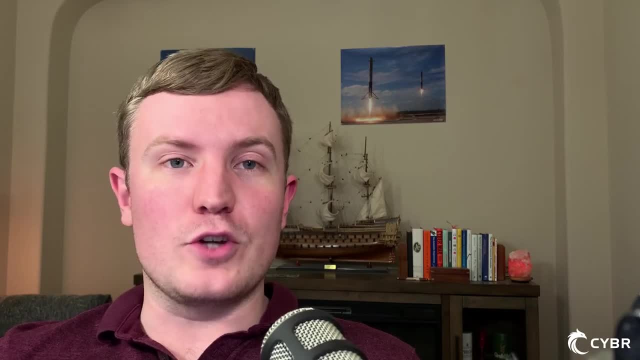 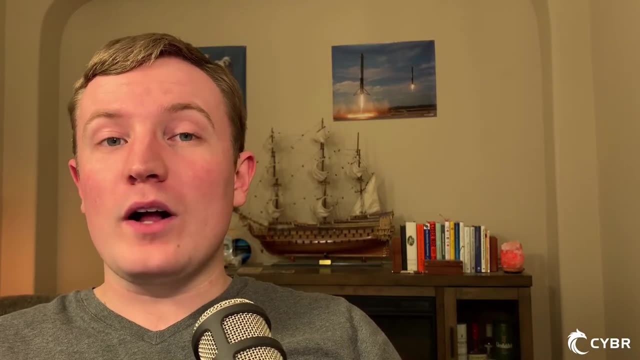 So we definitely want to make sure that you have OWASP ZAP up and running and good to go. But if you don't have any issues, please complete this lesson and I'll see you in the next one. In this lesson we're going to quickly go over SQL as a refresher, because understanding 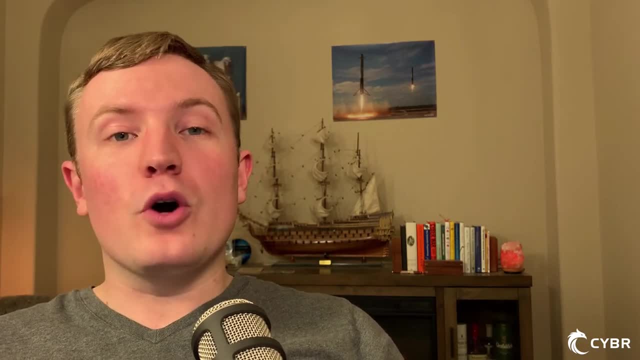 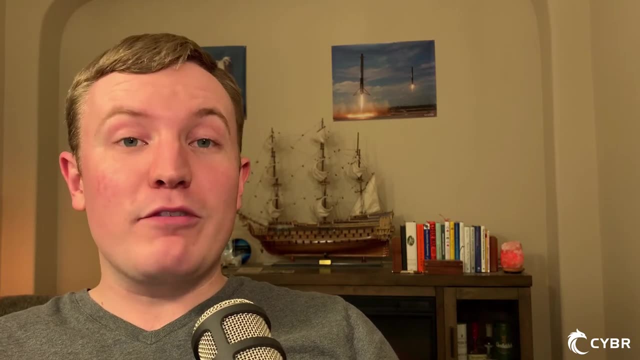 the inner workings of SQL is pretty important to understanding SQL injections. Now, this is not meant as a complete explanation of SQL, so if you have zero knowledge of it, I do definitely recommend that you pause here and go take a full course on the subject. 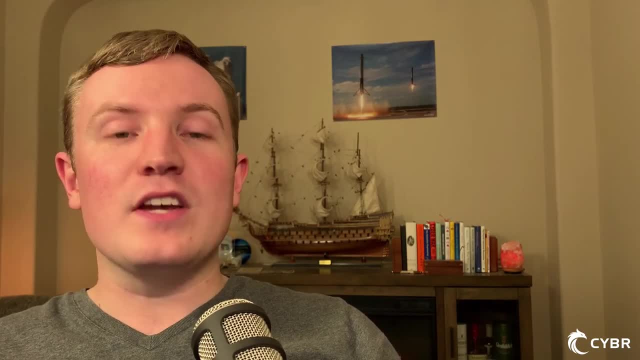 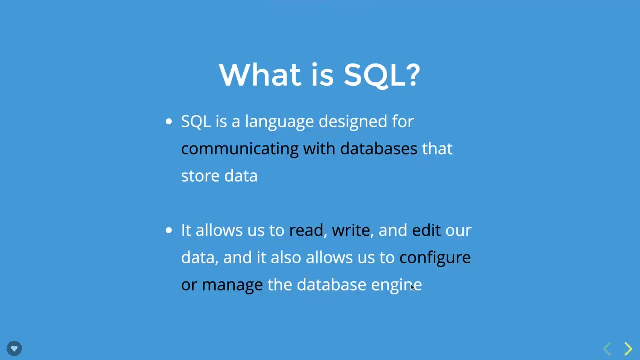 Think of this instead as a crash course to SQL in just a few minutes, in case you haven't touched it in a while. So SQL is a language designed for communicating with databases that store our data. It allows us to read, to write and to edit our data. 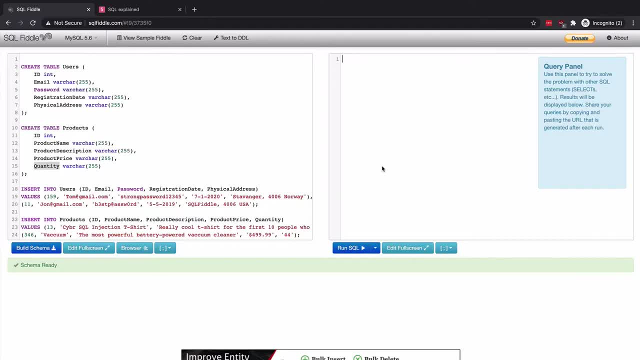 And it also allows us to configure or manage the database engine, And I'll be using a website called SQL Fiddle in order to demonstrate- And this is a free resource, so feel free to follow along. So let's say that we have two tables in our database. 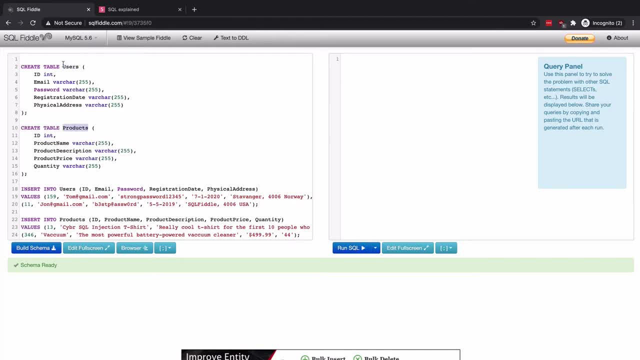 We have a users table and we have a products table. The users table contains all of the users for our application, including their ID, their email password, registration date and physical address. the products table contains all of the products that we're selling, including the ID product. 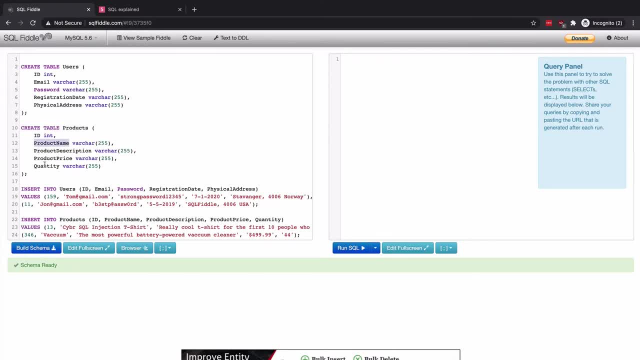 name, product description, product price and the quantity. And if we wanted to pull data from the users table, we might run this query And it will return all of the entries in our users table, including all of those different columns that we talked about. Or if we want just the registration, 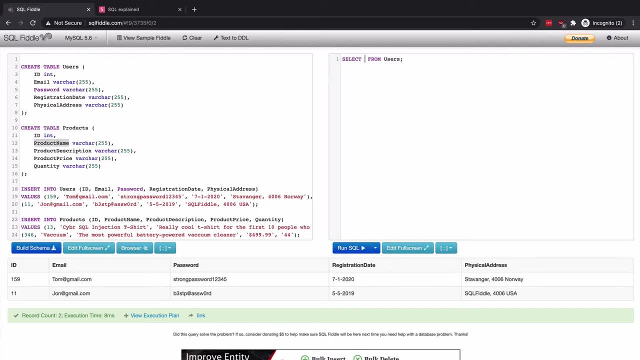 date for a specific user. instead, we could run select registration date from users And if we want to specify an email address, we could say email equals tom at gmailcom and run that query And we could see the registration date is 7-1-2020.. So, in order to run these queries, 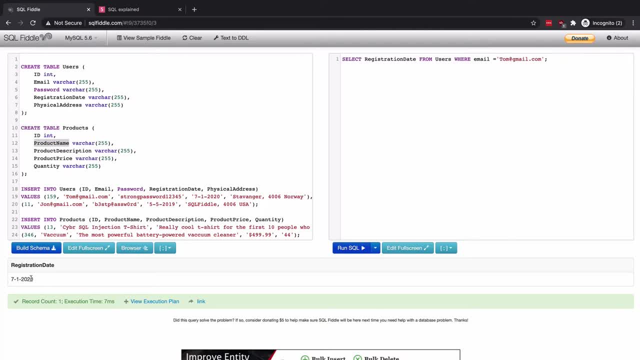 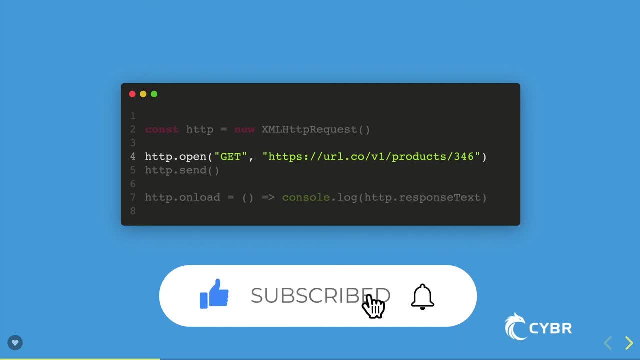 in some cases we have to use information submitted by our users of the application. For example, if a user is checking out a product with ID of 346, our application may request it like this: And here we have a get request for the products API call. And here we have a get request. 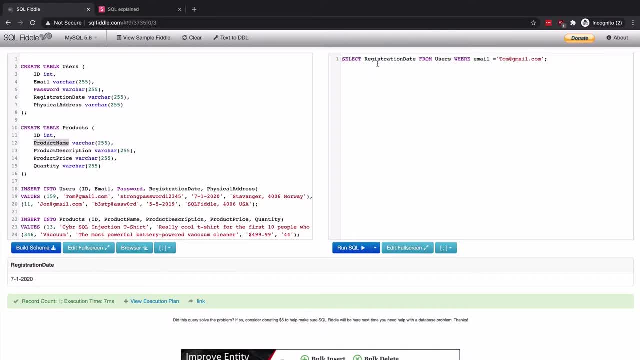 call with ID of 346.. And that API URL is running this SQL query Select from products where ID equals 346.. And if we run that, we'll see that the ID is for product name of vacuum with this product description, this product price and this quantity left in stock. And we could also run an. 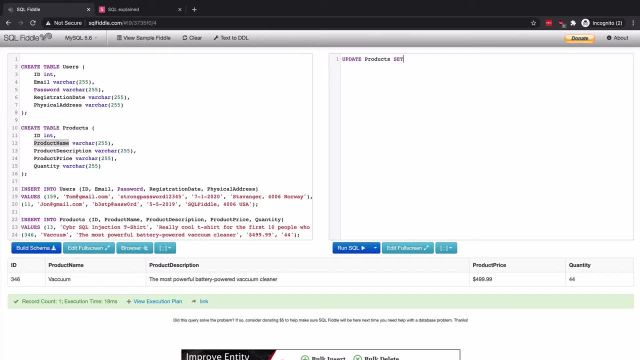 update query So we could do update products, set product name and we could also run an update. product price equals to zero where the ID equals 346.. And if we ran this query- which I can't do because SQL fiddle does not allow us to use queries like update and some of the other ones that we'll? 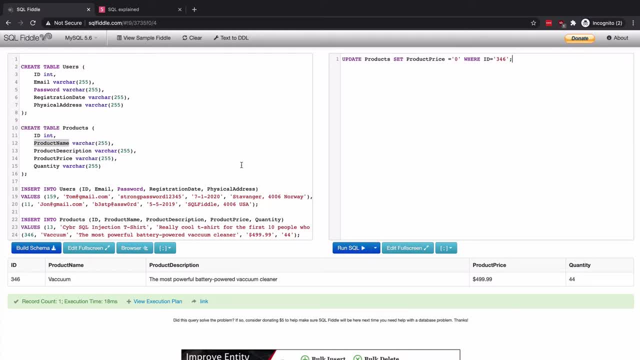 take a look at, most likely for security reasons. But if I were to run this update query, it would change the price of the ID 346, in this case of vacuum cleaner, to be $0 instead of $500.. And if we're an attacker and we're trying to do an SQL query, we're going to have to run an update query. 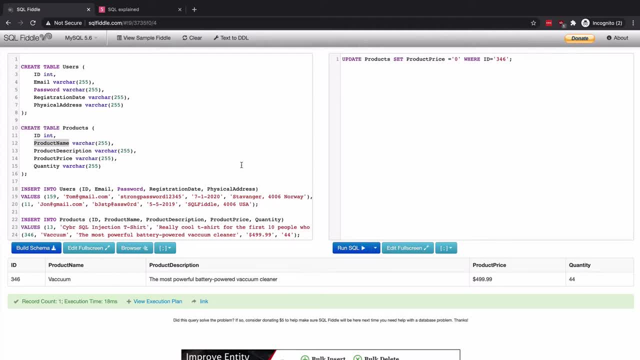 SQL injection and buy this product for nothing. That might be a query that we'd want to run. Another SQL operation we could do is called a union query. So let's say we did something like this: Select email and password from users. union. select product name and product price from. 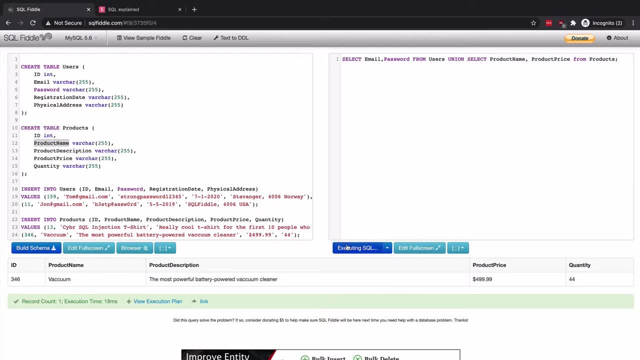 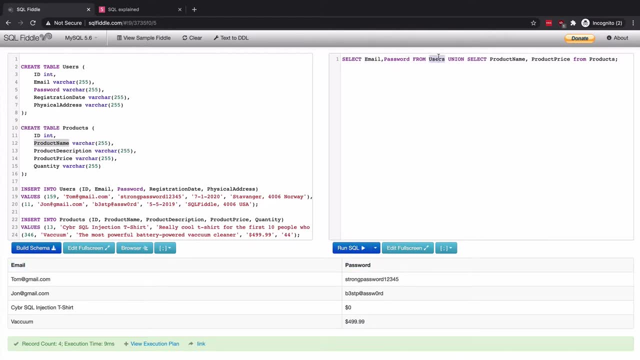 products. If we run this query, we can see that we have the email column as well as the password column. So we're going to run this query. And if we run this query, we can see that we have the email column because of this select statement here from the users table, But we're also combining the products. 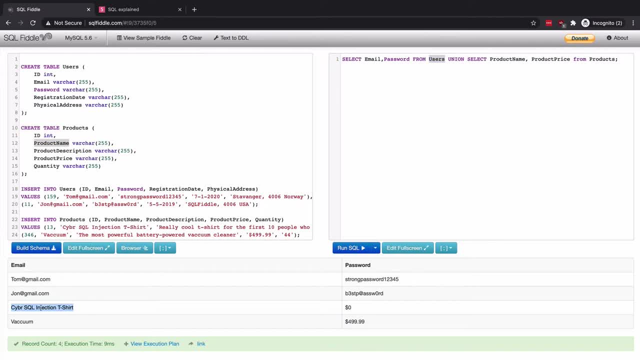 table with their product name and product price. So we have a product name here, cyber SQL injection- t shirt for the price of zero and the vacuum for the price of $499.99.. And so this is a very legitimate query And we'll see later, as an example of an SQL injection, why union queries can be. 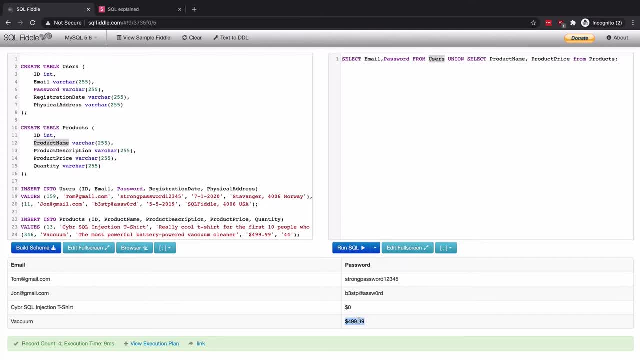 extremely helpful to an attacker because we can take a legitimate query and stream it to the string along additional results in order to pull from a different table. But again, I'm getting ahead of myself here. This is just an example of a legitimate SQL query. Of course we could also. 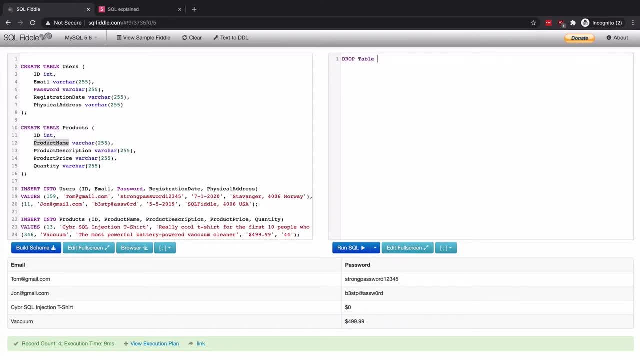 drop tables. So we could do drop table users. And again, I can't do this because of SQL fiddle restrictions, I'm sure for security reasons, But in this case we could do drop table users and it would delete this table, only leaving the products table. So if somebody was doing this, 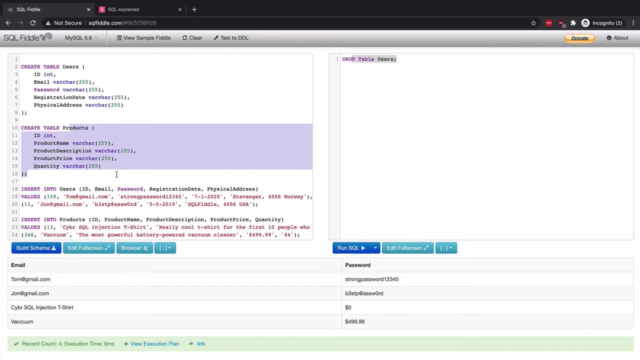 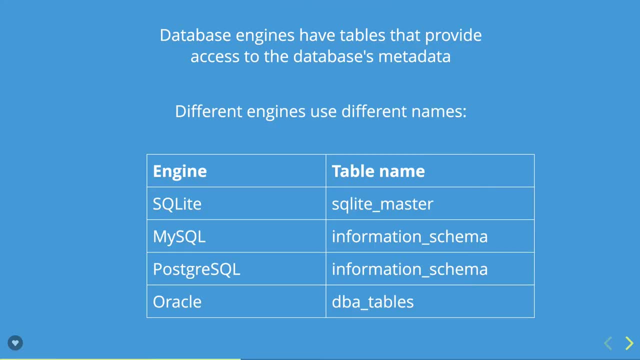 against our database and application. all of a sudden, we'd be missing a query, So we could do critical table, which means our application would no longer function properly. Now, one more thing I want to talk about is that database engines also typically have tables that contain general. 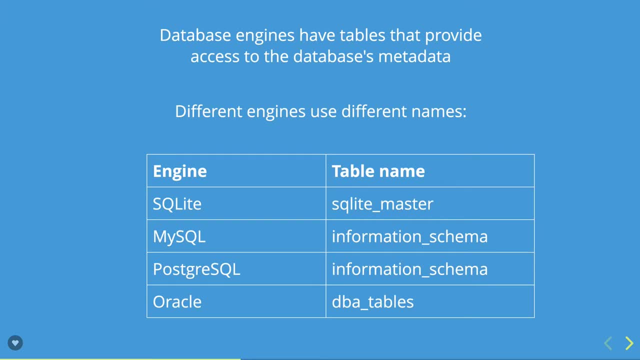 information about metadata, such as keeping track of all tables or the database's schema, basically the essentials for the database to keep running properly. And for different database engines it's a little bit different. So for SQL light we have SQL light master For MySQL, 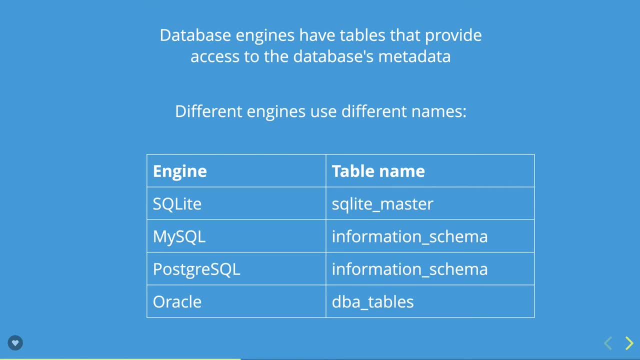 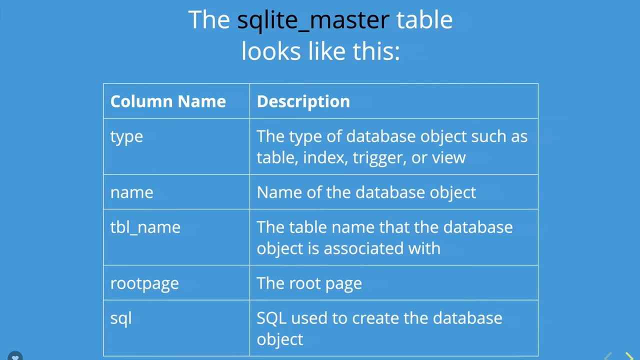 we have information schema For Postgres, we have information schema as well. And then for cool databases, we typically have DBA tables And, for example, the SQL light master table might look something like this: we have a column, name, of type of name, table name, root page and SQL. 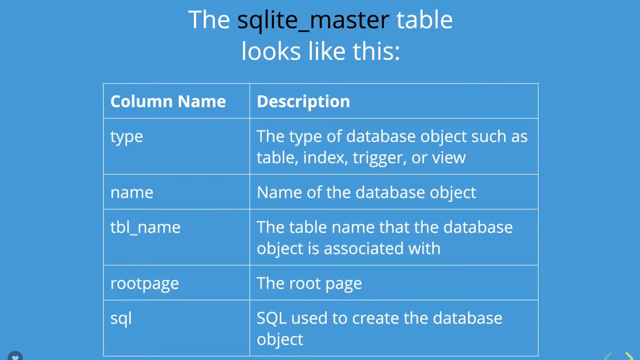 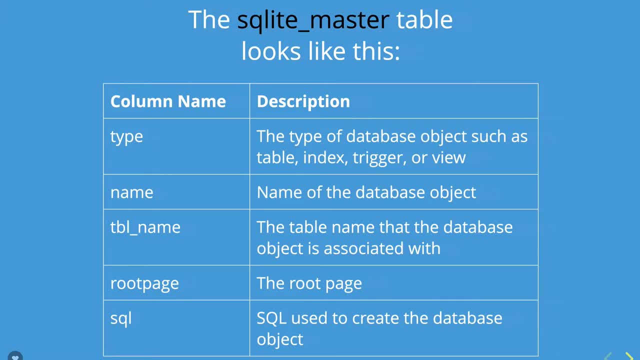 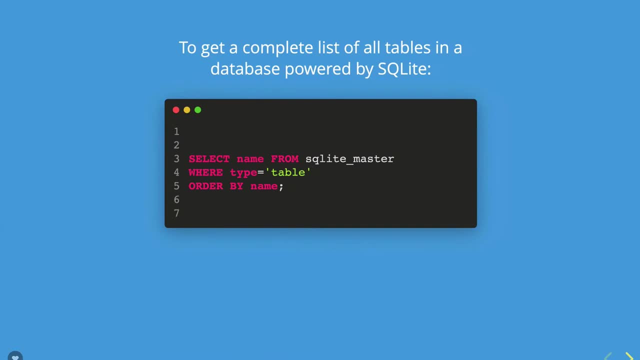 name and then we're going to do a table name. So to get a complete list of all tables in a database powered by SQL light, we could run this very simple query, select the name from SQL light master where the type is of table, and that would return a list of all the tables stored in that. 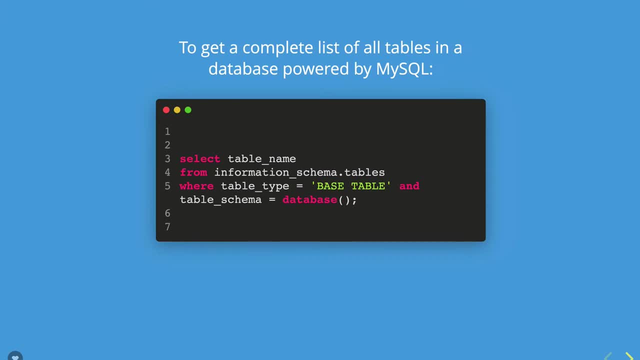 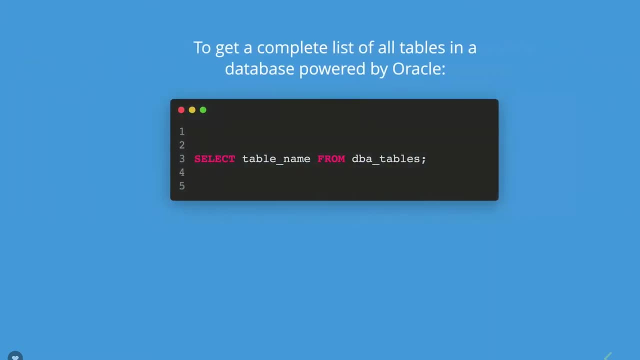 database To get a complete list of all tables in a database powered by MySQL. it looks a little bit different, but the end result is the same. Then, for Postgres, even simpler, And for Oracle, again very simple. All of what we've talked about to this point will be very important to SQL. 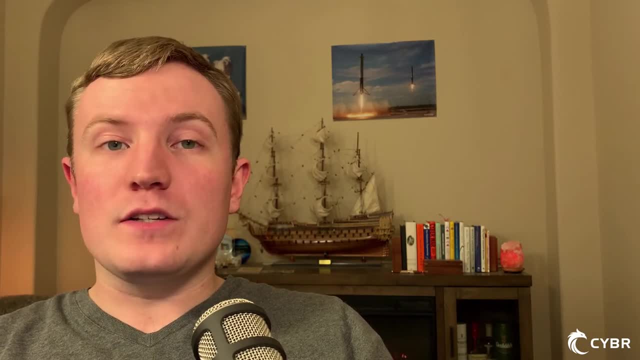 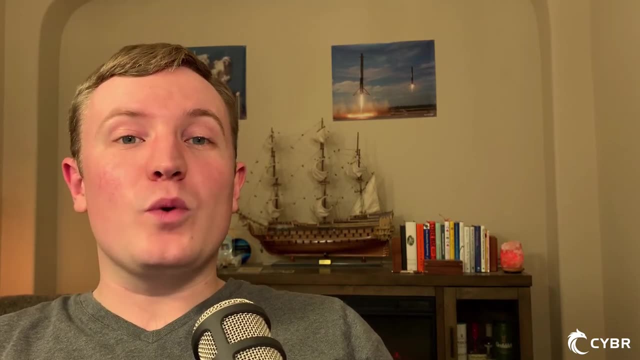 injections, because the very same things that allow our application to manage data in our database can be used to exploit that very same database. That's right. seemingly harmless queries can result in simple, all the way to massive exploits that can take down entire applications and entire. 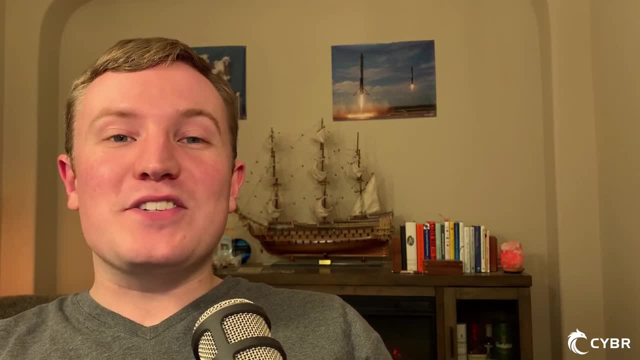 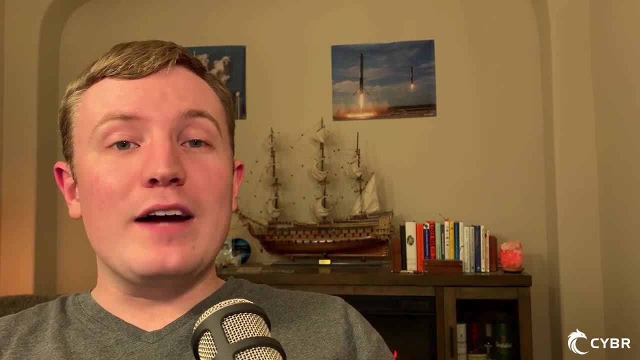 databases or extract sensitive data. So if we're going to do a table name, we're going to do a table name to extract sensitive information. Now let's complete this lesson and move on to the next lesson, where we will explain SQL injections. So we've talked about what SQL is and we've gotten a. 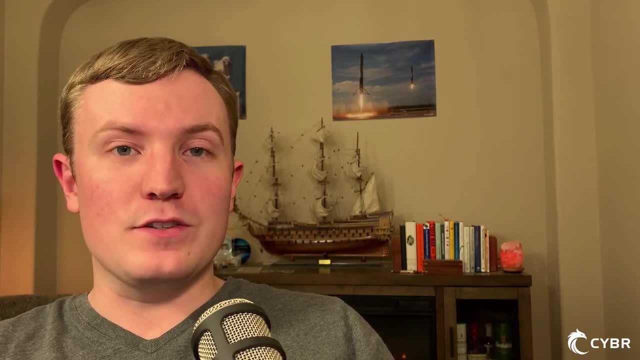 reminder of some common SQL statements that can be made by our applications. But now let's get to the good stuff. Let's talk about how seemingly harmless queries can be turned into SQL injections. Successful SQL injections allow an attacker to manipulate queries that an application makes to 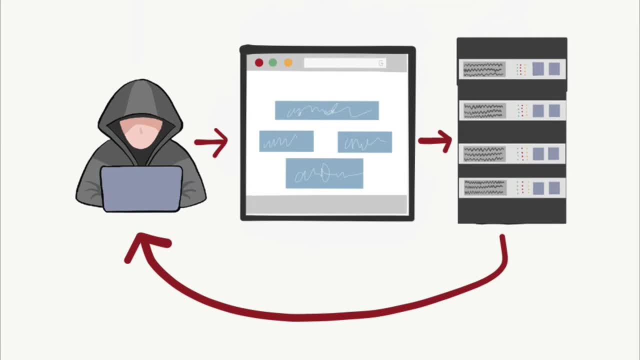 its database, And this results in attackers being able to see data they may not have seen in the database, manipulate that data in ways that they shouldn't have access to, or even modify the database itself in ways that could break the database in application In some extreme cases. 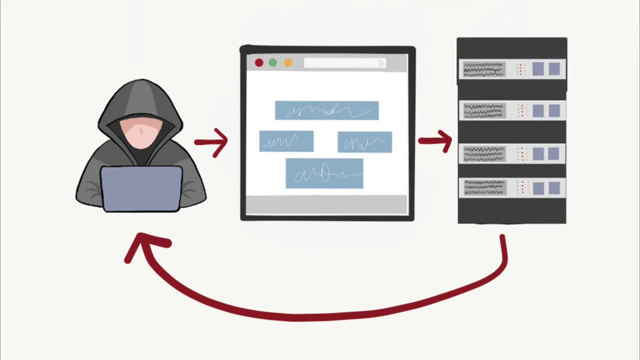 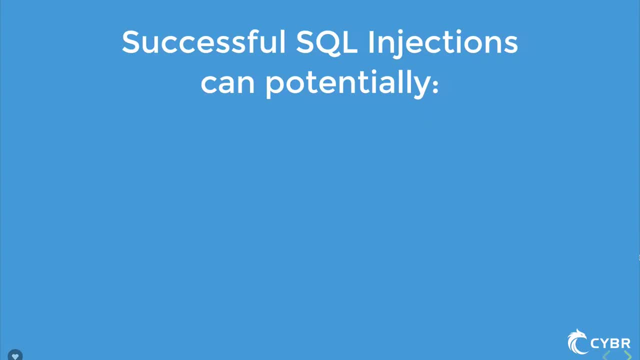 it's possible for an attacker to escalate an SQL injection attack to compromise the server hosting the database or perform denial of service attacks. More specifically, successful SQL injections can potentially read sensitive data from the database, modify that data with insert, update or delete. queries and modify it to the database itself. So in this example we're going to talk about how SQL injections can be used to manipulate queries that are not meant to see, manipulate that data in ways that they shouldn't have access to, or even modify the database itself in ways that could break the database in. 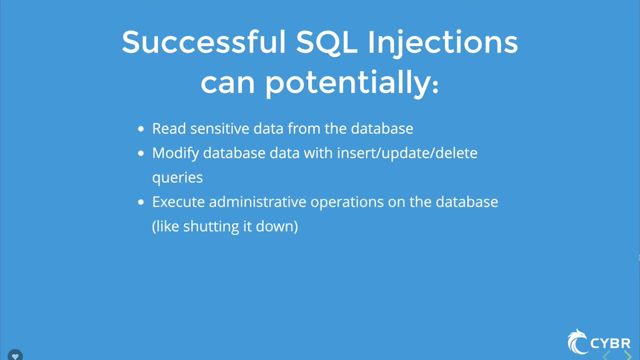 ways that they shouldn't have access to or even modify that data. in ways that they shouldn't have access to, Execute administrative operations on the database, like shutting it down. for example, extract the content of a file that exists on the database's file system. 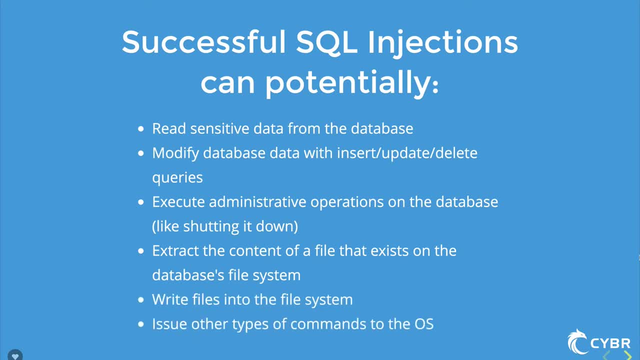 write files into the file system or even issue other types of commands to the operating system. Of course, some of these attacks will cause more or less damage than others, just like some of these attacks can be easier to carry out than others. And now that we know what impact they can have, let's explore methods and techniques. 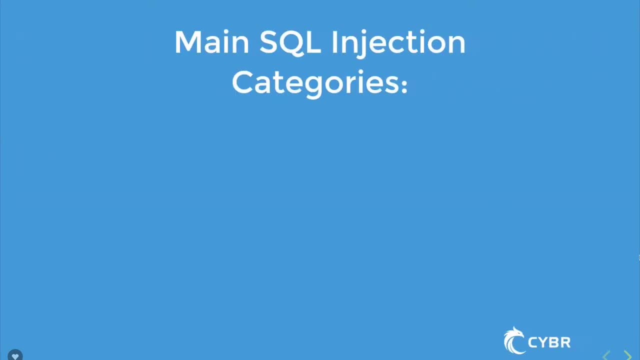 that can be used to achieve those results. Overall, SQL injections are often divided into three different categories. You have in-band, out-of-band, and inferential or blind. In-band attacks are the classical ones, where the attacker can both launch the attack and obtain the results through the same communication channel. 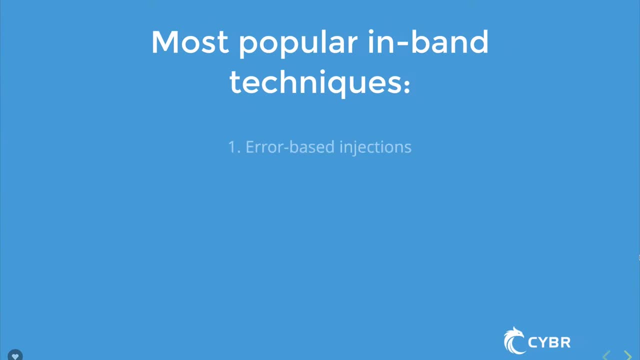 And the two most popular in-band techniques are error-based injections and union-based injections. Let's take a look at error-based injections. Error-based injections can get information about the database, its structure and its data from error messages that are displayed, which you may also know as information leakage. 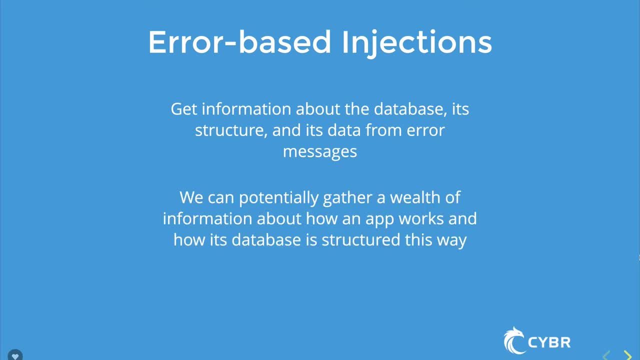 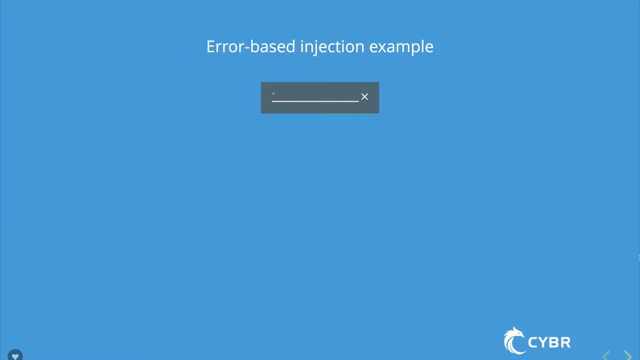 And, depending on how vulnerable an application and database are, we can gather a wealth of information about how the application works and how a database is structured, with error-based injections which can help us mount devastating attacks. Let's take a look at an example. Let's say that you type a single or double quotation mark in a search box. 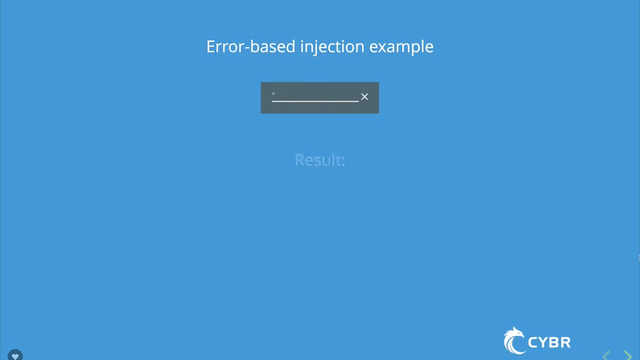 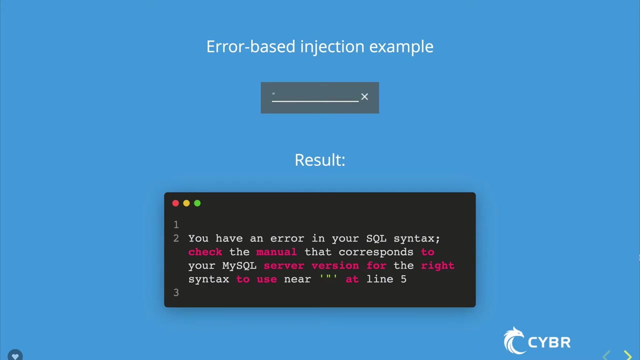 If you check the results of that query, you might see something like this: It might say that you have an error in your SQL syntax and that you need to check the manual that corresponds to your MySQL server version for the right syntax to use. near that. 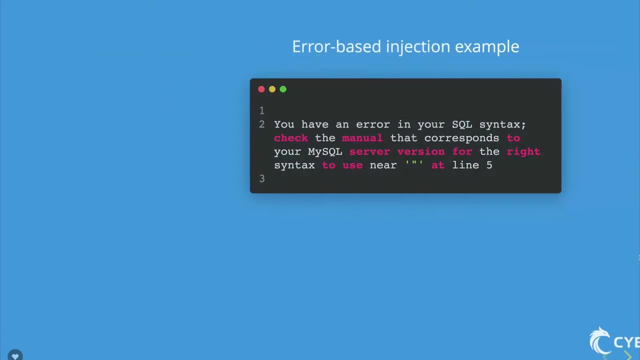 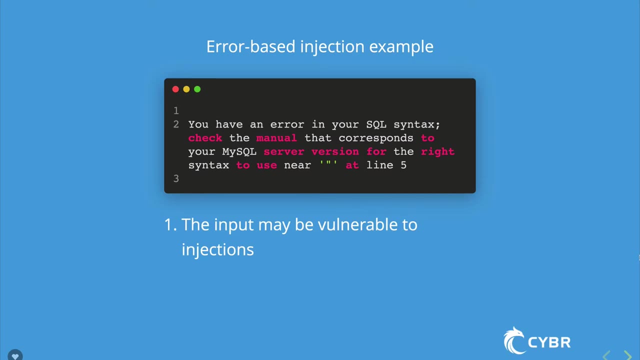 input you put in at line 5,, all of the sudden, you get two major pieces of information. You get that the input may be vulnerable to injections, since it tried to interpret your quotes, and that the database management system is MySQL. This is an answer to the question, but it also means that the 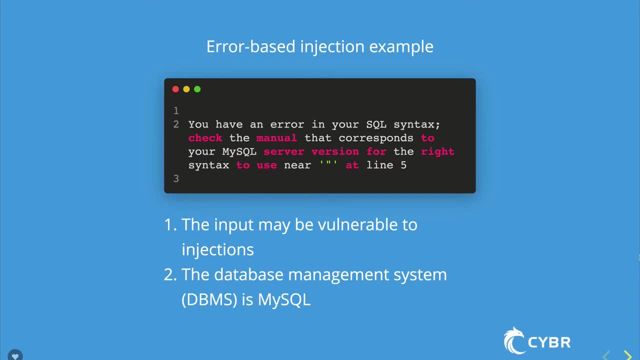 best way to avoid such a situation is to move the folder with a section of j 3000, but to not move the MySQL, And since different database management systems have different syntax and ways of doing things, that immediately narrows down the kind of attack that we can try, instead of aiming blindly. 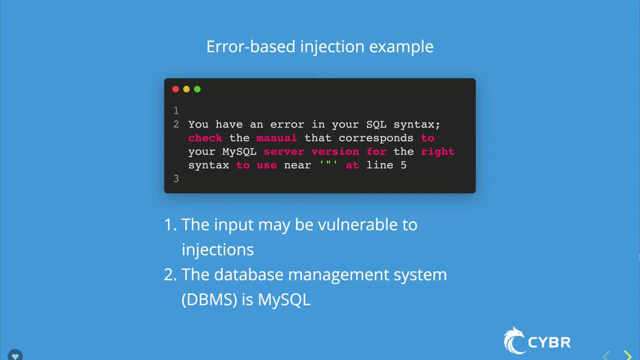 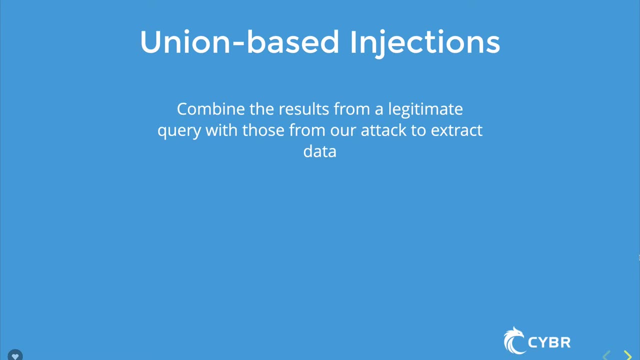 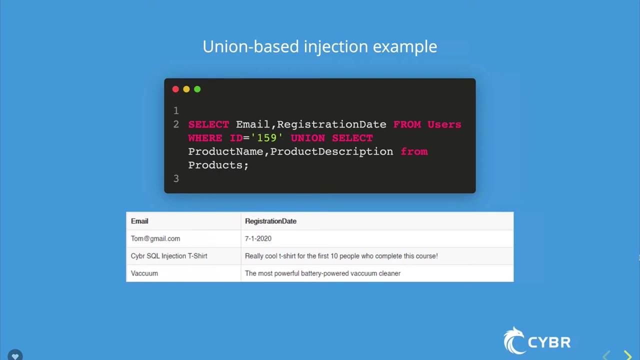 And you'll see what I mean in another lesson when we explore reference materials. Union-based attacks combine the results from a legitimate query with those from our attack to extract data. For example, here we have a select email and registration date from users where ID equals 159, and we union that with a select statement of product name and product. 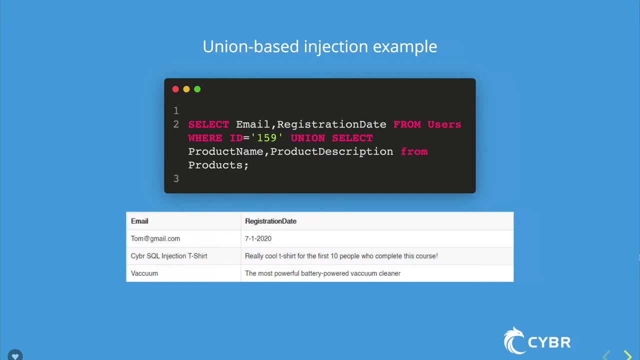 description from products. Now, all of a sudden, in the return table we have tom at gmailcom with his registration date and then we have the two different products. In this case, not necessarily something that's hugely impactful, but, as we will see, with SQL injections, in practice this can be. 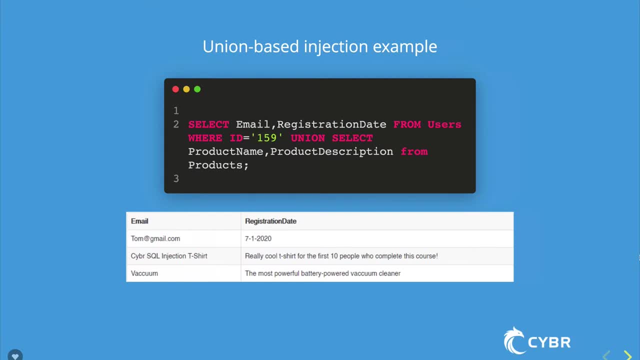 extremely powerful. Now, the thing is, both of these types of attacks require trial and error, since we need to try different things to get more and more information that the attacker can then use to perform a successful attack. That also means that these types of attacks should be detectable with the proper 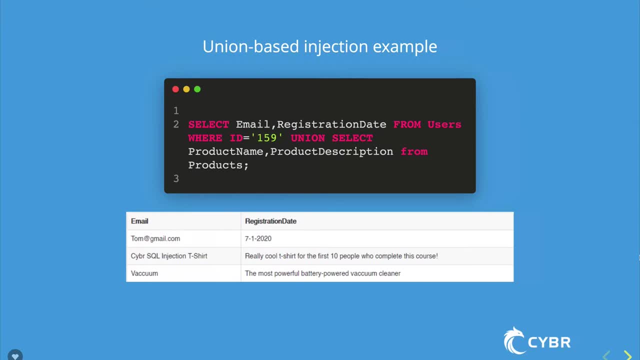 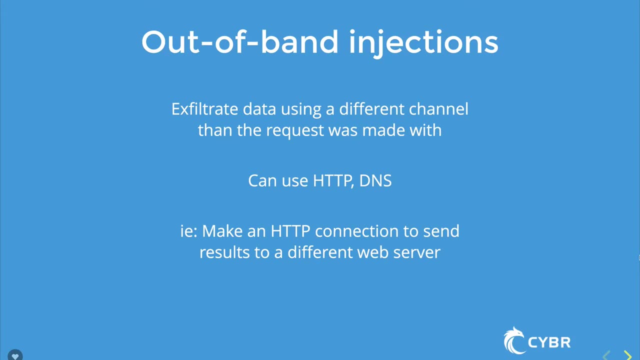 monitoring and logging in place, but we'll take a look at that in a future lesson. Then we have out-of-band attacks. Out-of-band attacks exfiltrate data using a different channel than the request was made, with using an HTTP or DNS protocol, And an example of that would 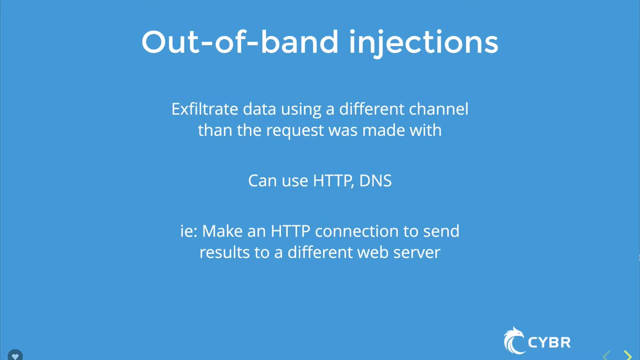 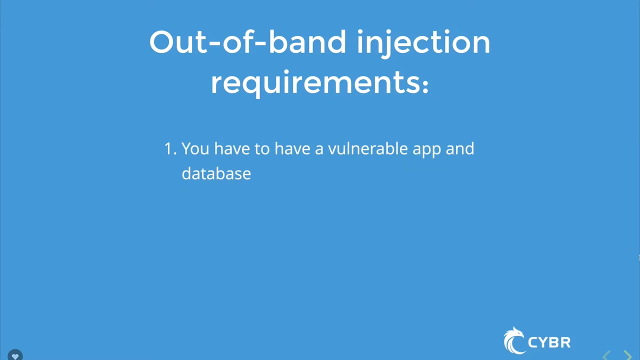 be making an HTTP connection to send results to a different web server. Now this attack requires access to enabled extensions in the DBMS server. initiate an outbound request without restriction, because information needs to be sent out. And number three, you need to gain sufficient privilege escalation to initiate that request. 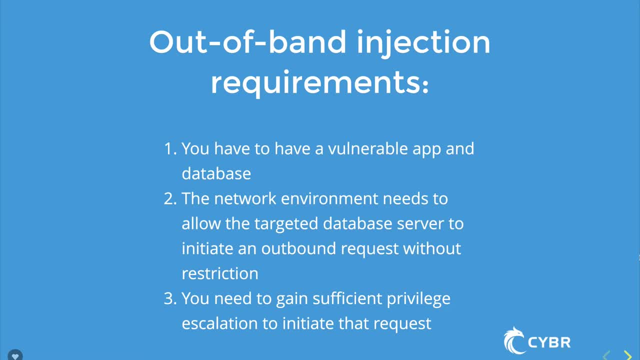 because, again, you have to be able to use enabled extensions in that database management system, which means you also have to have sufficient privilege to be able to call those extensions. Basically, if you're able to perform an out-of-band injection, the person setting 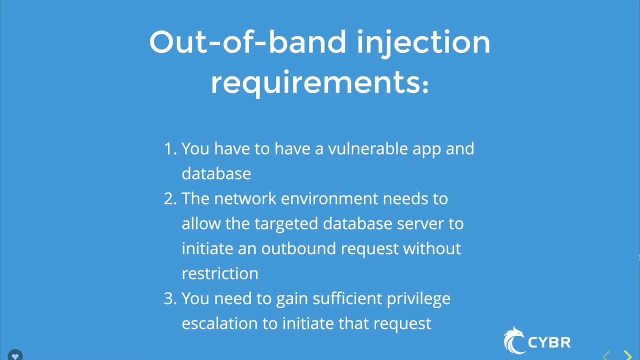 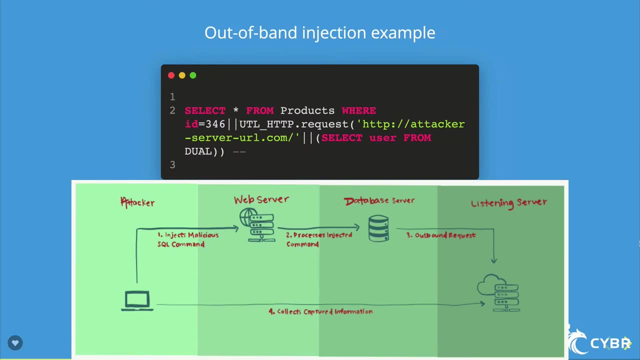 up security for the database was definitely sleeping on the job. But joking aside, let's see what this attack looks like. With this simple query, we would generate an HTTP request that contains a username, and we send that to the attacker's domain name, which in this case is attacker-server-urlcom. 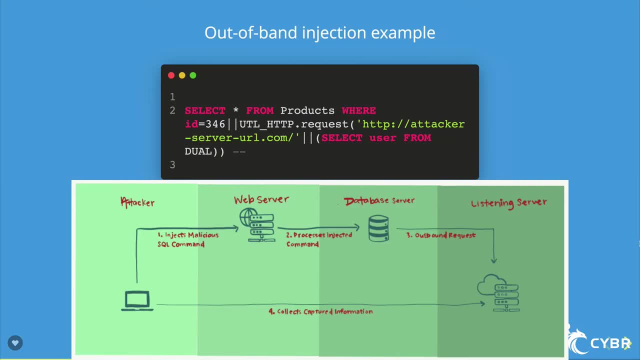 slash the username And since the attacker would be monitoring the web server's logs, they could see the database's username. Then we could do that with other information, piece that information together and we can continue on with further attacks. Next we have information. 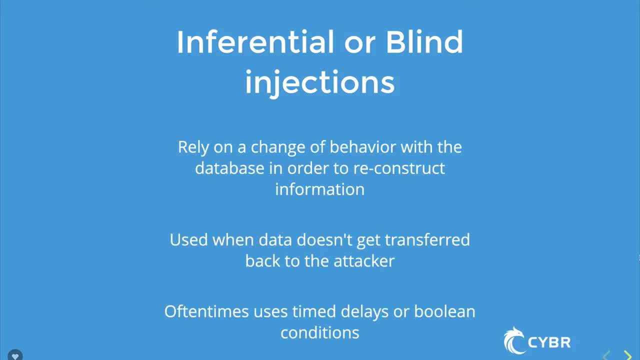 For example, if you're able to use an out-of-band injection, you can do that with an out-of-band injection. piece that information together and we can continue on with further attacks. And these attacks rely on a change in behavior with the database in order to reconstruct. 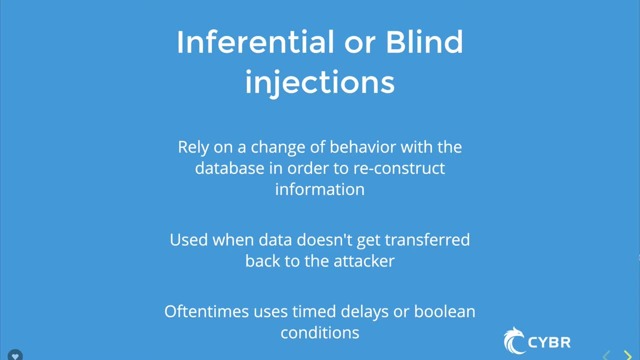 information, since the data will not be transferred back to the attacker, but they can guess what it is based on the response behavior. An example of this would be if you injected a time delay of, say, 5 or 10 seconds and the database took 5 or 10 seconds to respond back, then that would mean that there is a vulnerability. 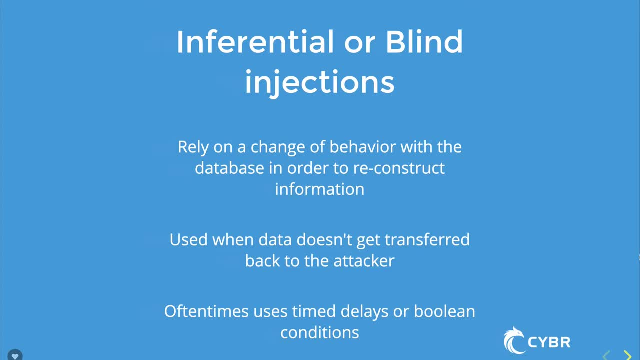 to injection, And this is usually regarded as a very slow method of attack. So if you're able to do that with an out-of-band injection, you can continue on with further. that requires a tremendous amount of queries, since the attacker oftentimes uses those time. 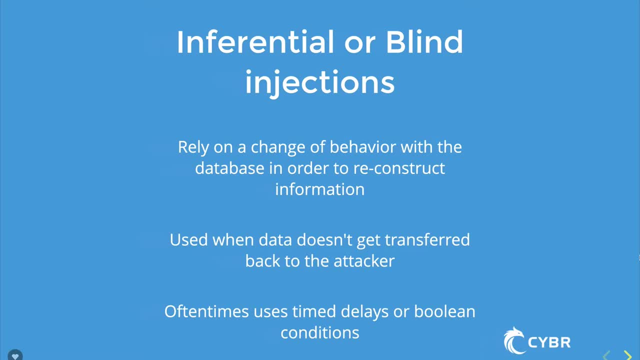 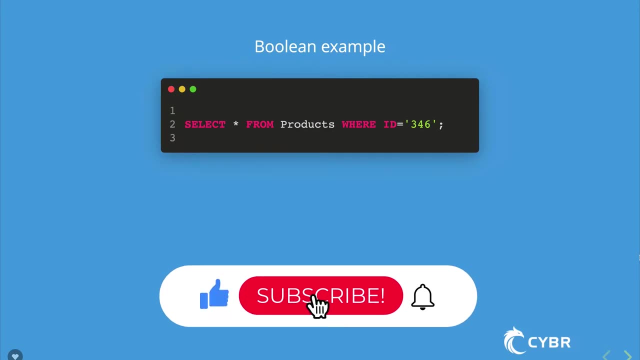 delays or true-false flags with Boolean conditions to make sense of the results. So let's take a look at Boolean conditions. If we remember back to the example from our prior lesson, we had this simple query which pulls all of the columns from the products table where the ID equals 346.. 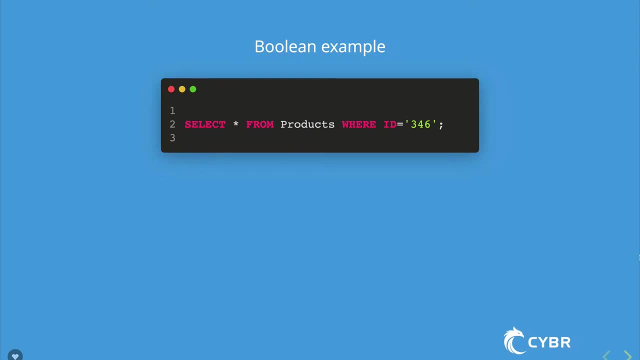 So in this case we might assume that we're displaying a product page for an e-commerce website and the user visiting your website- It selected a product with an ID of 346.. But let's say that they managed to modify the request going to your server from your. 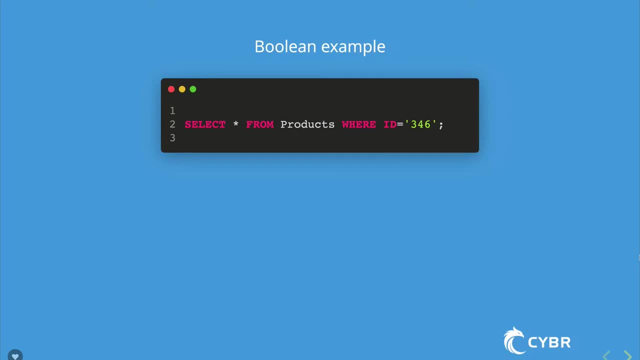 web application using a proxy tool like OWASP's app that we set up earlier in the course, And instead of sending ID of 346, we were to send this request where we have the product ID of 346, then a single quote, then a space represented here by the percent 20 for URL. 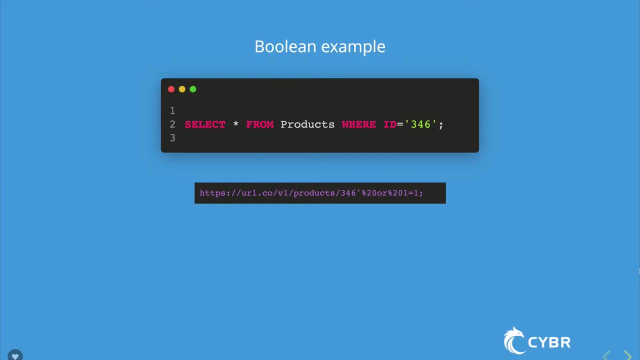 encoding, or again space, One equals one semicolon. Now the query becomes where ID equals 346 or one equals one. And since one does always equal one, that statement would always be true. And since we're saying where ID equals 346 or one equals one, the database will return. 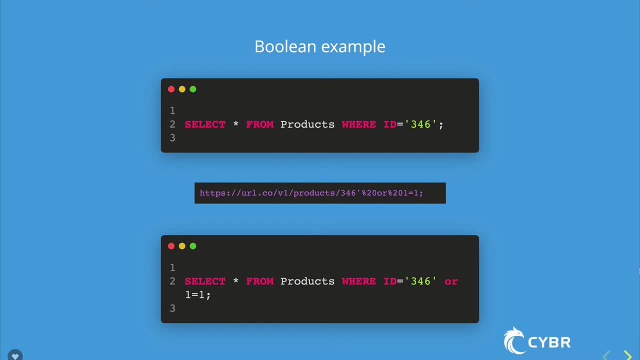 every single product in our database if it is susceptible to this type of attack, And this could mean that the user now has access to products that they shouldn't be able to buy or see, and perhaps even products that haven't been announced yet but that have all of the 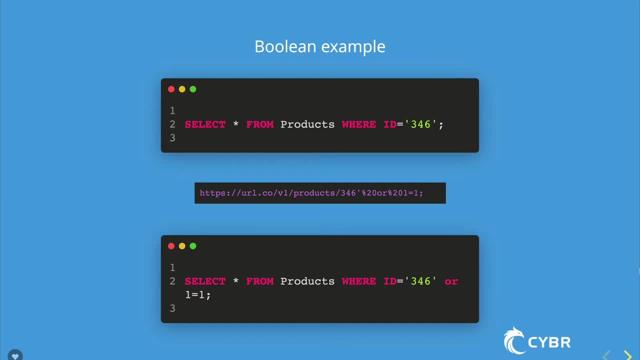 specs listed out in the database, and they can now sell that information to a news outlet looking to leak this story before anyone else does. So this is an example of a Boolean-based attack, since it uses the one equals one, which is true or false. 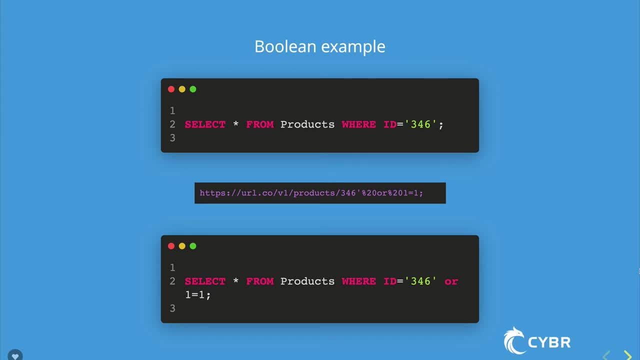 And this is a very basic example, but it is a powerful example because if the database is vulnerable to a Boolean-based attack like this, the attacker can immediately start to look for ways of executing the attack. So this is a great starting point when gathering information and when looking for vulnerabilities. 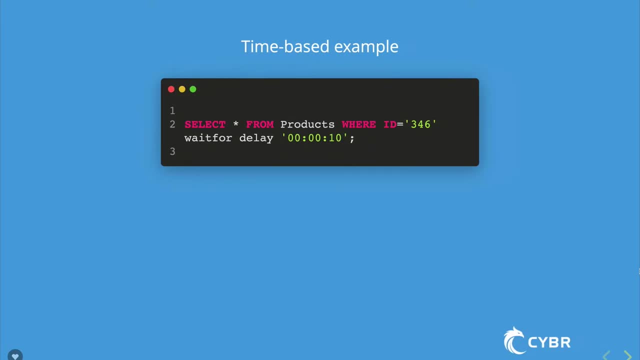 Next, we have time-based attacks, which rely on the database pausing for a specified period of time before responding, And doing this requires that you use the right operation, which will be database management system specific. so this would be an example of when knowing which database is powering. 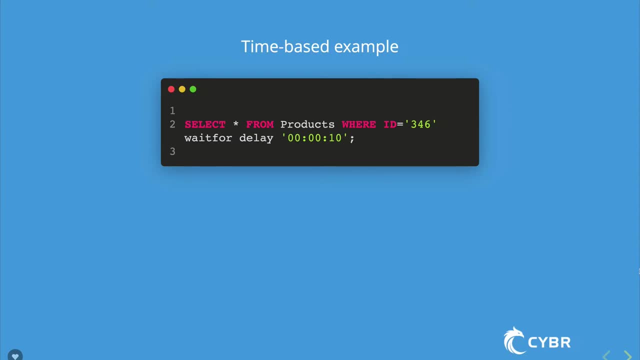 the application can really help out. For example, in SQL Server, we could use this query, where you have the wait for delay of 10 seconds, and if our injection is successful, the response will take 10 seconds, and that's how you know that it was successful. 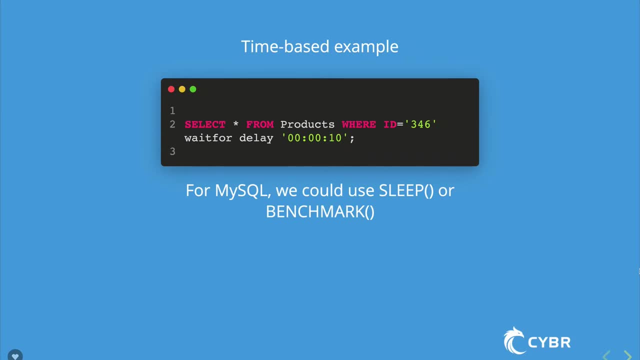 But for MySQL we could use something like sleep or benchmark. for example, if we're trying to guess a valid product ID in a table, we could put this attack together And we could have it to where if it's a valid user ID. then you would sleep for 10 seconds. 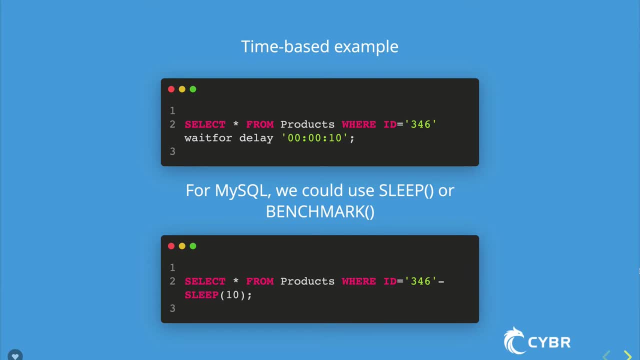 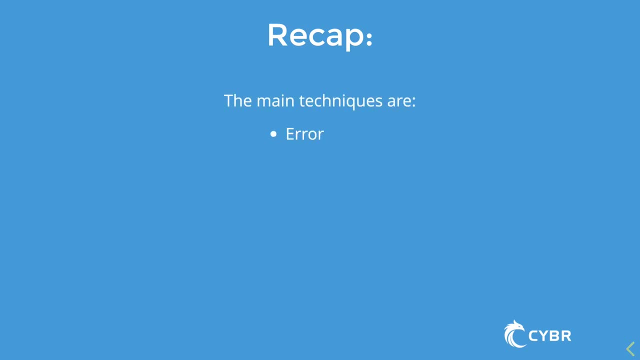 and if it's not a valid user ID, then it will return immediately and that's how you know whether it is or not. So, in conclusion, and to recap, the main techniques are error attacks, union attacks, boolean time delay and out of band. 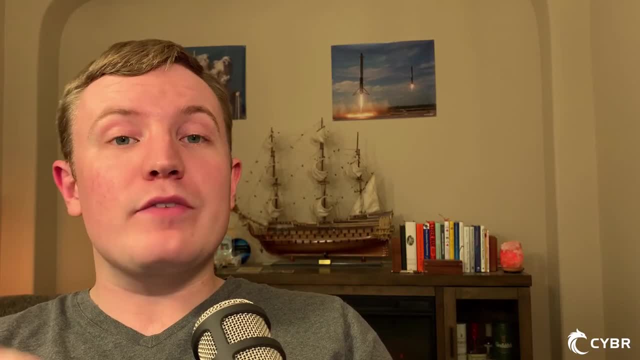 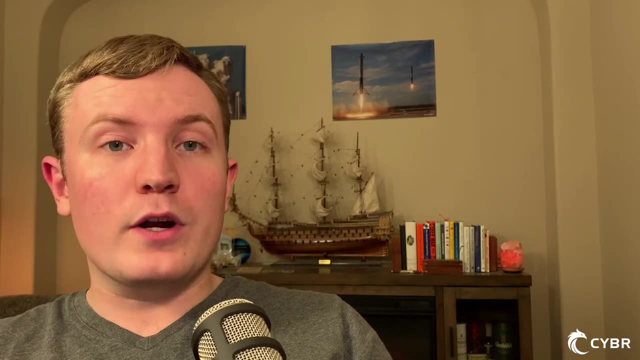 attacks. Now it is important to understand the various types of SQL injection attacks, because not all of them might work on different applications. Some attacks might work while others do not work, and so we might need to pull from these different techniques or even chain those techniques together in order to exploit a 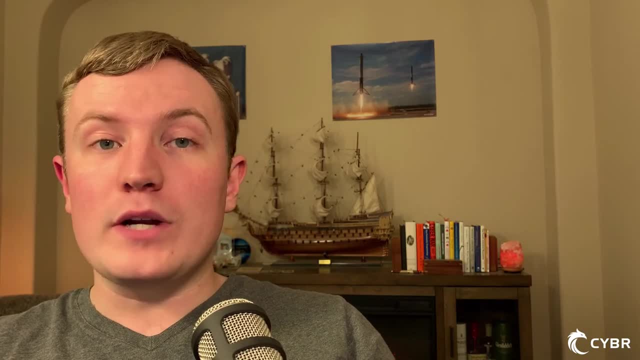 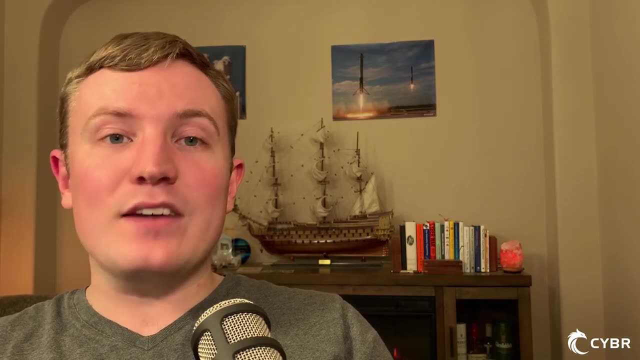 database and exploit an application. So, as we're testing our own applications, if we're doing pen testing and looking for vulnerabilities, we need to rely on all these types of different techniques and attacks, because that's what attackers might end up using against our applications. so we have 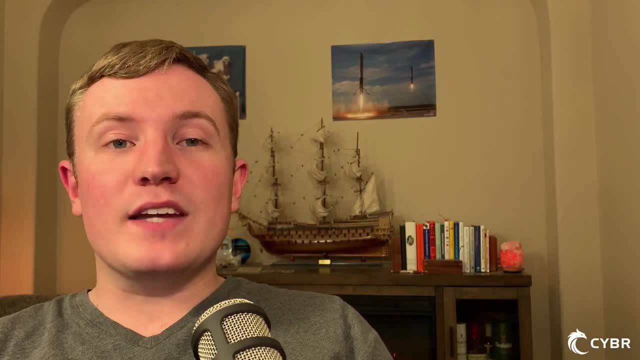 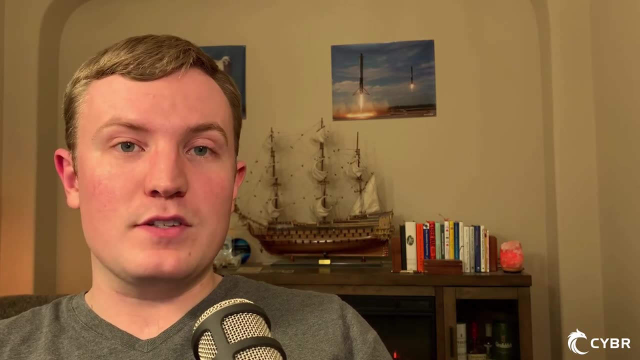 to verify for them. And now that we're familiar with the different types of attacks that can be carried out, let's take a look at how we can use the different techniques that we've been talking about with the help of cheat sheets and references, and those cheat sheets and references will be. 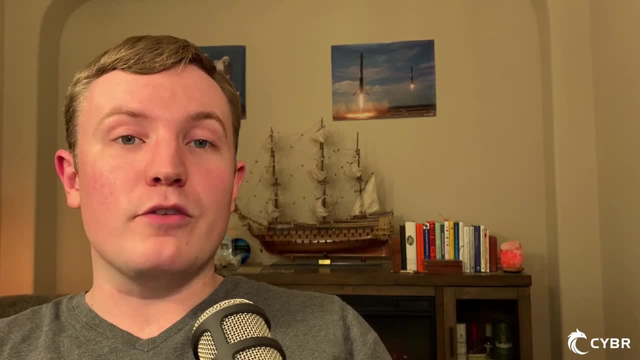 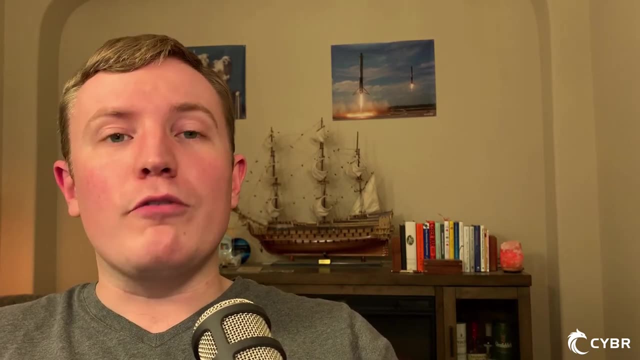 very helpful throughout the rest of this course and also throughout the rest of your career. So let's complete this lesson and let's move on to the next 1. We have to learn the differences in the syntax structure and available functions, depending 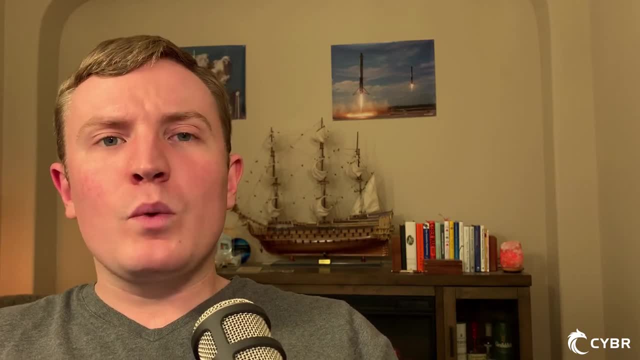 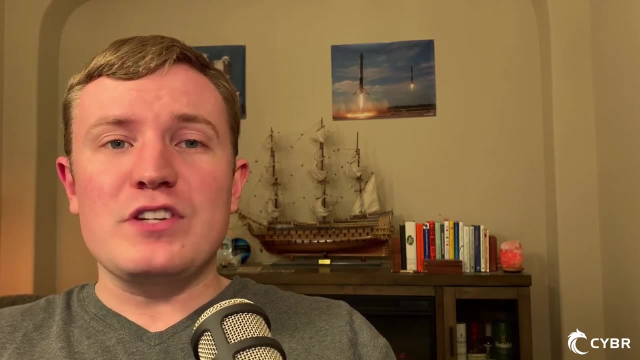 on the database management system that's powering an application. We have to learn the different quirks in order to effectively perform SQL injections, But most of us are not experts in every single database management system that's available out there, and that would take a very long time to gain that kind of knowledge. 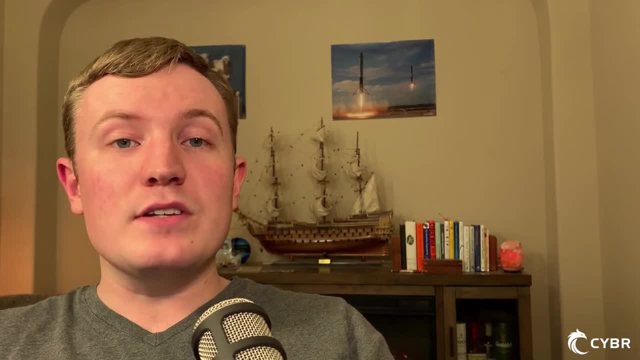 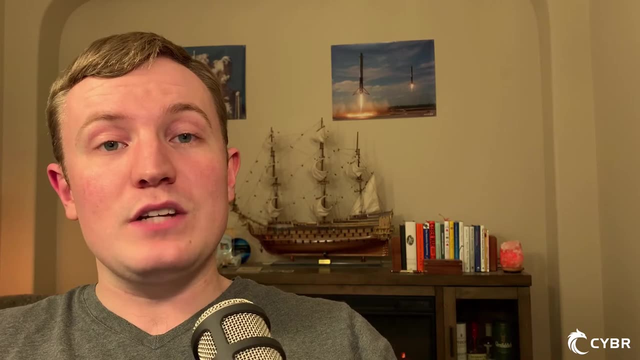 But, luckily for us, there are a lot of different cheat sheets and references that we can use and continuously reference, and which we will do in this course. So in this lesson we take a look at the types of cheat sheets and references that we can use throughout the rest of this section. 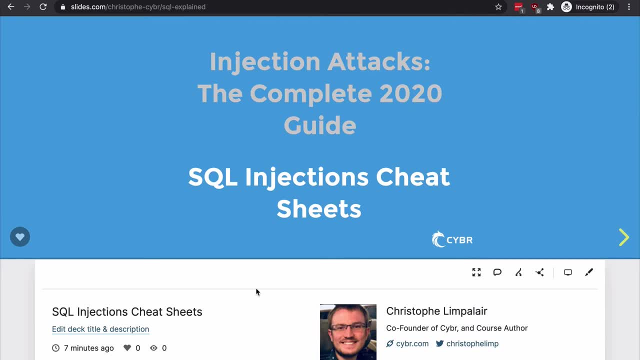 Now, I found all of these cheat sheets by just Google searching, so there are no paywalls or anything like that. these are all free resources And, by the way, I'll be sure to post this link so that you can go here and reference. 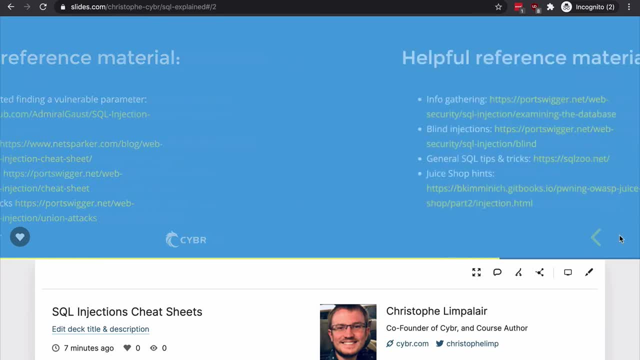 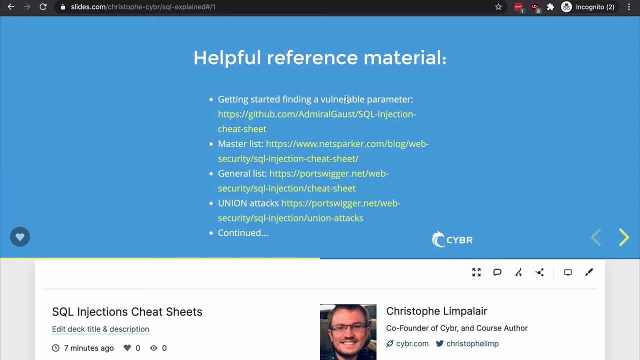 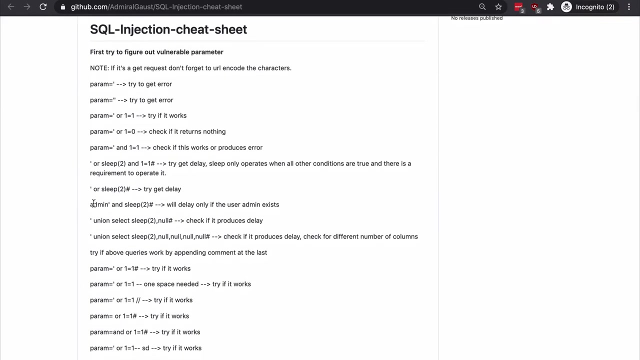 the material and click directly through these links. But the first cheat sheet we will look at is from GitHub and it's about getting started finding a vulnerable parameter. So if we go over to that cheat sheet, We can start from the top. As I mentioned in a prior lesson, one of the first steps that we will need to take to test 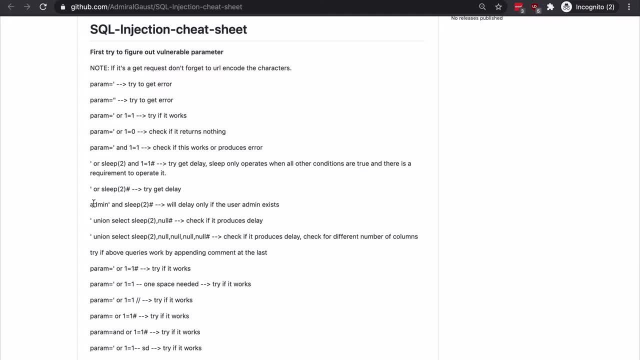 an application and its database for SQL injection vulnerability is to try to get any kind of non-expected response. Just think of this as prodding defenses to see if there are any weaknesses, And this first cheat sheet that we're looking at includes helpful inputs for that very purpose. 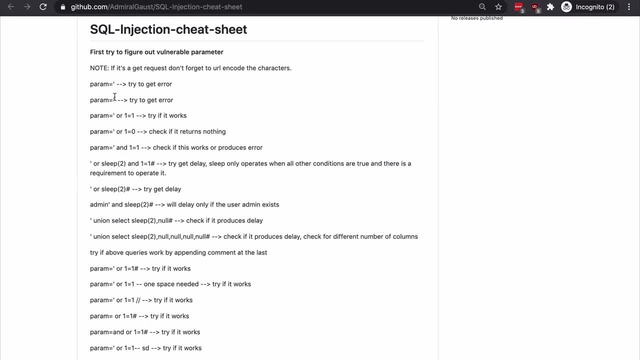 The first two parameters are a single quote and a double quote, which is trying to cause errors, so error based injections. Then we have single quote, or 1 equals 1, or 1 equals 0,, or single quote and 1 equals 1.. 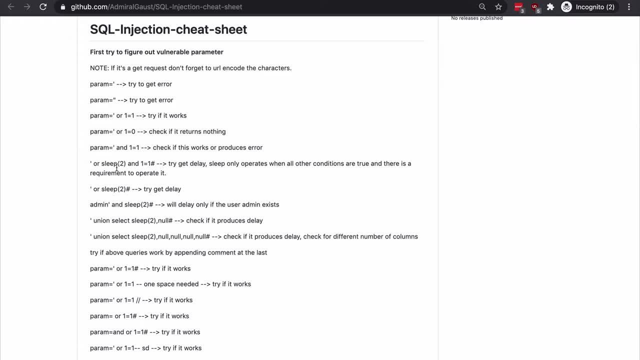 So in this case we're using boolean injections. Then they have single quote, still with: or sleep 2 and 1 equals 1 with the hash sign. And the same thing but without the 1 equals 1. we have or sleep 2 with the hash sign. 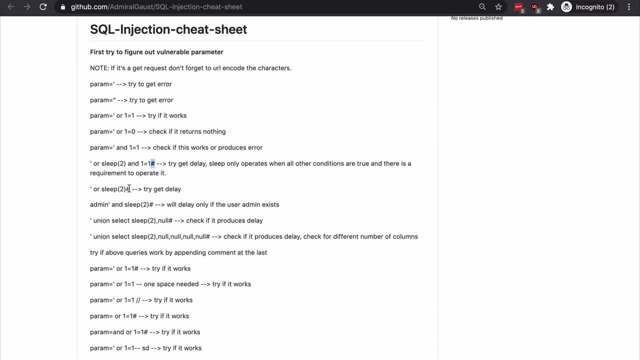 So in this case they're using time delay injections and they're also using the hash sign, which is for comments. if you're using MySQL, essentially causing SQL to ignore anything that would come after our injection- And we'll see this pretty frequently. We can also use dash dash instead of the hash sign for other database management systems. 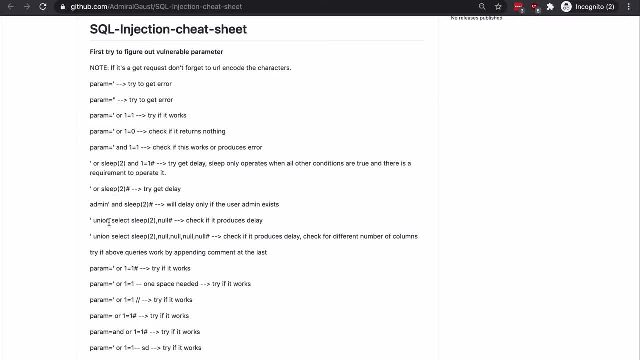 but we'll see this again in other cheat sheets. They also use a union injection with single quote: union select sleep 2 comma null hash. Here there's multiple nulls. we'll see this again, so I'll explain it a little bit more in a moment. 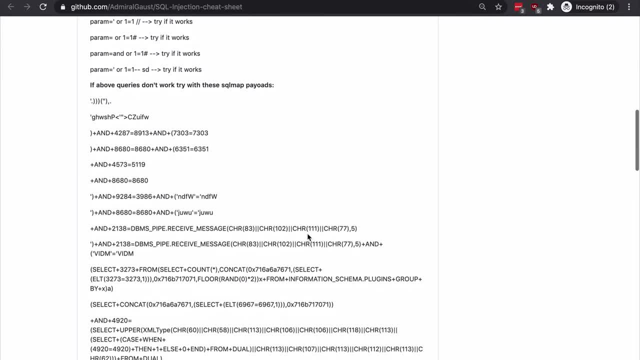 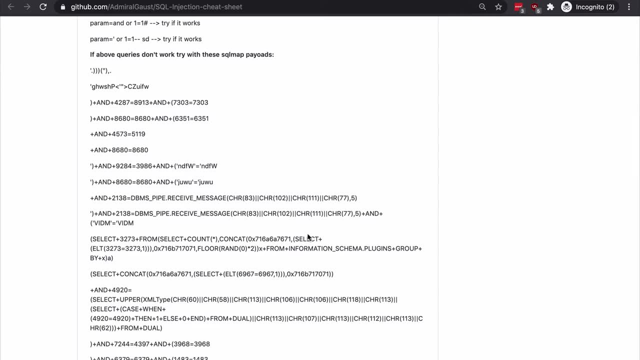 And then they have a variety of other types of payloads. Now if one or more of these inputs work, then we can use that to our advantage, but if none of those work, we can keep trying others. For example, this author included payloads from a tool called sqlmap, which we will take. 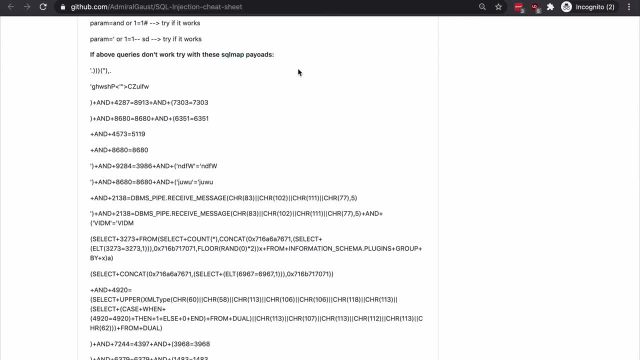 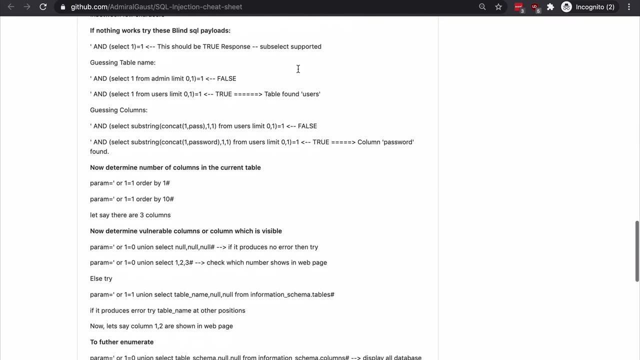 a look at in another lesson. Now these are some of the payloads that the tool uses to test for vulnerabilities, so they are also inputs that we can try to use manually, And further down there are other types of payloads that we can try, And then there are tips on how to determine the number of columns in the current table. 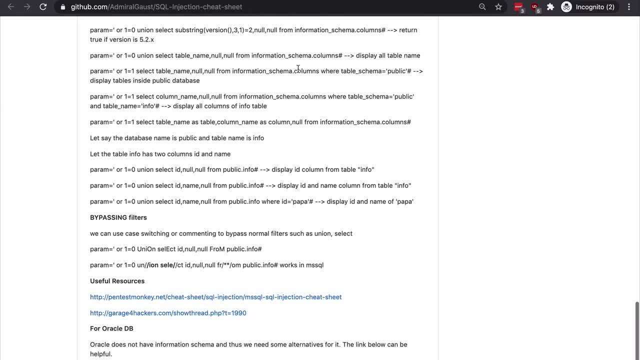 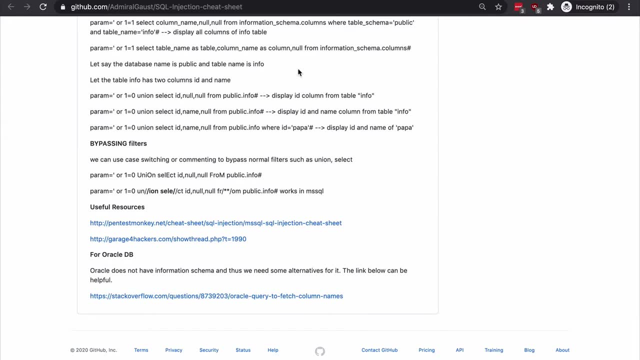 the available columns in tables, as well as displaying database column and table names through the metadata table, like we talked about previously. So this is a helpful cheat sheet and a great starting point. Next, we have what we'll call the master list, and I call it the master list just because 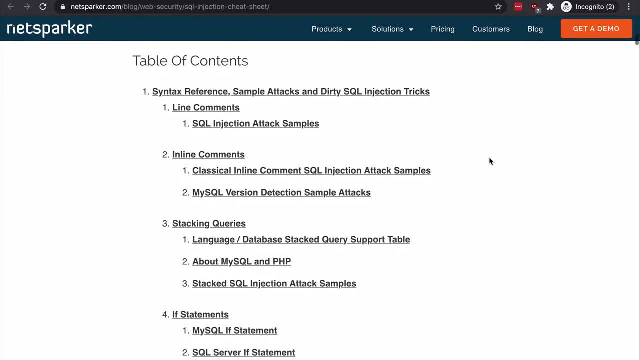 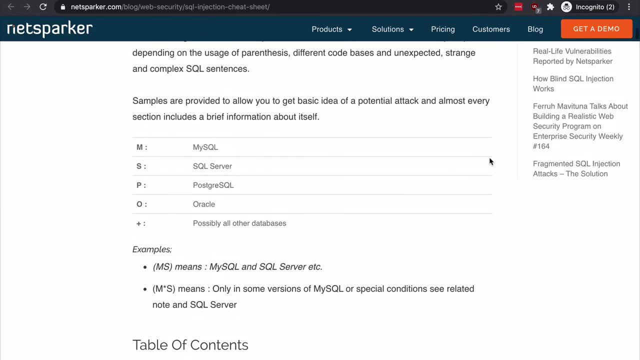 it's quite lengthy and also has a table of contents which makes it very simple and easy to jump around the different sections. They also include labels so that we can see what technique works for which database management system. They have a label of m for mysql. they have a label of s for sql server, p for postgres. 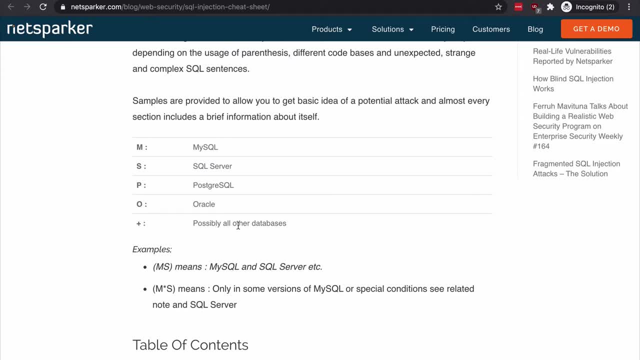 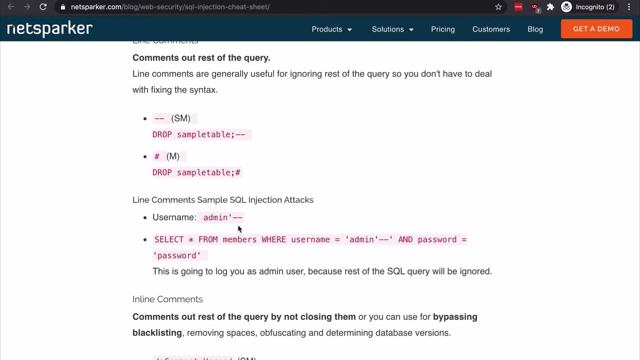 o for oracle and plus for other types of databases, And if we scroll down a little bit we can see what's going on. At the very top we have what we talked about earlier, which is commenting out the rest of the query. So when they have dash, dash. 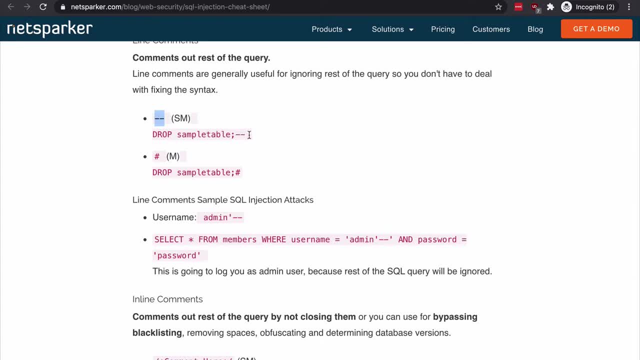 Like drop Sql table Semi colon, dash, dash. This would ignore anything else that would come after this query And since they put an s and an m next to it, it means that it works for sql server and for mysql And, by the way, this also works for sqlite, postgres and oracle. 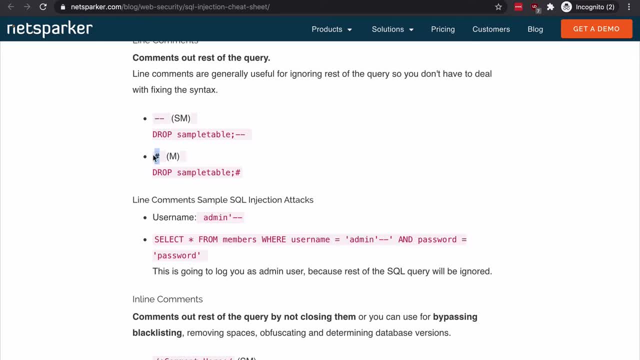 On the other hand, they have the hash sign, which also comments, but this time specifically for mysql. So, as we can see, this cheat sheet is not completely comprehensive and you have to verify some of the information, But it does give us a great head start. 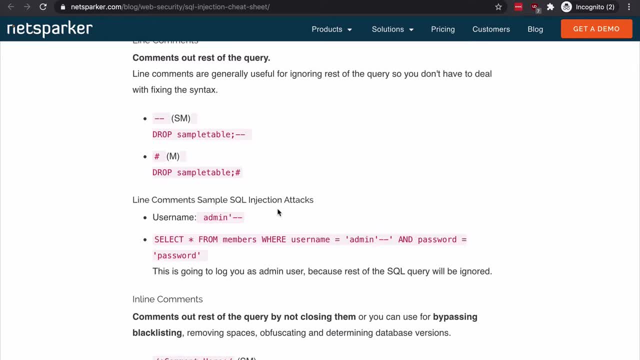 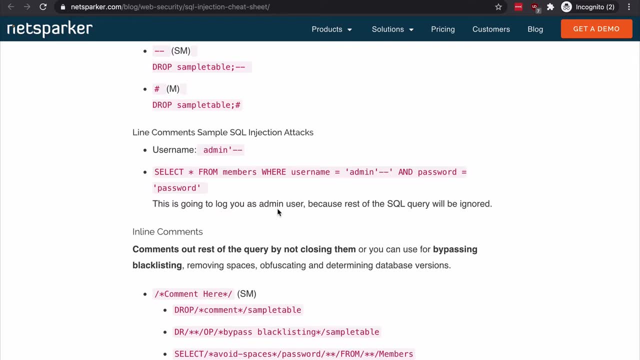 And it's a helpful reference material. And, by the way, they also include an example of when you could use commenting for an sql injection, And let's say that you try to log in as an admin user. If the app were vulnerable to this injection, you could type admin, single quote: dash, dash. 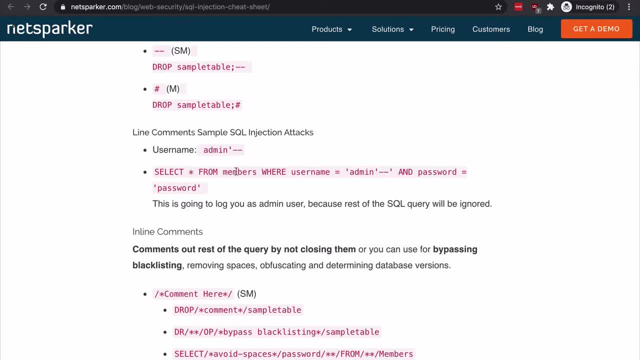 which would result in this sql query. You have select from members where username equals admin, dash, dash and password equals password. But again, because this is what's triggering a comment, Everything Afterwards is considered a comment. So what we end up with is select from members where username equals admin. 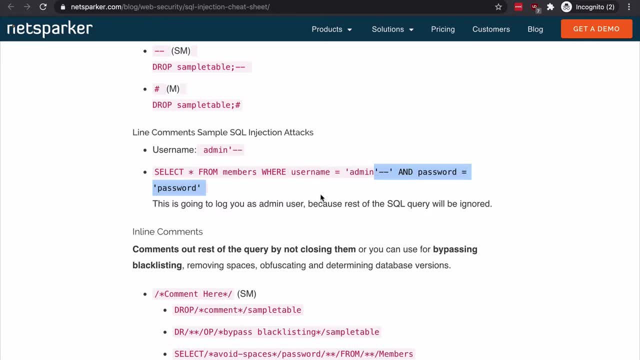 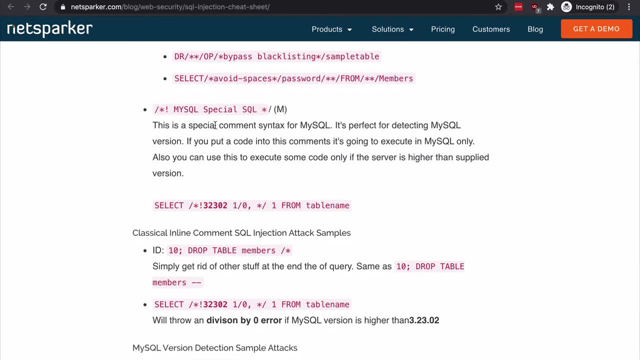 And then everything else is commented out, Which, again, if this is vulnerable to it, would allow us to log in as an admin. Another comment that they include here, which is kind of interesting, is specific to mysql, And so we can use this to try to determine the version of mysql that's running powering. 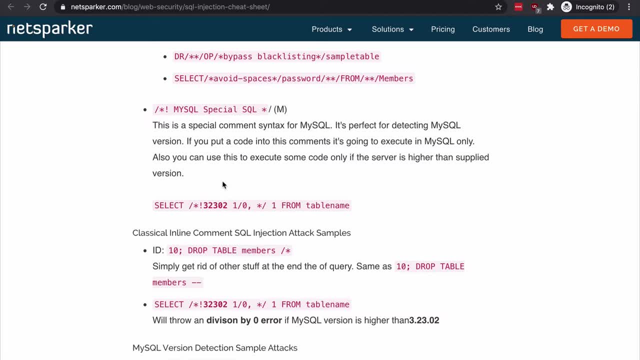 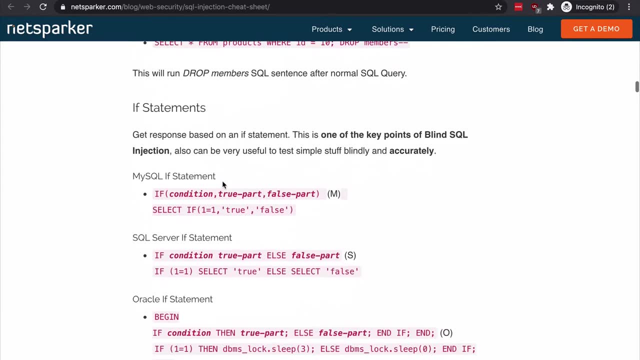 that application Which, again, If we don't know the specific version, we can look up for specific vulnerabilities to that version. There's a whole lot more to this article that we're not going to cover in this lesson, so please spend a little bit of time scrolling through and taking a look. 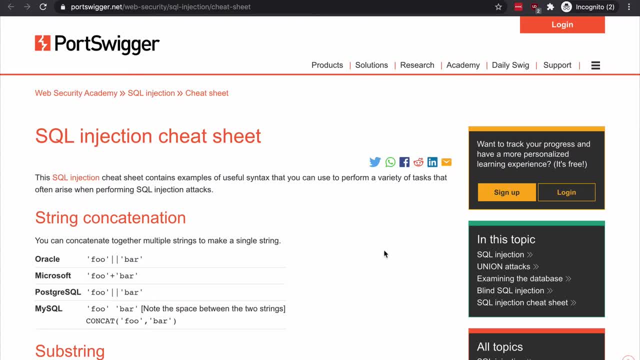 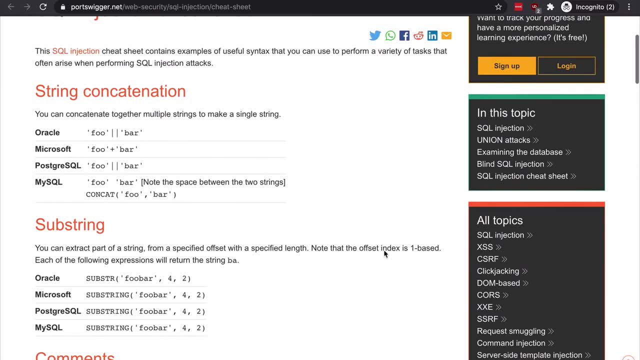 But next we're going to move on to what I'll call our general list, And this is created by a company called Portswigger, who also created burp suite, And here they include tricks on how to perform things like string, concatenation, substrings. 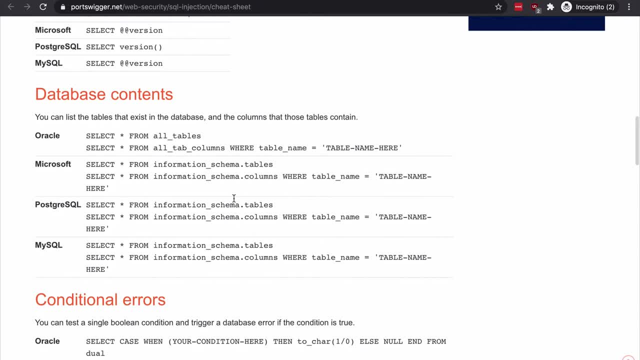 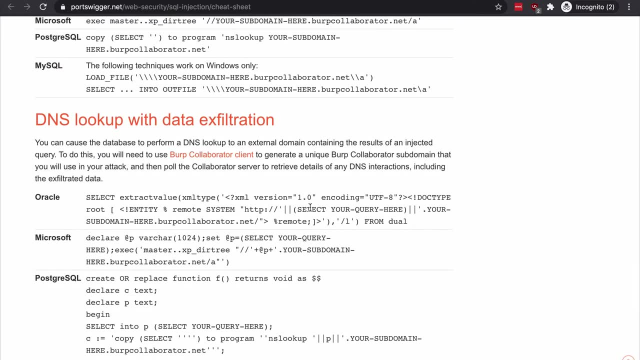 comments, like we just saw, Pulling up database versions Or database contents, like we've talked about Conditional errors, batch queries, time delays and more. Now we've seen these tips, or some of these tips, on other pages, but I found that the 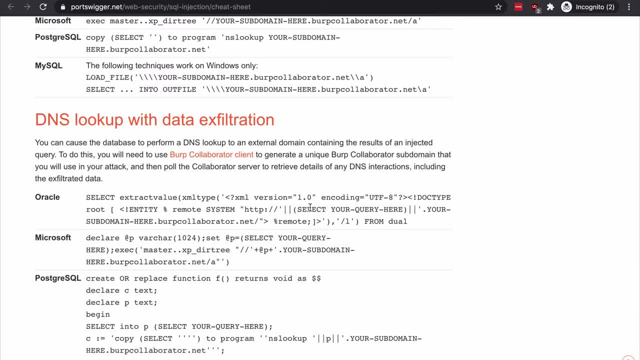 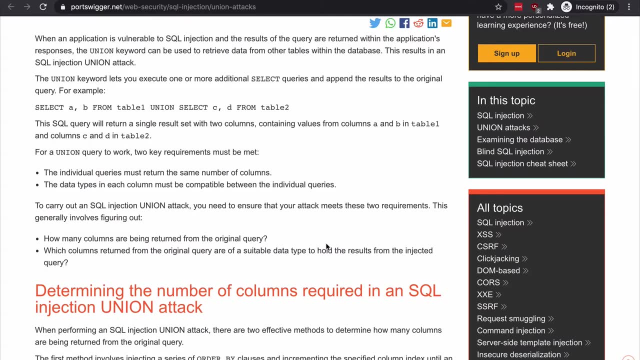 format is quite nice, so I did go ahead and include it here. Next, they also have a page dedicated to SQL injection union attacks. This is one very helpful cheat sheet, as you're doing union attacks, and I do recommend that you take some time reading through this reference, but I will point a few things out. 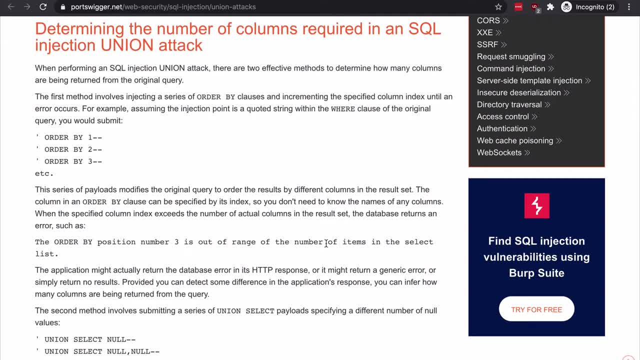 Here's the key: When performing a union attack, you have to match the number and the data type of columns from the tables that you're combining. That's why it's important to determine the number of columns that are being returned from the original query, and they list two methods here of doing that. 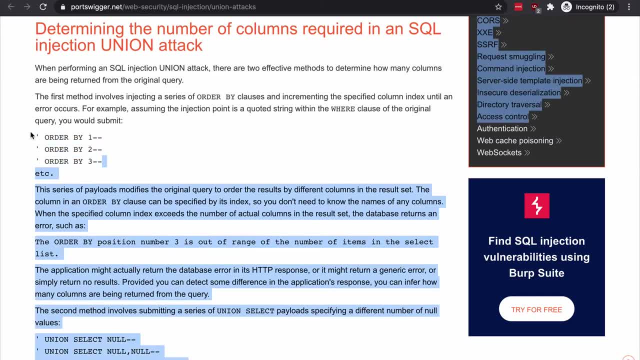 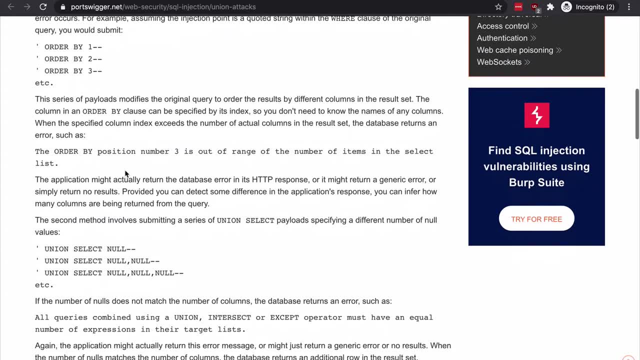 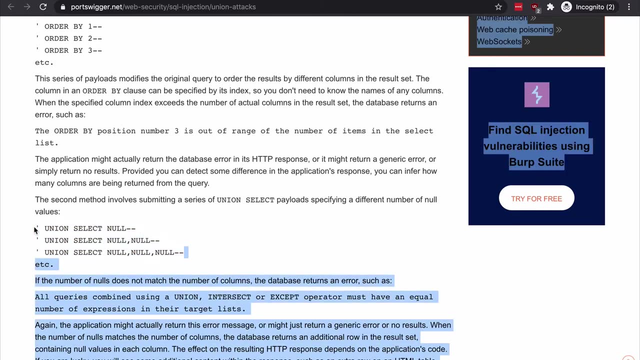 The first method injects a series of order by clauses and increments the column index until an error or change in behavior occurs. The second version is submitting a series of union select payloads: payloads with a different number of null values until you get an error or change in behavior. 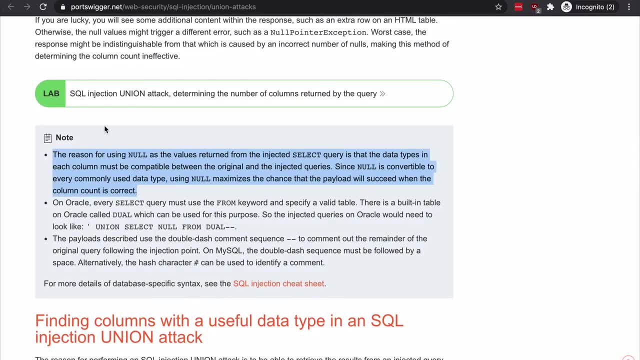 And, by the way, and they also explain this on this page- but the reason that you would use null is because it's very helpful with union attacks, since null can be converted to every commonly used data type, so it maximizes our chances of success. if we don't know, 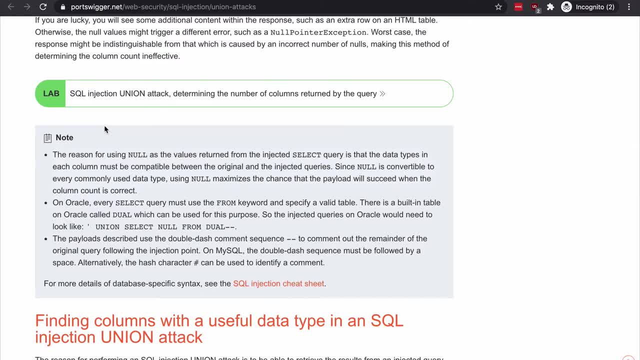 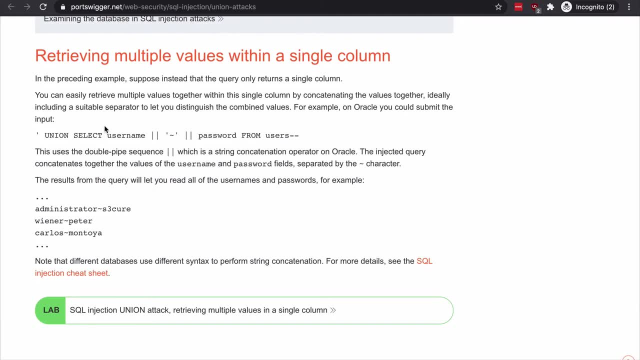 what each data type for each column is. Also, if you ever run into a situation where the legitimate query only returns a single column and you're trying to extract multiple columns worth of data, you can use the concatenation trick that we saw previously to combine results into one column. 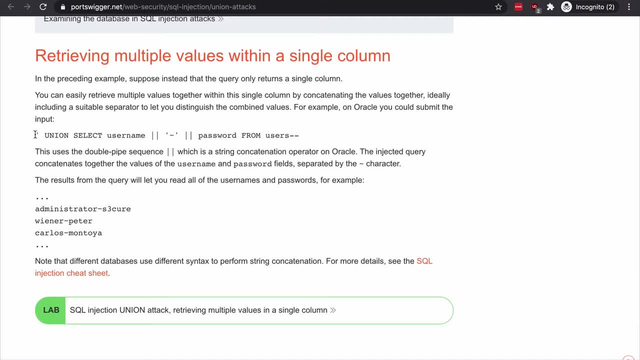 And their example here shows that they combine the username and passwords from users and they use the tilde to combine the results, which also makes it much easier for us to separate out the values after we've extracted the data from the database. The next cheat sheet that I include here is also from Portswagger. 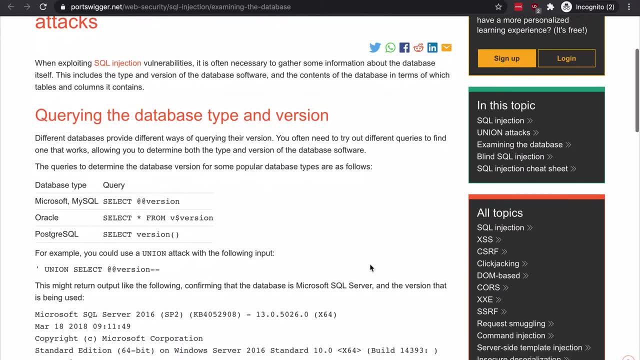 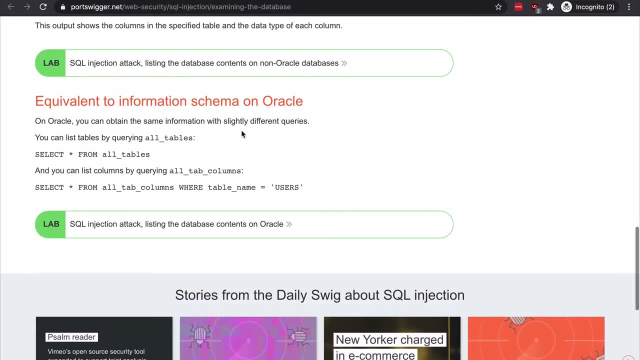 But in this case it is used for information gathering, such as querying the database type and version, listing the contents of the database- and we've already seen this before- and the equivalent for Oracle Database- Again, we've seen this, but I really like the format of how they put this on the pages. 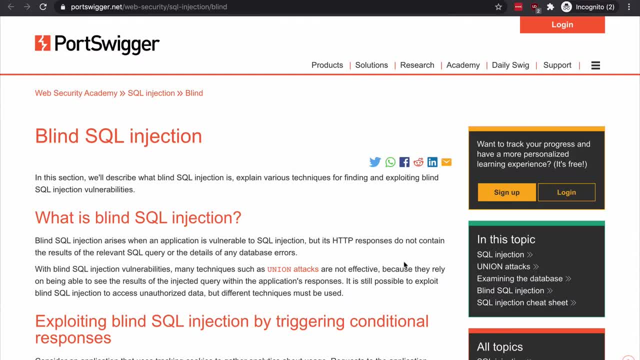 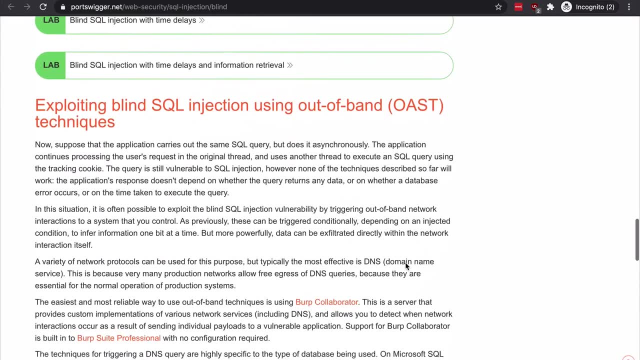 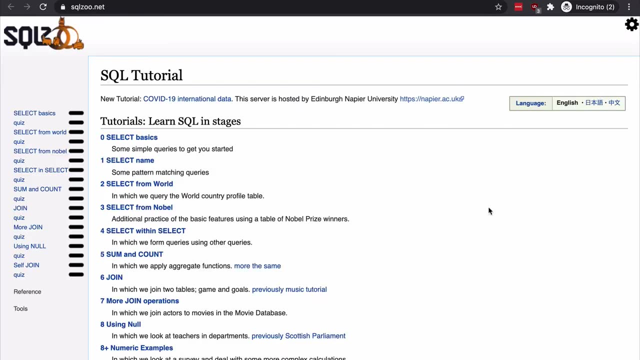 so I've included here for your reference. Next, they have one on blind injections- Again same thing, and they include things around conditional responses. so another helpful resource in a pretty simple way, And I've also included a list of general SQL commands, tips and tricks that contain: 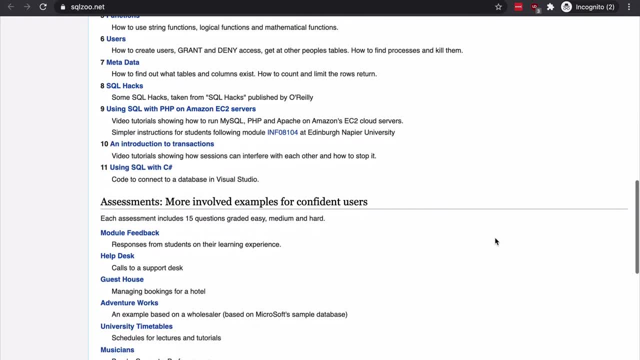 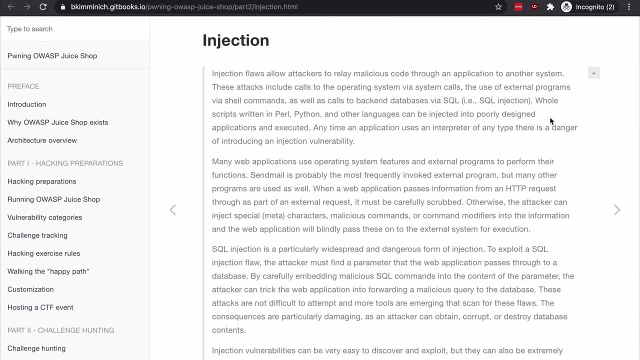 helpful information, not just for SQL injections, but also for general SQL usage, So feel free to reference that if you'd like. And finally, as we prepare to launch hands-on attacks against safe and legal environments, I wanted to share this cheat sheet for the OWASP Juice Shop injection attacks. 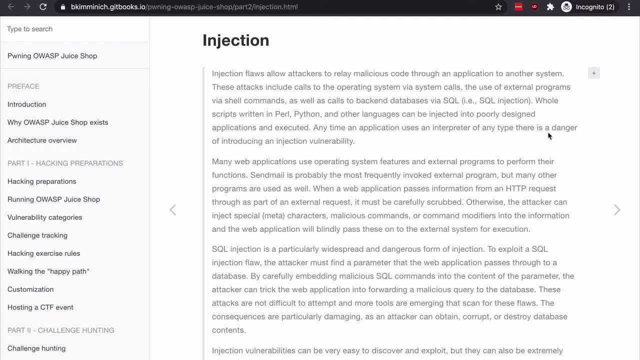 The OWASP Juice Shop is one of the environments that will be used to store and store data, the environments that we will be using throughout this course, and they provide helpful hints throughout this documentation to help us uncover and then exploit SQL injections in the application. 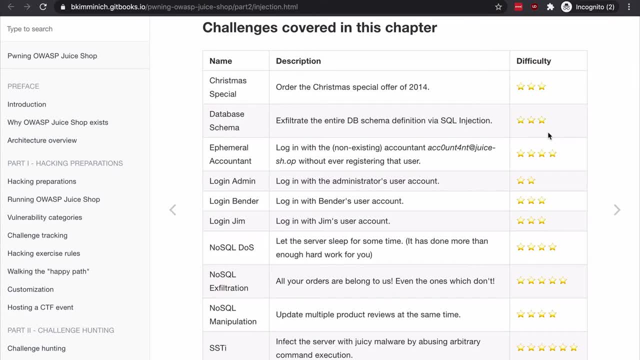 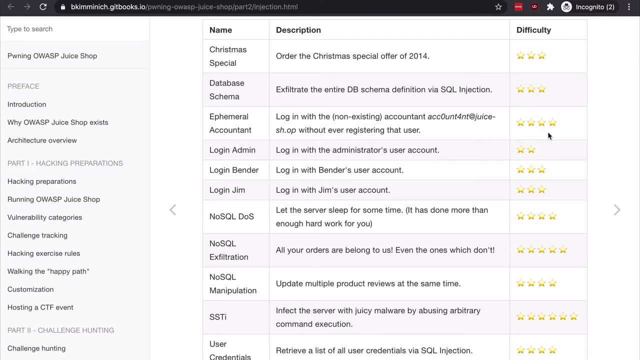 It also includes a list of the challenges that we'll find in the osp-juice shop that are relevant to SQL injections, as well as their difficulty level. So, as you complete this lesson, be sure to spend some time reading through these references. 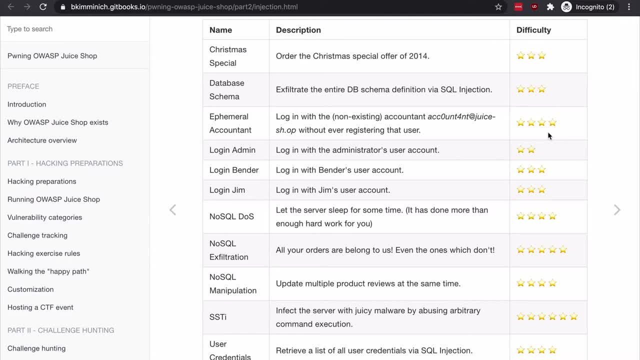 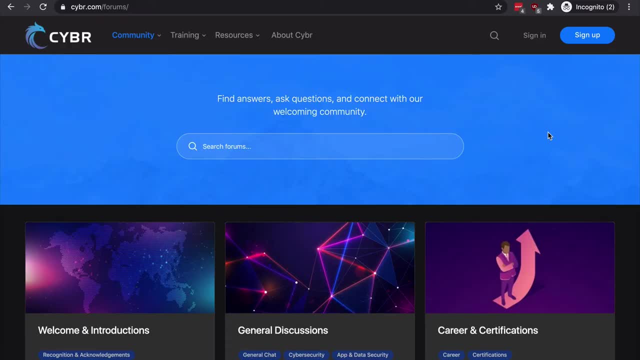 because in the next lessons, we will use knowledge from everything we've learned to this point in order to gather information and then exploit applications and databases. And, by the way, if you find or know of any other cheat sheets that could benefit the community, please do share with us at the cybercom slash forums. 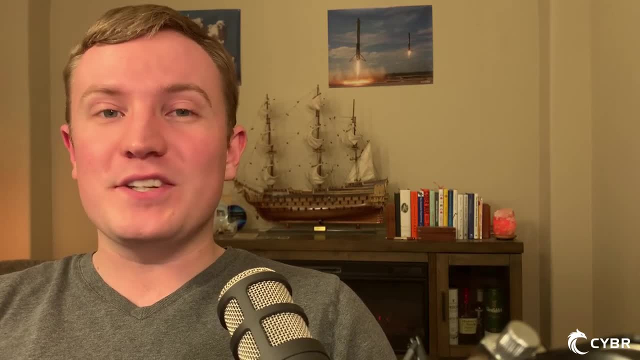 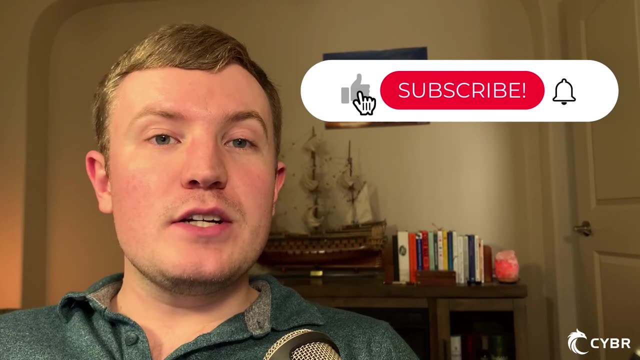 Now, with that, let's make sure that we bookmark these references, and then let's complete this lesson and move on to the next. Now that we have our environment and tools set up and configured and we've learned the concepts of SQL injection, it's time for us to do information gathering before. 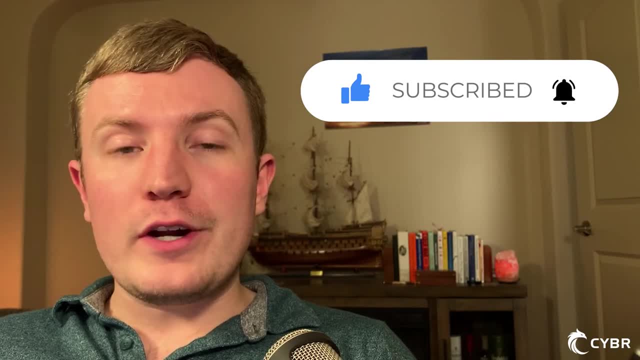 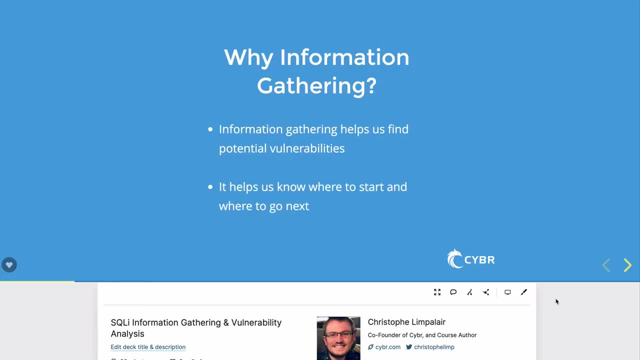 performing our main attacks. Information gathering will help us find critical information about how the application runs, the technology that's powering the application, and potential vulnerabilities, And this, by the way, is an important step, not just for SQL injections. So, while I would normally do much more information gathering to find other kinds of potential, 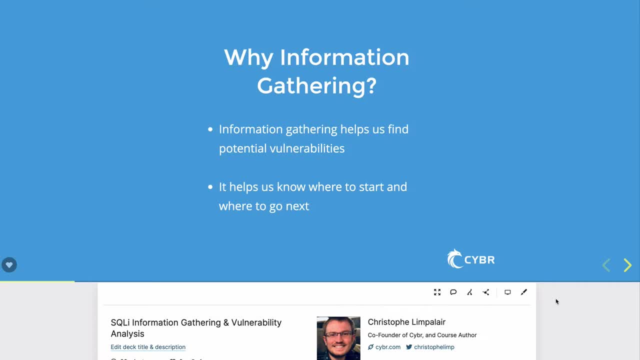 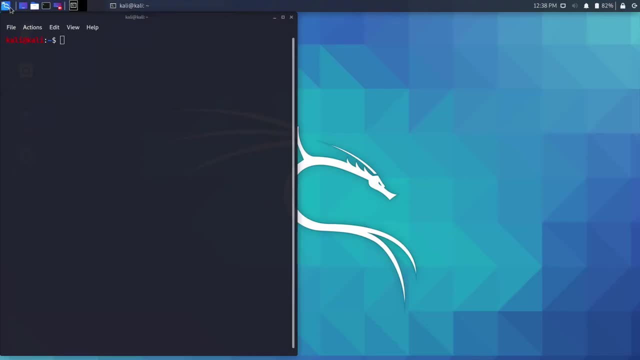 vulnerabilities. I will keep this lesson more focused, But without information gathering, you wouldn't know where to start or what to do next, so it is a very important step, And there are multiple ways of gathering information, one of which involves osp-zap. 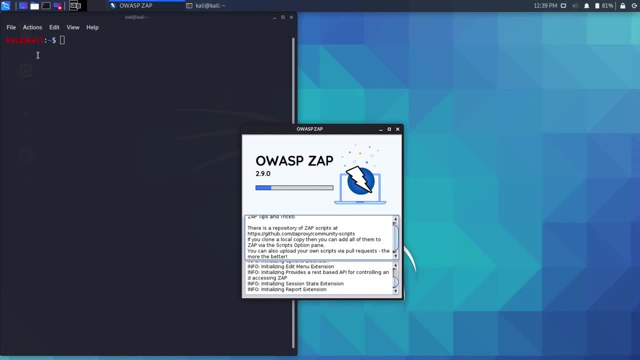 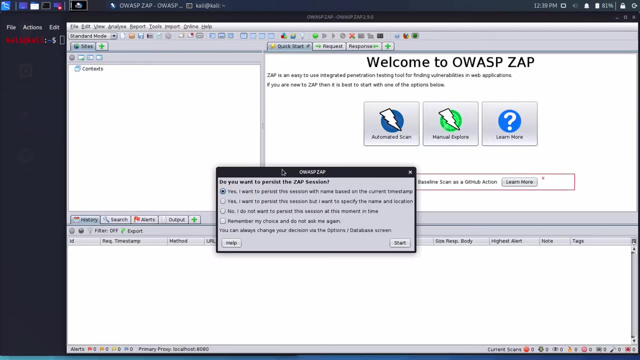 With zap, We can use the automated website scan in order to crawl all of the links that it can find from the website. Then the scan looks for vulnerabilities in the links that it found using techniques such as fuzzing, And we could manually use fuzzers, and zap provides that functionality if we wanted to. 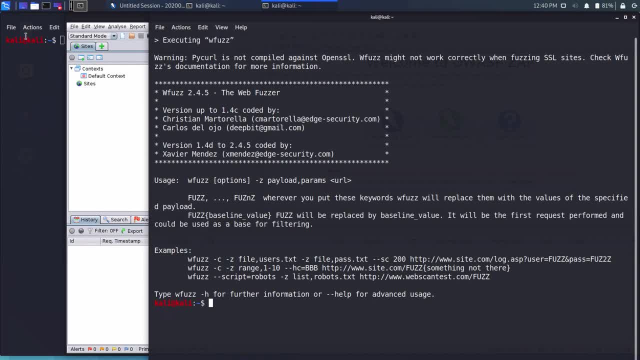 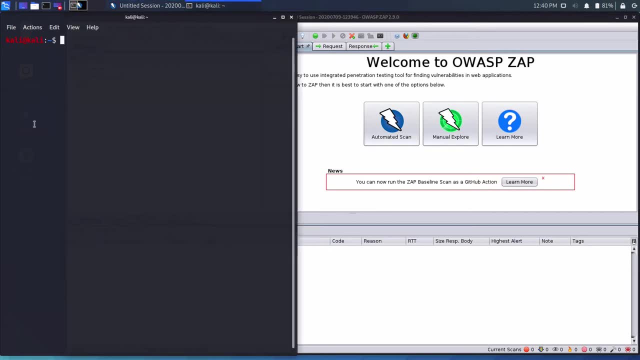 use it that way, and there are other tools made for that very purpose as well. Now, if you don't currently have the osp-juiceshop application running yet, let's go ahead and do that now. As long as you followed the steps from a prior lesson, you can type systemzap. 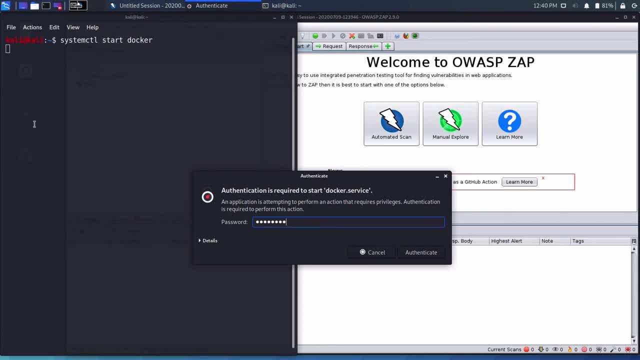 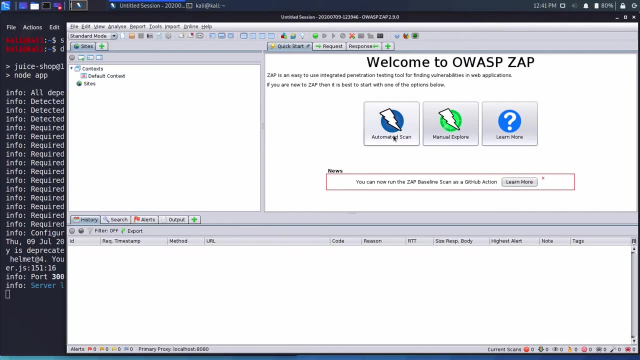 ctl, start docker. it will ask you for your password and then we can go ahead and run the container with docker. run dash, dash, rm, dash p at port 3000, and then we'll pull in the image And once it's running we can go back to osp-zap and we can start an automated scan. 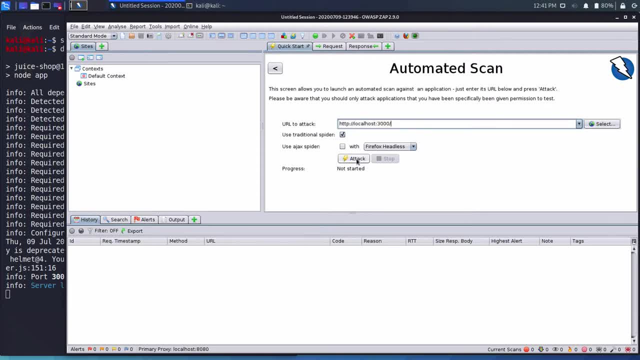 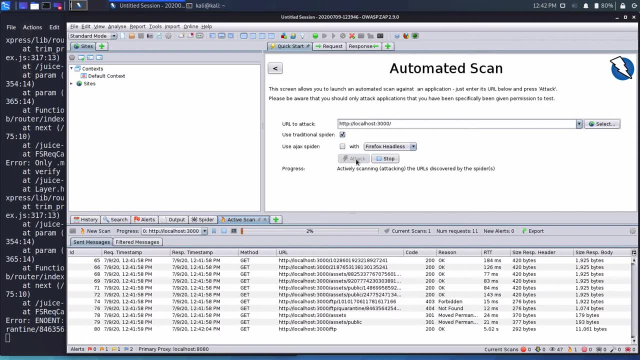 We'll type in localhost, port 3000, and then we can start the attack. Now, this can take a while, so we're going to start with that and then we're going to let it run in the background. And another step we can take to gather information, of course, is manual exploration. 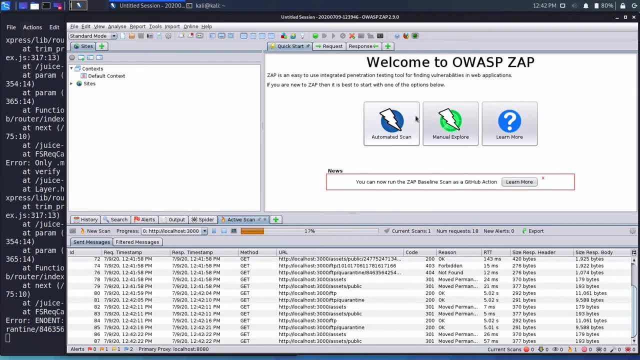 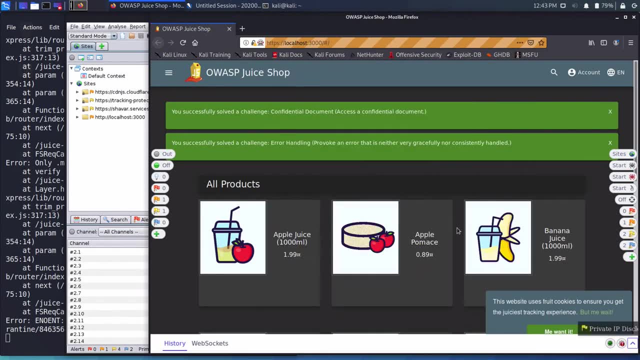 So, while the active scan is going on, let's go ahead and do some manual exploration of the osp-juiceshop, And as we perform manual exploration to find potential SQL injection vulnerabilities, we need to think like a developer. what I mean is that we have to try and we have to think. 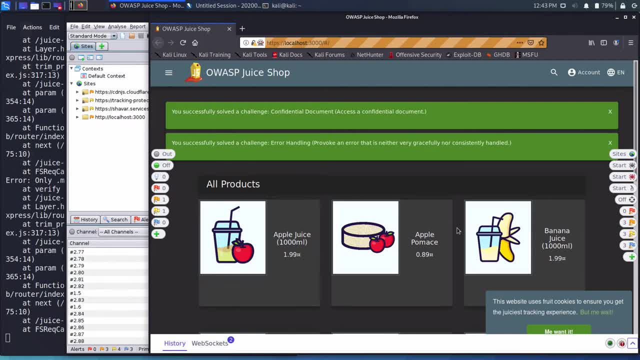 about how the target application works, such as when it might be making database calls and what kinds of calls they might be making. So look for things that stand out and then take note of any time you see any input field, such as a login form. 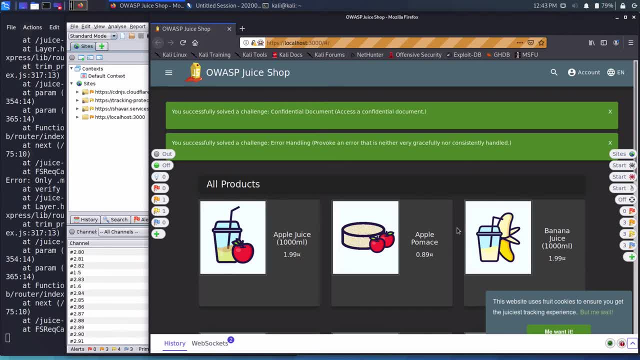 search form or anywhere that is likely to be pulling from some kind of database. So at the very top we can see that there's a search icon which is likely searching from a database. so that is a potential place of attack. In fact, let's go ahead and try some error based attacks and I'll go ahead and pull up. 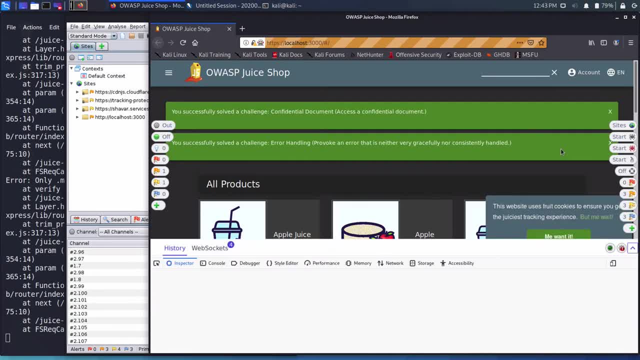 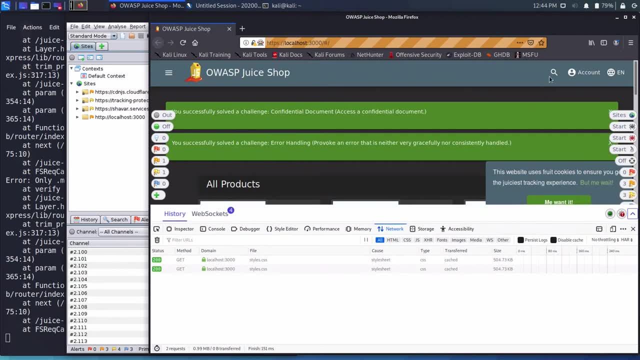 the network tab from Firefox in order to see what kinds of requests and responses are going through. So I'll open this back up and then I'll just put a single quote and press enter. So we can see here that a GET request was made to search. and if we look at responses, 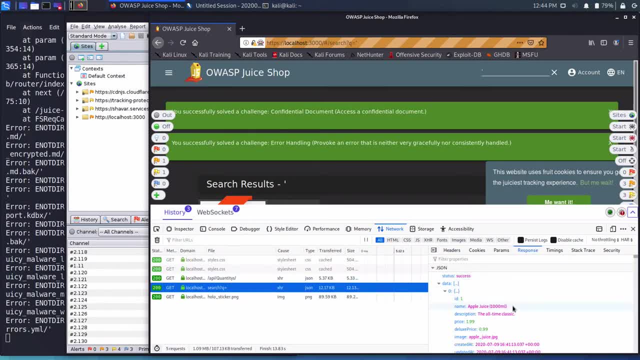 we'll just see that it responded with JSON that says a status of success and then a bunch of data that contains different products. So it looks like it's returning a normal response and there's not much else going on here And, by the way, it's showing that we solved. 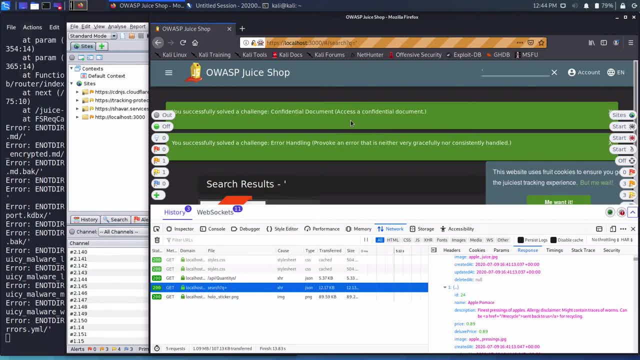 things here, but I'm pretty sure this is happening from the automated scan, not what we just performed, so don't get confused by that, But also, by the way, this is where something like the OWASP, ZAP, HUD can really help us out. 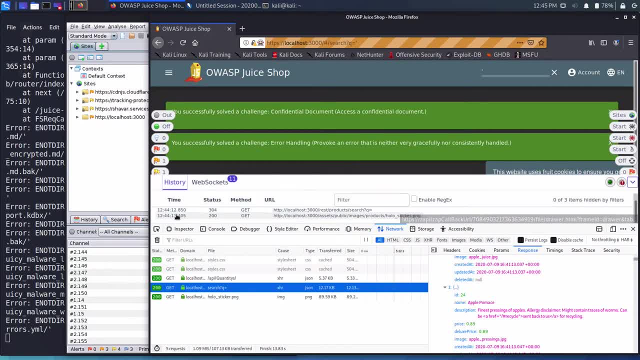 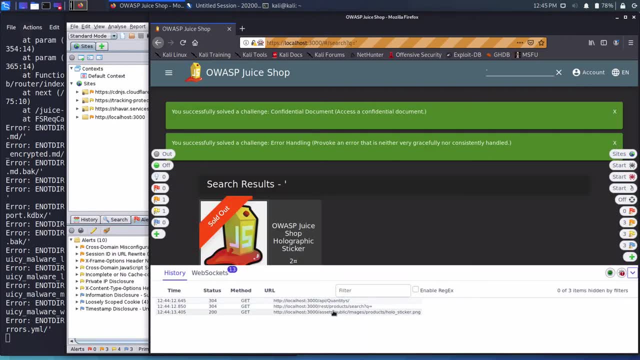 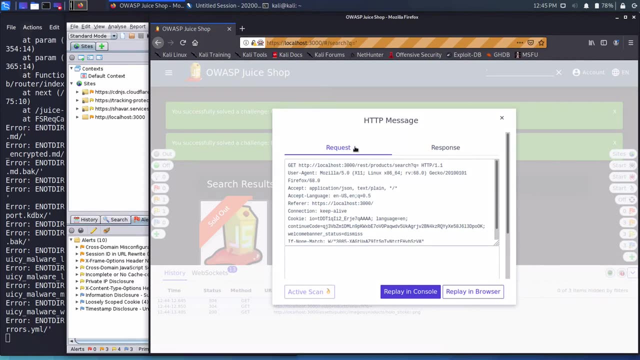 because ZAP actually includes something called history. So if we click on history here and I close out the networking tab, we can see a history of our requests. So this is very similar to the network tab, except we can do more with it. For example, if I click on that search query, we can see the request. 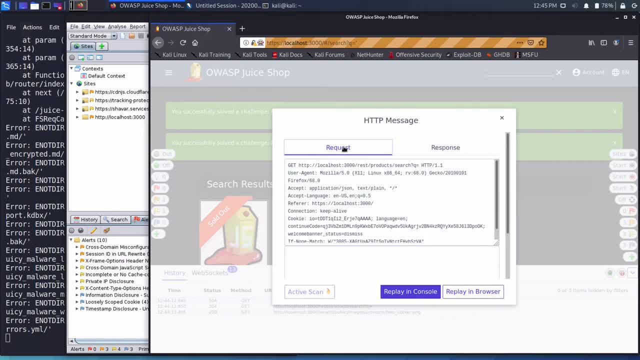 and then we can see the response. Better yet, we can actually modify the requests, and then we can replay them, either in the console or replay them in the browser, And one of the reasons we want to do this, by the way, is because we can now communicate. 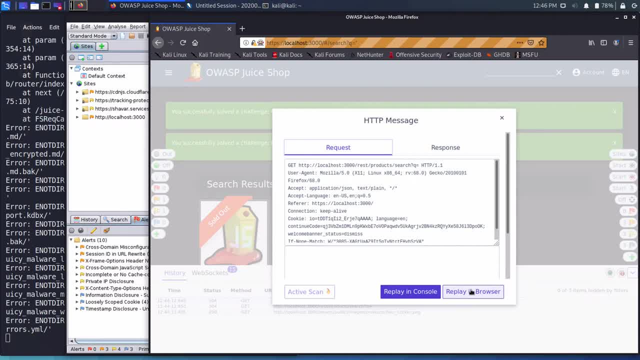 directly with the application's APIs instead of going through the potential front-end security controls. So let's try a different attack just by using double quotes now, And I'll go ahead and replay in the console. We see again a success with the same data. 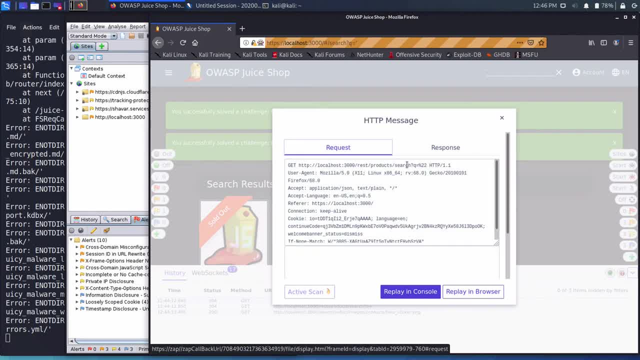 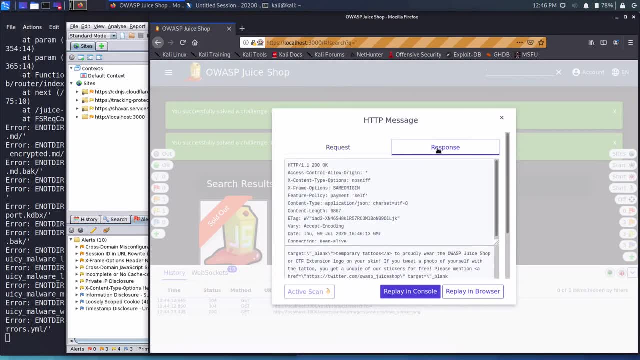 So this didn't seem to work, But if we look at the request, by the way, you will see that it properly URL encoded the double quotes. But again, no errors have been shown yet. However, we do have some interesting information already. If I make this a little bit smaller so that we can see the JSON: 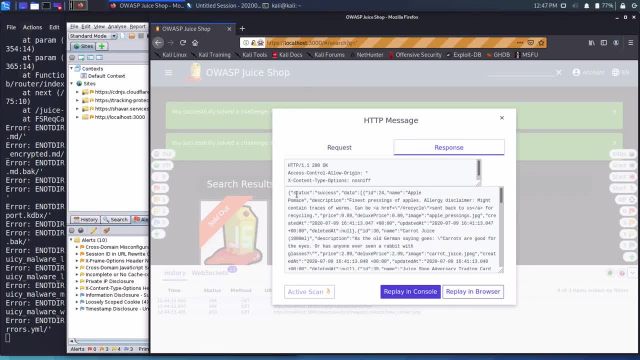 I'll point out what I mean. Let me scroll all the way back to the top, And it can help us understand how data is structured and how it might potentially be stored, Because, while it's possible that the API structured this data differently than it was stored, it's also entirely possible. 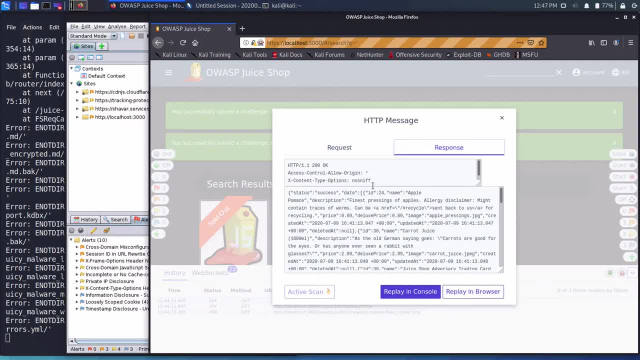 that it closely resembles the database structure. What I mean by that is we now know that there's an ID for each product. There's a name for each product, a description, a price, a deluxe price, an image, a created at date and timestamp, Same thing for the updated at, And there's also a 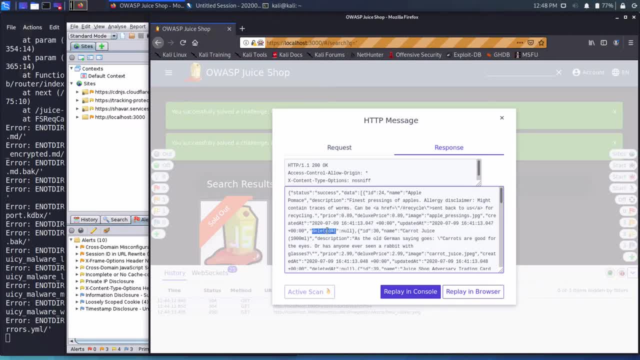 deleted at. So right off the bat, that's a little bit strange to me, because there is a deleted at column which tells me that there's probably this parameter that's hiding products that have been deleted and should no longer be available to customers. So that's interesting to know. 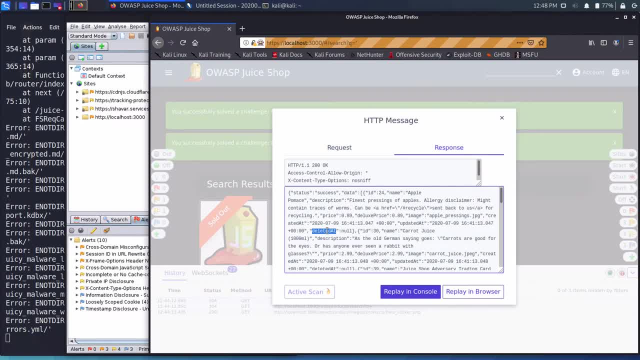 Also, we looked at all those different parameters being returned back And if we count them it comes out to nine. So that might tell us that there are nine different columns in this products table, which will be very helpful information once we perform unit attacks. 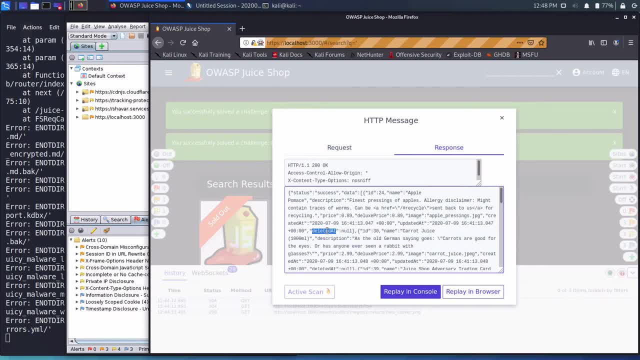 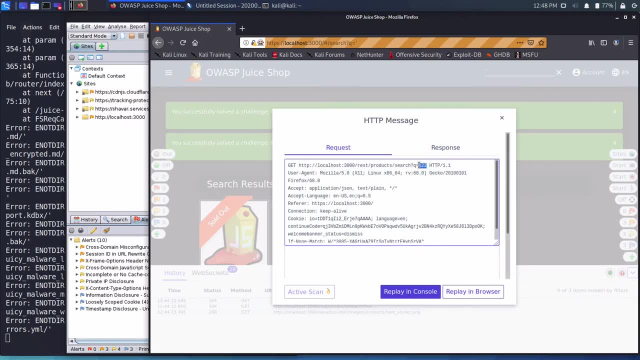 But so far we don't have any indication that this application is vulnerable to SQL injections. So let's go ahead and step it up a little bit. Let's go back to request And instead of single and double quotes, we're going to try a Boolean attack. 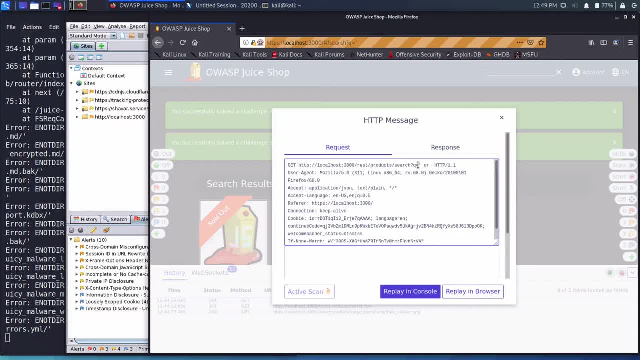 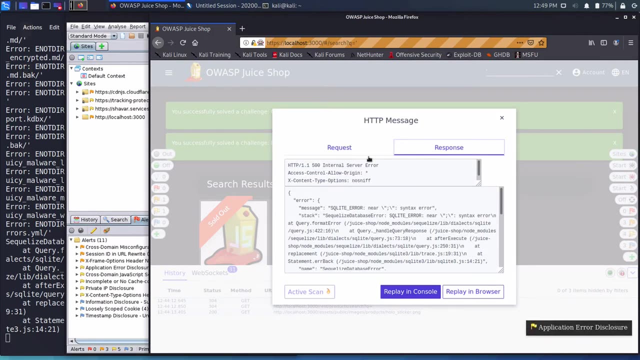 So we'll do single quote, space or space one equals one semicolon, and then the dash, dash to comment out the rest of the SQL query And let's go ahead and replay that in the console. If we look at the response this time now we're getting somewhere. First of all, 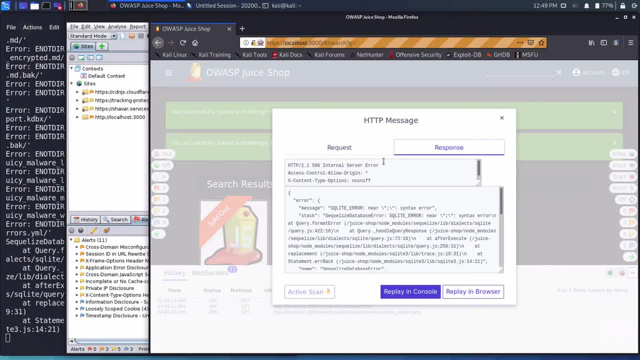 we get a HTTP 500 internal server error back, which is a very good sign if we're trying to attack the server. So let's go ahead and replay that and the console. If we look at the response this time now, we're getting somewhere. First of all, we get a HTTP 500 internal server error back. 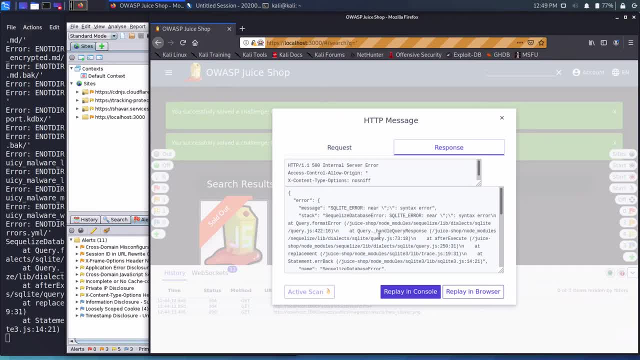 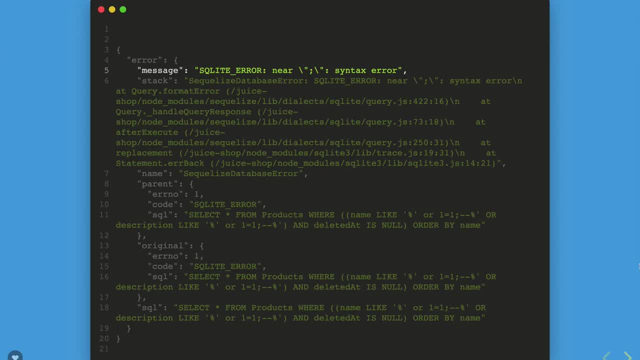 which is a very good sign if we're trying to attack this application. But second of all, we actually get the error message back. This error message is full of useful information. Immediately, we can see the SQLite error message which tells us that this database is running SQLite. We also see file paths which can help. 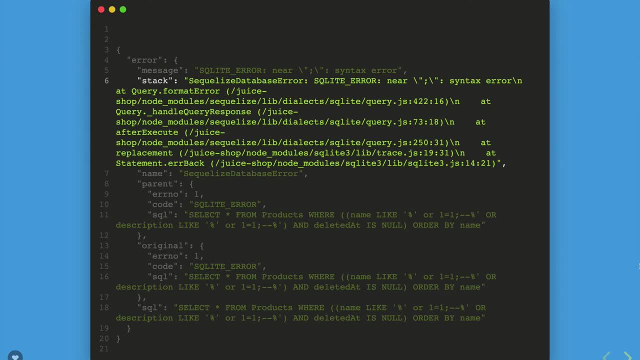 us for a number of reasons, such as helping us understand that the application is using node packages and what those packages are. We also get to see the exact SQL query, which is absolute gold and will help us construct better attacks. So here we have a select from the products table. So now we know that the products 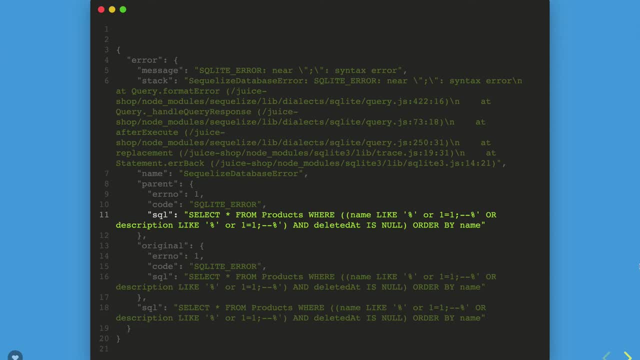 table is named products where the name is like our search input or where the description is like our search input and deleted at is null. So now we know for sure that deleted at is being used to hide products that are supposed to be deleted, but they're probably still in the database. 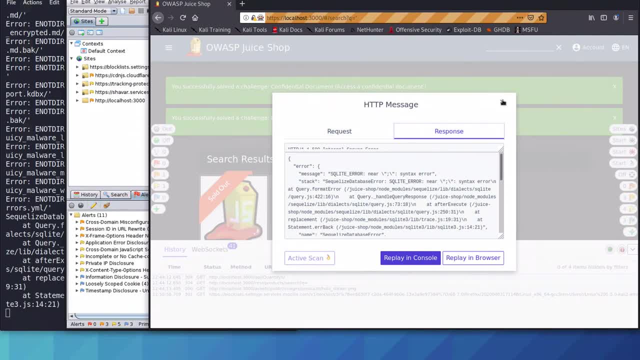 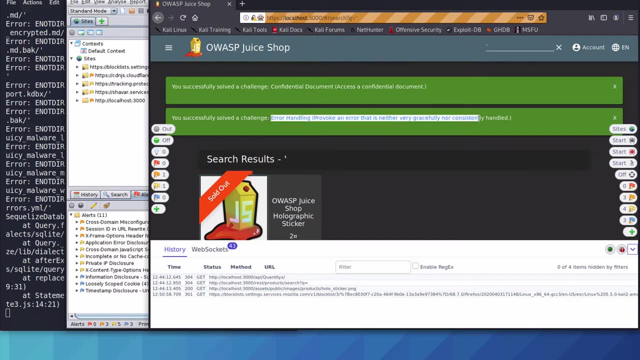 And, by the way, if we go back to the application, if this challenge had not already been triggered by our active scan, we would have now successfully solved the error handling challenge, which hopefully this has convinced you that proper error handling is extremely important because it can reveal way too much information. So now that we have an idea of how many columns 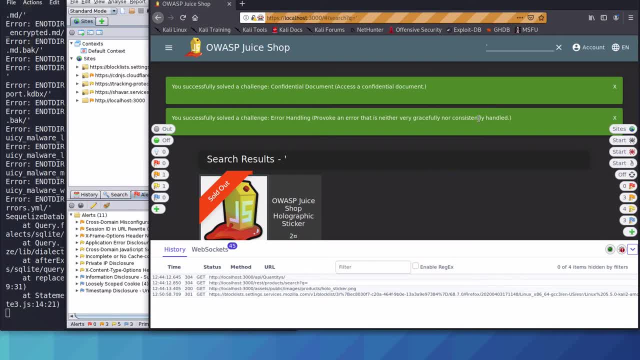 there are and what the query looks like. maybe we can use a union attack to try and extract information about how many tables are in the database and what those table names are. So let's go ahead and give it a shot. So again, we know that the application is running this SQL query. 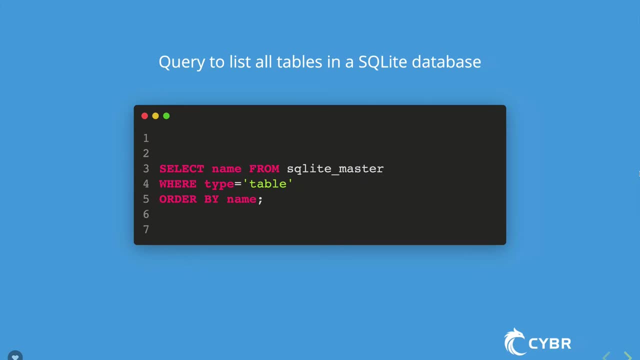 and here's what we would like for the query to look like. And since we know from prior lessons how to access table names from SQLite, we can formulate our SQL injection to look something like this: So this would be our payload, Again, since we believe there are nine columns to match from: 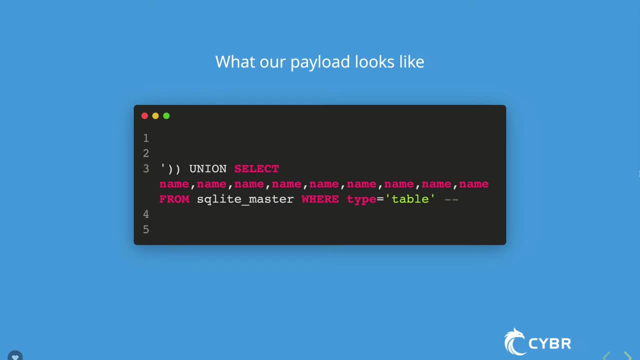 our products table. we can try to use the name for all nine of those columns and we would finish it with the dash dash in order to comment out the rest of the query And, as a result, this is the query that the application should execute. 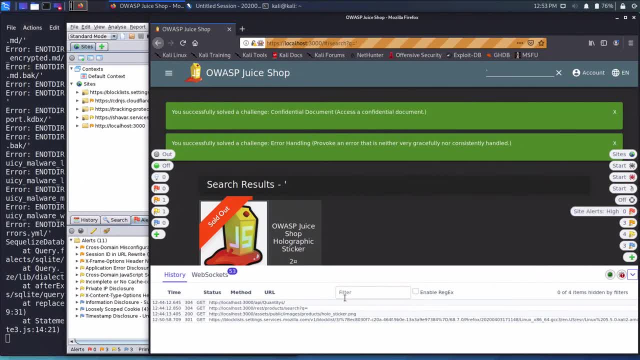 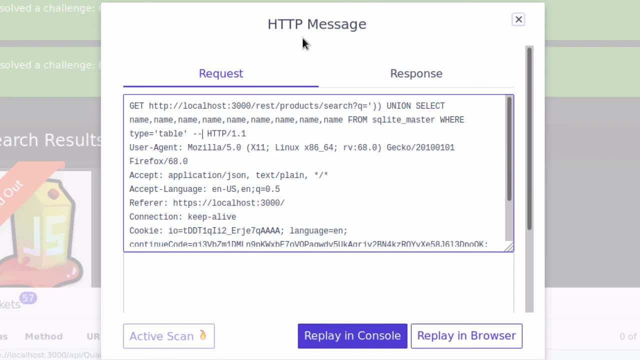 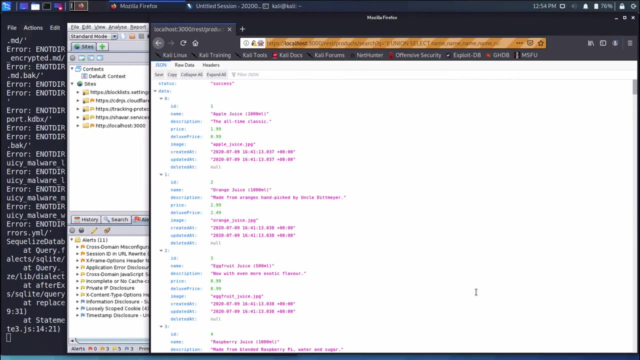 So if we go back to the application and we open back up the search request, we can input our SQL injection payload And now we can replay. but let's go ahead and replay in the browser And as we do that, we see the JSON output from a successful query. 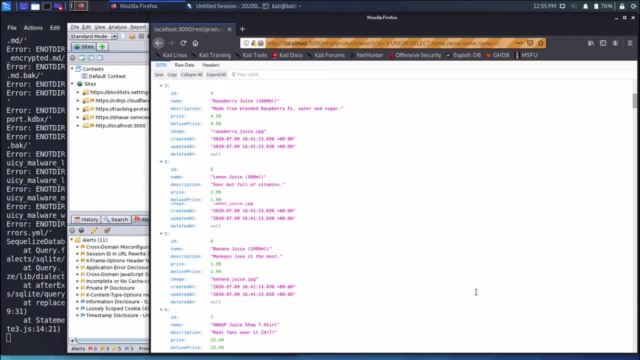 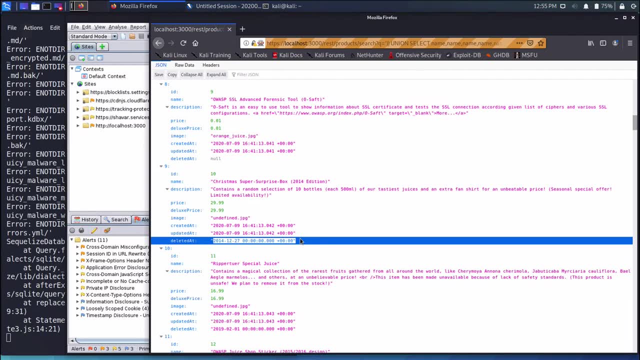 which is a very good sign, And we can see all of the products printed out, which, by the way, we can see some of the products that are supposed to be deleted because they have a date and timestamp. So we're not supposed to be seeing this Christmas super surprise box. 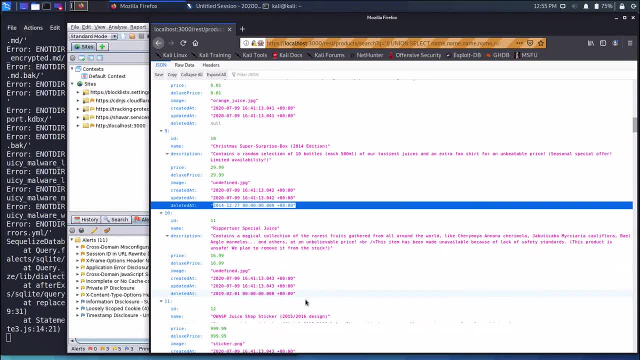 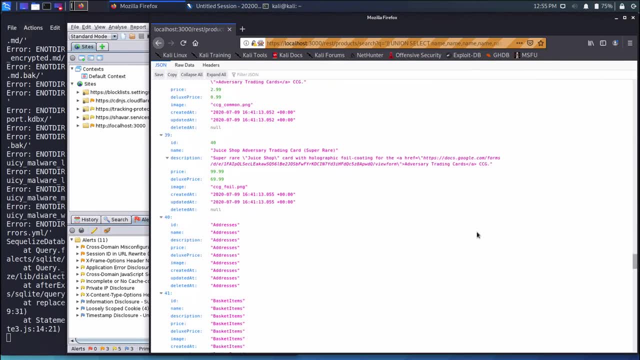 2014 edition or some of the other products that have been deleted. But if we keep scrolling down all the way to the bottom, we should also see our union attack results. And here they are. We've got an addresses table. We've got a basket items table. 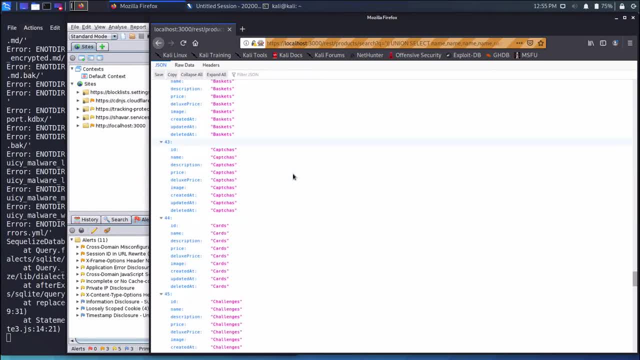 baskets, captchas cards, challenges, complaints, deliveries, feedbacks, image captchas, memories, privacy requests, products, purchase quantities, quantities, recycles, security answers, security questions, users, wallets And finally we have SQLite sequence, which is just a default SQLite table And ta-da. 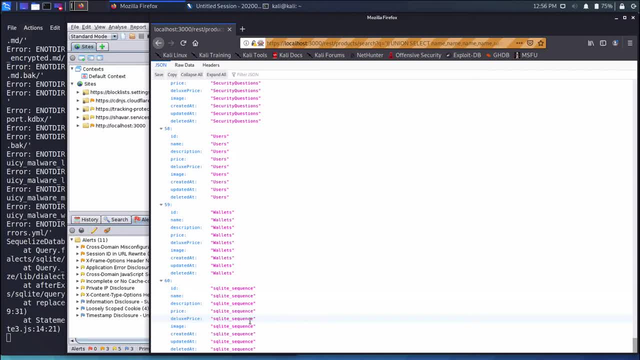 we now know every table name in this database using a fairly basic union injection attack And we can also use this table name in the SQLite table. And we can also use this table name in the SQLite table. And we can also use this table name in the SQLite table And we can also use this. 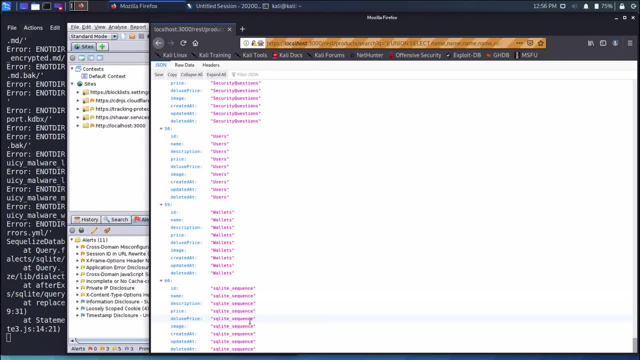 same type of attack to get the SQLite version that's being run by this database, which can help us find vulnerabilities for that specific version, especially if it's not updated to the latest version, And that can also help us formulate more advanced attacks in the future. So let's go back. 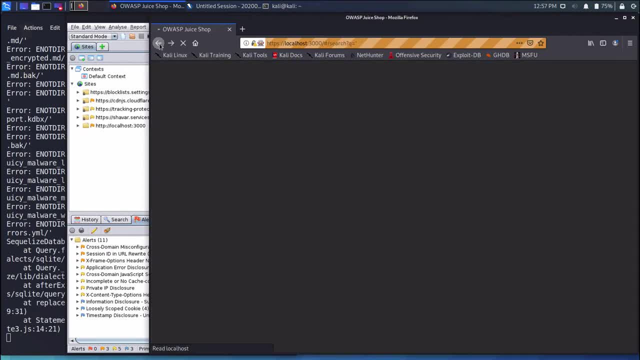 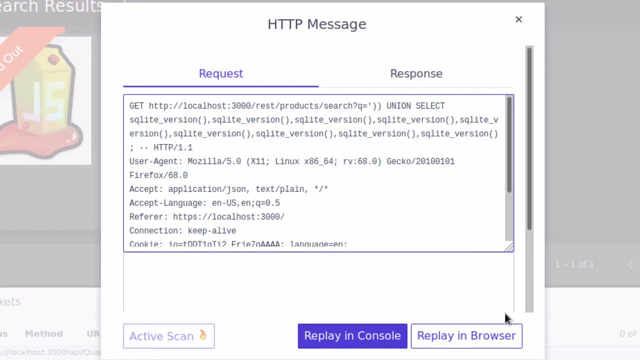 and let's change the attack. We'll click on this request again and we'll formulate our payload. It will look very similar, Except this time, instead of using the name column and pulling from that SQLite master table, we're going to use an SQLite function that returns its database version. 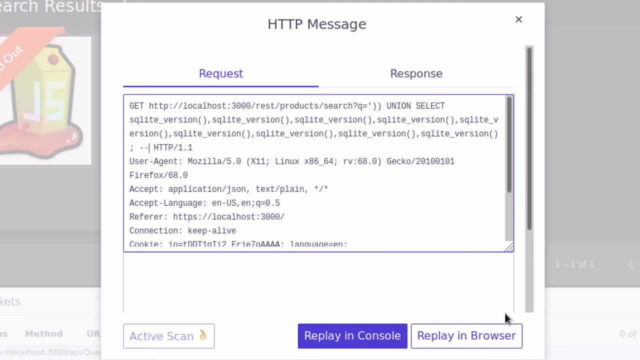 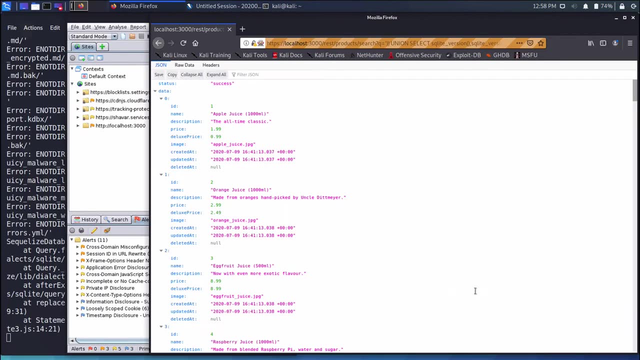 But we again have to use it nine times in order to match the number of columns in the products table. So now let's go ahead and replay this in the browser once more, And if I scroll all the way at the bottom, I can see that this database version is running. 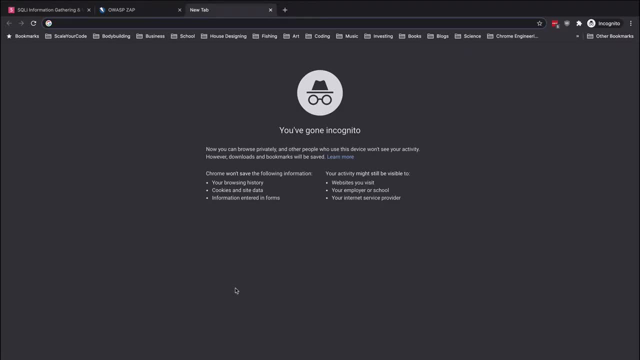 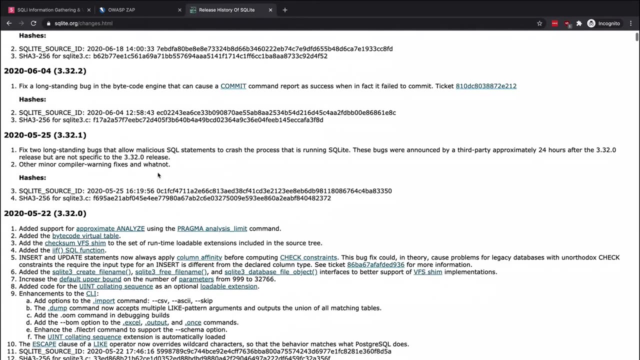 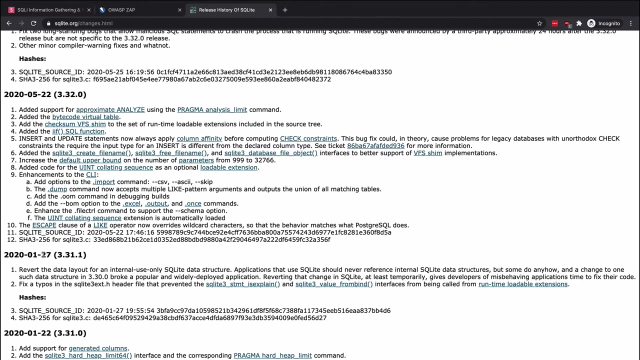 3.31.1.. And let's do a quick Google search to see if this is the latest SQLite version. And because we have 3.31.1,, we can see that, even though it's a fairly recent version, it was from January 27th of this year, which means that there have been newer versions of SQLite. 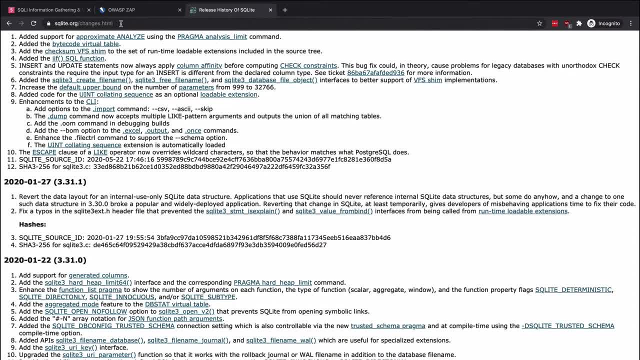 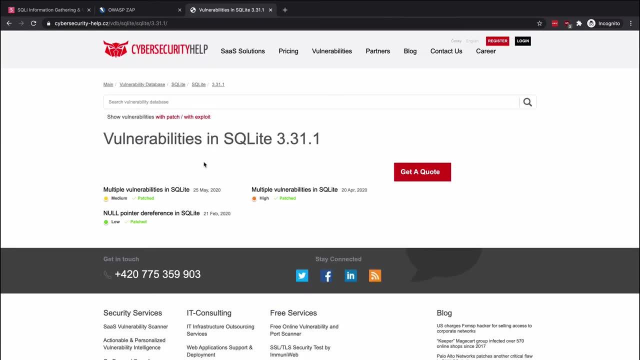 and we do not have the latest version. I can also search for specific vulnerabilities for this exact version or prior versions, So I could do SQLite vulnerabilities for 3.31.1.. And if I click on this first link here, it looks like this search engine has different. 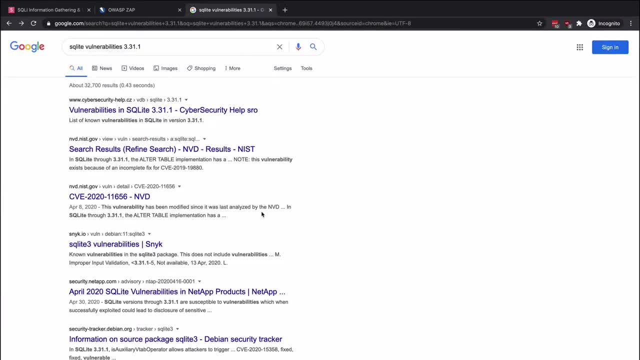 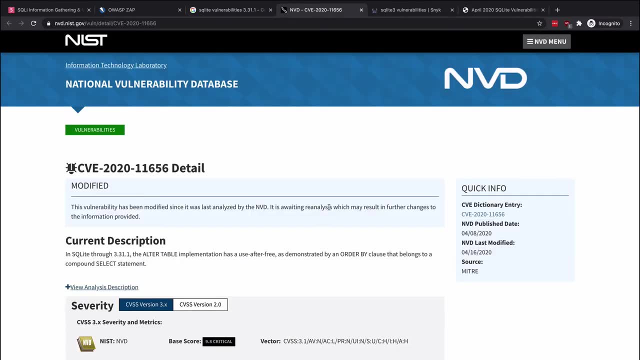 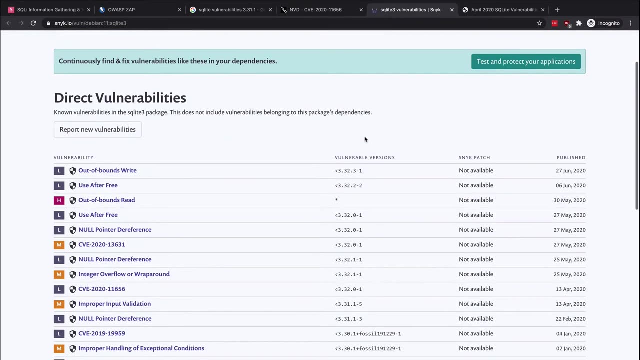 vulnerabilities that might be interesting to explore. Let's take a look at a couple more. I'll pull up the one from NIST, one from Snyk and I'll pull up one from NetApp. It looks like they do have a vulnerability, with a description of what it looks like. Same thing here. 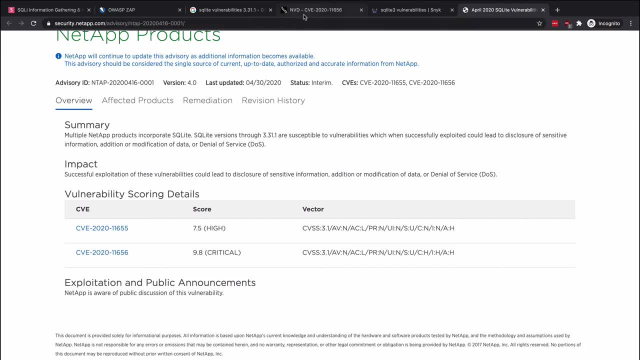 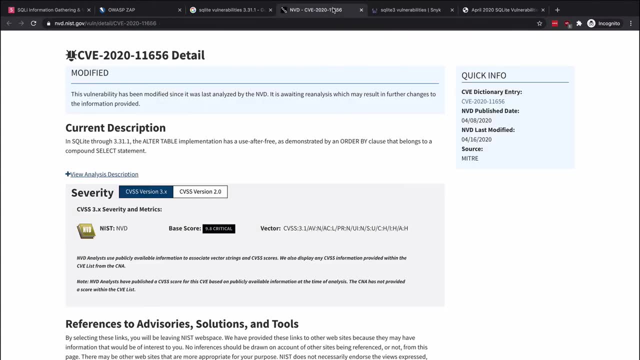 And NetApp is just listing the CVEs which we have one of them pulled up, the 2020 11656, which is this critical, with a 9.8 score. So that might be interesting to look into, But for the sake of time I won't be exploring these. I do recommend, though, if you're interested. 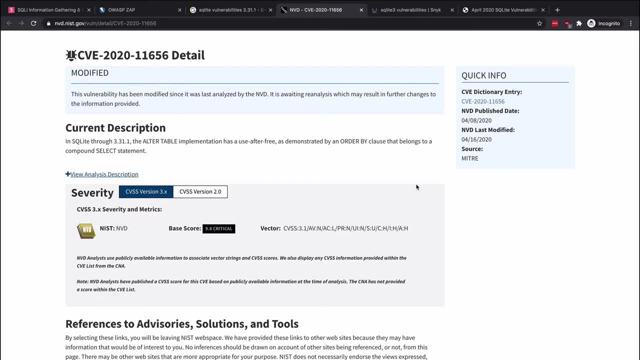 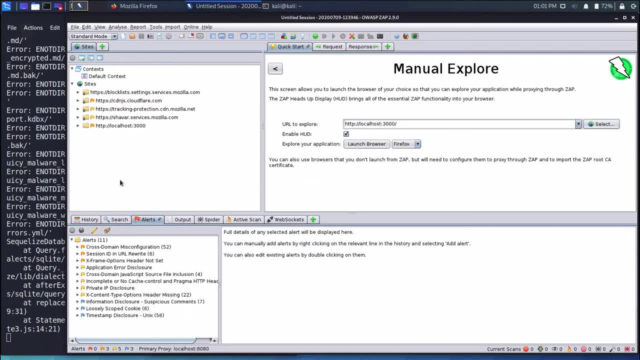 definitely recommend them and explore them further and try to see if you can exploit them through this application. But let's pause here for the manual inspection and let's pull up Zap, which should be done with the scan, And if not, I'll go ahead and fast forward. 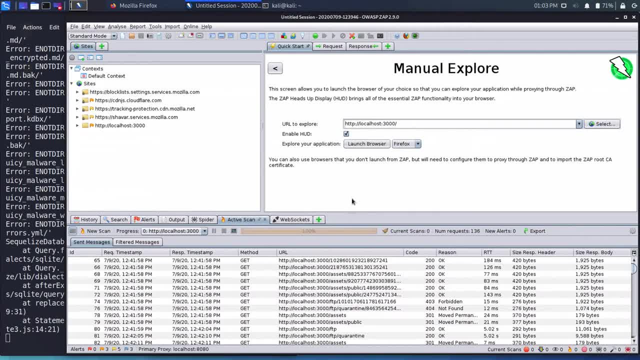 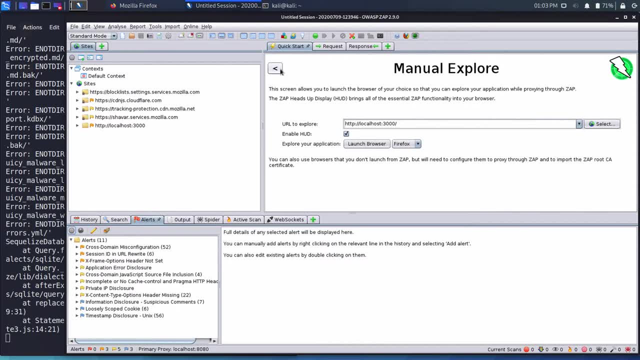 And it looks like the scan may have stopped before it was actually completed, because it should have found more things, such as an SQL injection possibility. So it's probably because of what I was doing. Let me go back and try it again and I'll just fast forward to the results. 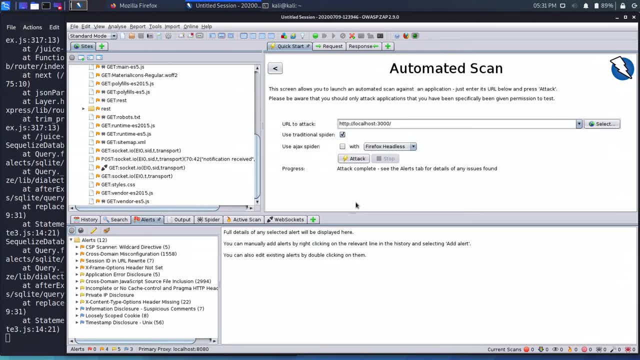 At this point, I actually decided to run a different scan on the application, using the Ajax spider instead of the traditional spider, because it typically works better with modern applications, but it does take a significantly longer time to complete. However, when I did that and the scan completed, here's what I had. 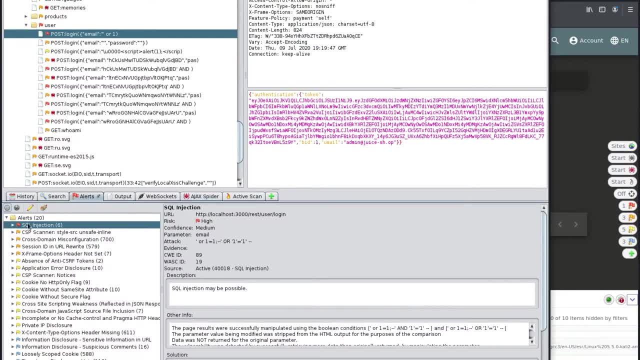 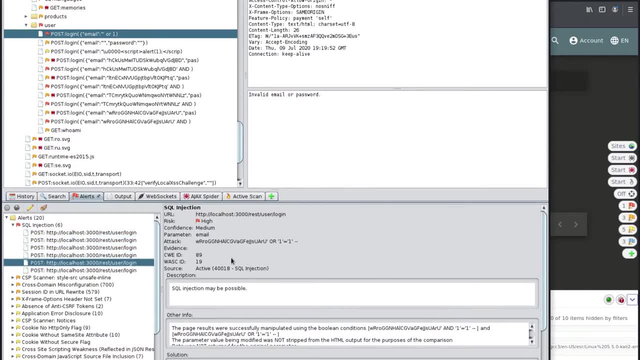 In the alerts tab we can see multiple potential SQL injections and they are all at the REST user login endpoint, but with different attack payloads that we can examine. For example, the last one is a single quote, or 1 equals 1 and dash dash. 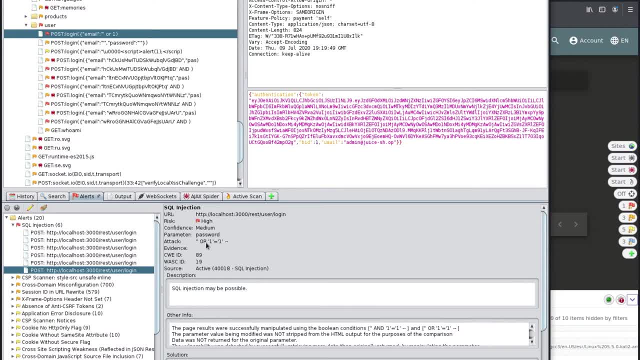 Which is good to know, because we haven't tried attacking the login form yet. but OWASP Zap Fuzzing found a successful SQL injection, which we can see from the results above. We'll try this attack in the next video lesson, since this completes our information gap. 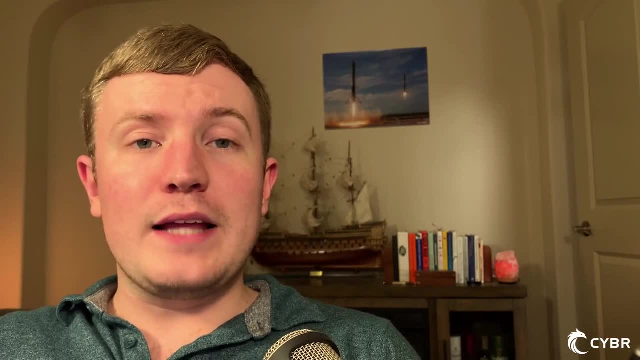 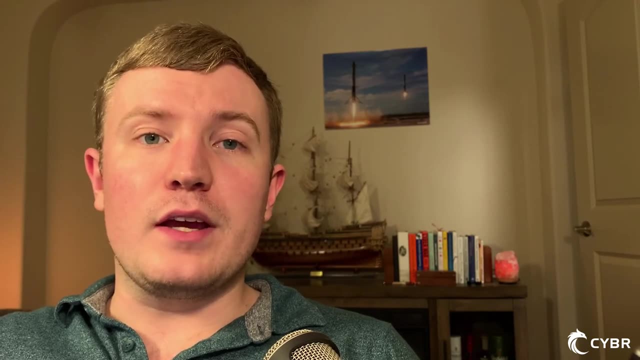 And, by the way, the reason that we don't just rely on automated tools like OWASP Zap to find vulnerabilities is because, even though it can be great at finding some of the low hanging fruit, it won't find everything, and a great example of that is that OWASP Zap did not. 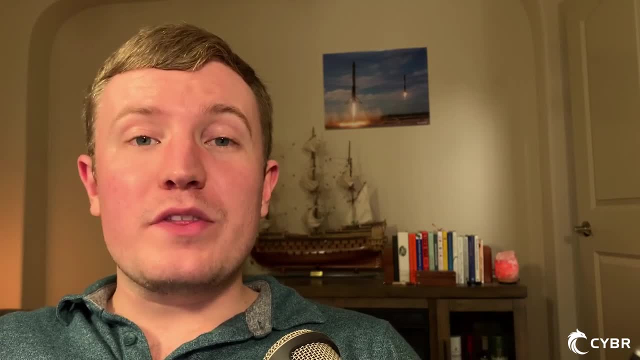 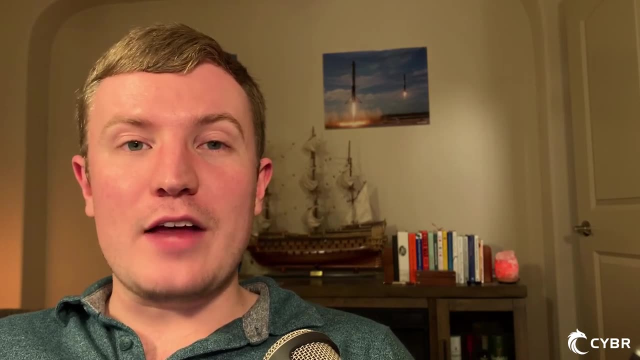 find the vulnerable search API Now. at this point, we have more than enough to step up our attacks, so go ahead and complete this lesson and I'll see you in the next one. In the prior lesson, we performed information gathering, which proved critical to providing. 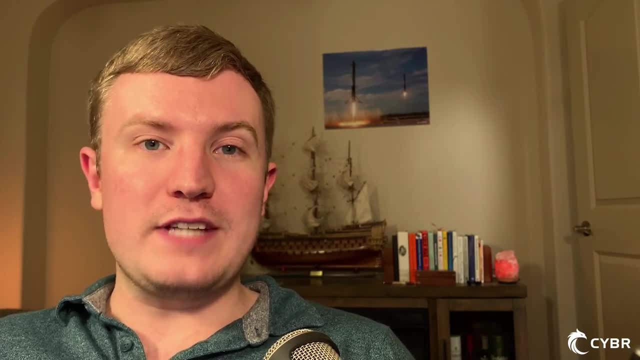 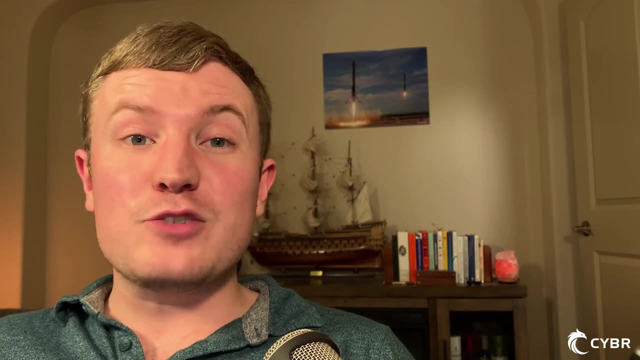 very helpful information that we can now use for more fruitful attacks, And we'll do just that in this lesson. We'll do things like compromising administrative accounts, extracting usernames, passwords and emails from the database, and more. So let's pick up where we left off. OWASP, Zap, scanning and fuzzing. 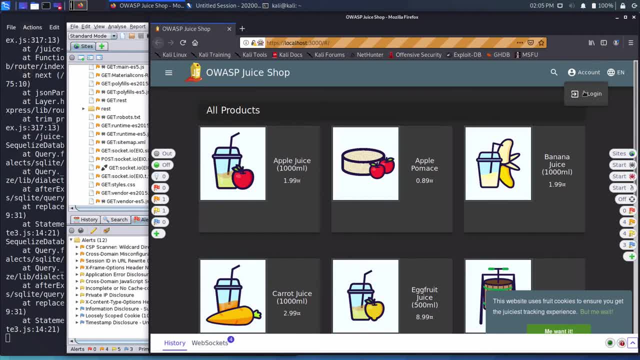 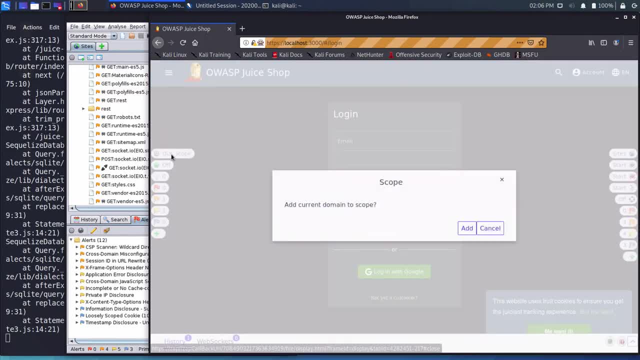 had detected a successful injection on the login endpoint, so we can start there. And before I try the attack, I'm going to turn on a few settings. First of all, I want to make sure that this is in scope, So I'll go ahead and click on add if it's not already. showing the red target within, So I'm going to go ahead and click on add if it's not already showing the red target within. And before I try the attack, I'm going to turn on a few settings. First of all, I want to make sure that this is in scope, So I'll go ahead and click on add if it's not already showing the red target within. 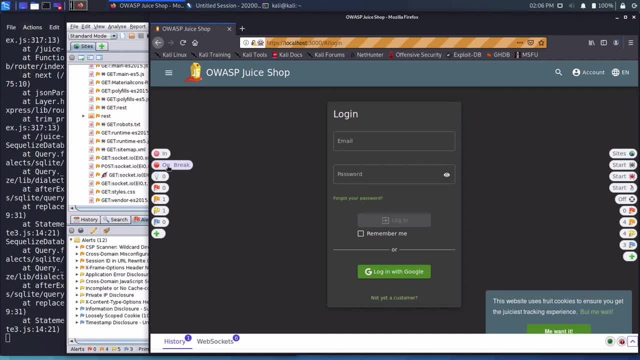 And before I try the attack, I want to make sure that this is in scope, So I'll go ahead and click on add if it's not already showing the red target within Next. I want to turn on breakpoints Because we want to intercept the request and the response. 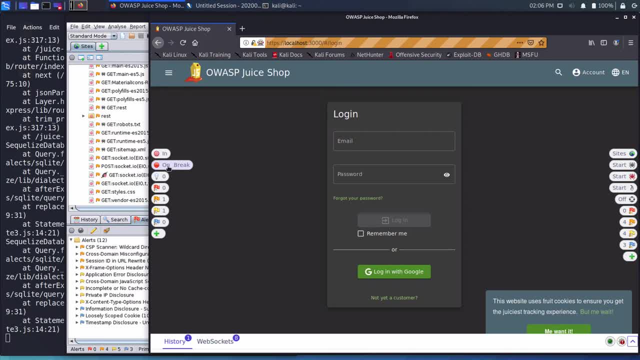 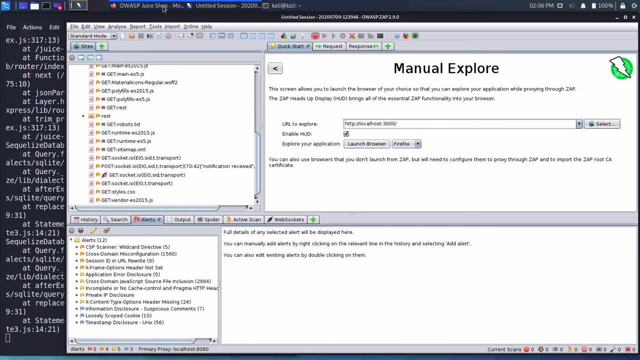 through the Zap desktop client instead of through the HUD this time, And I can verify and make sure that it is turned on by clicking on this green button turning it red. So now that we've got the breakpoints turned on, let's go ahead and perform our attack. If you remember, it was a 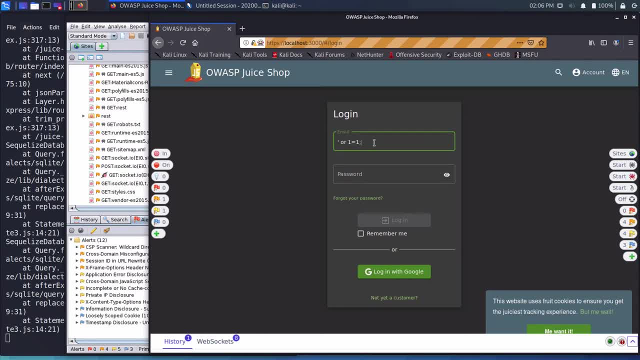 single quote, or one equals one, We'll also add a semicolon and then we'll add dash, dash in order to comment out the rest. For the password, frankly, you can put whatever you want. So I'm just typing in gibberish And we'll click on login. So now, if we pull up the desktop client, 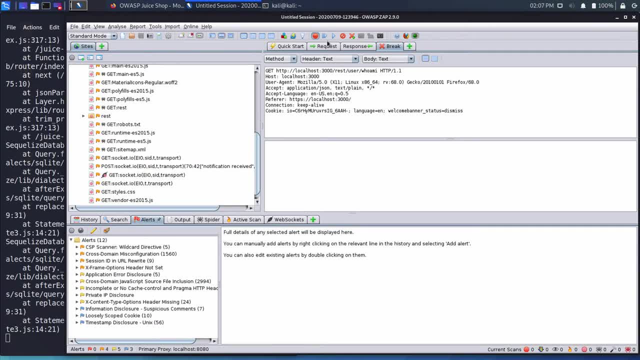 we'll see the requests and the responses And we can step through each one. So we see a 200.. Okay, we'll keep going. And now we'll see the post request for this endpoint rest user login with this information that we inputted. Let's go ahead and step through. We see a challenge. 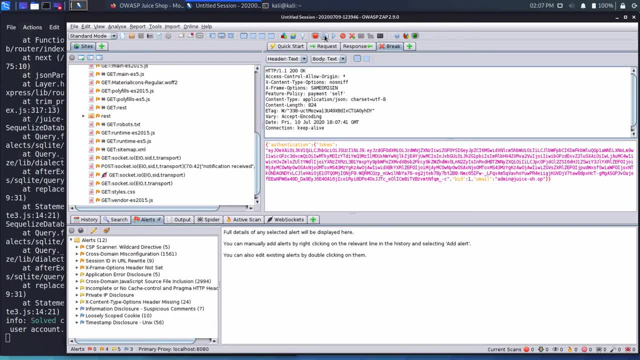 solved, which is a very good sign, And then, if we step through one more time, we'll see the response from the API. Here we have a JSON response which has authentication with a token with a BID and a user email. The BID is one and the you email is admin. at juice dash sh period op. 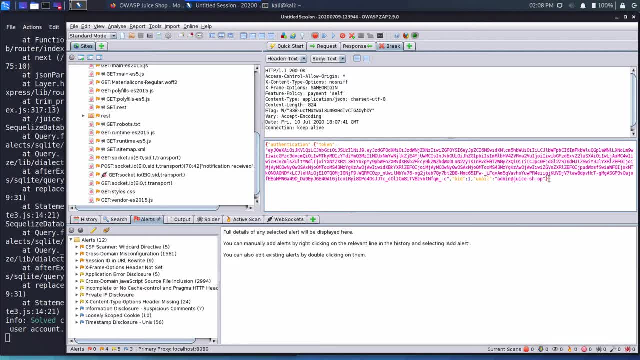 so juice shop. So what I think our attack was able to do is probably just completely ignore the password requirement And instead let's go ahead and run our attack and see what happens. So let's log us in as the first user in the database which has an ID of one, and that happens to be. 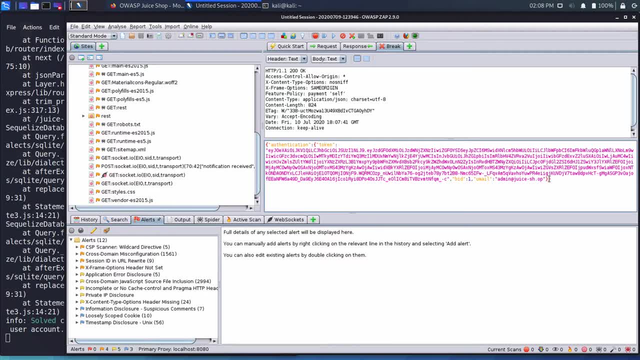 an admin, And while I don't want to deviate too much from SQL injections in this lesson, this token is quite interesting, So let's see if there's anything that we can exploit there. I'll go ahead and copy this entire token And then I'll pull up a regular Firefox window. 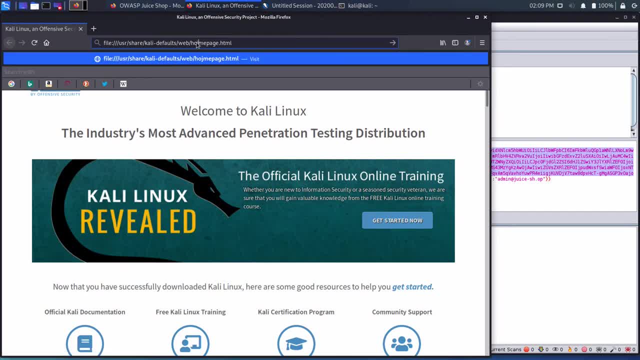 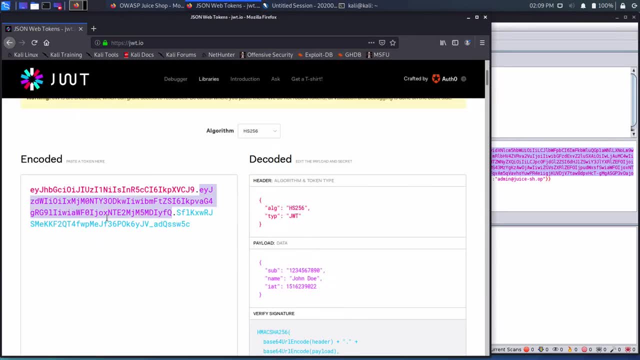 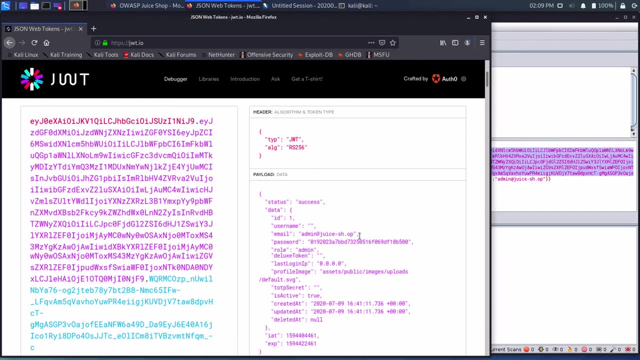 just to keep it separate from this, And I'll search for JSON token. The first website is what I was looking for And if you scroll down just a little bit, we can paste this token in order to decode it, And then we'll see the payload data on the right hand side, which contains the 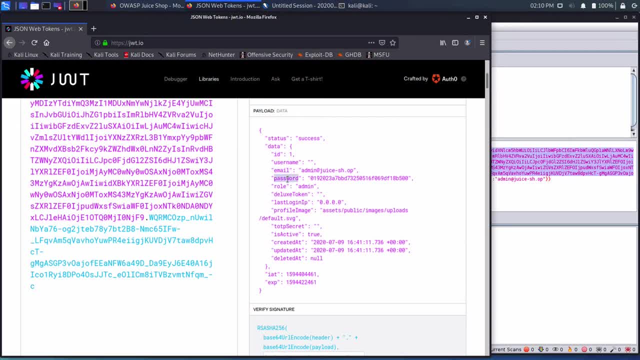 username, email ID, password, role and more information. So this password definitely looks like some kind of hash. Hopefully it's an empty five hash, because maybe that means we can crack it. So let's go ahead and copy this And then we can use a tool integrated in Kali Linux called 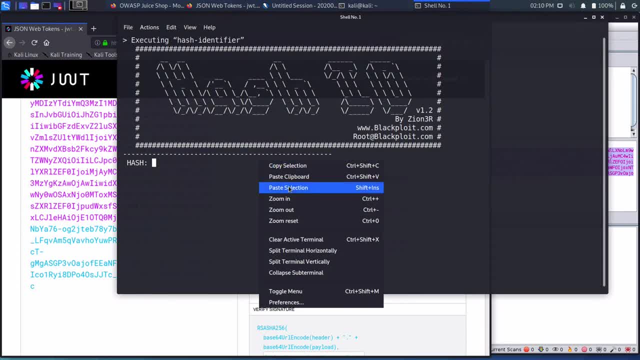 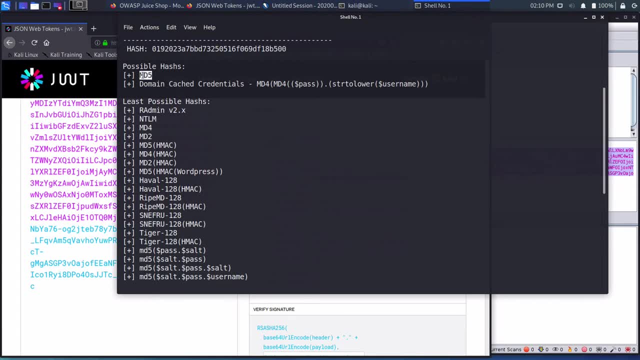 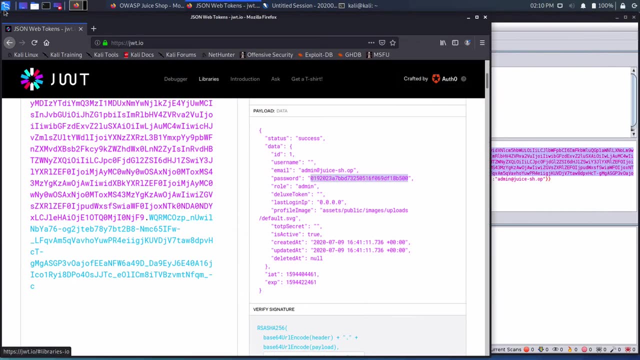 hash identifier And I'll paste the value in here. Press Enter. If we scroll up just a little bit, we'll see that the possible hashes are indeed MD five, So that's a really good sign. Now let's go ahead and use hash cat in order to try and crack this MD five hash, If you haven't used hash cat. 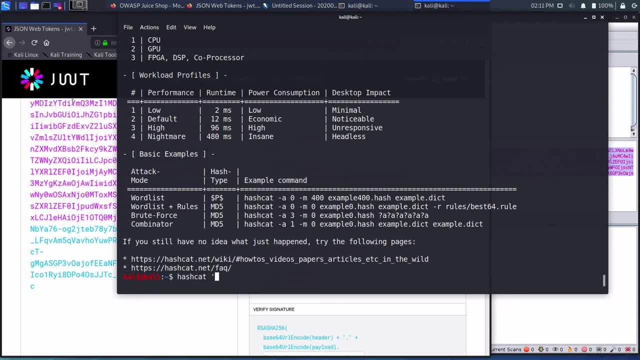 before. it's pretty straightforward. We'll type hash cat, then we'll put a single quote: enter our MD five, hash. make sure to close that single quote. And then we'll use a password list Now instead of pulling a custom password list. 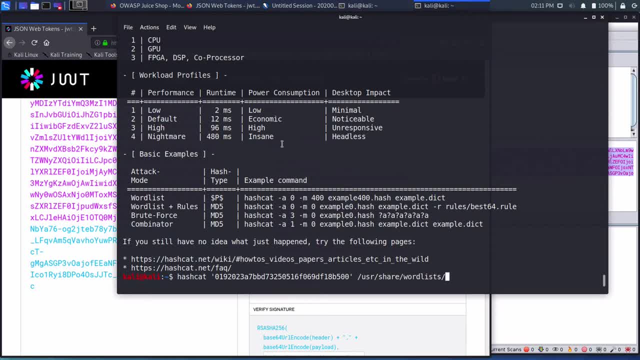 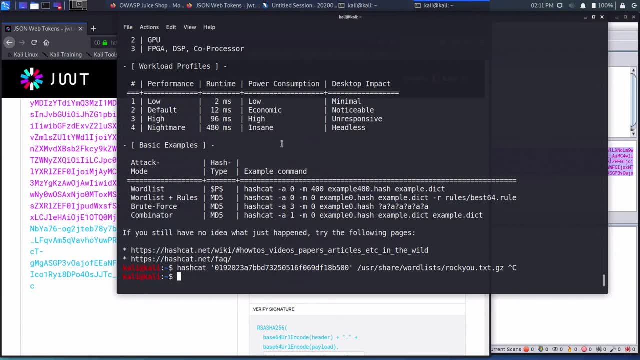 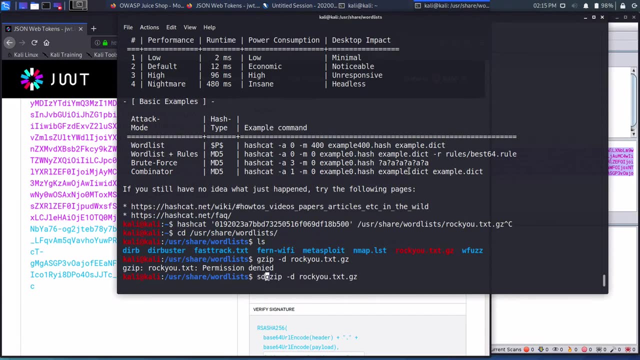 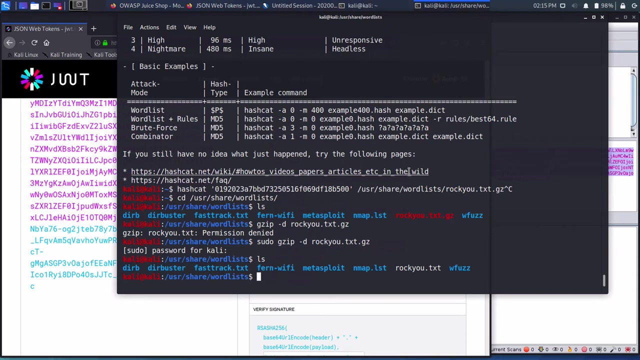 I'll just use the one that comes pre-installed in our version of Kali Linux, which is rockutxt, But first I'll have to extract it, which I forgot to do, So let me exit out of this. Okay, At this point we should have the text file, and we do fantastic. Now let's proceed with our 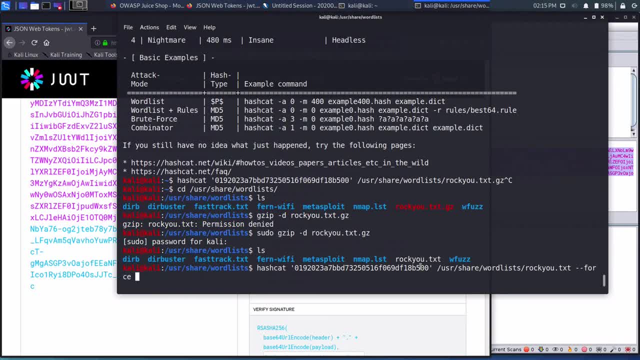 application, And then I'll use a command called force, because otherwise it will complain about not using the right drivers, which does drastically slow down the cracking operation. but it'll be sufficient for what we're doing here, And then I press enter. I let us do its thing for a few. 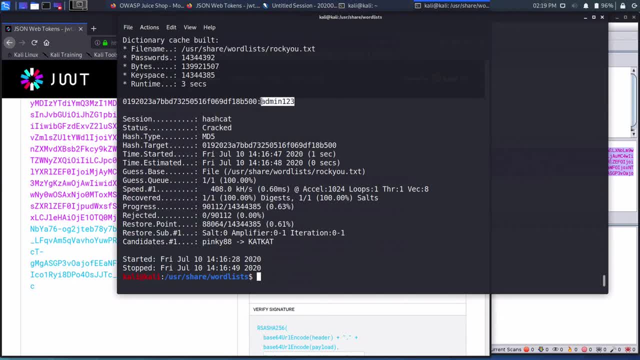 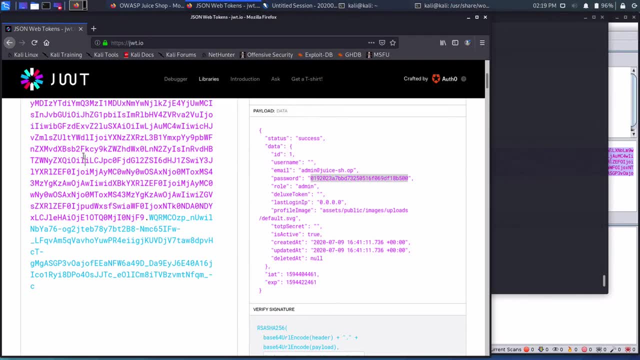 seconds, And literally within seconds, we get a password back which is admin one, two, three. So we've successfully cracked this hash from this JSON token that we received through the application. So let me go ahead and close this out and go back to the application. 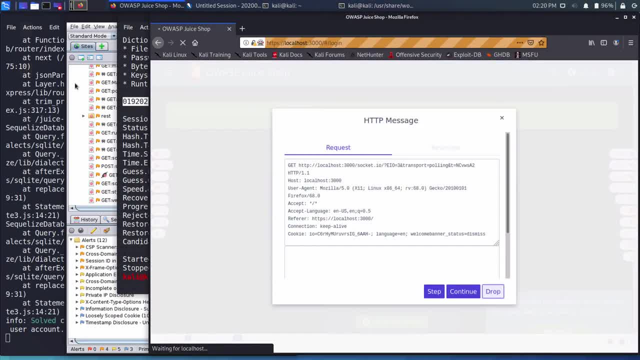 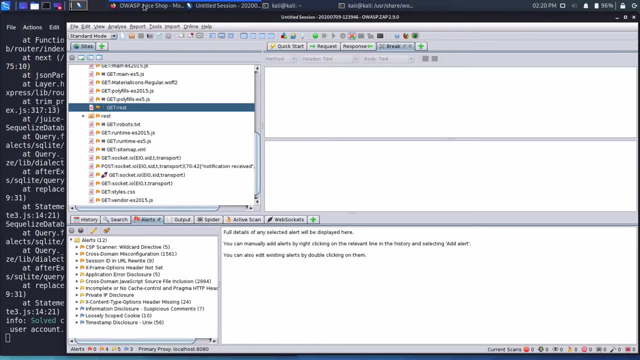 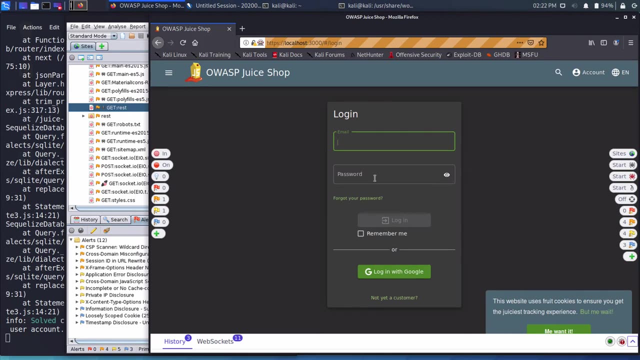 I'll close this window out, but I'll also need to end this breakpoint so that it stops hanging the requests. I'll step through all the way, And so now we can try to log in with the legitimate email and password. And, by the way, 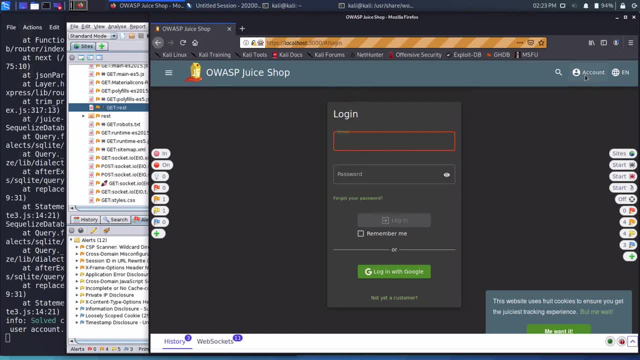 if you're logged in from the prior attack, you can log out by clicking here and you'll see log out Instead of log in. you'll come back to this page here- type admin at juice-shop And then the password will come back. 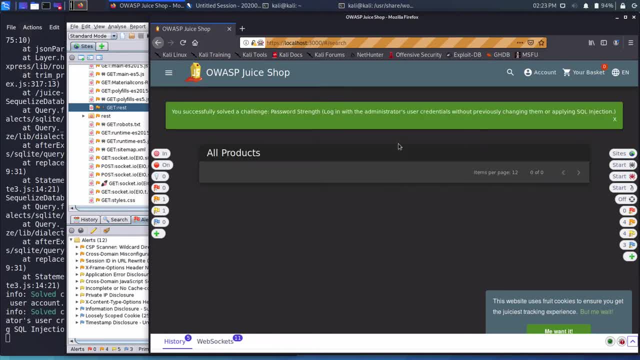 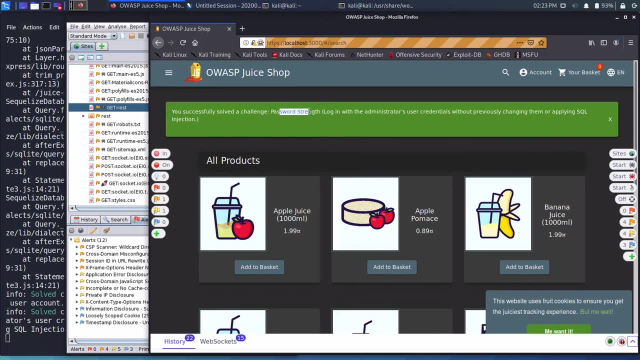 The password will be admin one, two, three, press enter And you've now successfully solved a challenge of password strength, because it was way too easy to crack that password And that also tells us that other accounts may be vulnerable. but how can we find those other accounts and potential MD5 hashes? 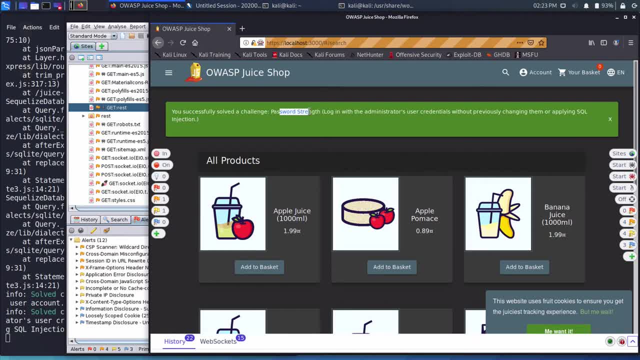 Well, we already know that there is a users table from a prior union attack that we performed, And I'm assuming that this is where they are storing emails and passwords, but I don't really know what the names of the columns are, And we could either assume that they are email and password. 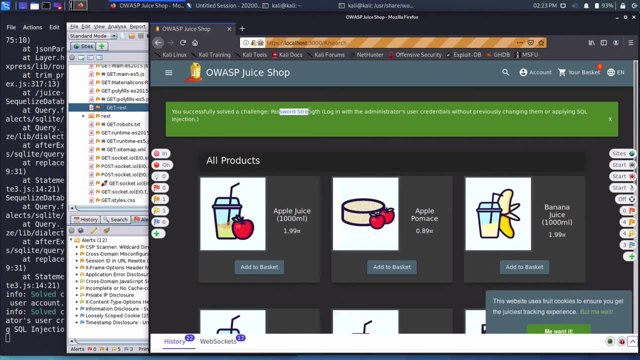 but to validate. there are a few ways that we could do it. And you know what? Let's try those different ways Instead of just doing it one way. let's try one first and then we'll do a second approach. So first let's log out and let's try to cause an error from the login form. 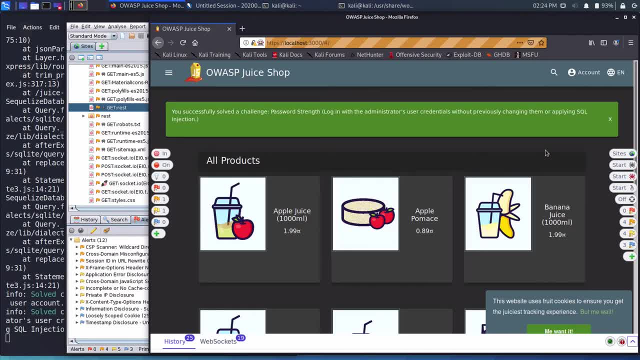 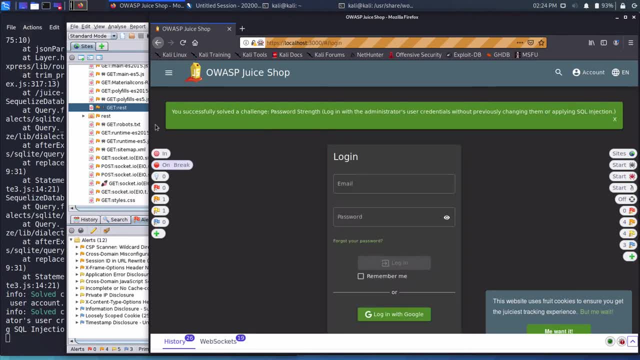 just like we did with the search form and API endpoint, because it showed us the SQL query, which was extremely helpful. So let's go back to the login page, Let's make sure our breakpoints are still on And let's just put a single quote with gibberish password. 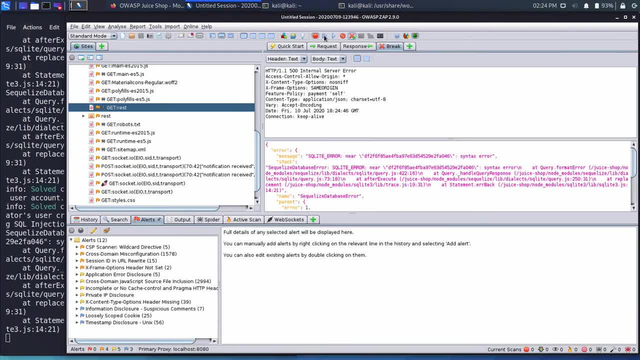 If we go through here and step through, we get the error that we were hoping for, which is fantastic. We can see the SQL query, which is select everything from users where email equals our input and password equals an MD5 of our input and deleted at is null. 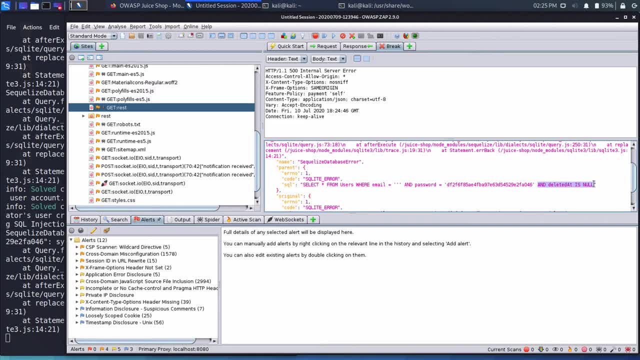 So now we know that there's an email column and a password column, as we suspected, And these are the columns that we will want to return values for. We also saw an ID being returned earlier in addition to the token, So we can assume that there is an ID column And since we already know that the search is, 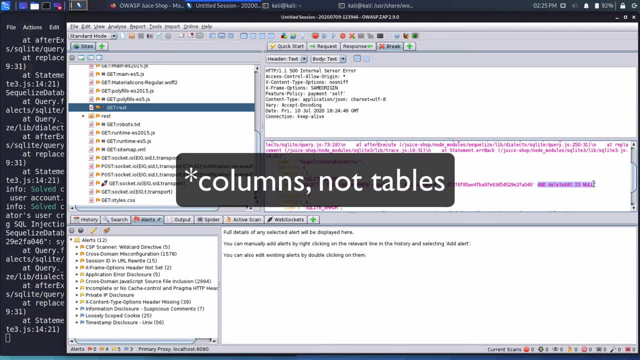 vulnerable and that the products table has nine tables, we can use another union attack again in order to return all emails and passwords stored in the database, or at least in theory. So go back to the search and submit another query, making sure that the breakpoints are on, and we will modify the request with our payload. 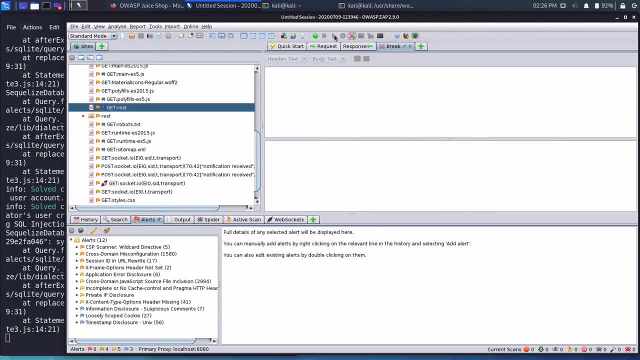 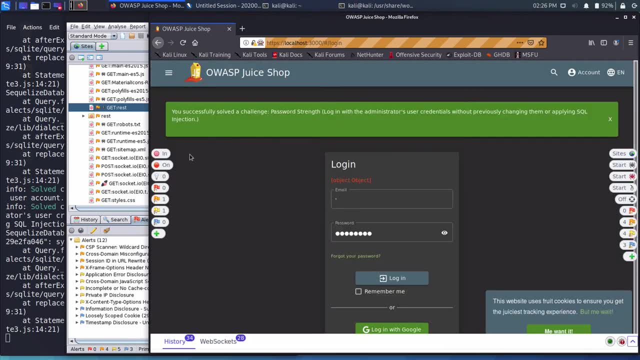 So for now I'll turn off breakpoints so that it doesn't mess with our navigation. Close these windows out And then make sure that the break option is off. Then I'll log in as the admin, just for the sake of it, And it's faster to do the SQL injection. 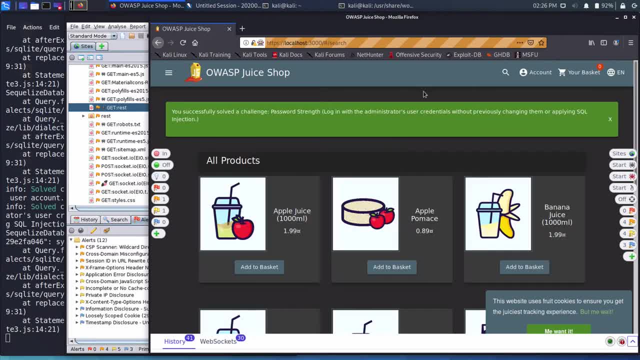 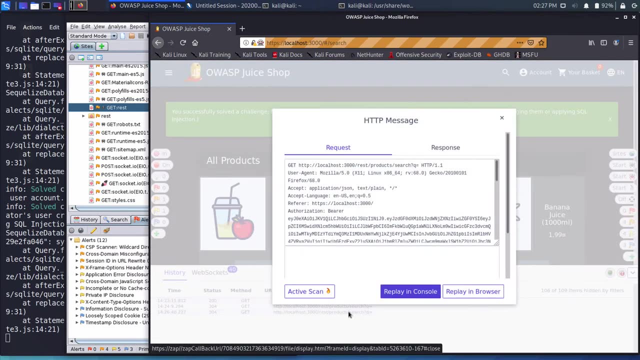 than the actual legitimate username and password. So I'll do that. Then I'll turn the breakpoints back on And I'll pull up our history so that we can find that search endpoint. I'll click on that, which, by the way, again, I can do this from the desktop client instead. 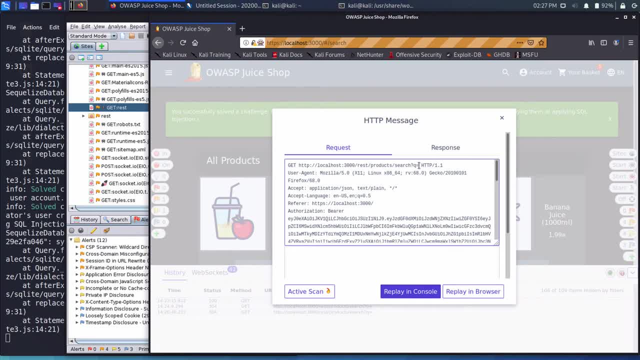 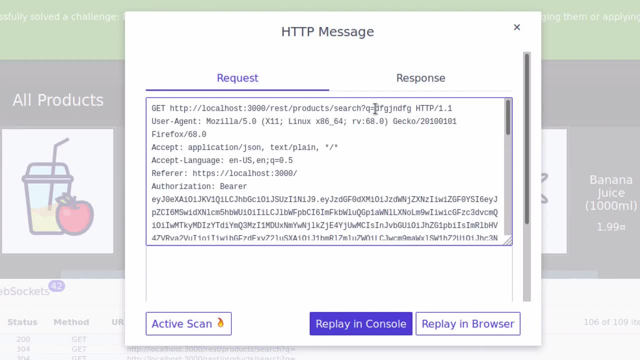 but the history makes it real easy to find through here, And this time I'm going to add just random characters because I don't want the search for the products to return anything, Because last time we had so many different products to sift through and we had to scroll. 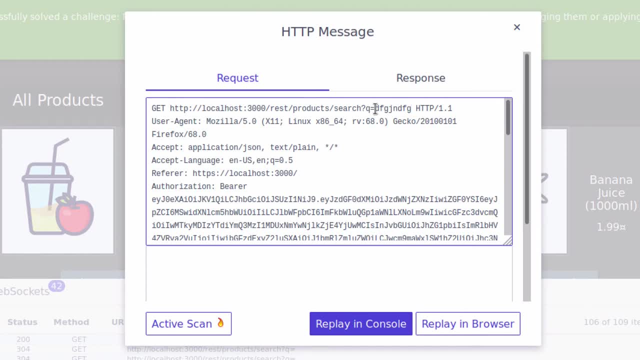 all the way at the bottom. But if I put random gibberish here, it won't return any products from the search query And instead it will just show us the results from our union attack. So I'll do that Single quote, two closing parentheses, and then we'll do the union attack. 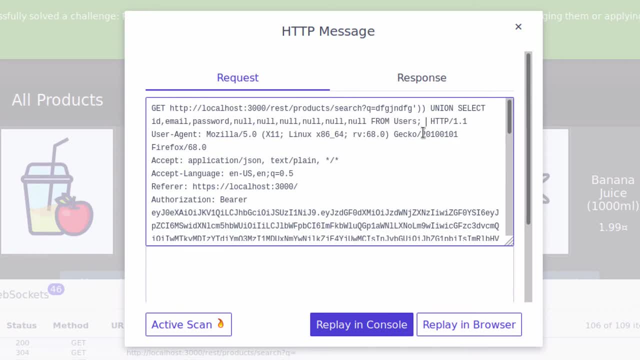 And then we'll do from users: table semicolon and then comment the rest out. So let's go ahead and replay in the browser. Not that it matters, because I've set the breakpoints anyway. so we can go back here and we'll see it through here. 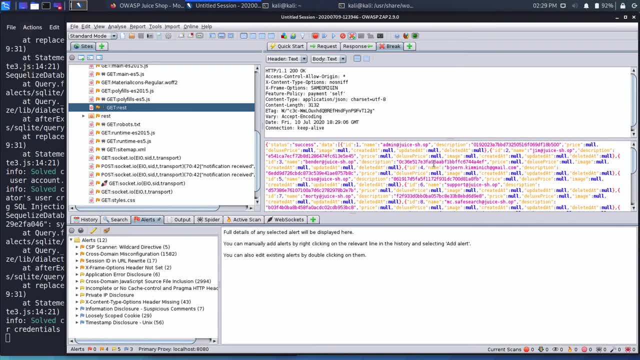 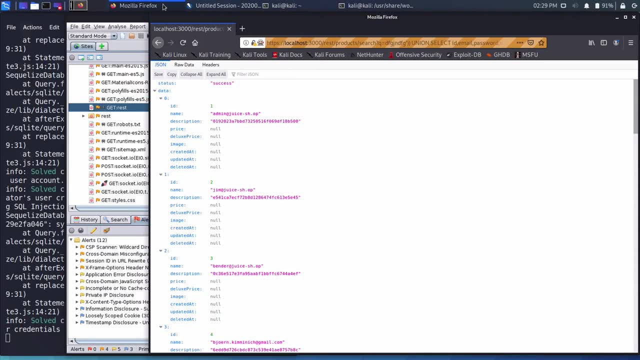 So we have the result here, if we wanted to, but I'll go ahead and continue it forward so that we can see it through the browser. It just did a little bit cleaner that way And, as a result of this attack, we get an output containing all of the users and their information. 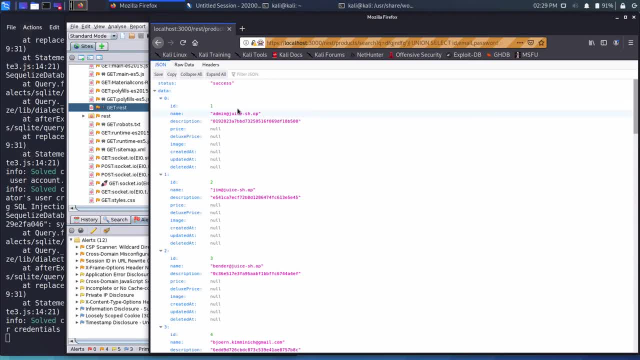 from the database. For example, we have idea of one with the admin email, the password. This is not really the description, Remember, it's mapping to those product columns. So this is the password hash, And then we have all of the other users contained in this database. 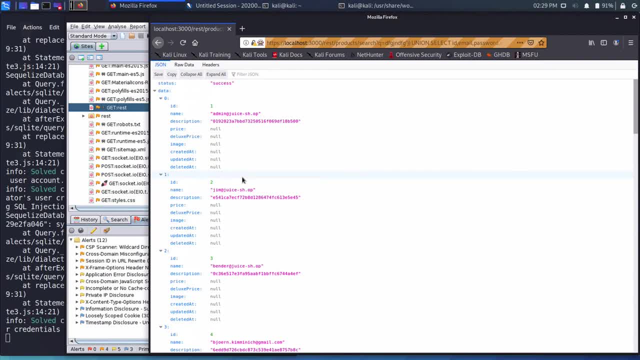 Sure, We've got a little bit more information about what we need to know first. So let's go back to our And, as a fun exercise, you could try to crack some of these passwords in order to access these different accounts, or get creative with other SQL injection attempts. 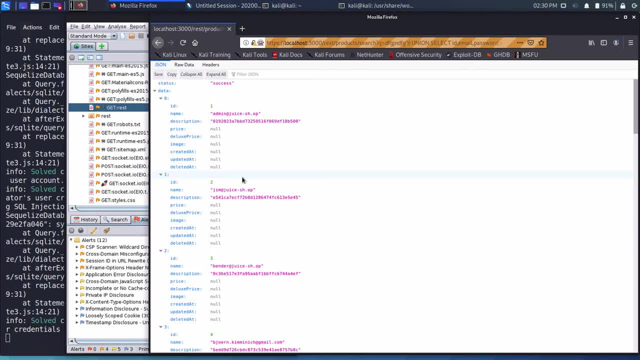 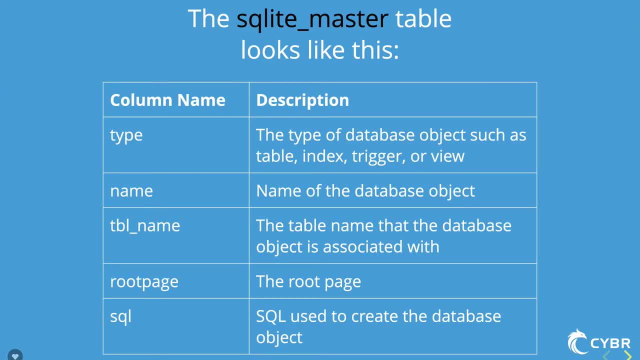 But instead of doing that, I'll try that different method that we talked about to achieve this same result, but with a completely different approach. Because, if you remember from a prior lesson, the SQLite master table contains not just the table names but also the SQL queries used to create those tables. And since SQL queries used to build, 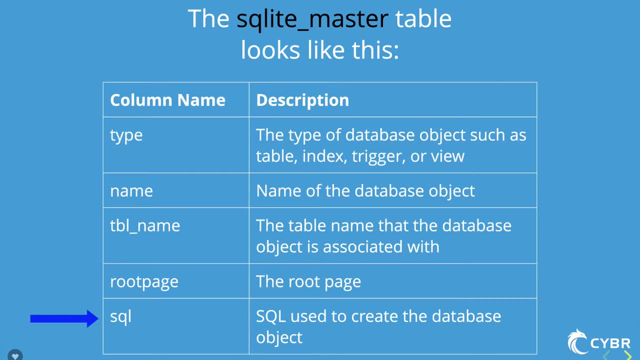 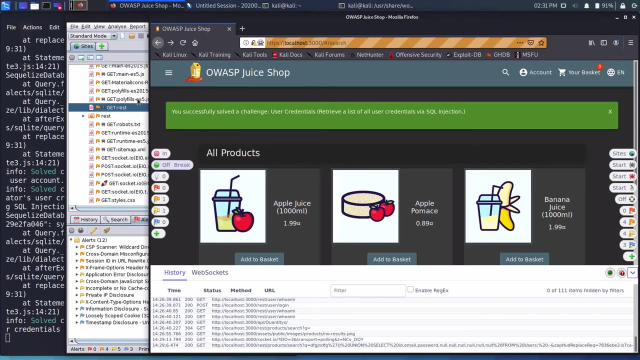 schema contain the columns and their types. that could be extremely helpful information, So let's try to extract that now. If I go back- and this time I'll turn breakpoints off, just so they could go a little bit faster- Make sure that's off as well. I'll pull up the history. 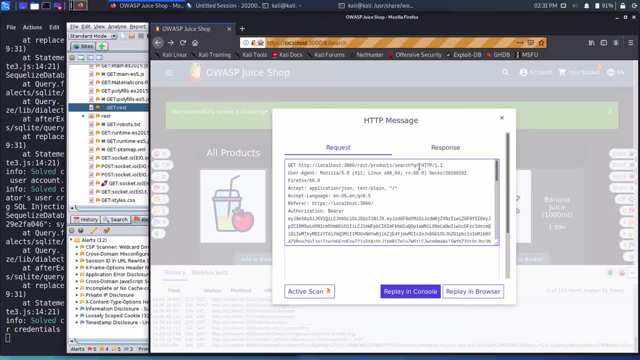 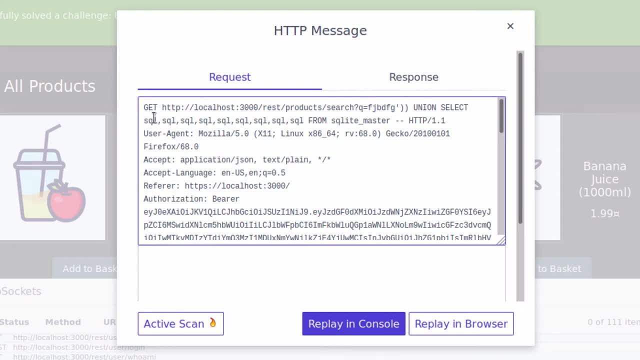 again pull up the search query and let's do another union attack, but this time pulling from the SQLite master table. So we're doing a union select SQL for nine columns from SQLite master. Let's go ahead and replay in the console. 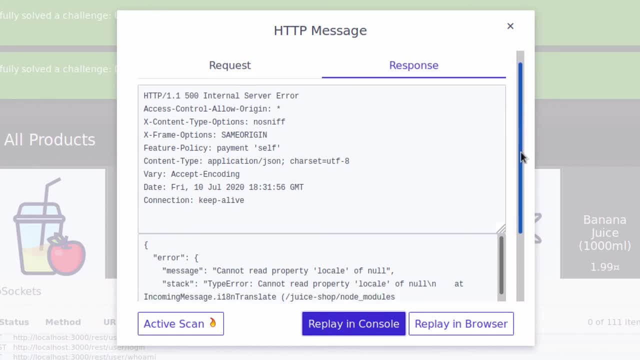 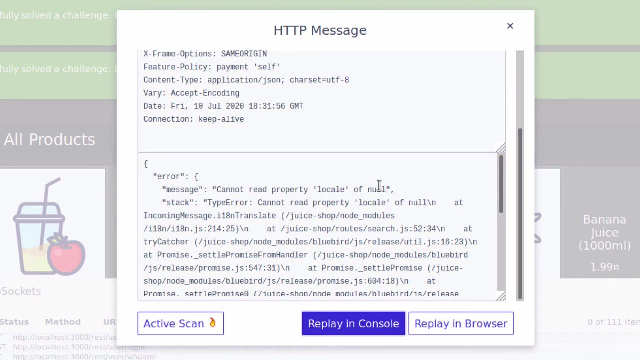 Except this time we get a 500 internal server error and we get an error message that says: cannot read property of null. So it didn't like us using SQL for each column, So let's try something a little bit different. Let's go back to the request And, instead of doing 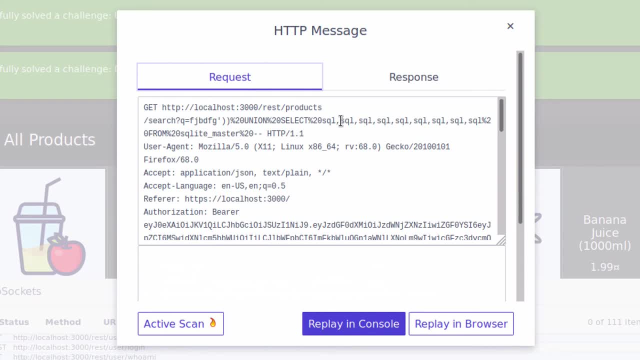 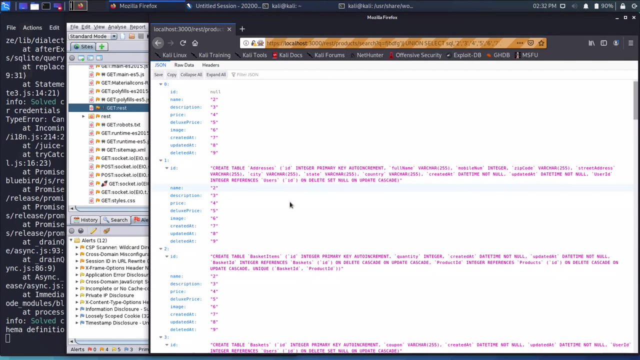 SQL for all of them. what I'll do is just SQL for the first one. I'll use numbered strings for the other eight columns. So we'll do two, three and hopefully this time it goes through. Okay, perfect, it does. So now we can see that for each of the tables. 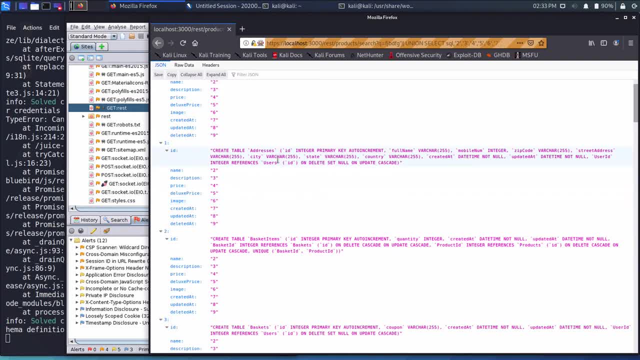 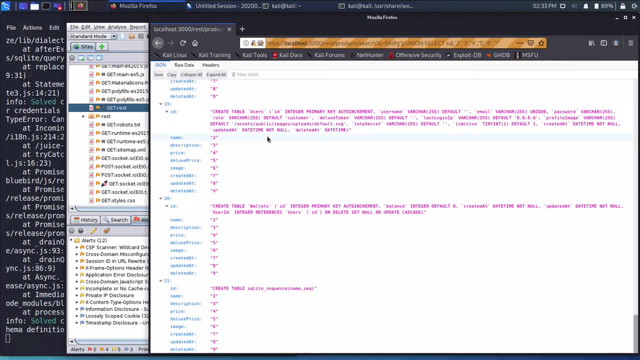 we have the SQL that was used to create that schema. In this case, we're looking for users specifically, So I'll scroll down until I see users, which is near the bottom, And I'll go ahead and copy and paste this in a better format so that we can look at it. All right, so we've 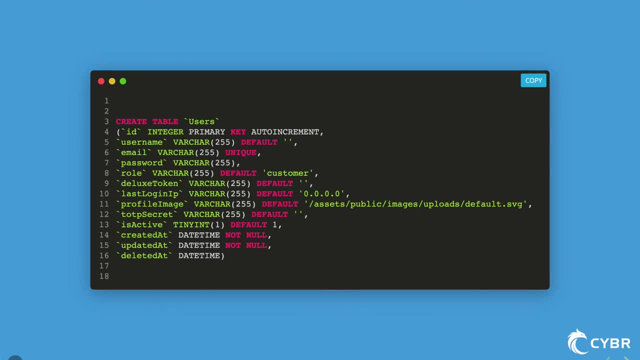 got the ID, username, email, password, role, deluxe token, last login IP profile image. COT P secret is active, created at, updated at and deleted at. Now I'm not entirely sure what the deluxe token is for at this point, but the TOTP secret probably stands for time-based one-time. 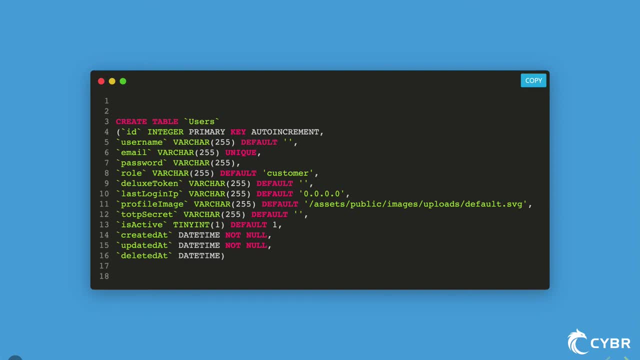 password, which might be something that we can work with, if we wanted to, for a different attack, But that's not really what we're doing right now. Let's go back instead and modify our prior attack to include some of these columns, And I'll do nulls for the last three, because I just don't. really care about: created at, registered at and deleted at, So let's go ahead and do that. Okay, so now we're going to go ahead and copy and paste this in a better format, And I'll go ahead and paste this in a better format. And I'll go ahead and paste this in a better format And I'll go ahead. 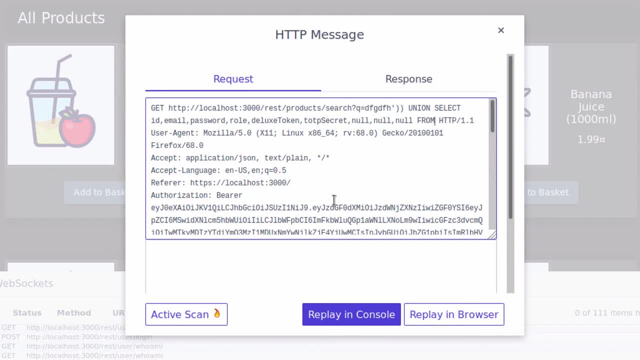 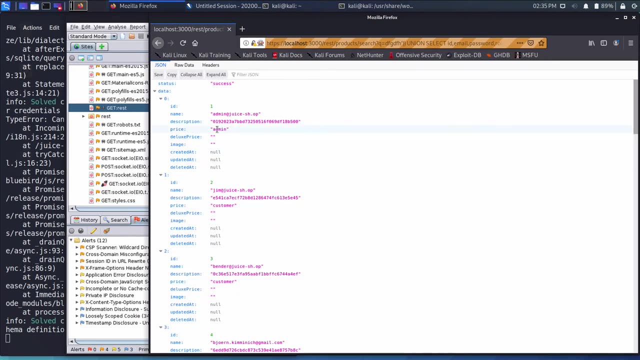 about created at, registered at or deleted at, And then we'll do from users And let's run that in the browser. Okay, so we see the same results, except now we also have a role, we also have the deluxe token and we also have that time-based. 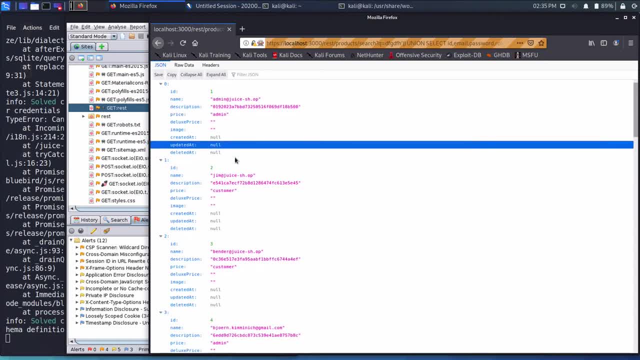 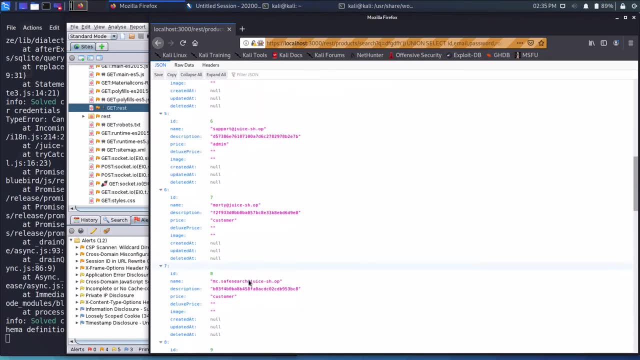 one-time password secret. Some of these do not have the values, So let's scroll down and see if we can find some that do. So this one does, And this one also has something in it, And so we can look at that Again. very similar results, except this time we were able to approach. 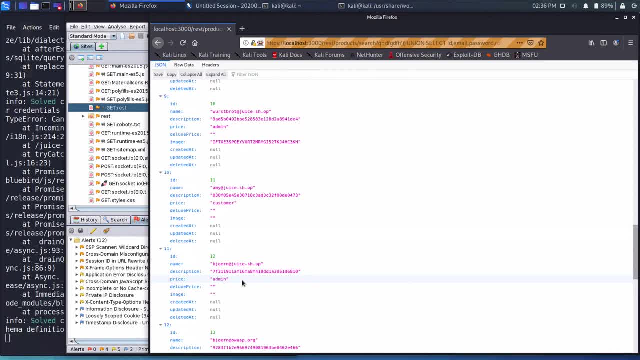 it a little bit differently because we know exactly how the user's table is structured, which helps us formulate that union attack better. All right, let's perform one more attack on the juice shot before moving on Now. we saw in a prior lesson that there is a deleted at column. 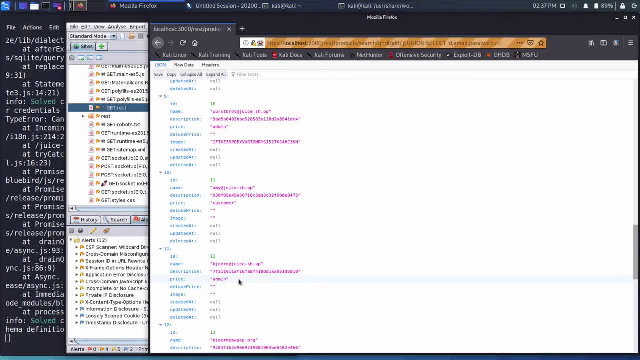 for products and we saw some products that were still in the database but that weren't supposed to be seen by customers. So let's try to order one of those products First of all. I'll go ahead and do that, And then I'll go ahead and do that. So let's go ahead and do that, And then I'll go ahead and do that. 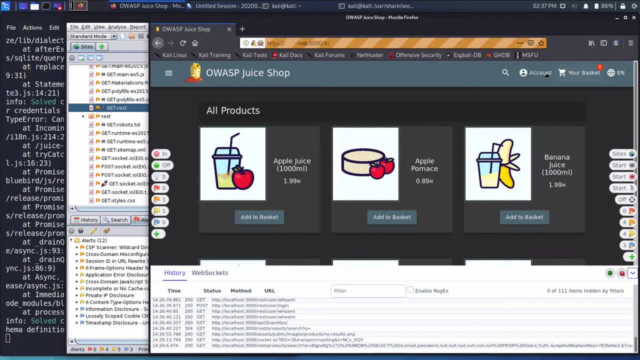 clear all of this. go back to the home page. Let's make sure that we're logged in- And we should see a basket if we're logged in- And then let's also make sure that our breakpoints are turned on. Now let's go ahead and add one of these random products to our basket, But because we 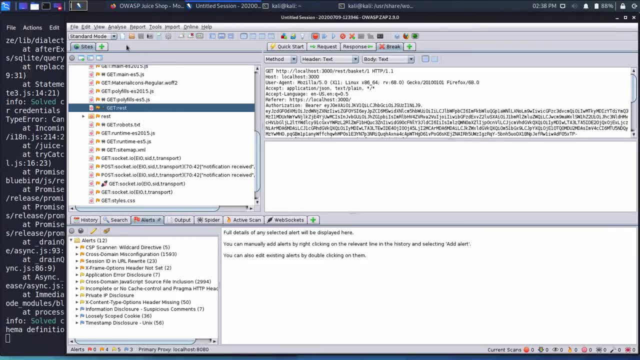 turned on a breakpoint. we should see an intercept. the request through here, So let's go ahead and step through until we see what we're looking for. Okay, still not there? All right, perfect, This is exactly what we're looking for. Okay, still not there? All right, perfect, This is exactly what. 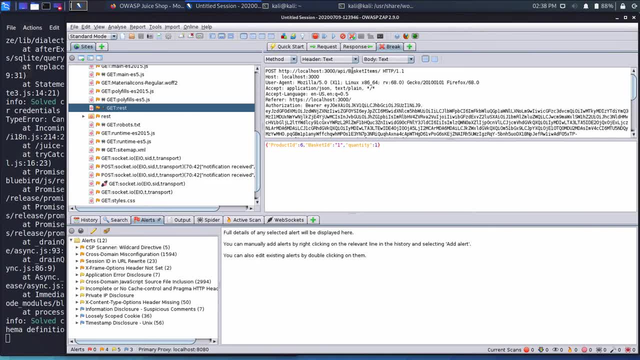 we wanted. So this is a post request to an API for basket items, But in this case it's sending the product ID that we want to add to our basket. It's sending the basket ID- our idea happens to be one- and then it's sending the quantity, But instead of sending product six, what I'd like to do is send. 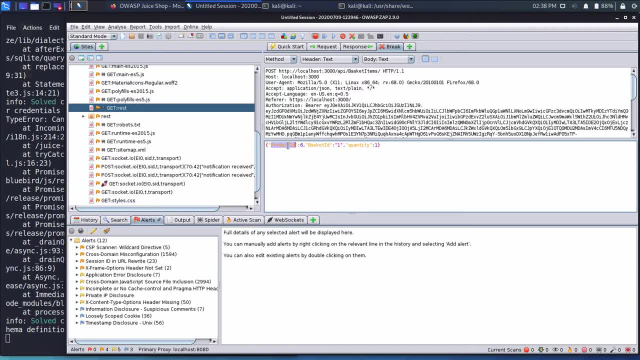 one of those hidden products And if you remember from a prior lesson, one of those hidden products was ID of 10.. So we'll change it from ID of six to ID of 10.. We could even change the basket ID and the quantity if we wanted to. So let's go ahead and do that. So, let's go ahead and do that, All right. 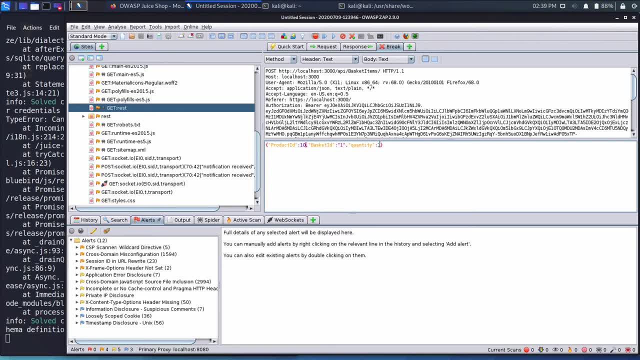 we want to try that and see what happens, But I won't do that for this example. We'll leave the defaults instead And then we'll step through which essentially is going to hijack this legitimate request, send it to the database and application And then let's see what happens. 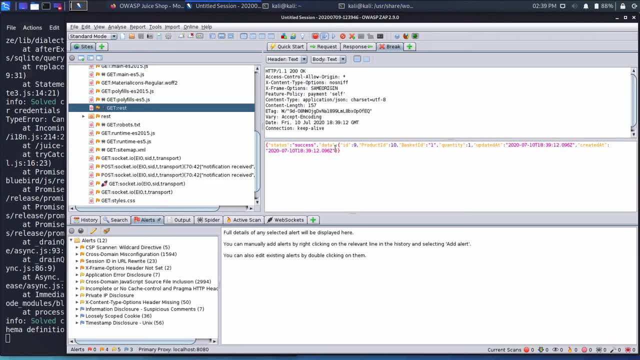 Step through some of these other calls And we see a success. This is the response we were hoping for. So success with data ID of nine, probably for the ID of the request, product ID of 10.. That's the one that we intercepted and changed the correct ID. 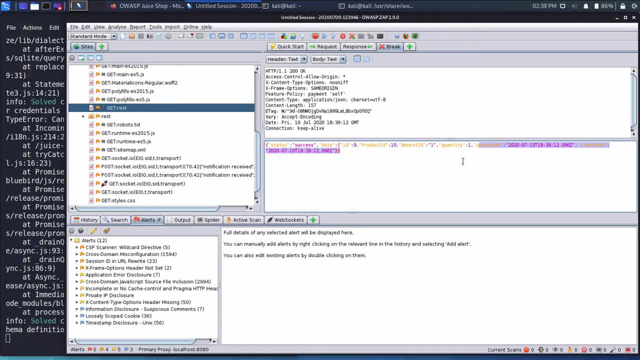 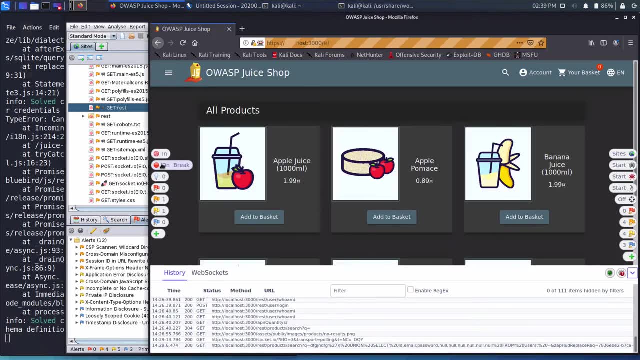 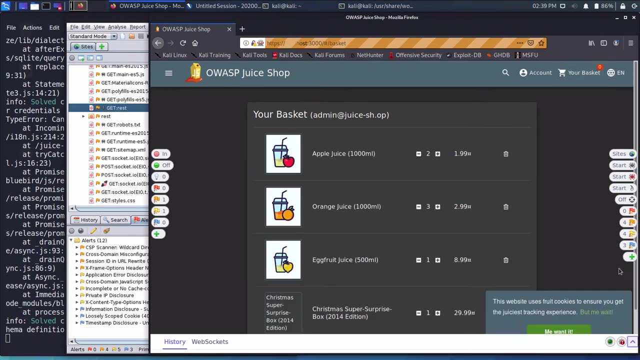 for the basket and quantity, and then some information that we don't really care about. So let's go ahead and step through the rest of these requests Now. let's pull back the application, Let's turn off breakpoints And let's go to our basket. We'll see various items We can delete. 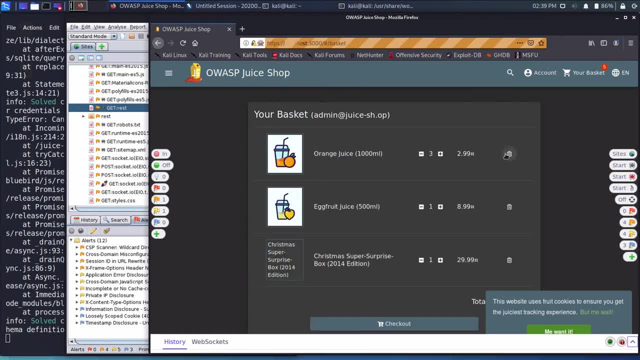 these if we want, But the one that I'm mostly interested in is the Christmas super surprise box 2014 edition, which is the one that we're not supposed to be able to order. So let's go ahead and check out to see what happens. So let's go ahead and check out to see what happens. So let's. 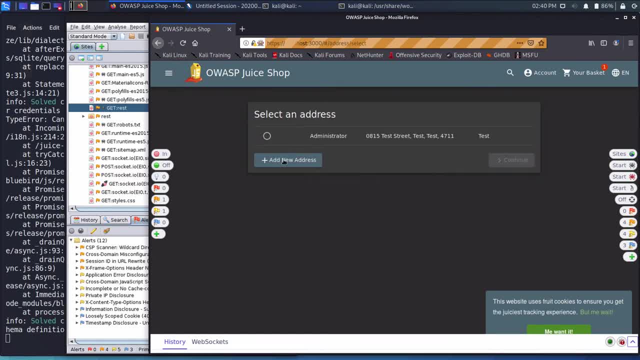 go ahead and check out to see what happens. We can select an address or we could add our own address here. Obviously, the administrator already has an address, But if we wanted to order this maliciously for ourselves, we could try to add a different address. But let's go ahead and select. 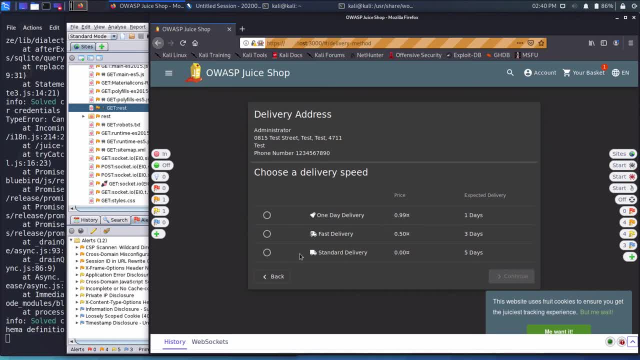 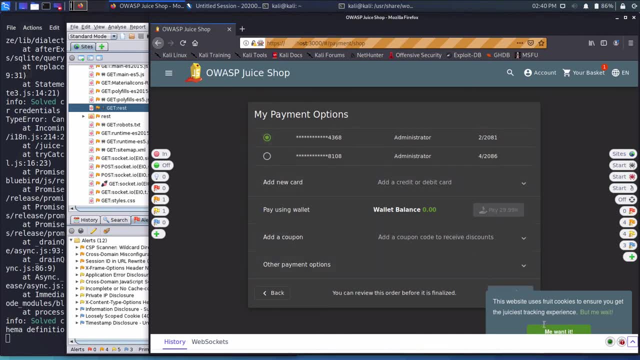 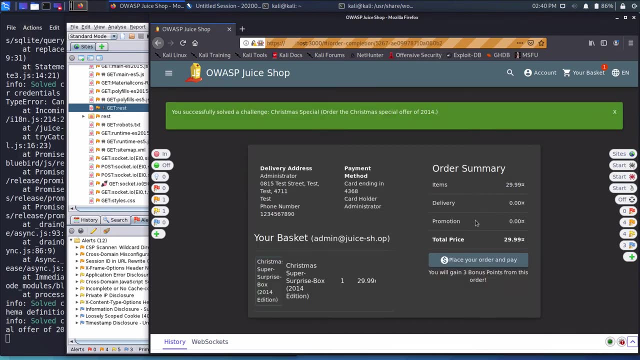 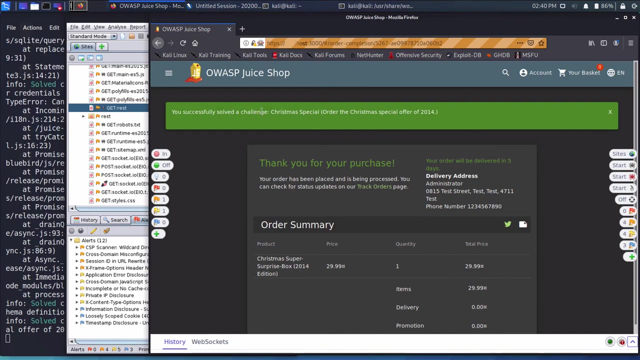 the administrators. We'll continue. We'll select one of the admins cards, We'll continue, And then we'll place our order and pay. Thank you, Mr Administrator. We've now purchased a Christmas super surprise box and we've also successfully solved a challenge called Christmas special In this lesson and 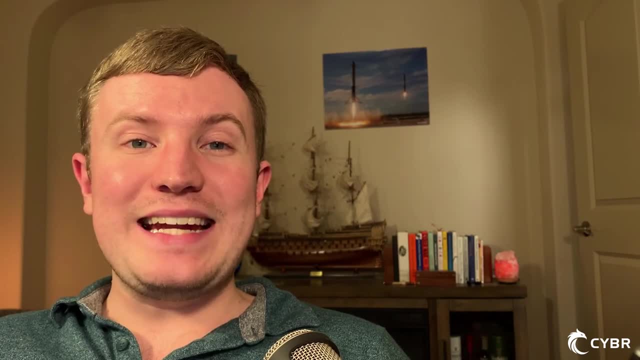 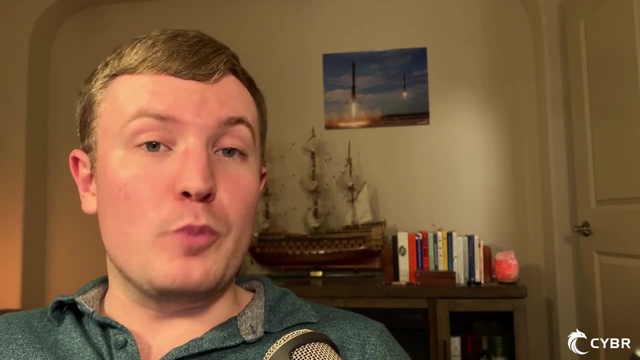 prior lessons, we not only used SQL injections to gain access to administrative accounts, but we also did things like extracting user information, And we found products that weren't supposed to be for sale anymore, but that we were able to add to our cart and then check out, And 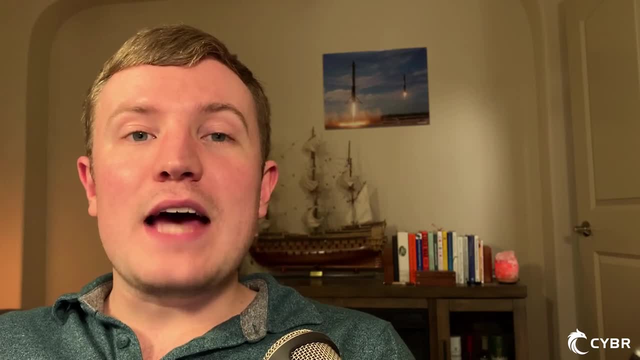 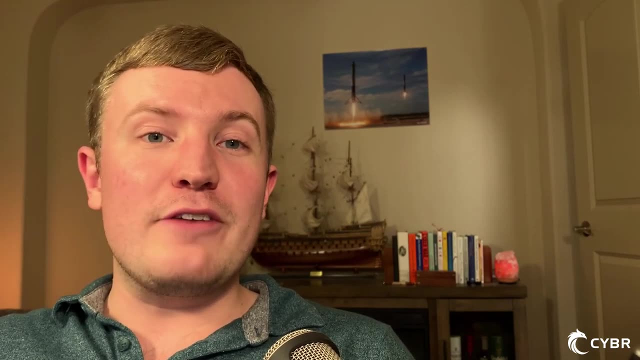 we did this by chaining a number of different attacks, But all of those attacks came from SQL injections And if we're trying to defend this application and not be malicious, then we have a lot of work left to do in order to defend this application, because clearly it's. 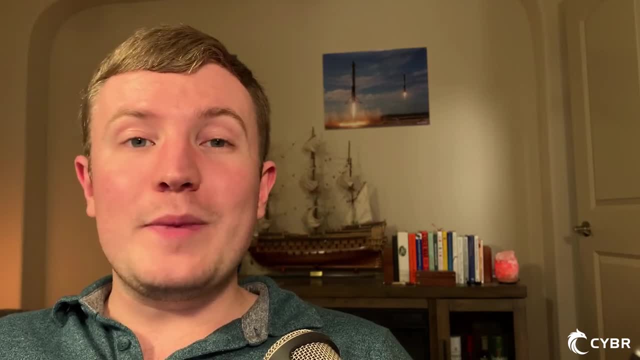 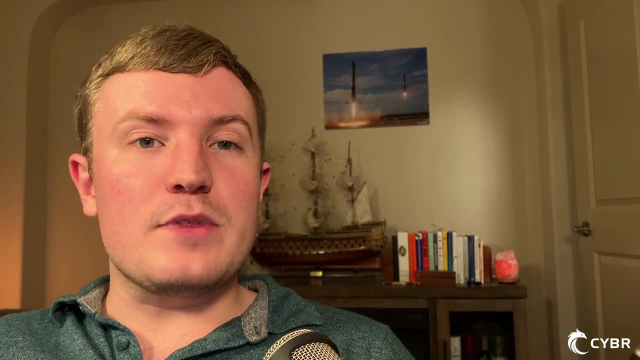 very vulnerable. Now, in the last few lessons, even though we used automated scanning with OWASP Zap, most of our attacks were very manual, And that's fine, And that's a great way to go about it and definitely something or a tool that should be in your arsenal, But we also have access to 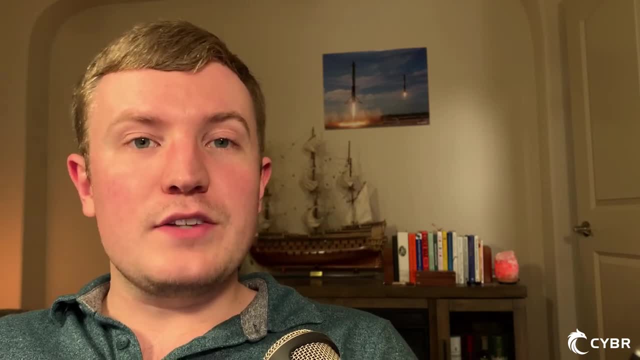 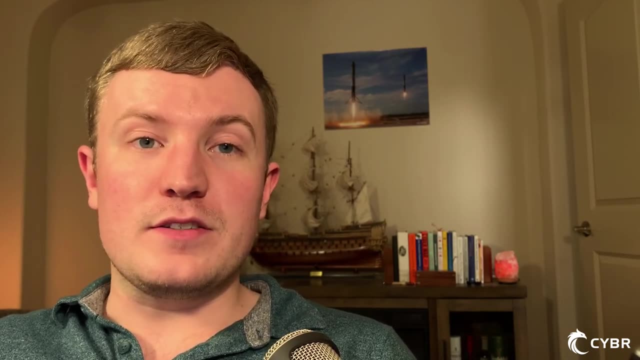 automated tools in this case, So why not use them? So in the next lesson, we'll take a look at a tool called SQL map, which can help us understand what's going on in this application, And we'll help us find vulnerabilities and then execute payloads to compromise databases. So go ahead. 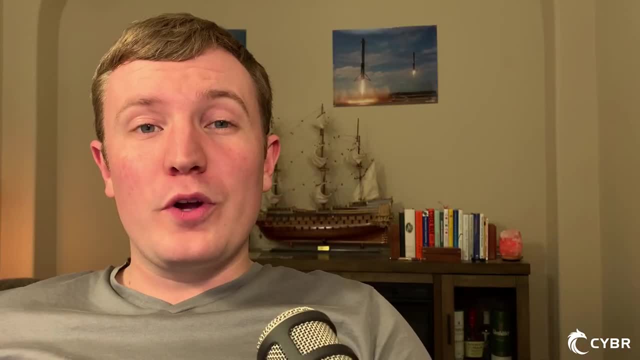 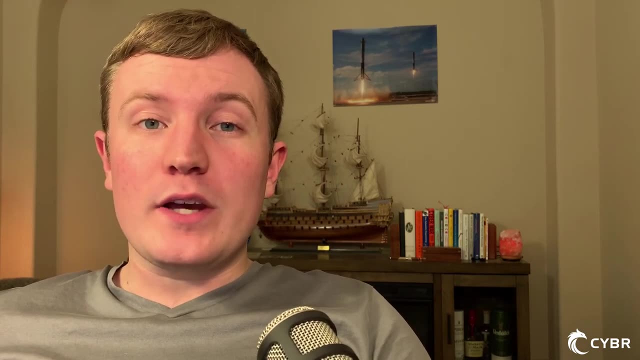 and complete this lesson and I'll see you in the next one. And until this point, apart from an automated scan by OWASP Zap, we've been performing SQL injections by hand, And in this lesson we take a look at an automated tool called SQL map. Let's take a break from the OWASP. 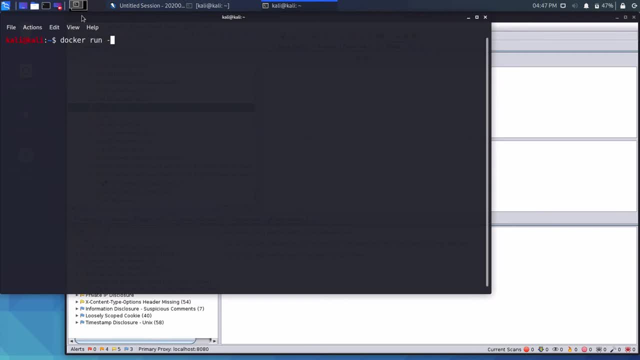 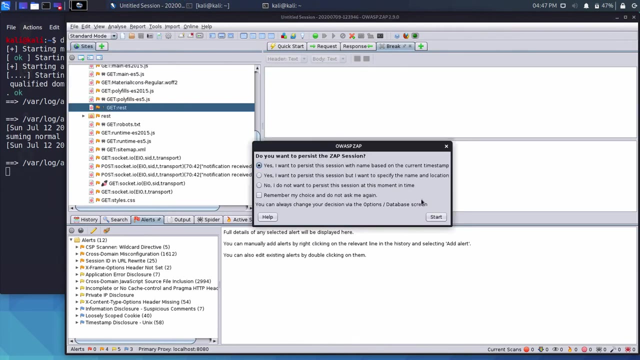 juice shop for a bit and let's switch it up. Let's pull up the damn vulnerable web application. While that's happening, we'll also start a new OWASP Zap session so that we can have a clean workspace. Once that's done, we can go to quick start and then we'll do manual exploration. 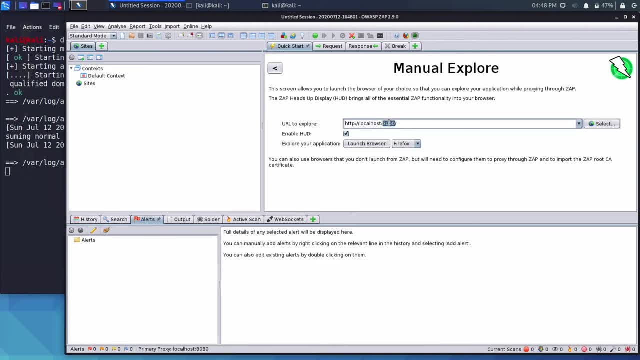 but this time we'll remove the port 3000, since the DVWA is just on port 80.. Also, in this case I'll actually disable the HUD so that we just use the OWASP Zap desktop client. Now I'll go ahead and launch the browser. We can log in with a. 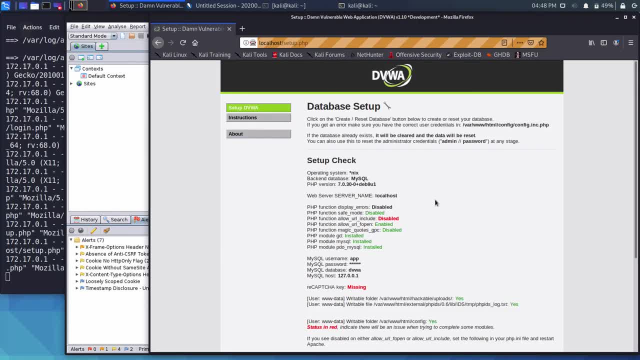 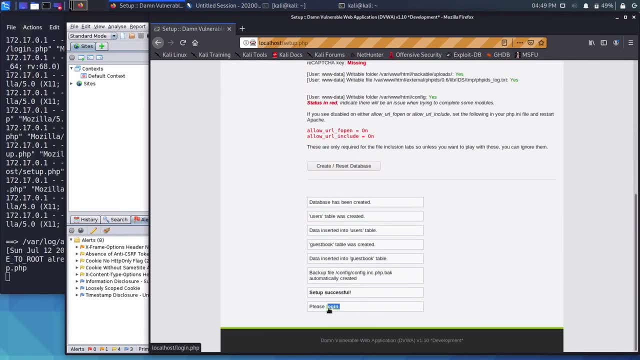 password. I believe it's admin, admin, if not, admin password. Okay, Admin, admin worked Great, Let's go down and create slash, reset the database And then we'll go ahead and log back in, And this time I believe it is admin password. Okay, yep, That worked. Now the first thing I'll 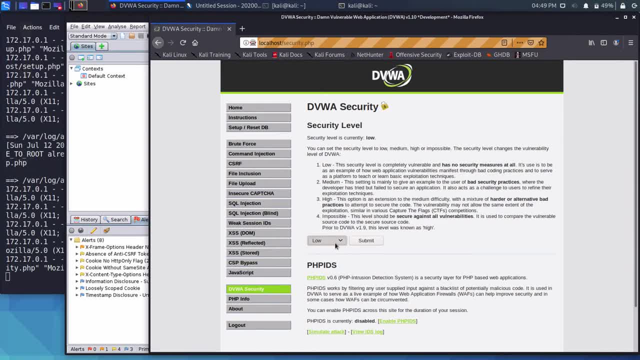 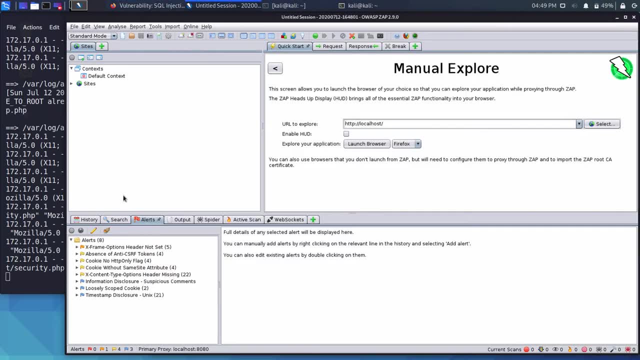 do is I'll change the security level from low to medium just to make it a little bit harder. Then I'll go over to SQL injection, the blind version. Now I'll go back to OWASP Zap and I'll click on the history tab so we can see what's going on, just like we could with the history in the awasps app. 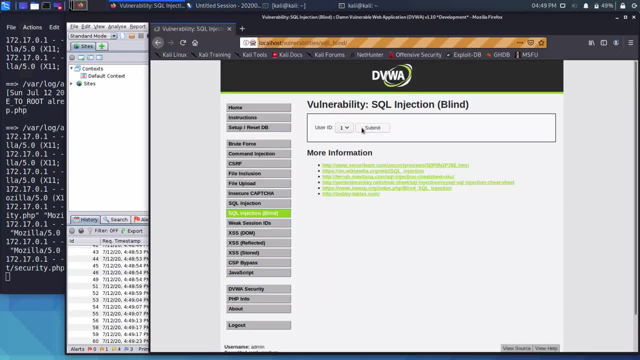 hud, i'll go back to the browser and then i'll make sure user id of one is selected- but doesn't really matter, it could be any id- and then i'll click on submit. now we get this message back and then we can see that there was a get and post request and we can open up what that request looks. 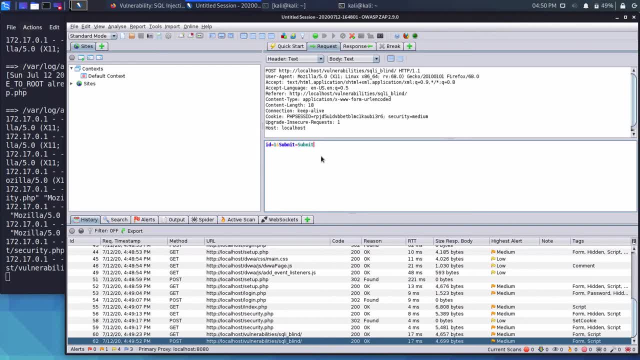 like. we have data with id of one and submit equals submit. we have a post request with this endpoint, here we have user agent, some other htp headers and then we have cookie information with php. session security equals medium, and i think that's all we'll need for our attack. so at this point we're 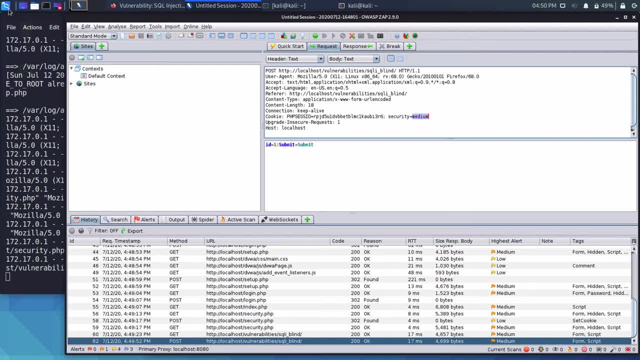 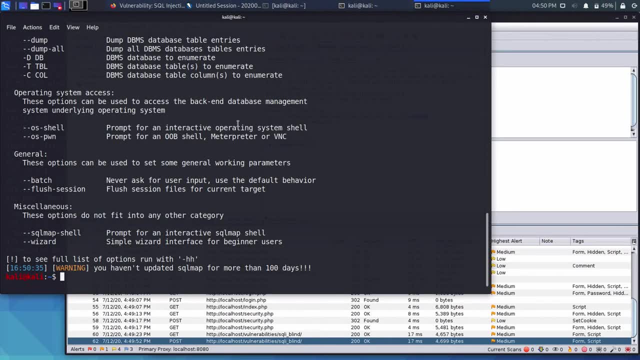 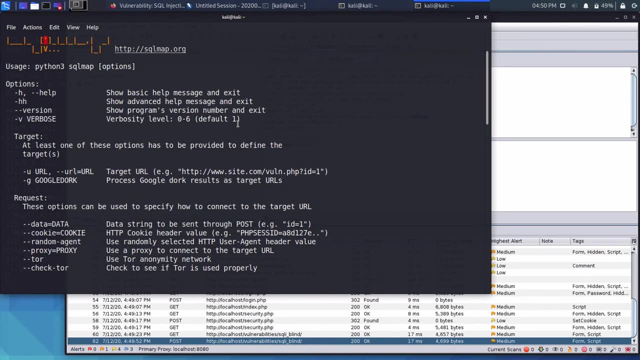 ready to pull up our tool, sql map. we can click on the kali linux icon search for sql map and pull that up now. i won't go through each setting and option, since they are fairly well documented, and i'll show you how to find that towards the end of this lesson, but there are a few options that 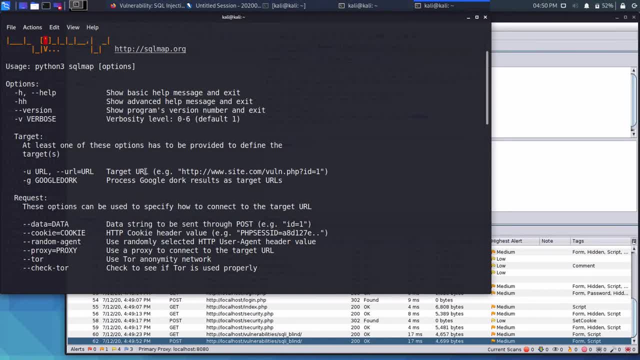 i want to mention because we will need to use them. of course, we'll need to be able to submit a target url so we can do dash url or dash u, i mean, and then dash. dash url equals url, so those two options are valid. we'll need to be able to submit data and this is the data string to be. 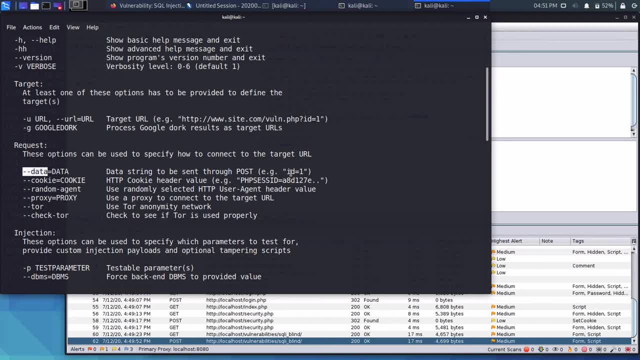 sent through the post request, such as an id number, for example, which is what we'll use in this case, but it doesn't have to be an id number. we'll also need to input cookie information and i've just pulled that up through that post request so we can see that we've got the data string and we've got. 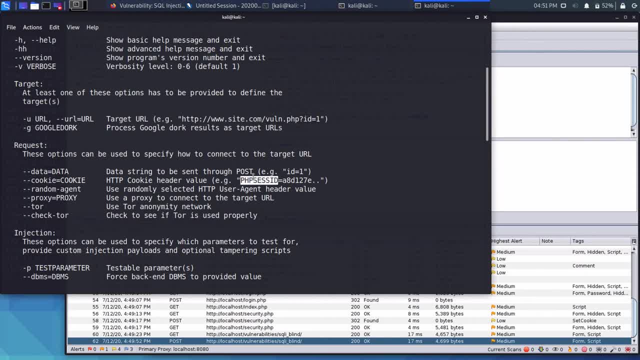 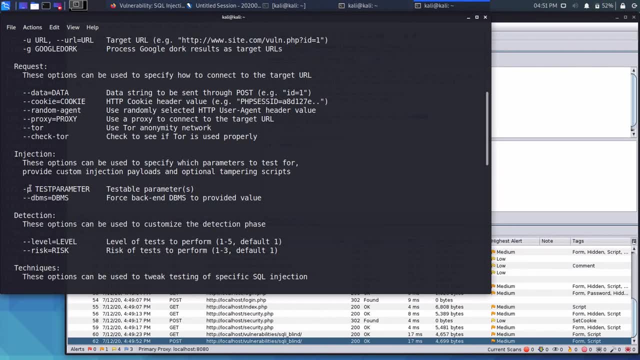 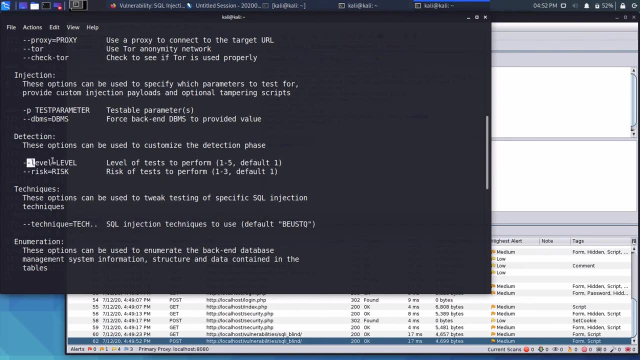 a php session id and this is what sql map will use to authenticate its requests on our behalf. we can also use the dash p option, which is the testable parameter, so in this case, again, it would be the id parameter. there are a couple of detection options where you can specify a level of tests to. 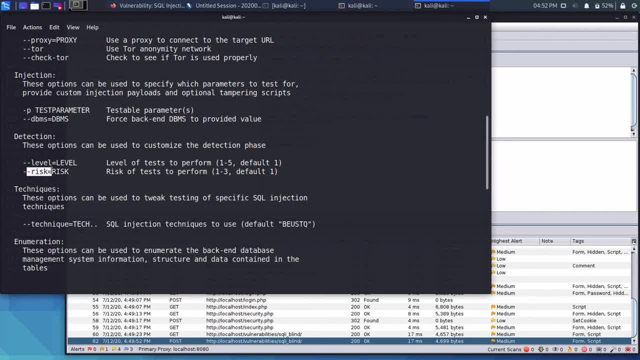 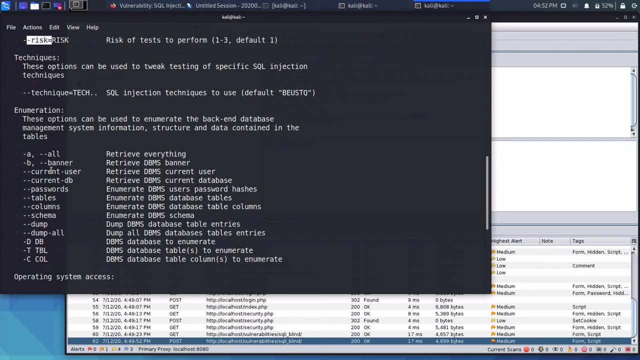 be performed and the risk level as well. again, this is fairly well documented, so i won't go into too much depth, but i'll show you how to find this information if you are curious. and then there are options that can be used to identify the testable parameter. so, for example, if i want to identify a 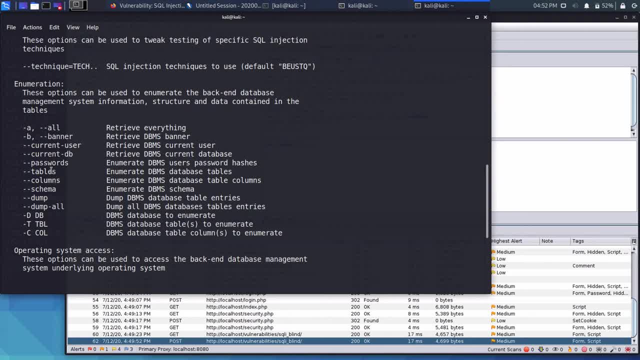 testable parameter. it will be a list of the data that's being used to enumerate the backend database system structure and data, and i don't see it listed here, by the way, but we will use one that is dash dash dbs, which enumerates the dbms databases. so keep in mind that these are not the only. 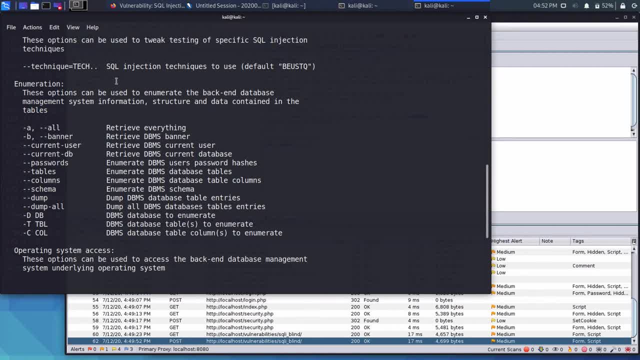 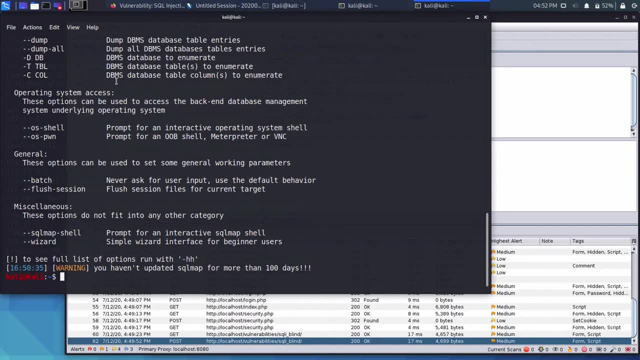 options you have access to. this help menu here does shorten down the list of options, so there are more that you can find in the documentation. so, okay, let's go ahead and formulate our attack and payload. i'll start with sql map. dash you for url and then i'll paste the url from our 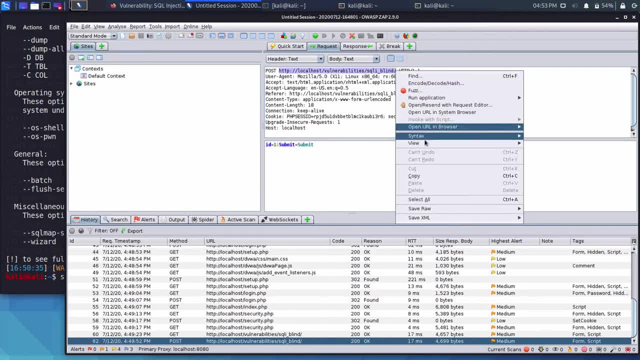 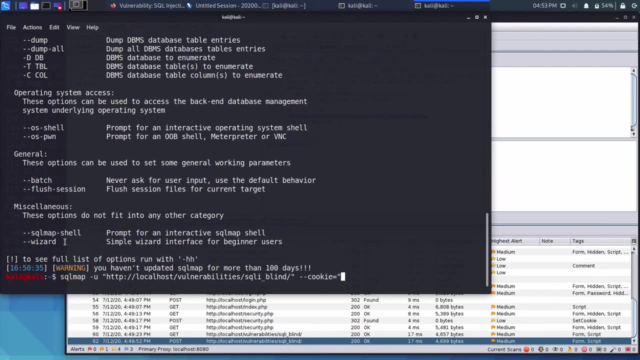 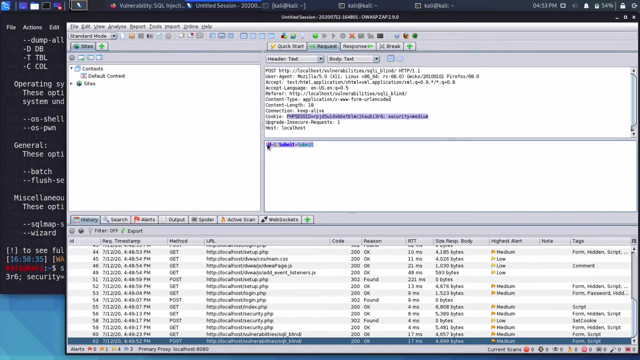 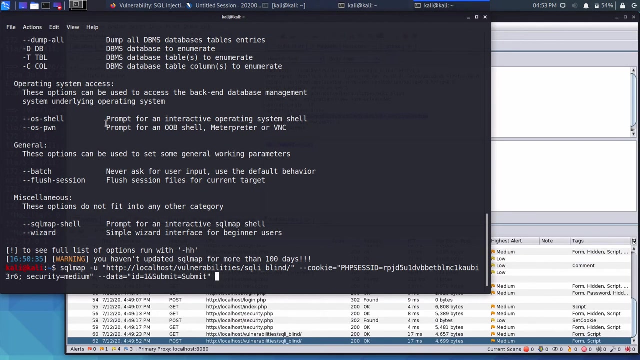 our request, Then we'll put in our cookies again. this is something I can copy from here. I'll want to put in my data which is going to have the ID submitted, and submit equals submit, And then we'll want to specify the parameter that we want to try and attack, which is the. 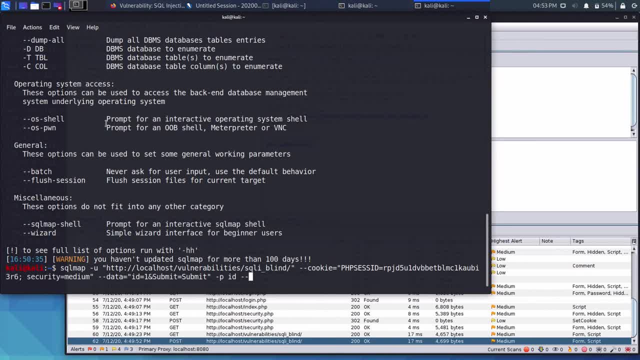 ID parameter. And then again, like I said, the last option we'll put in is dash dash DBS in order to tell SQL map that we want it to enumerate the database management system databases. so that we can see what's going on, I'll go ahead and press enter now. 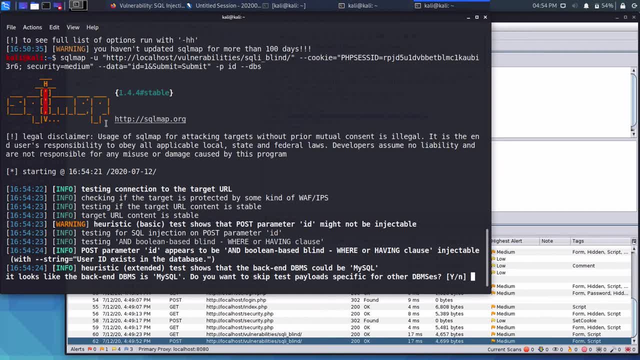 Now, as this happens, sometimes, we'll get different prompts, which is SQL map asking us how we want to proceed. There are defaults, and next time I'll show you how to skip these steps so that it just goes with the defaults. But for now I'll go ahead and say yes, because in this case, it seems to have found out that 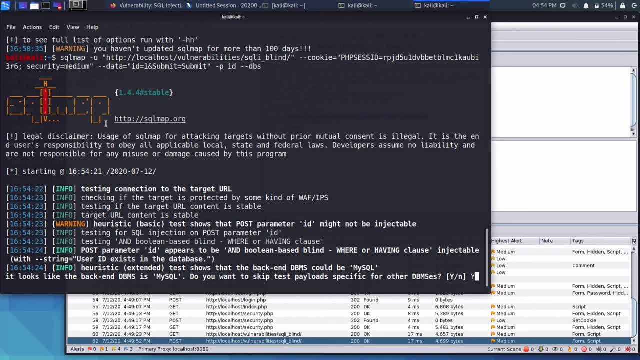 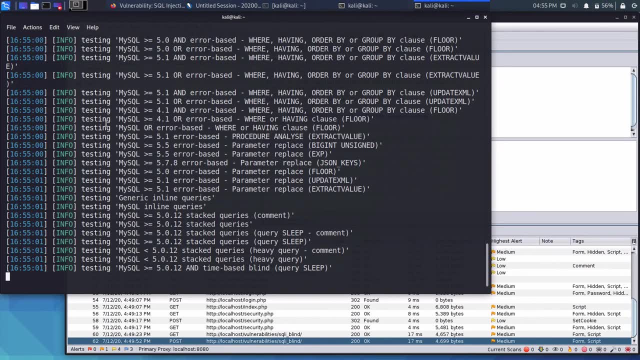 the DBMS is likely to be MySQL, so it will help it narrow down the types of attacks that it will perform. Again, I'll say yes to this, And now we can see, via the verbose information, what kinds of attacks are happening. 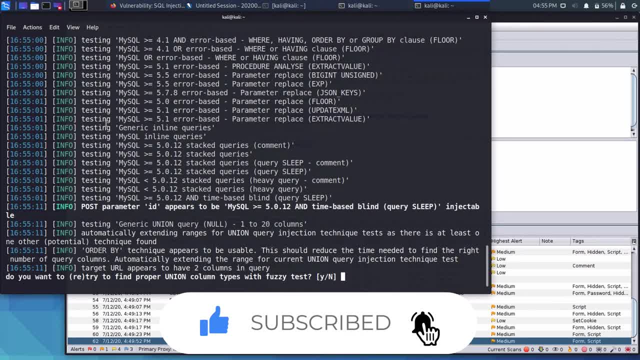 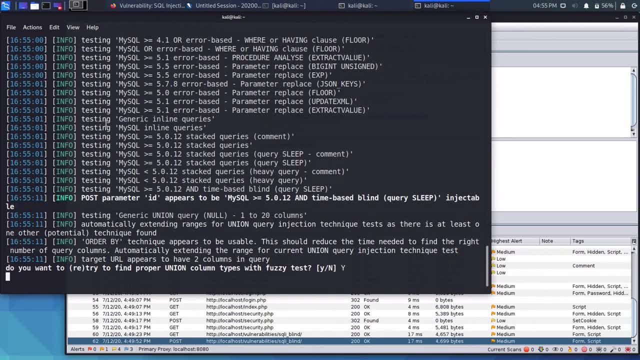 And, as we can see, there are stacked attacks, time-based attacks, error-based attacks and others. Now it asks us if we want to try to find proper union column types with fuzzy test And we'll say yes, But it tells us that the injection is not exploitable with null values. 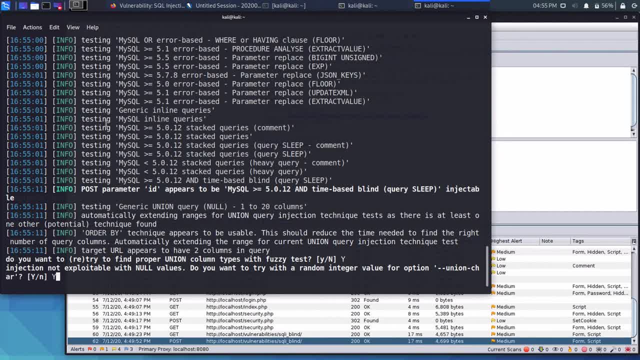 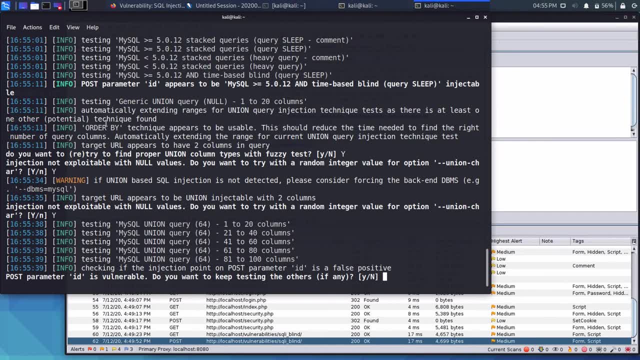 So do we want to try a random integer value for the option? We'll say yes Again. yes, So it has found out that the ID parameter is vulnerable. So it's asking us if we want to keep trying to test other parameters, And since we don't have any others that we want to test, we'll just go ahead and say: 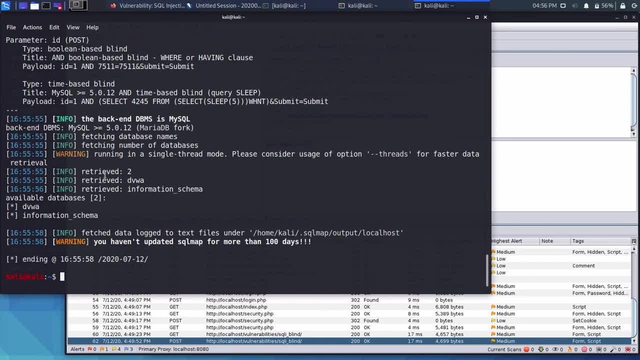 no, And now it's retrieving the information and it's found out that there are two databases. There's a DVWA database and the information schema, which we're already very familiar with. Okay, so we found a vulnerable input and we've got two database names. 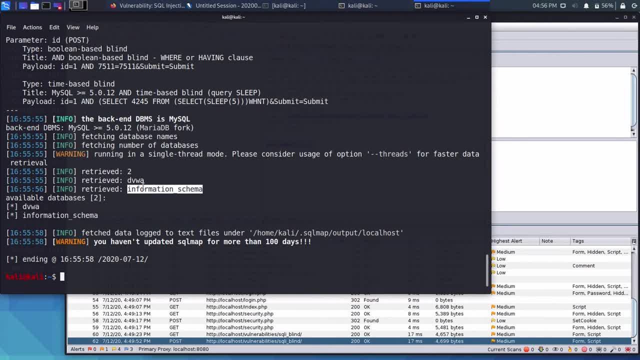 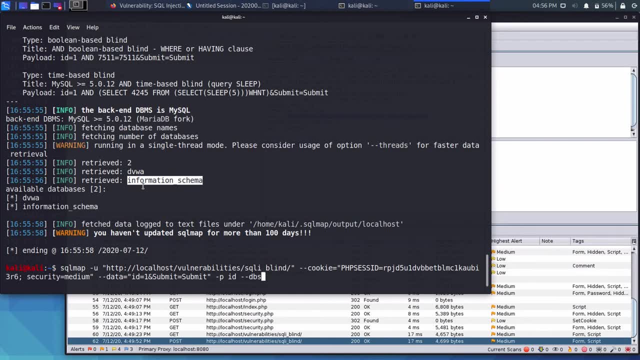 Now let's go ahead and explore the DVWA database. So we can replay the same command that we did previously, But this time, instead of running dash dash DBS, we will want to extract the table names with dash dash tables. But since we really only care about the DVWA database, I'll do dash D DVWA to limit our 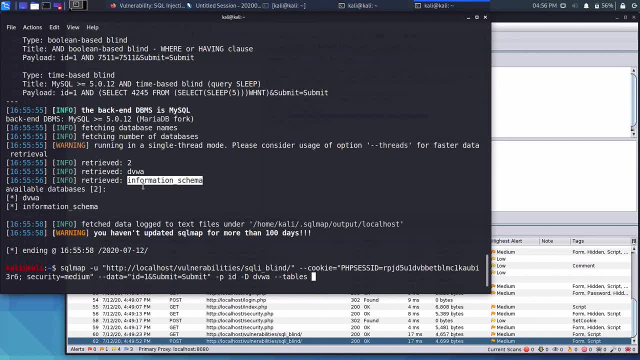 results. And instead of having to answer every single prompt, like we did last time, which can be annoying, I'll do dash, dash batch, which will automatically go with the defaults. Also, to speed things up a little bit, I'll increase the number of threads to five. 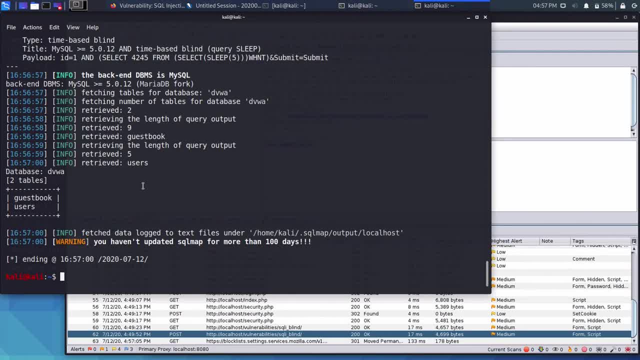 Let's go ahead and press enter and see what happens. Okay, That was really fast. So in the DVWA database there are two tables: We've got a guest book table And we've got a user statement. To speed all of this up, we'll go ahead and create an instrument that does all the same. 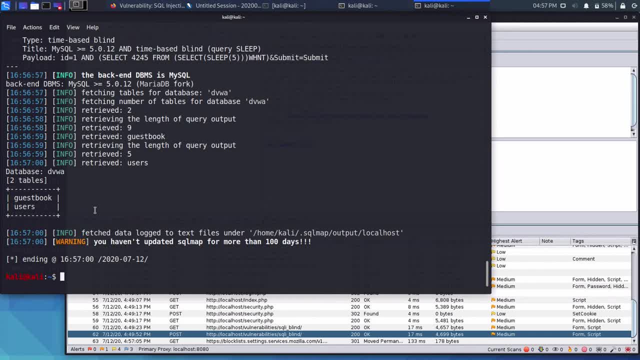 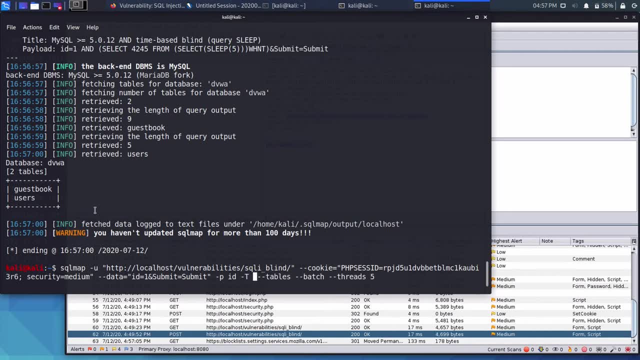 users table. So let's go ahead and extract information from that users table and we can replace the dash d option from our prior command to instead be dash t for table and then specify the table name of users. We'll remove the dash dash tables. We'll keep batch and threads, but 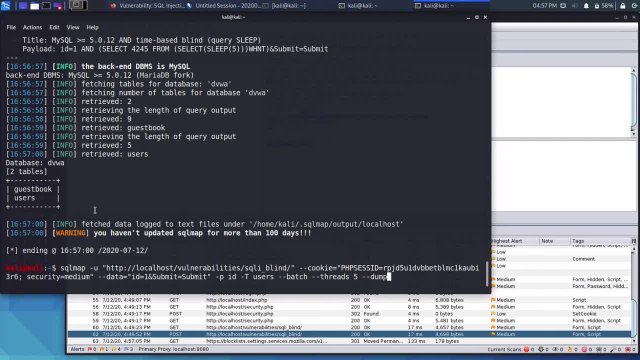 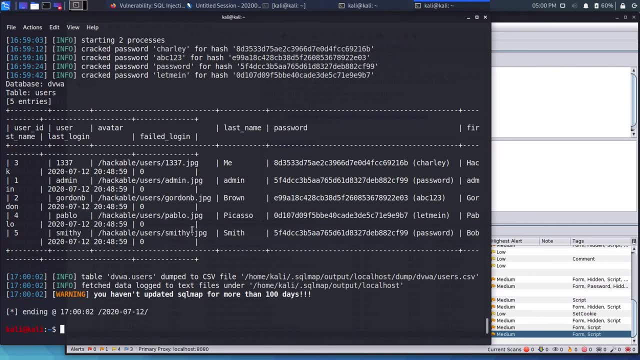 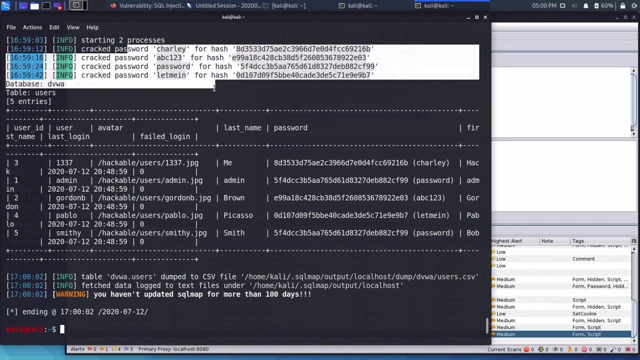 the last thing I'll add is dash, dash dump so that it shows us what information is in that table. Now, at this point, not only did it extract all the information from the users table, but the default options also attempted to crack the passwords, as we can see up here And since, 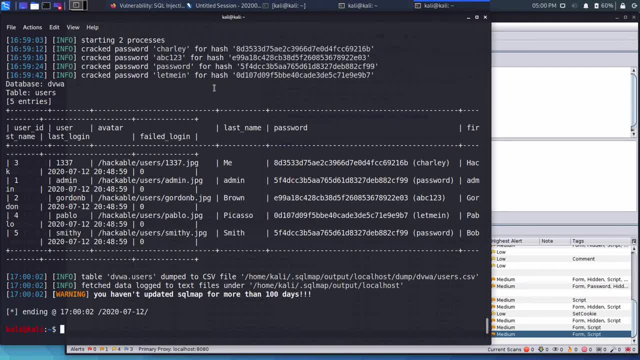 they were easy passwords and md5 hashes. it cracked them in very little time. This maybe took a couple of minutes in total. So now the output contains the md5 hash, but it also contains the actual cracked passwords. So already you can start to see the amount of data that we can 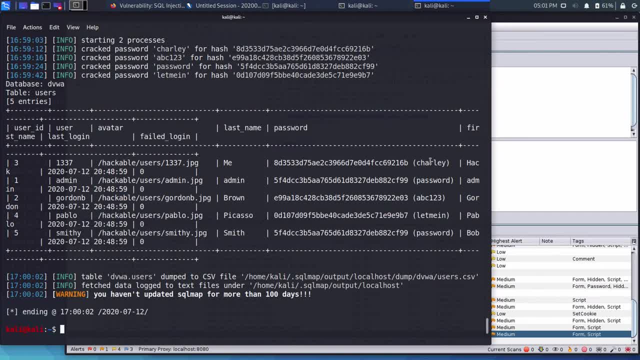 extract in a very short amount of time using a tool like sqlmap, because doing this manually, while still very possible, we're going to have a lot of data that we're going to be able to extract in a very short amount of time using a tool like sqlmap, because doing this manually, while still very 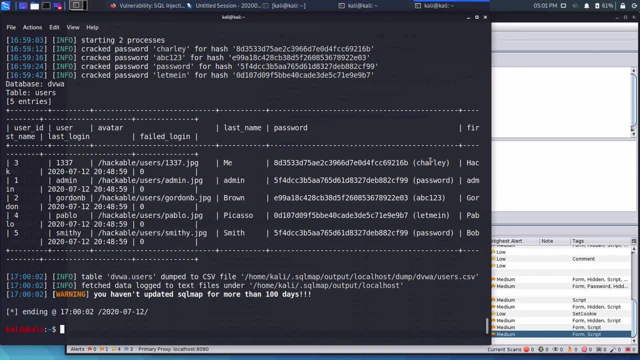 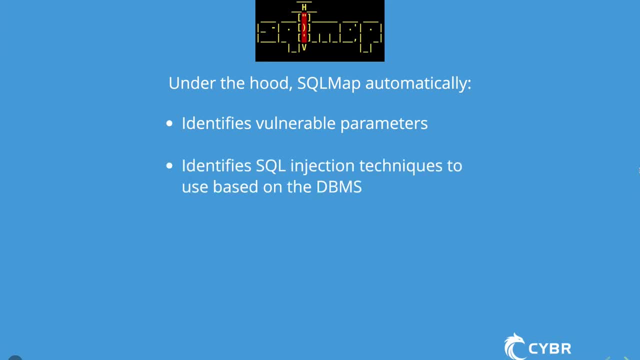 possible. we're going to have a lot of data that we're going to be able to extract in a very Sean, much, much longer. And it's able to do this because, under the hood, sqlmap automatically identifies vulnerable parameters. It identifies which sql injection techniques can be used to. 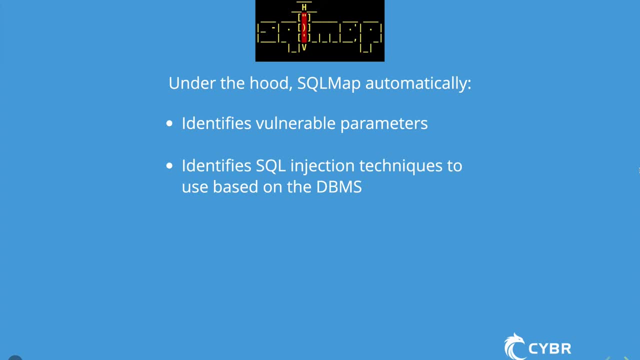 exploit those vulnerable parameters by trying various techniques for different database management systems, unless it already knows what the DBMS is running, in which case it can drastically reduce the number of techniques to try. It also fingerprints the backend DBMS so that it can gather as much information as it can back end to back-end DBMS. 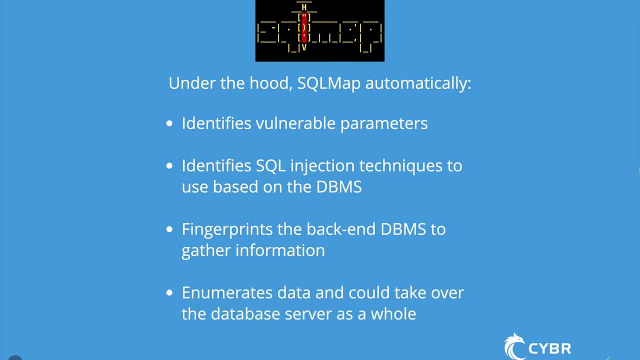 again helping narrow down attacks. And depending on how vulnerable the application is and also what options you choose, SQL Map can automatically enumerate data or take over database servers as a whole. For example, if you're curious and interested, there are ways of using SQL Map to take control of the underlying operating system. 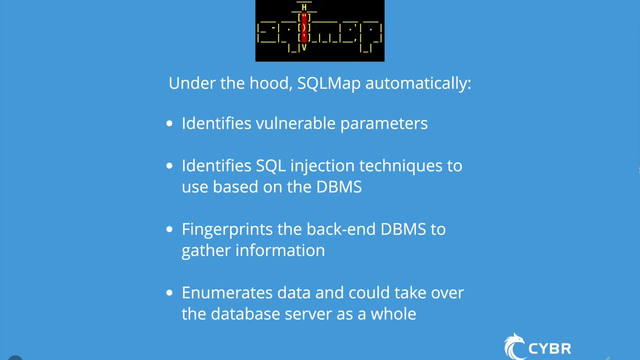 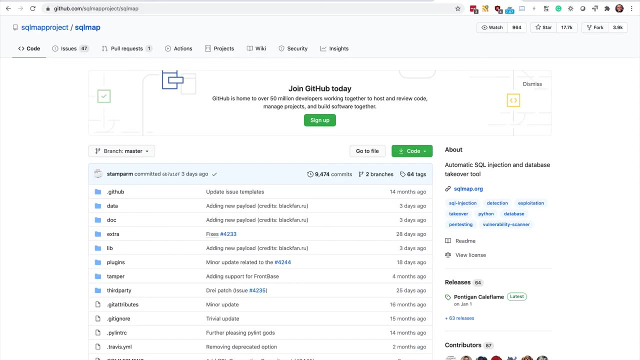 and at this point I'm not actually sure if that's possible on the damn vulnerable web application. but, like I said, if you're curious, definitely something to look into. Oh, and one more thing: SQL Map uses the same techniques that we've already learned about. 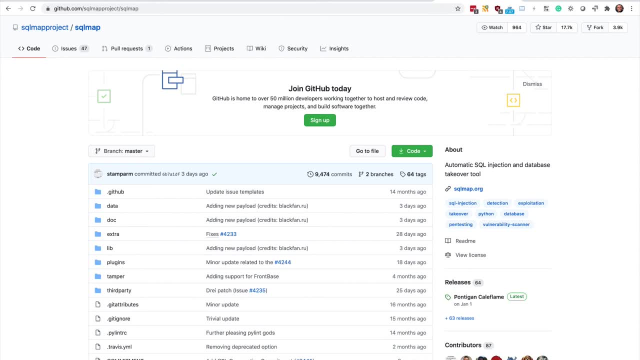 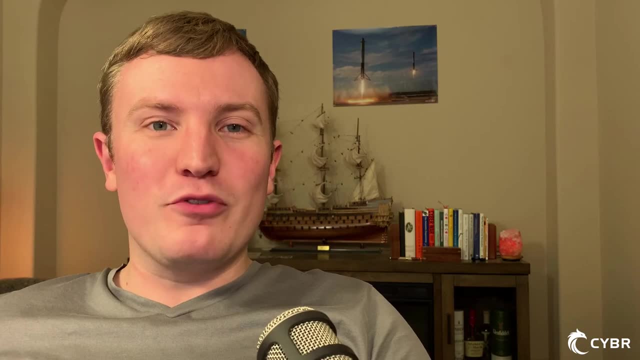 but if you're really curious to learn more about it, definitely check out its GitHub as well as its documentation. And that concludes it for our attacks with SQL Map. you may now complete this lesson and move on to the next. We've now shown what SQL Injections are by discussing and performing different types of. 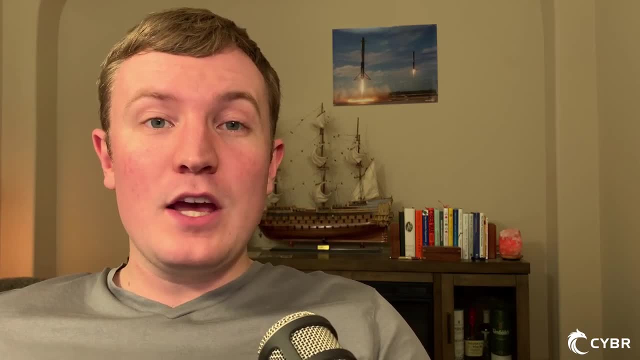 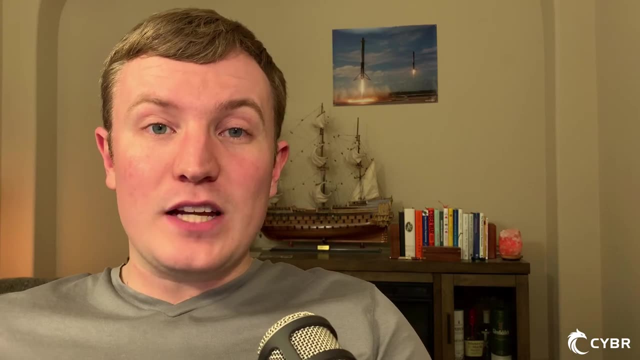 attacks, and we've seen how powerful, successful attacks can be without even looking at a single line of code. But the question remains: what can we do to defend our application and its databases against SQL Injections? In the next few lessons we'll take a look. 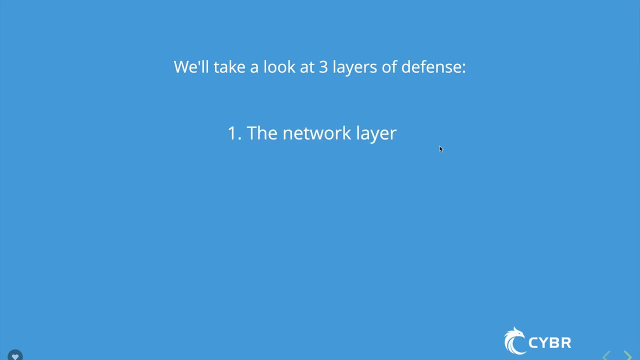 at three layers of defense. We've got the networking layer, ie firewalls, we've got the application layer and we've got the database layer, Because, while the implementation can vary a bit depending on what languages, DBMS and environments we're running, there are a set of key concepts that remain constant. 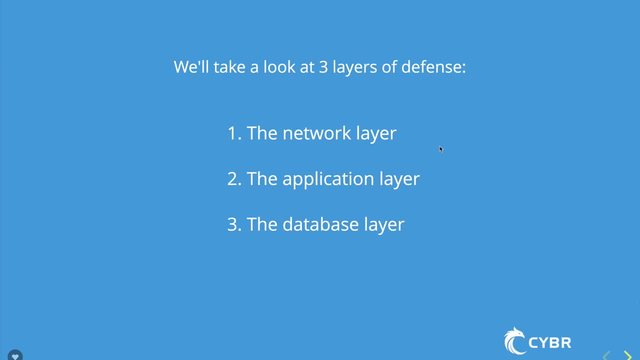 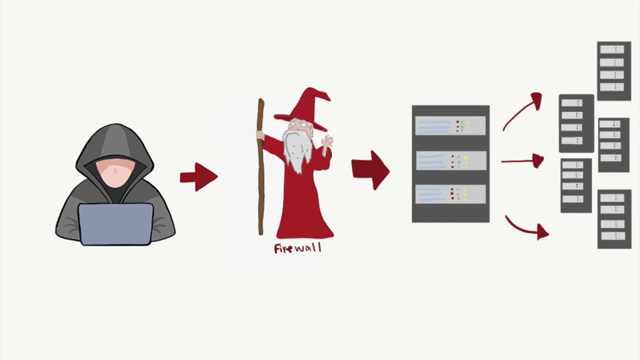 and that we should be familiar with. So let's start with the network layer. Before a request ever gets to your application and database, it can be analyzed by a web application firewall, or WAF for short, And we talked about WAFs in our Introduction. 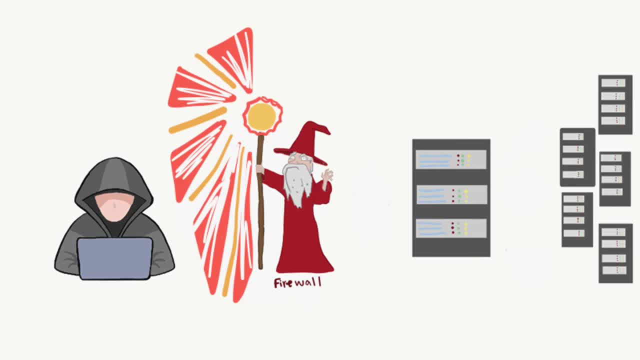 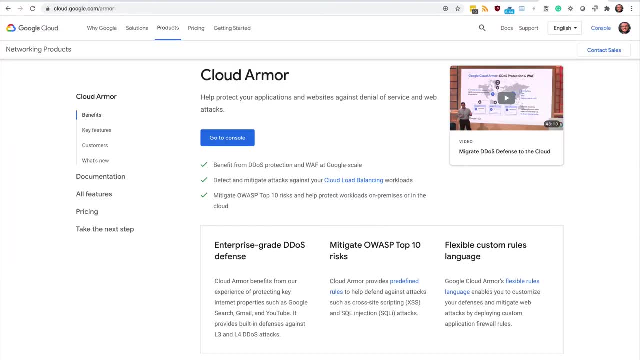 to Application Security course because they can help block requests that look malicious or abnormal. There are many of them out there. for example, AWS, Azure and GCP all have their own versions of WAFs, and there are third parties that also offer their own, and they all vary. 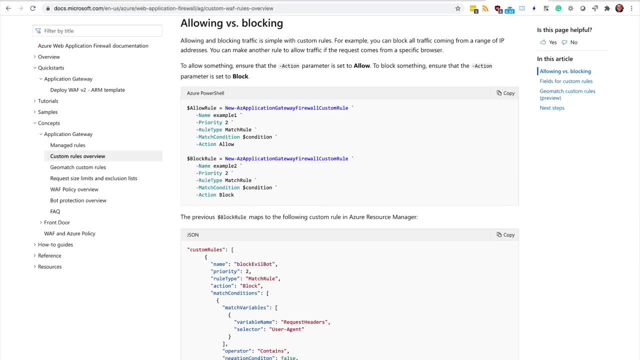 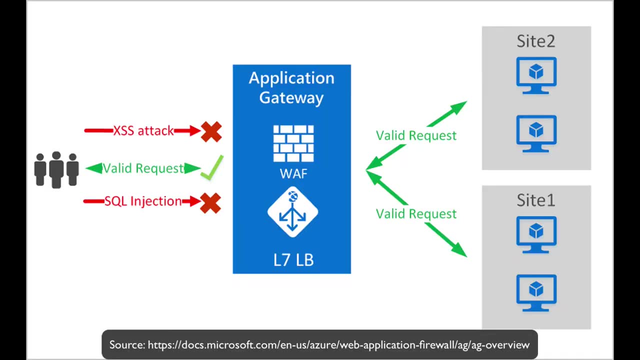 in terms of complexity and in terms of how advanced they are. A lot of them. let you customize rules and they come with their own set of rules that can block a lot of common SQL Injections, so that the requests never even reach a single line of your code in the APIs. And, of course, 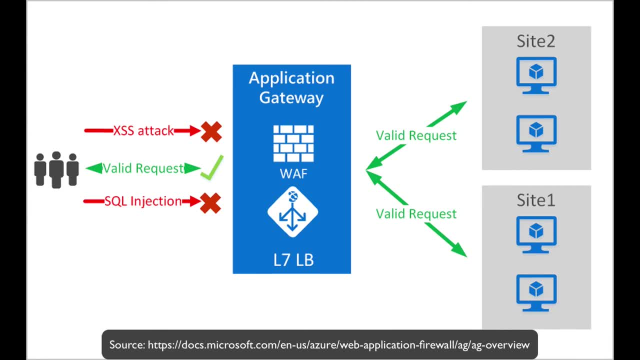 that's what we want to happen, because ideally we want to block SQL Injection attempts as far away from the database as possible. But firewalls are not a silver bullet. they can only do so much, In fact. the then-Oracle VP of Database Security. 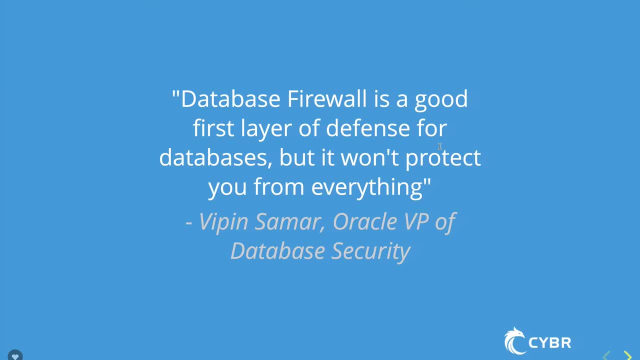 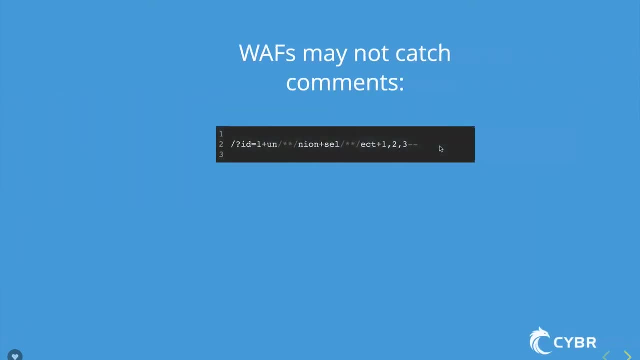 was quoted as saying that database firewall is a good first layer of defense for databases, but it won't protect you from everything And in fact there are ways of bypassing WAFs. For example, some web application firewalls may not catch comments, And in this case 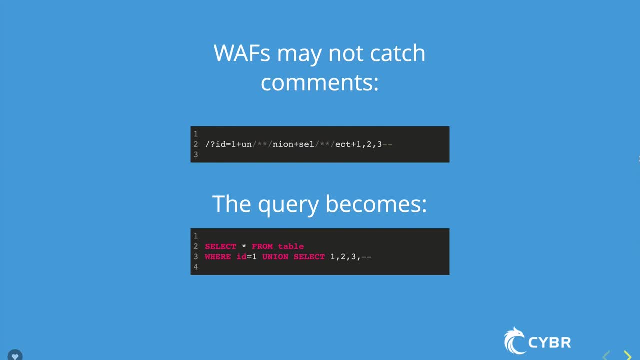 the request would become a SELECT FROM statement where id equals 1 with a union select 123.. Some also only look for lowercase or uppercase SQL keywords, so we can switch it up a bit. Also, we can use synonyms so we could replace equals and not equals with these signs instead. 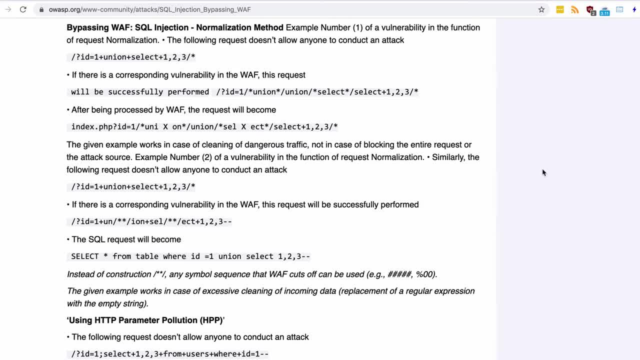 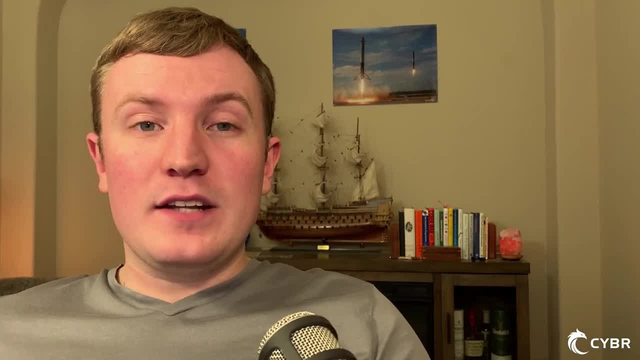 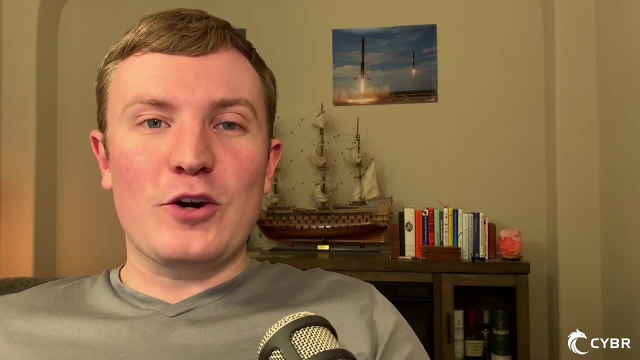 And these are just some of the examples, but there are many more examples of bypassing WAFs at this URL. So when we build our applications, we have to pretend like there's no firewall in place and build security controls in the code itself. But that concludes it for this lesson. you may not complete it and move on to the next. 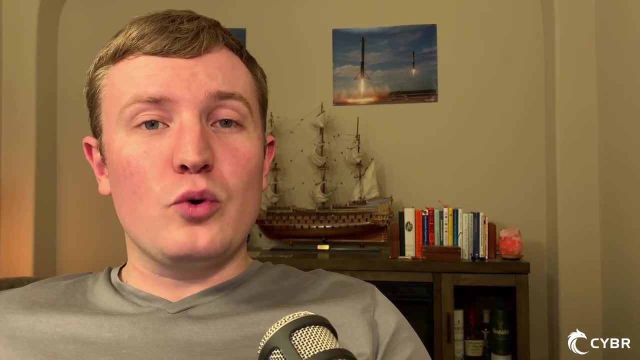 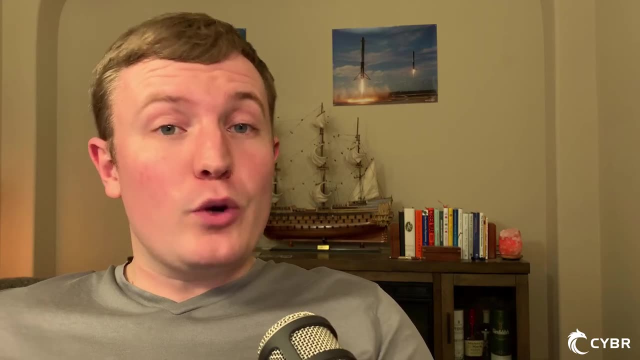 Now that we've looked at the networking layer, let's take a look at some security controls and defenses that we can apply at the application layer, And the good news is that preventing SQL Injections is actually quite simple, Since SQL Injections happen when users. 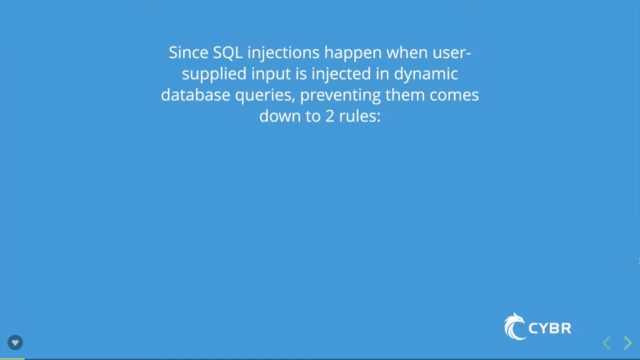 supply a dynamic database query with a user-supplied input. Now the bad news is that SQL Injections are still very common, which means that FAR too many applications are not implementing these two basic rules. Don't be one of those applications. JETGRAVE, SCREEN ihrem. 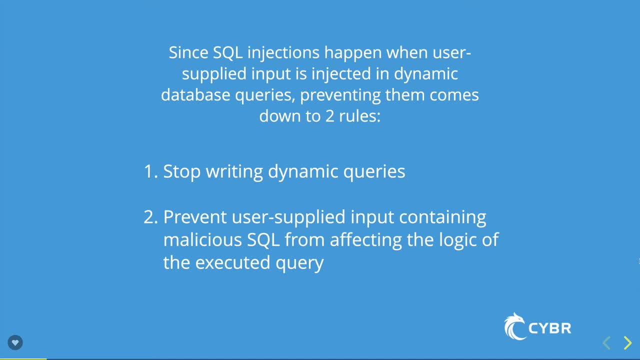 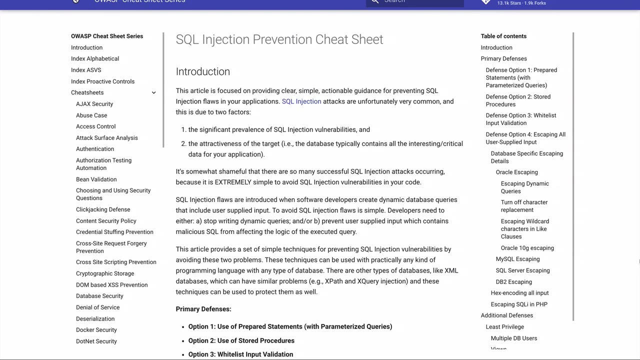 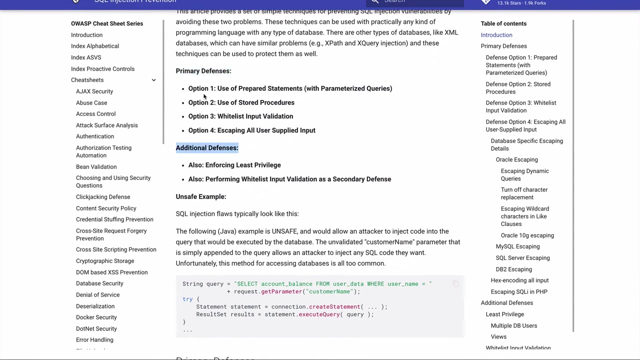 The OWASP organization has created numerous resources that can help us defend our applications, so let's go through them so that you can reference them as needed. The first one we'll look at is this SQL Injection Prevention Cheat Sheet, and on this page they list out primary defenses as well as additional defenses. 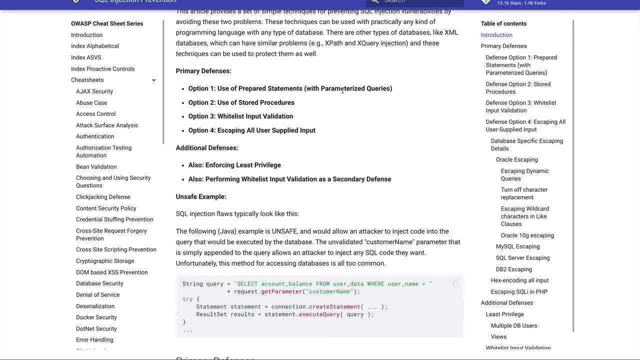 The first option is using prepared statements with parameterized queries. Option number two is use of stored procedures. number three is whitelist input validation and number four is escaping all user-supplied input As additional defenses. they also mention enforcing least privileges, which we'll. 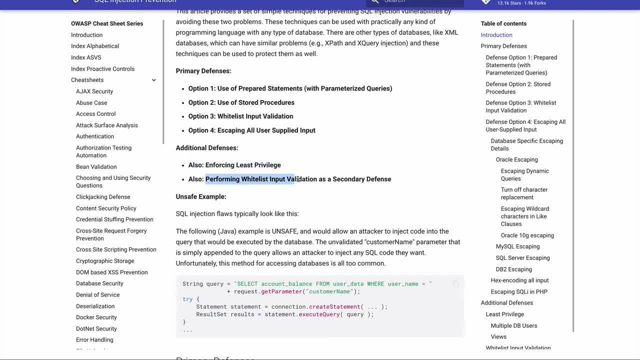 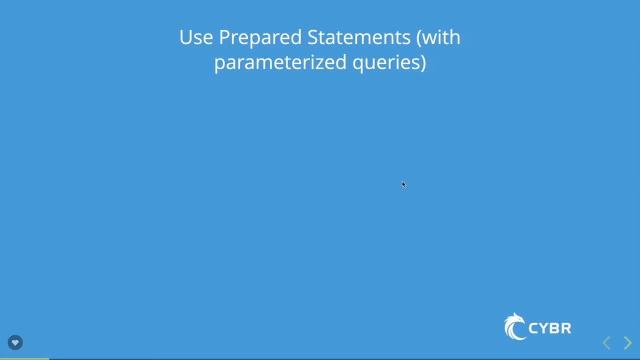 talk about in the next lesson, and also performing whitelist input validation as a secondary defense. So let's take a look at all of these in more detail. Prepared statements are beneficial because, number one, this coding style helps distinguish between code and data and, number two, prepared statements define the intent of the query. 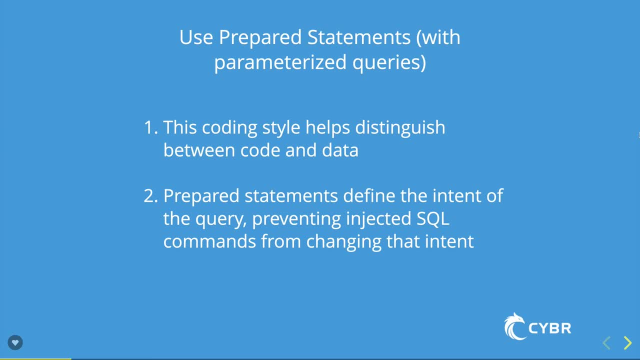 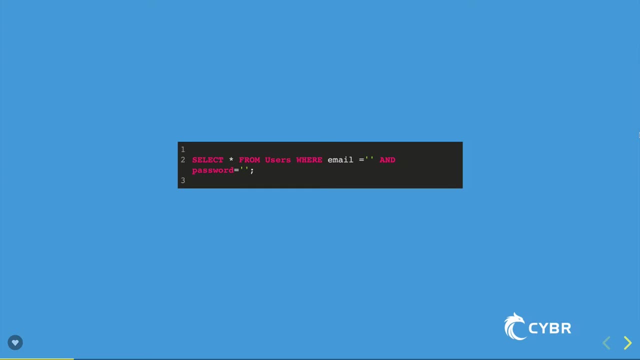 preventing injected SQL commands from changing that intent. So if we have this SQL code which is to select everything from the users table, where email equals a user input and password also equals a user input, if an attacker tries to inject this code, it would turn that injection into a harmless string. 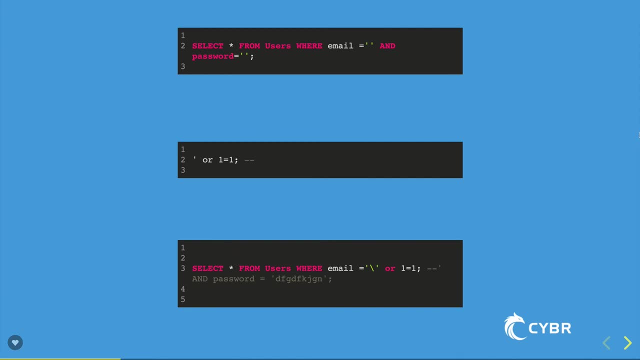 So it would actually evaluate that SQL injection as a string instead of evaluating the or one equals one statement, and in fact I just realized that my interpreter is interpreting the commenting out of and password, but in reality, with our prepared statements, it would not comment. 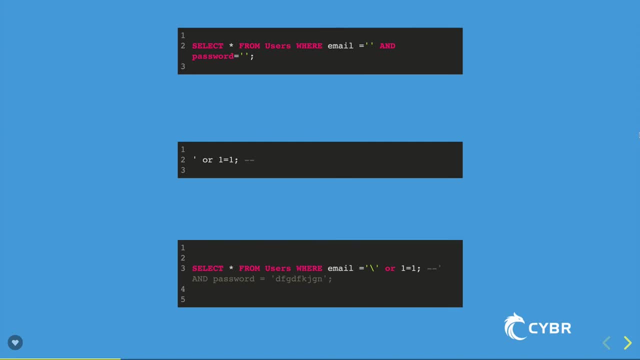 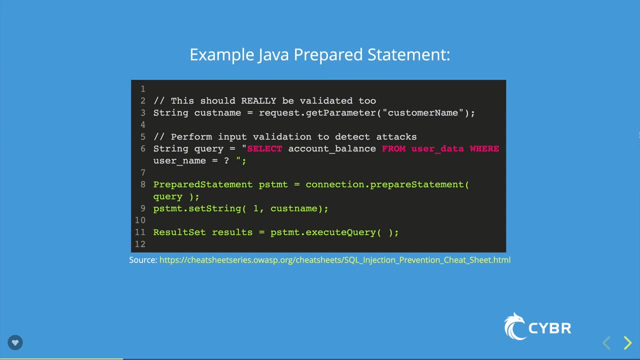 it out, it would look at that as a string. So here's an example of a prepared statement in Java code and this is pulling straight from that SQL injection prevention cheat sheet, and they do have some other examples on that page Also. we'll take a look at some other examples ourselves. 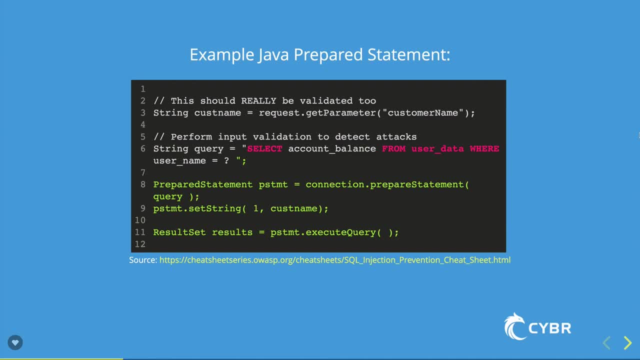 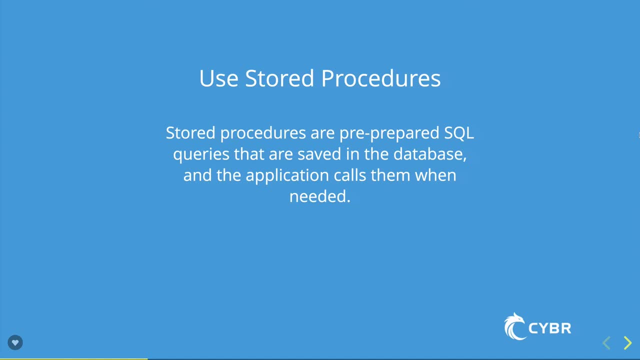 Now, another benefit of this approach is that SQL code stays within the application, so if you end up swapping out databases in the future, it's not going to be as easy to get back into the database. Next, we have stored procedures, And stored procedures are pre-prepared SQL queries that are saved in the database. 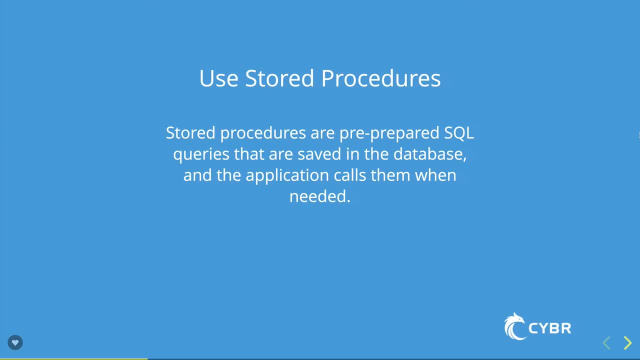 So if you need to pull a data feed from the database to display a news feed, for example, and you expect that action to happen fairly frequently, you could create a stored procedure and have the application call that procedure when it's needed, And you can build SQL statements with parameters that are automatically parameterized. so the 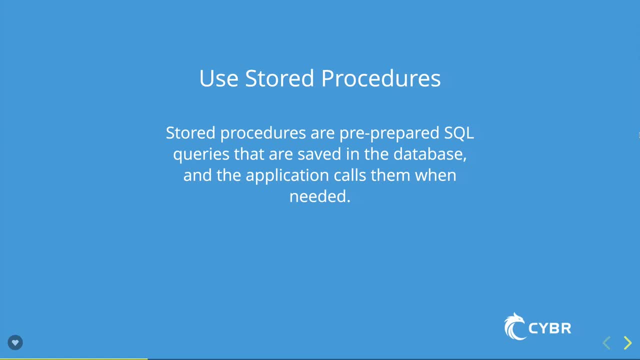 difference between this and prepared statements is that these are automatically parameterized. these are stored in the database itself and just called from the application, instead of being both constructed and called from the application. While you should aim to not use dynamic input in stored procedures, if you have to just 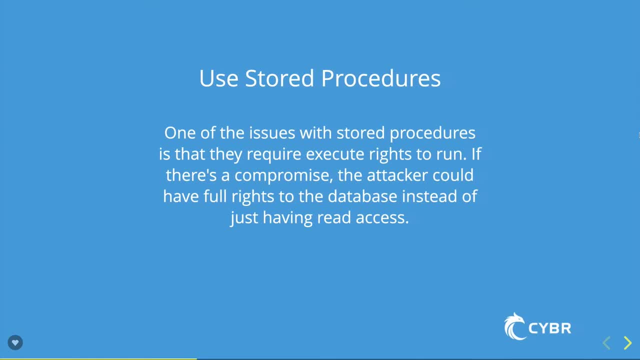 make sure that you properly validate and escape the input. Now, one of the issues introduced by stored procedures is that they require execute rights to run. This could mean that if there's a compromise, the attacker could have full rights to the database instead of just read access. 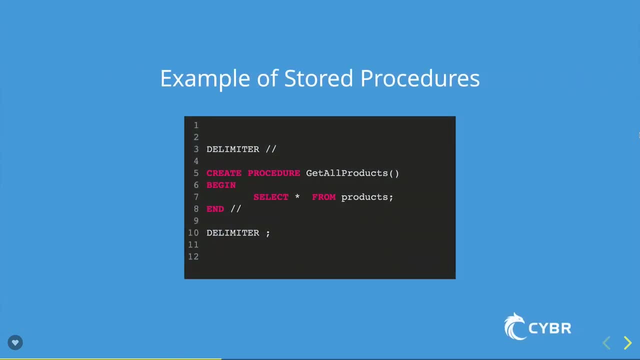 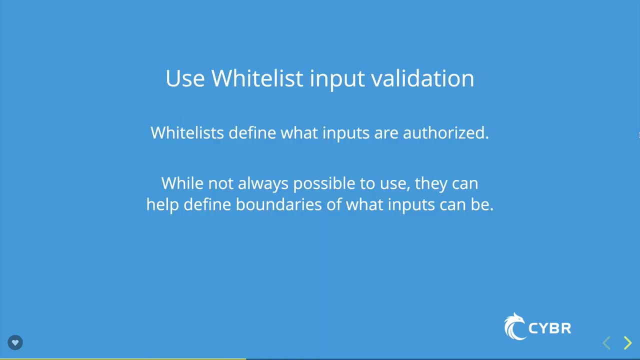 Here's an example of a stored procedure. In this case it's grabbing all of the products and we can call it with the getAllProducts stored procedure. The next security option we'll look at is using whitelist input validation. Whitelists simply define what inputs are authorized. 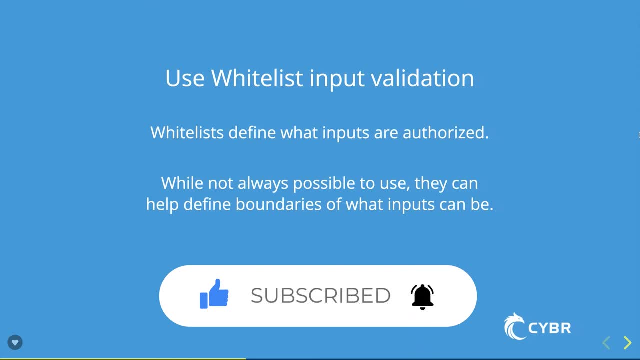 While this is not always possible, in cases where we know what a user inputted value should look like, we can set up whitelists of accepted inputs. The example used by OWASP is for table names. If we are expecting an input from the user that selects the database table name, we could 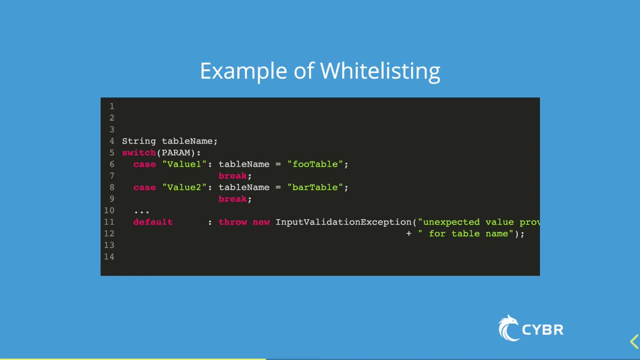 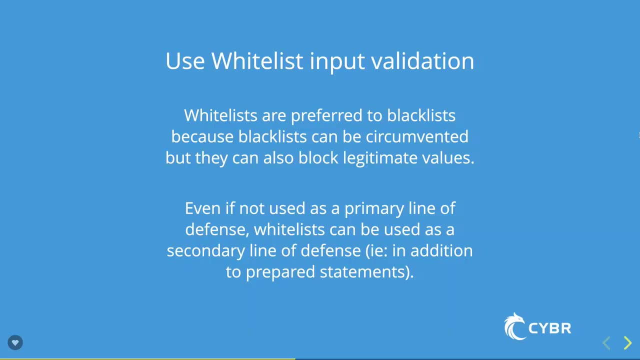 use a switch statement that checks the input for all potentially valid options. If it doesn't match those valid options, it simply throws an exception and rejects the input. Whitelists are preferred to blacklists because blacklists can not only be circumvented, but 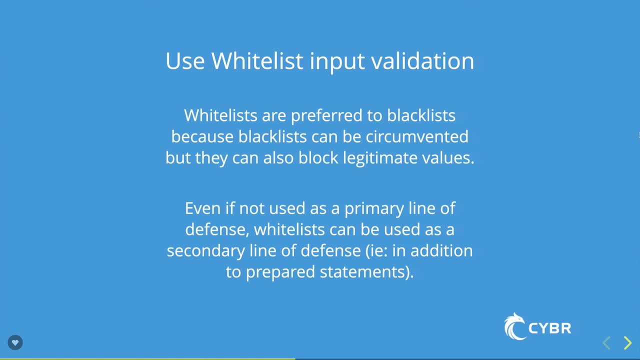 they can also block legitimate values. Whitelists are also described as a secondary line of defense, since they can be used as an alternative to binding variables when we can't implement that for whatever reason, But they can also be used to detect unauthorized input even before being passed to an SQL. 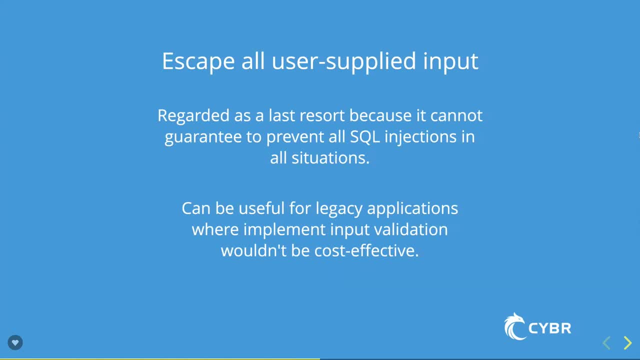 query that uses binded variables, Escaping user-supplied input is regarded as a last resort and when none of the prior options are possible to implement, because it cannot guarantee to prevent all SQL injections in all situations. A use case of this would be for legacy applications, where implementing input validation would 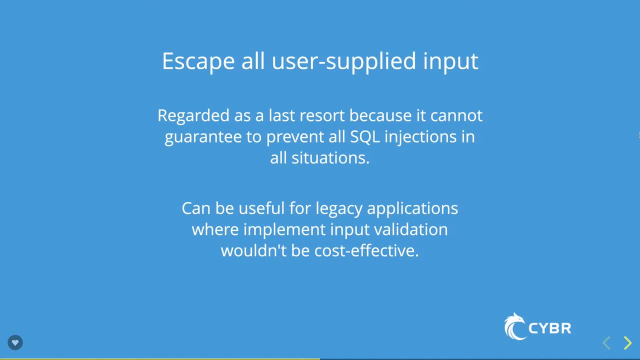 not be cost effective, And escaping is implemented a bit differently. There are libraries out there that can help with this. For these reasons, I won't be spending more time on this method of security, but feel free to reference the OWASP page if you'd like to learn more. 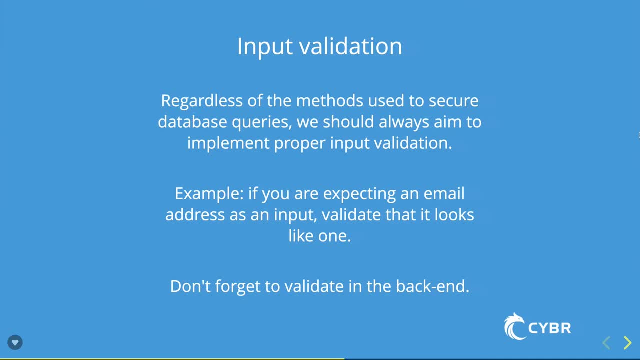 Now, regardless of the methods that we use to secure our database queries, we should always aim to implement proper input validation. Input validation by itself should not be considered as a foolproof security control, but it can help. For example, if you're expecting a user's email address, input validation would verify. 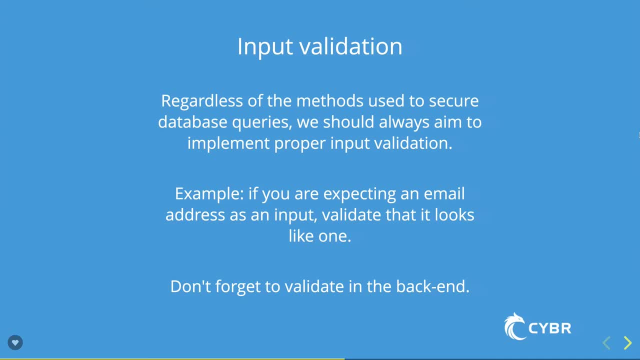 if it looks like an email or not, and if it doesn't, then it would simply reject the input before it even makes it to the database. For example, in the case of the OWASP juice shop, my single quote, or 1 equals 1 attack. 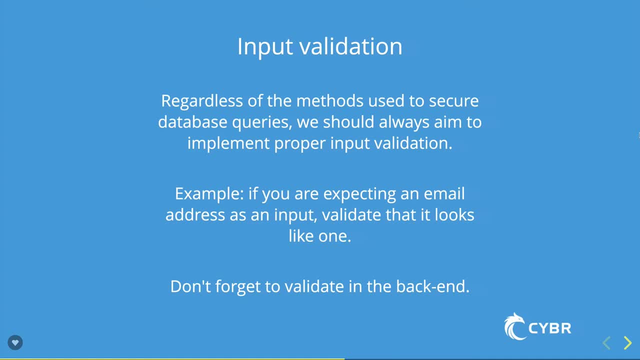 would have been prevented with input validation, since that clearly does not look like an email. A word of warning here is that front-end validation can be bypassed, as we saw, so we would also want back-end validation, And if you want more information on input validation, please check out this link. 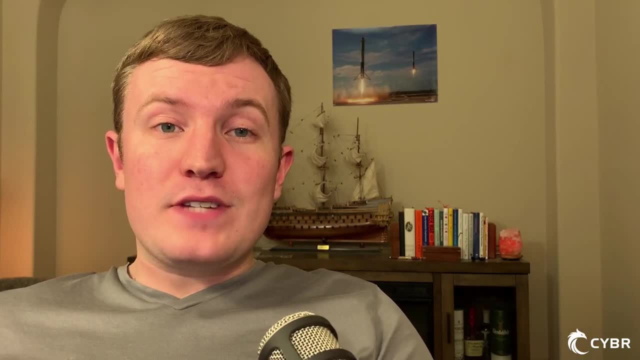 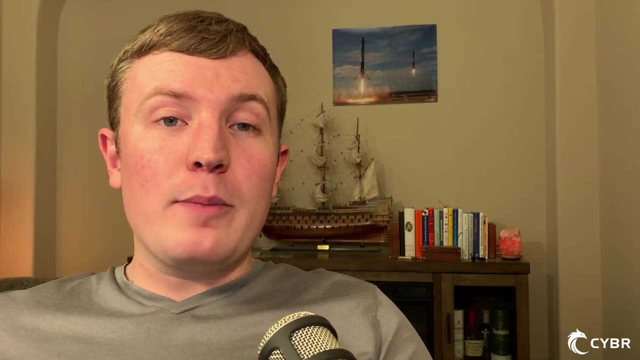 Now, everything we've talked about so far is great, But it won't make a difference if we don't implement it properly. So, as we develop our applications, it is important that we review database calls and how our application handles user inputs before we deploy code to production. 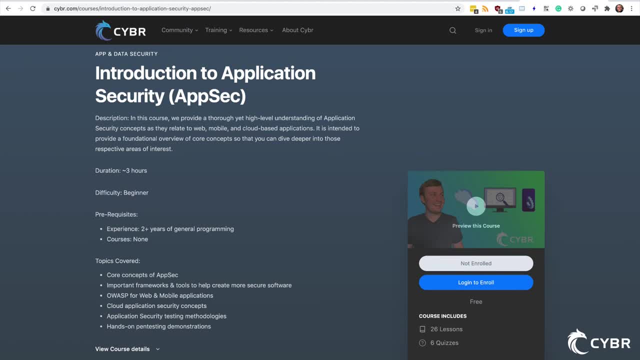 We covered this concept in our Introduction to Application Security course, but pentesting should be used as one of the last resorts. Ideally, we would catch these security issues when reviewing code either written by ourselves or by our peers. Now developing an eye for issues in code is very important. 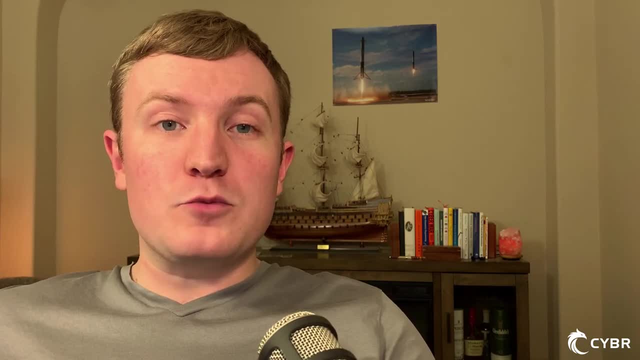 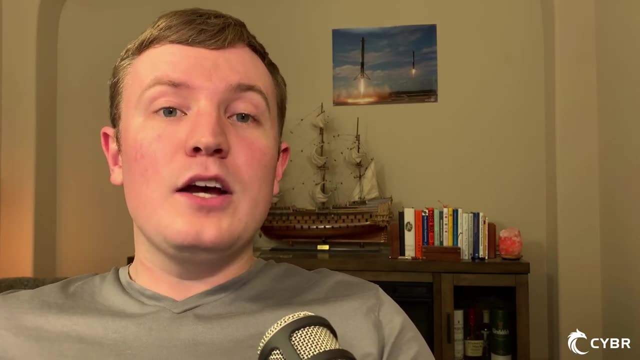 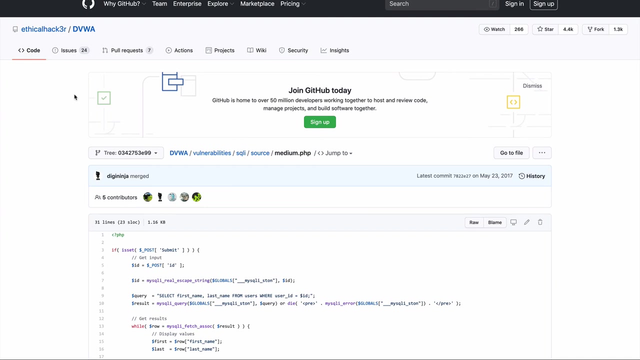 So, with that in mind, Let's pull up the GitHub repos for the OWASP juice shop and DVWA so that we can look at the issues in the code and then look at defenses that we could apply to protect against SQL injections. Remember, anytime you see inputs being grabbed directly from the user and executed without 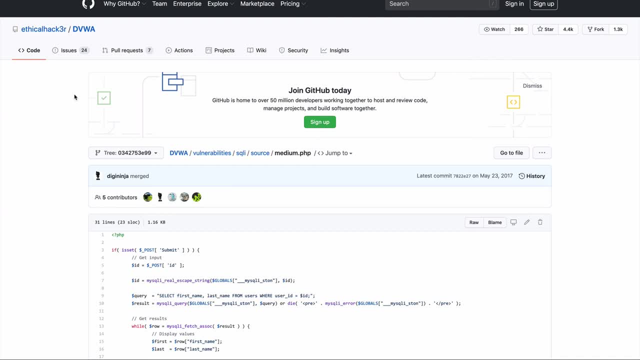 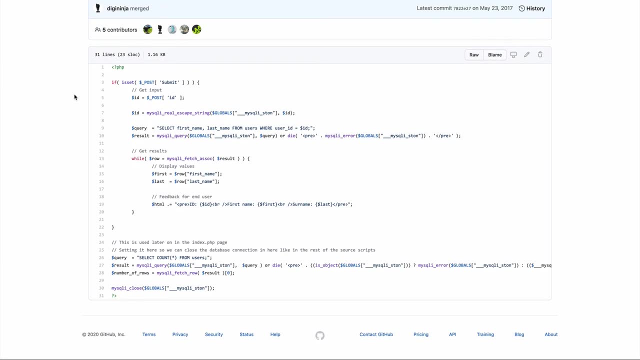 anything else, cleaning those inputs in between. you should have a massive red flag pop up in your head. Now, looking at the DAM Vulnerable Web Application medium security level for the SQL injection vulnerability that we were able to inject in a prior lesson. this is what the code looks like In this case. 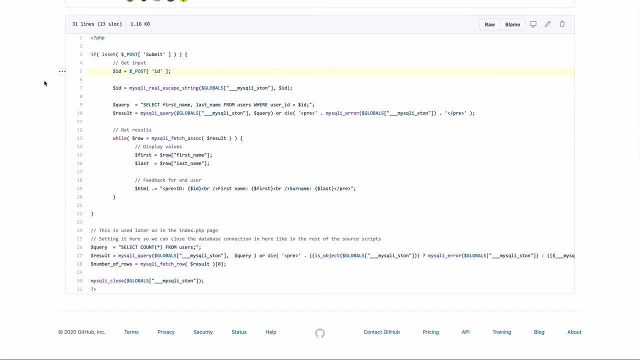 on line 5 we grab the id from the input submitted. Then on line 7 we use the mysqli real escape string which takes the current character set of the connection in this globals variable and then escapes the id. Then the query is prepared on line 9 with the id directly injected in and then the 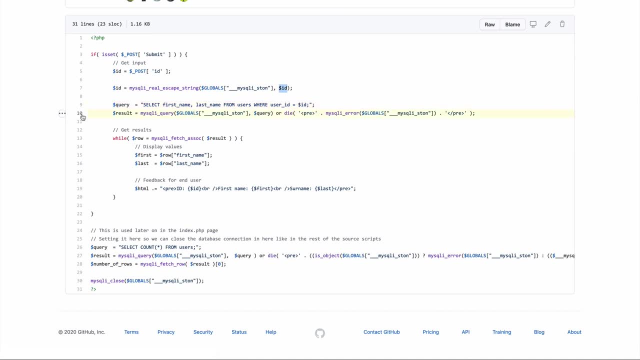 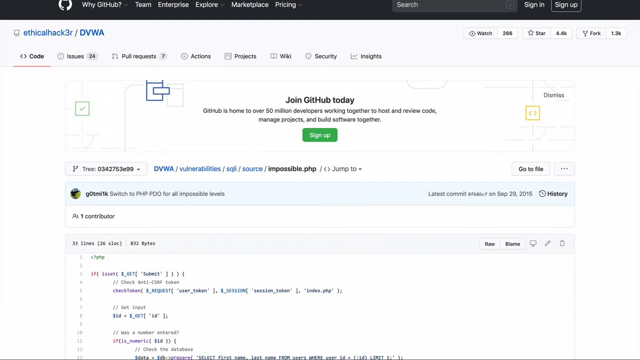 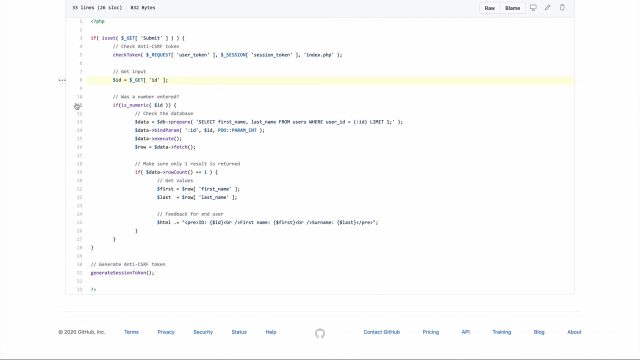 query itself is executed on line 10.. So, as we mentioned before and as is showcased here, escaping inputs by itself is not sufficient. If, instead, we look at the impossible version of this code, we will see the proper security controls. We grab the id on line 8, just like. 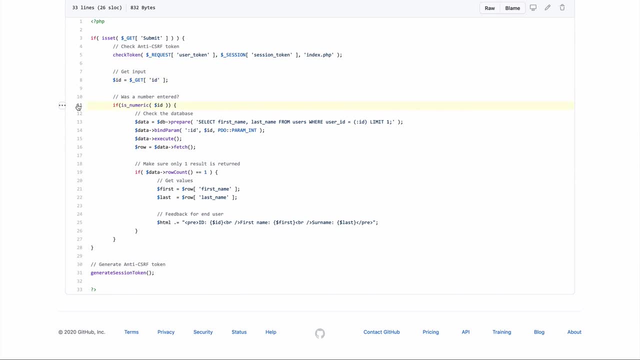 we did in the prior one, but then we perform input validation, since the id should be a numeric value. We then use a prepared statement with parameterized query where we prepare the sqli real escape string which takes the current character set of the connection in and then. 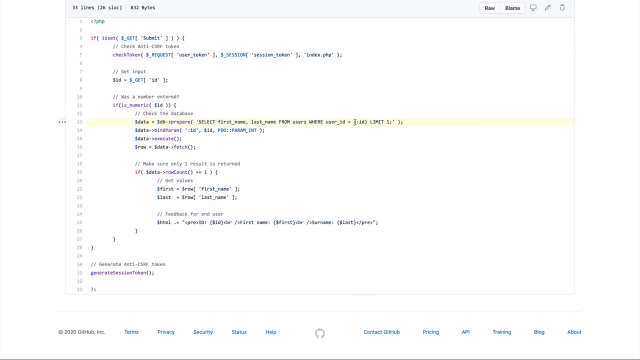 sets placeholders for our inputs. In this case we just have one input, which is the id. We also set a limit of 1 for the results, so that we only return a single row. We then bind those parameters with the bind param method on line 14, which binds a variable to its corresponding variable in the 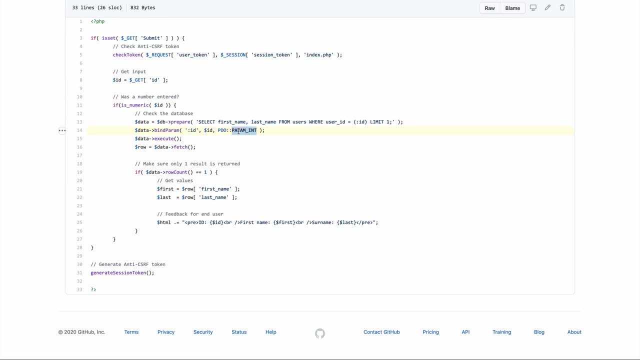 prepared statement and we specify the data type with pdo param int to set it as an integer data type, And then, finally, we execute that query On line 18 and 19. we again make sure that only one row was returned, since there are sqlinjections that could comment out the limit 1 option. 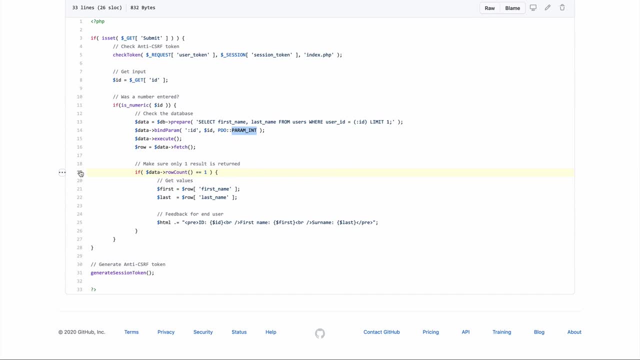 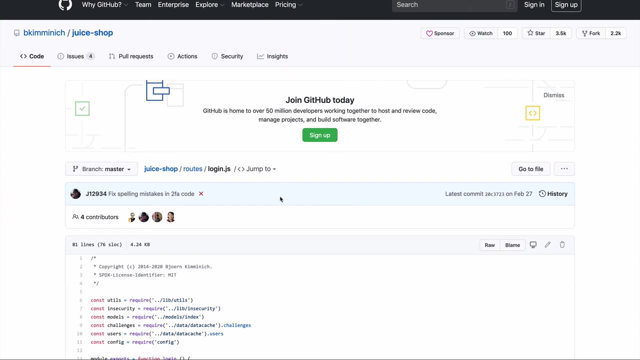 in which case we want to prevent the response from making it back to the requester. Now let's take a quick look at the OWASP juice shop login code to identify the issue that allowed us to perform an sqli injection before moving on. So here's the code. here We can see that we can see. 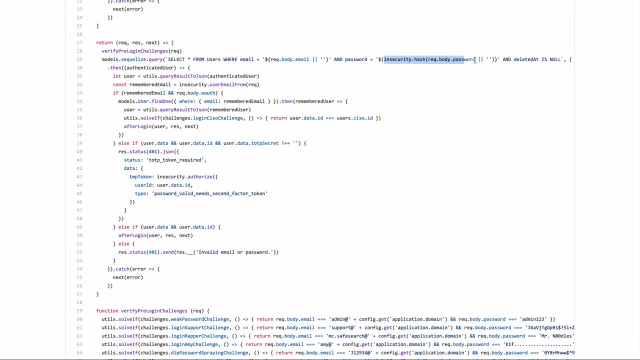 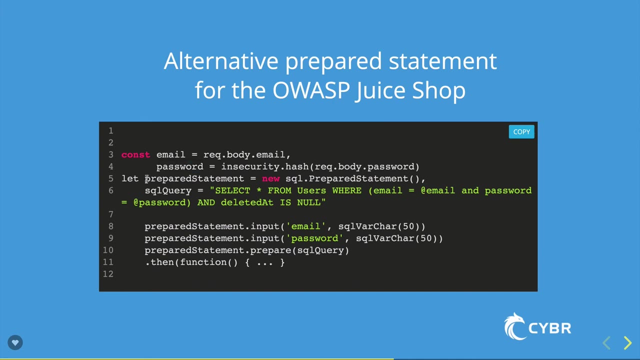 that the email and the password are directly grabbed from the user, submitted input and injected directly in the database, with nothing in between. Instead, we could do something like this, where we grab the email, we grab the password and then we create a prepared statement, We set placeholders. 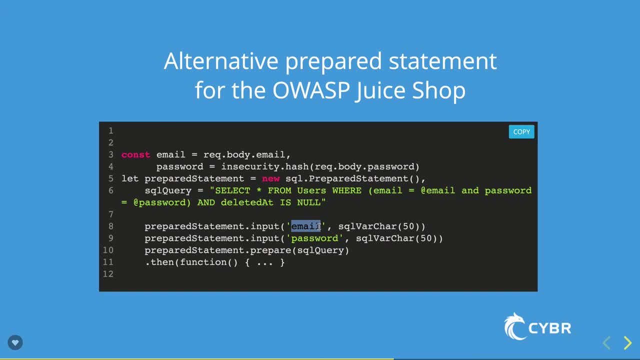 for the email and password. we add those email and passwords to those placeholders checking for their checking that they match our expectation in terms of data type and also in terms of length, and then we execute the query itself. Now we could also add additional checks, like making sure that only one record was returned. 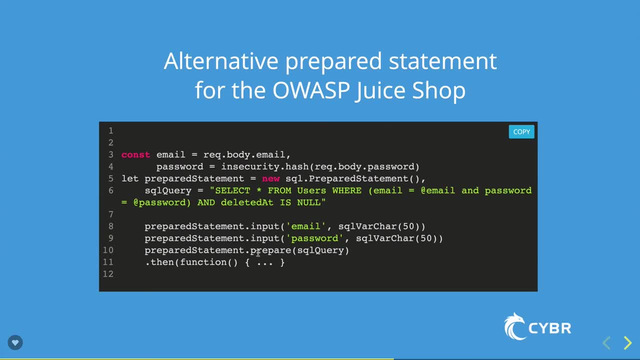 and that the email was properly formatted, etc. Also, this is untested code and just a proof of concept, but we are again using placeholders for the email and password and using a prepared statement, Now that we're aware of security controls that we can use- and we've seen examples. 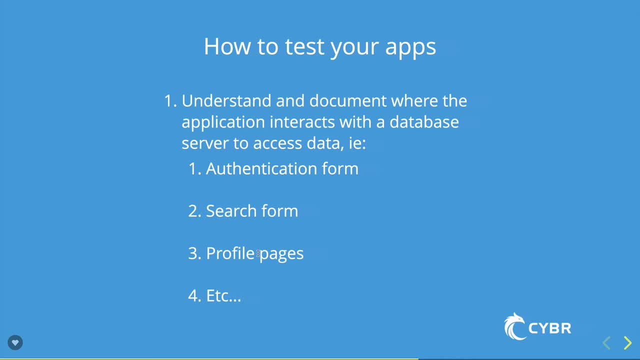 of insecure as well as secure code. let's wrap up this lesson by talking about how to test our own apps and their security. Thanks for watching and I'll see you in the next video for SQL injection, especially since our apps are likely to have multiple locations. 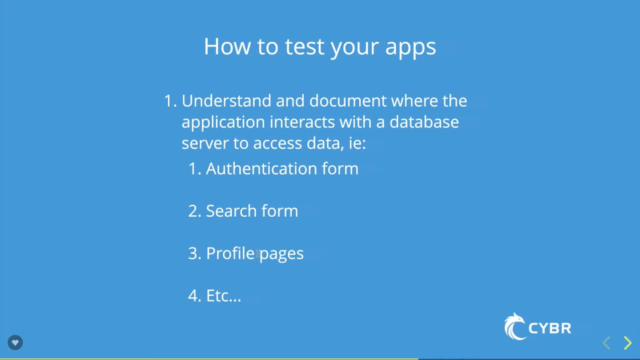 that could be vulnerable to SQL injections. Now, one of the first steps that we can take is to understand and document where our application interacts with a database server in order to access data, And this could be an authentication form, a search form, profile pages, etc. We then need to make a list of all input fields whose values could be used. 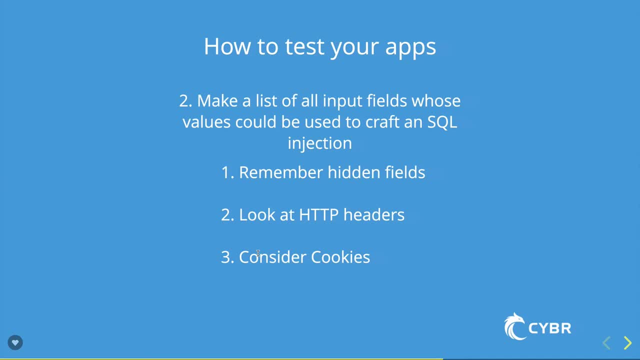 to craft an SQL injection- And here it's important to remember any hidden fields, HTTP headers and cookies- Then we can not only manually test via methods that we've learned, but we can also use fuzzers and automated tools like SQL Map to look for any signs of weakness. 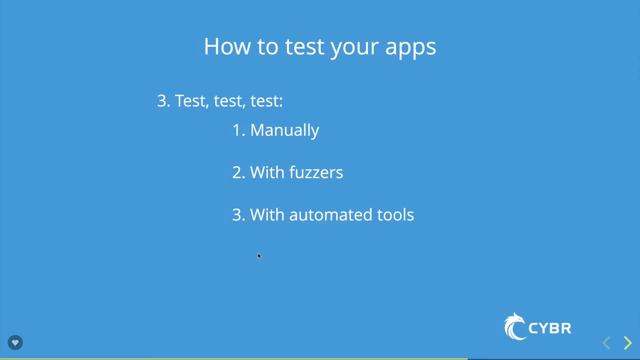 We can then monitor responses from the server, look at the source code being returned for any information leakage and keep an eye out for any unexpected or changes in behavior. And to help with this, I also recommend that you create abuse cases. A bit of a twist here is that if you have an abuse case, you can create an abuse case. 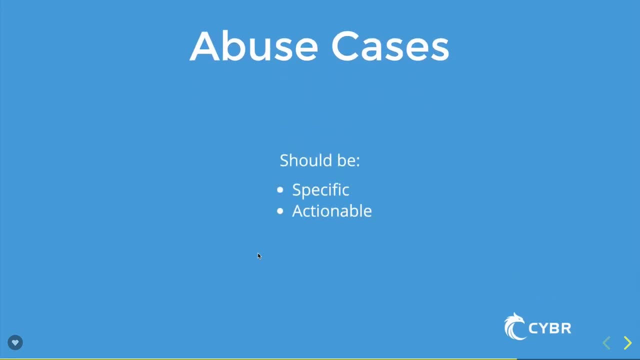 where you can create an abuse case. where you can create an abuse case. where you can create an abuse case. Abuse cases should not be generic. Instead, they should be specific and actionable. If you are running an agile project, the definition of abuse cases should be made. 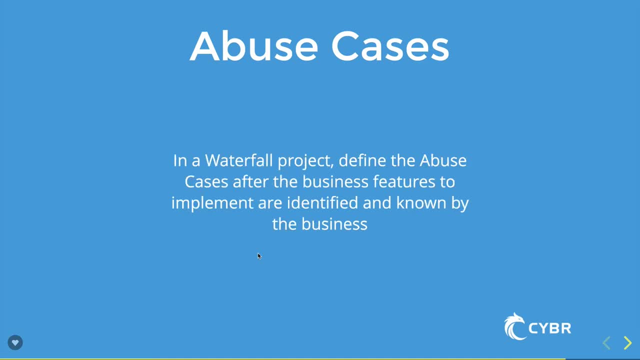 after your user stories are included in a sprint In waterfall projects, they should be made when the business features to implement are identified and known by the business. Then the abuse cases become security requirements in each feature specification section or user story acceptance criteria In an example abuse case: 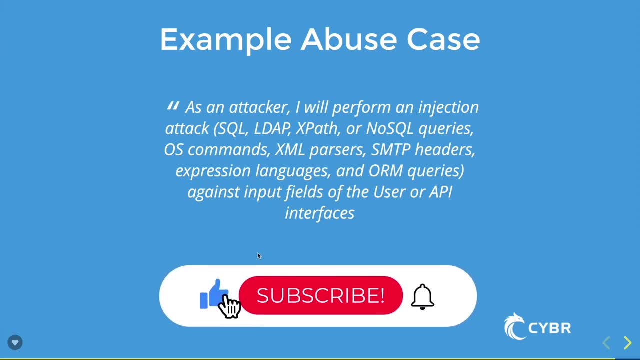 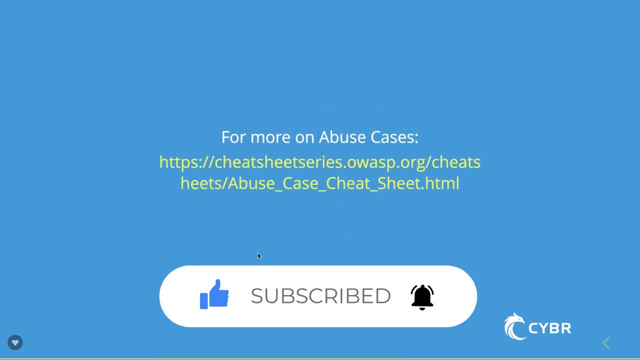 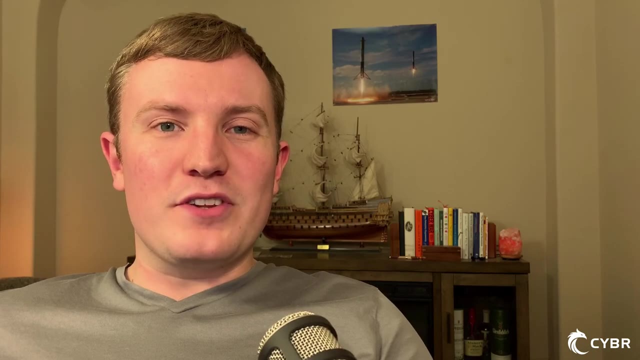 this might be the case. As an attacker, I will perform an injection attack against input fields of the user or API interfaces. For more information on abuse cases, definitely check out this cheat sheet Now. that concludes this lesson on defenses for the application layer. let's complete this lesson and move on to the next. 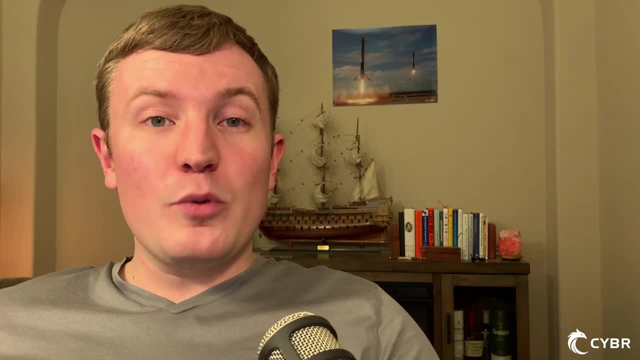 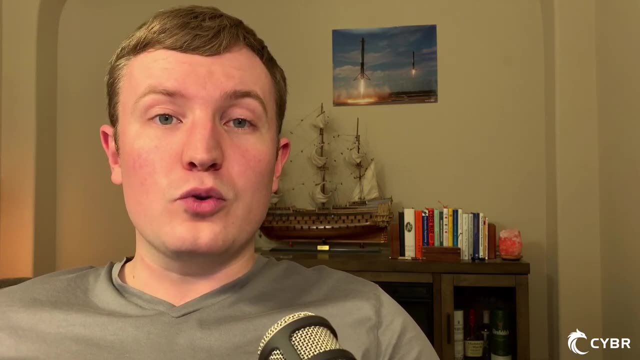 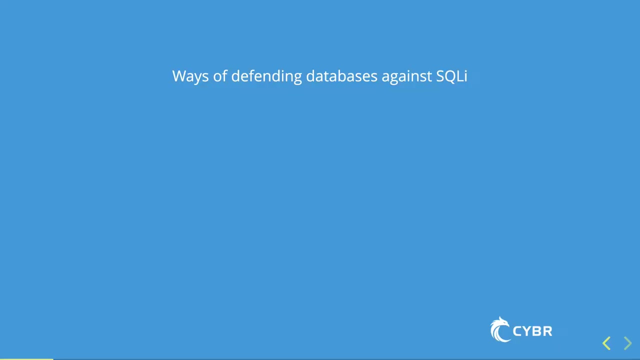 Just like we need to build our applications with the assumption that they will be under SQL Injection Attack, we need to construct our databases with the same mindset and assume that not all of the security controls are protected. We need to think about minimizing privileges of database accounts. 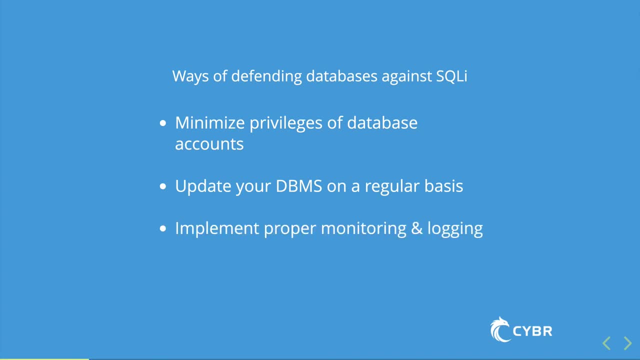 updating our DBMS on a regular basis, implementing proper monitoring and logging, and we also need to know that no SQL databases can be vulnerable to injections, even if we haven't talked about them yet. So, when your application runs SQL queries, it does this by assuming the privileges of a user that was selected by the user. So when you run SQL queries, you need to assume the privileges of a user that was selected by the user. So when you run SQL queries, you need to assume the privileges of a user that was selected by the user. 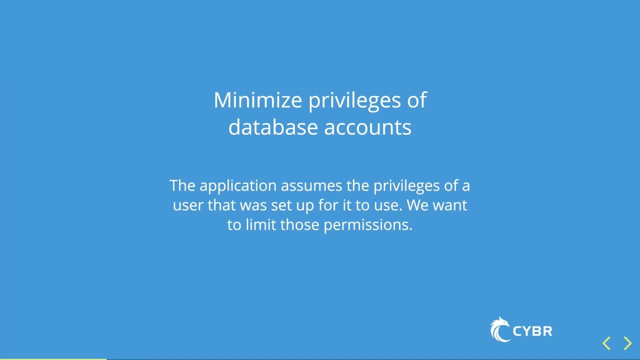 So when you run SQL queries, you need to assume the privileges of a user. that was selected by the user, And a lot of times it's much easier to configure an administrative user for that purpose, since we don't have to mess with permissions. But this is a mistake. 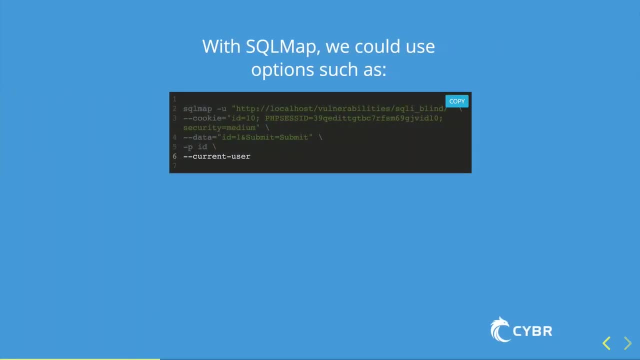 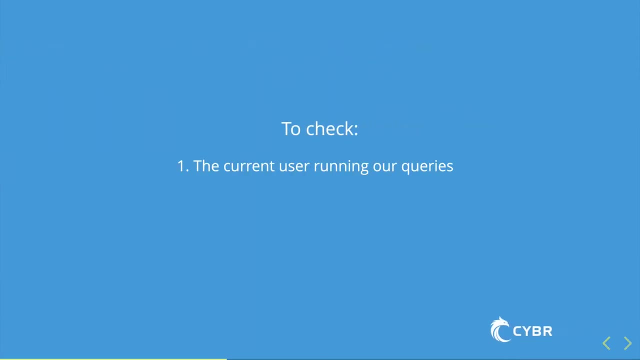 In the lessons where we used SQLMap to compromise a database, we could use options such as CurrentUser and IsDBA, which would have allowed us to check the current user running our queries and whether that user has administrative privileges, And if we had access to an admin account, we could have done. 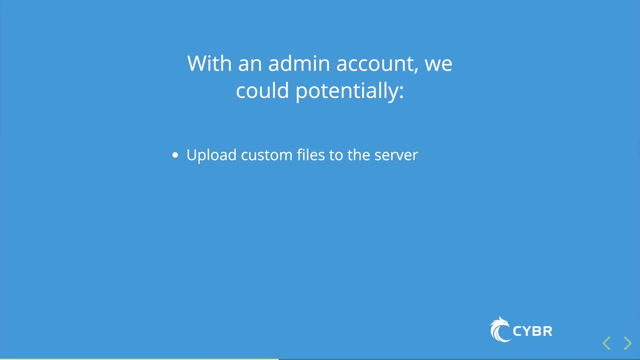 far more damage, including a lot more damage to our database, Including potentially uploading custom files on the server, creating or deleting other database accounts, creating, running or deleting stored procedures and more So. by limiting privileges and even creating different users for different web applications, we can limit how much damage. 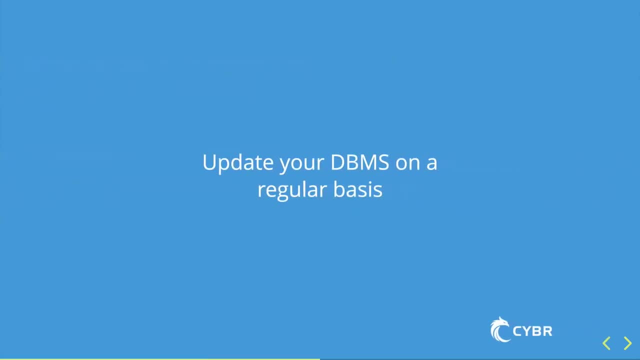 successful attacks can do. Now, of course, this list would not be complete without mentioning updates to our DBMS. I know updates can be a pain, but they are an important part of maintaining secure systems, especially when the updates to our DBMS are not complete. I know updates can be a 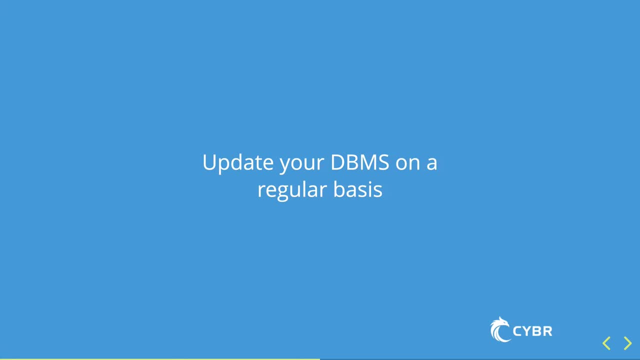 pain, but they are an important part of maintaining secure systems, especially when the updates to US cryptocurrencies can be done quite effectively And within that first 7-8 day cycle, you basically just tell your DBMS structure that it made, certo, the same stuff, but you 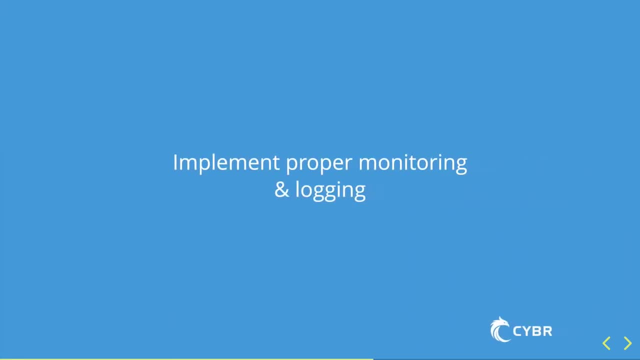 don't have to do over-defining to fix the bugs. One other critical piece in keeping databases secure is implementing proper monitoring and logging. For example, errors should be logged all the way from sql errors to database administration errors, For example, failed login attempts. 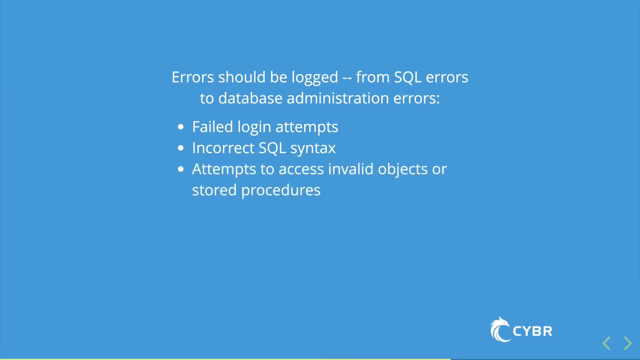 incorrect SQL syntax, attempts to access invalid objects or stored procedures out of range, errors such as when trying union attacks and errors involving permissions of any kind, errors involving extensions like sendmail command, shell and others. We also need to look at certain data. 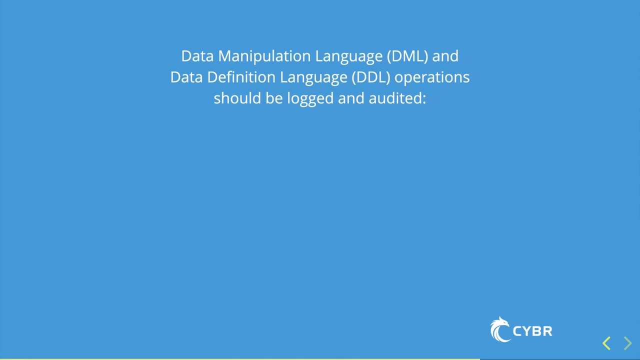 manipulation, language or data definition language operations, and those should be logged and audited. For example, we've got password changes. that should be logged and monitored. we have login attempts, logout attempts, database operations and permission changes. We can also set thresholds. 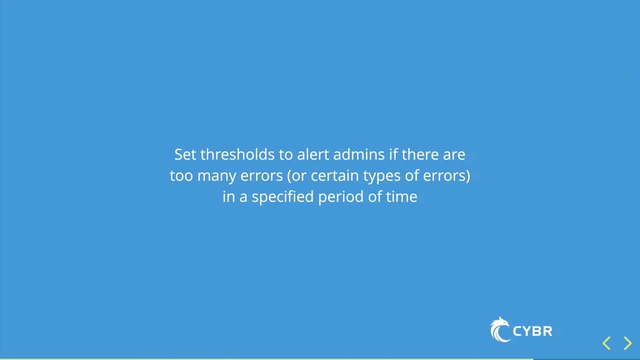 so that if too many errors or certain types of errors happen in a specific time window, it alerts someone to take a look, Because unless you haven't thoroughly tested your system, there should not be very many errors happening from application requests. So if there is an uptick in errors all of a sudden, it's definitely something that you should. 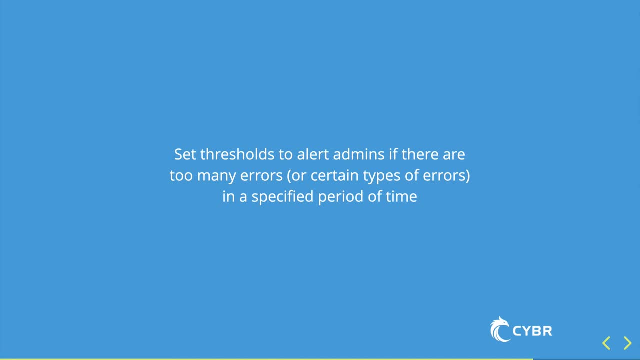 look at And, of course, implementing logging and monitoring does depend on your system, whether you're on-prem or not. Now I had to throw this one in here, because while we focused on SQL injections with SQL database engines, NoSQL is also vulnerable to injections. It used to be a 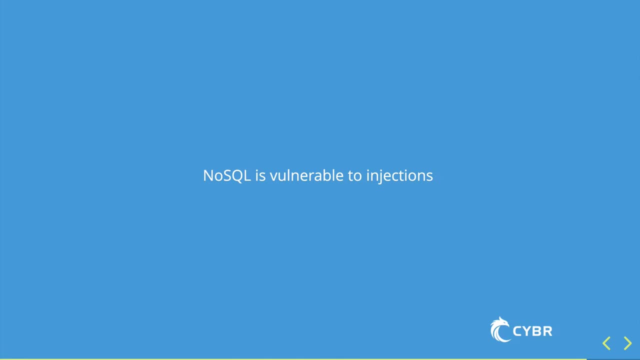 common belief that NoSQL was not vulnerable to injections, but that's been proven wrong time and time again. So if you're running NoSQL databases, don't think they can just skip on security controls, even if they look a little bit different. And if you'd like more information on securing and hardening, as well as